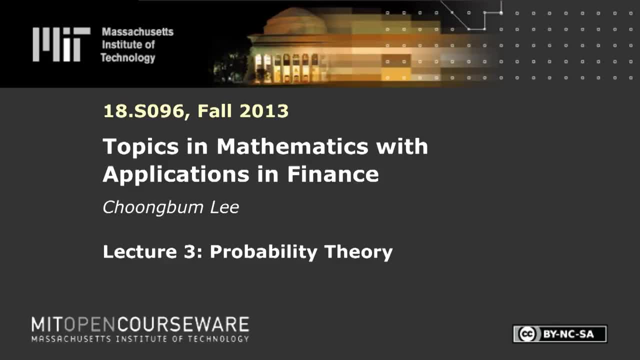 The following content is provided under a Creative Commons license. Your support will help MIT OpenCourseWare continue to offer high-quality educational resources for free. To make a donation or view additional materials from hundreds of MIT courses, visit MIT OpenCourseWare at ocwmitedu. 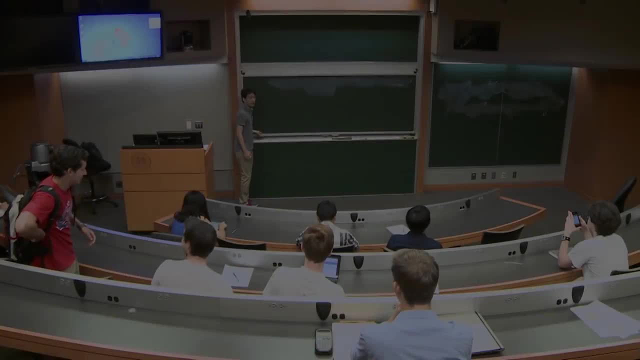 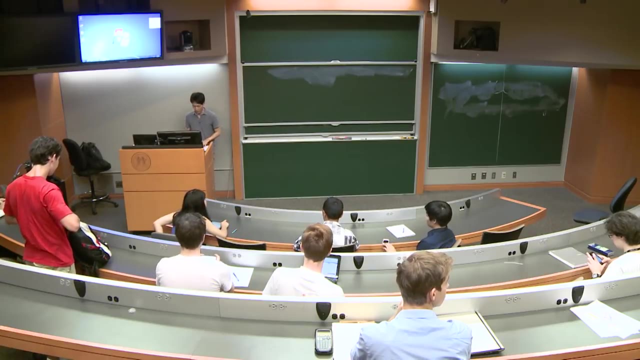 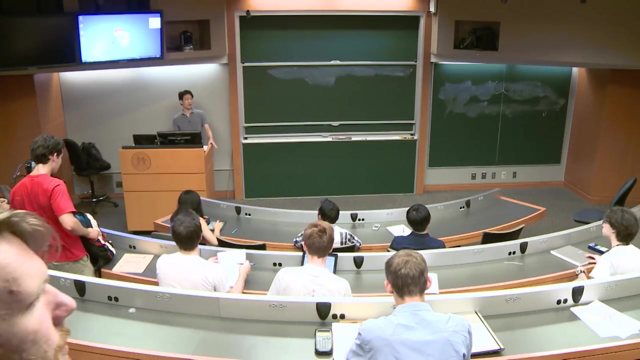 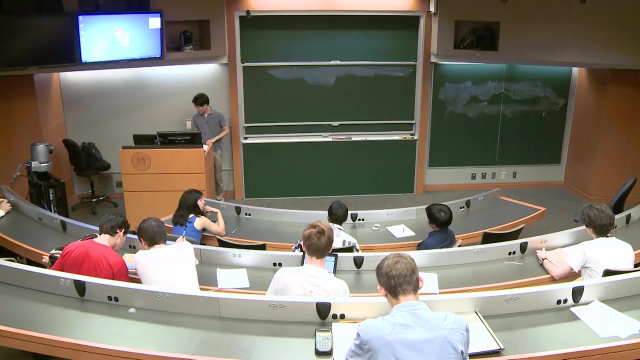 Okay, so good afternoon, And today I will. we will review probability theory, So I'll mostly focus on- I'll give you some distributions, so probabilistic distributions that will be of interest to us throughout the course, And then I will talk about moment-generating functional. 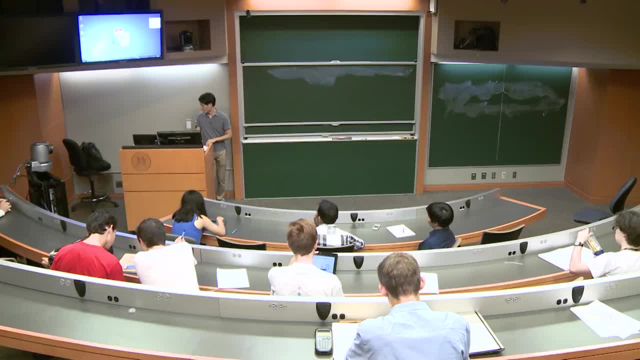 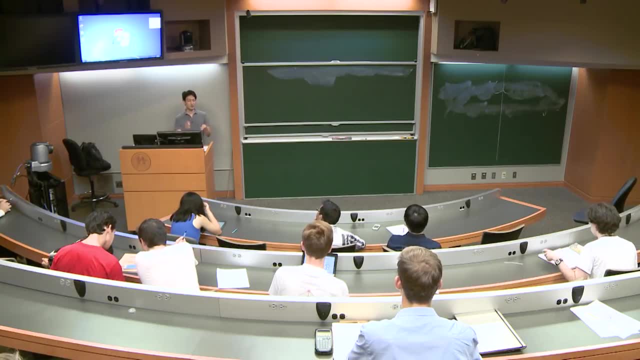 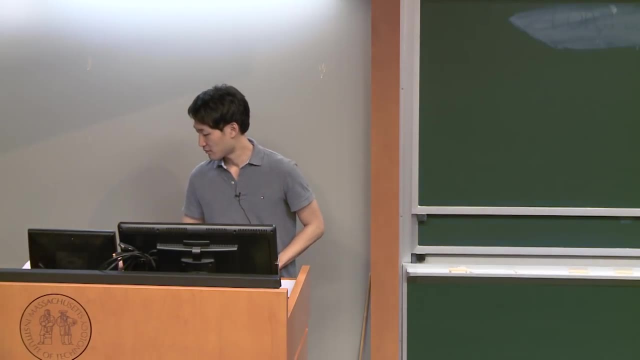 a little bit Afterwards. I will talk about probability, Okay, about Law of Large Numbers and Central Limit Theorem. So who heard of all of these topics before? OK, that's good. Then I will try to focus more on a little bit more. 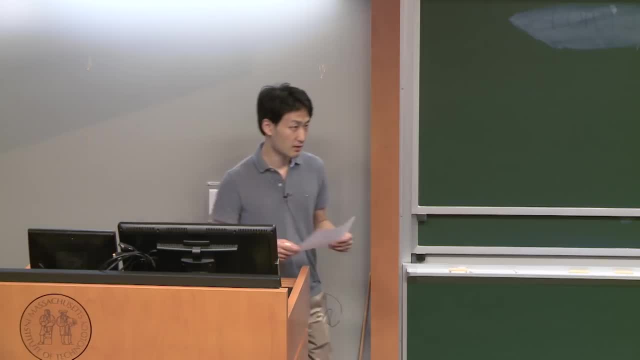 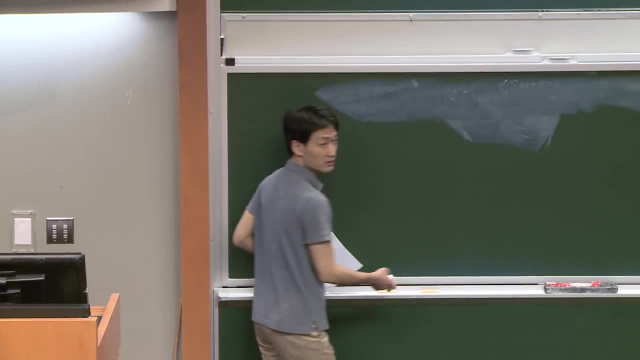 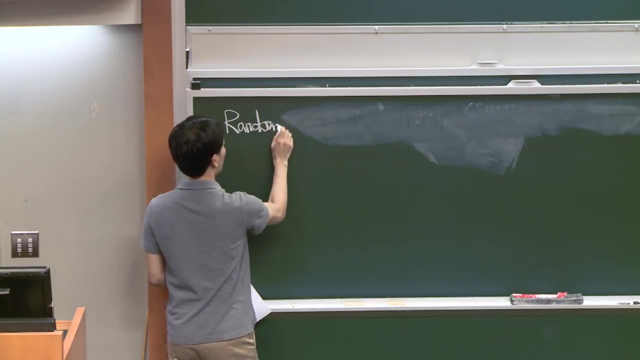 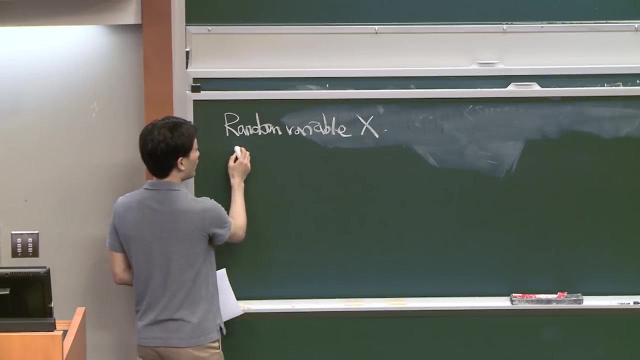 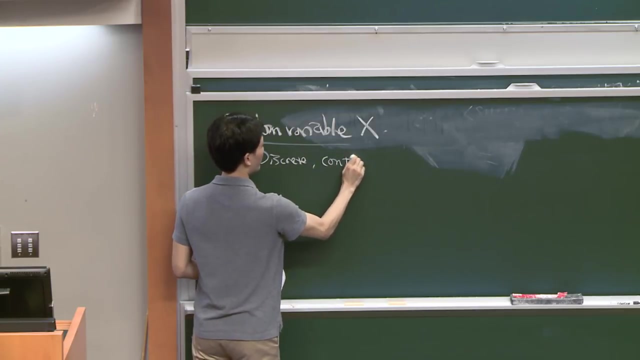 advanced stuff, But yeah, then a big part of it will be a review for you. So first of all, just to agree on terminology, let's review some definitions. So a random variable X. So we will talk about discrete and continuous random variables. 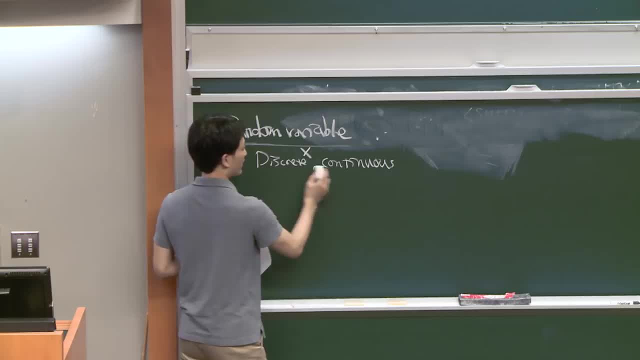 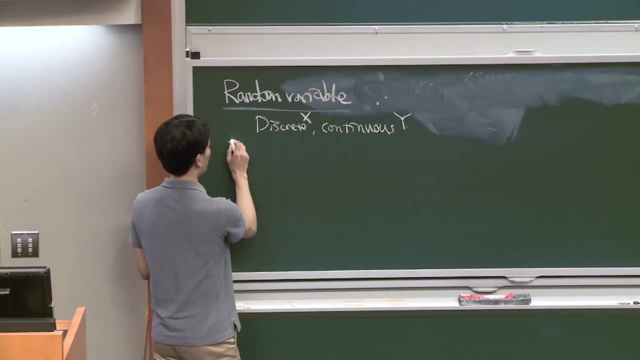 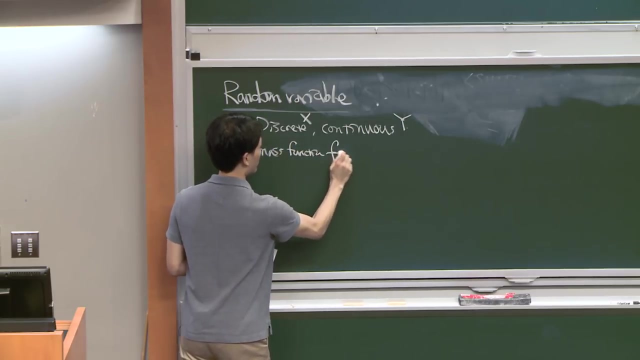 Just to set up the notation, I will write: discrete at X and continuous. This random variable is Y for now. So they are given by its probability distribution. Discrete random variable is given by its probability mass function F sub X. I will denote. 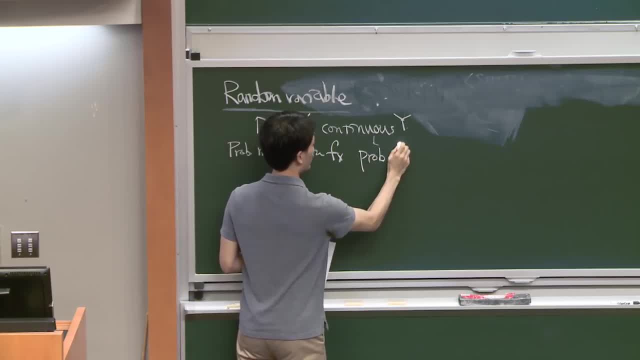 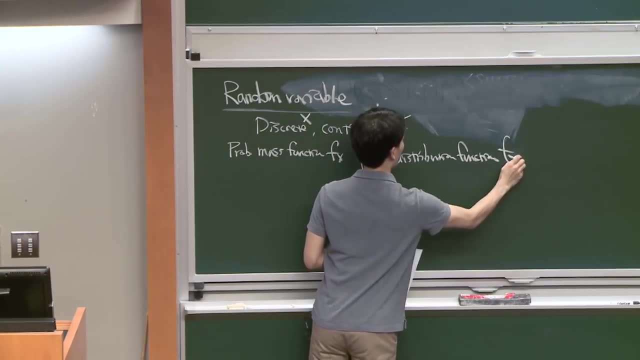 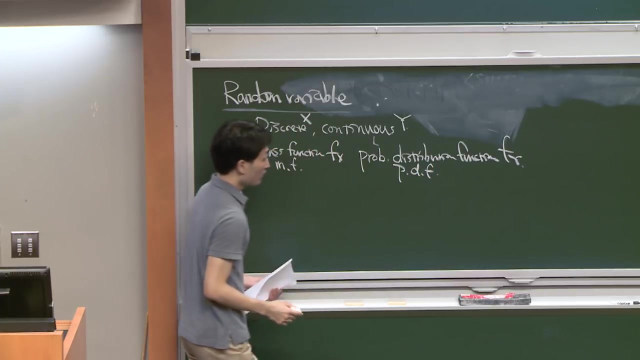 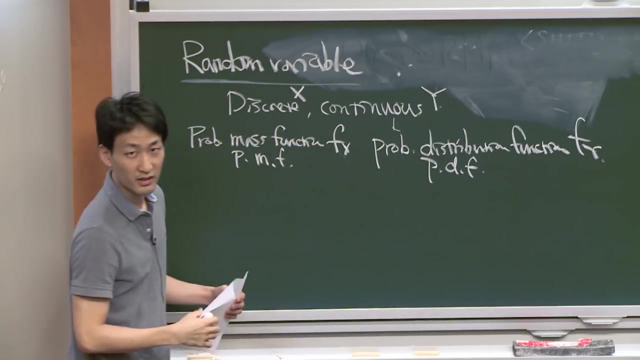 And continuous is given by probability distribution function. I will denote by F sub Y. So PMF and PDF I mean here I just use a subscript because I want to distinguish F sub X and F sub Y, But when it's clear which random variable we're talking about, 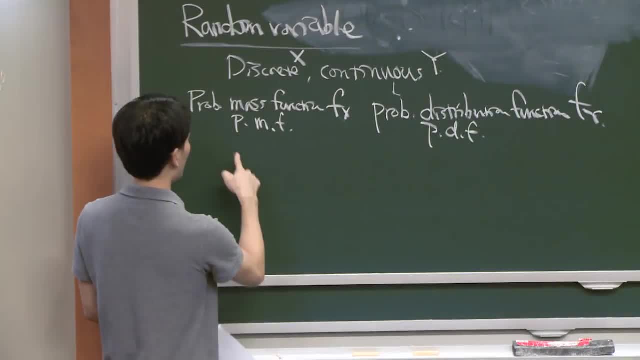 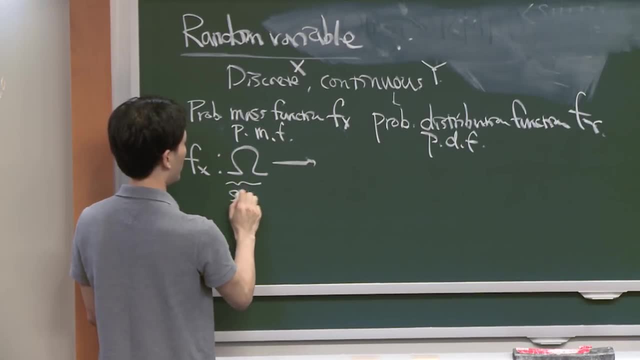 I'll just say F. So what is this? A probability mass function is a function from the sample space to non-negative reals, such that the sum, which is the sum, the number of reals, is equal to 0.. So you have the sum. 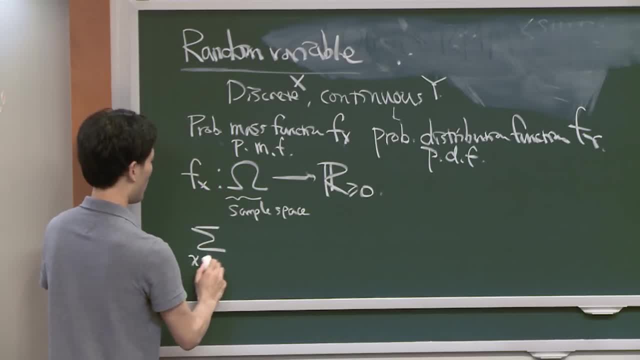 You have the problem, You have the dimension, You have the function, You have the function, You have the function, And then you have the function, You have the function, You have the function. over all points in the domain equals 1.. 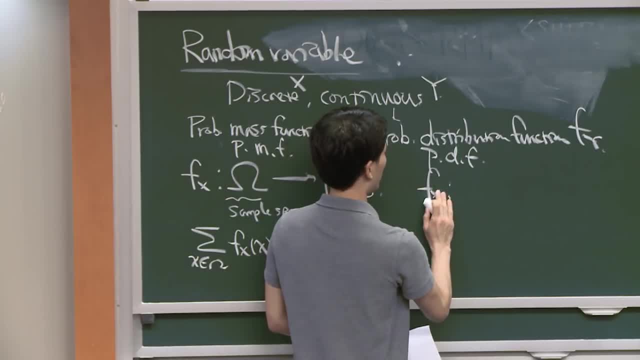 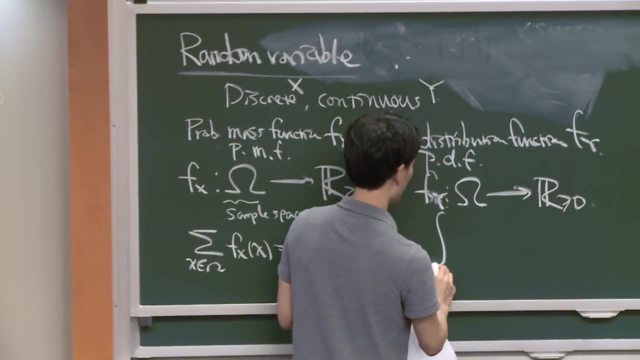 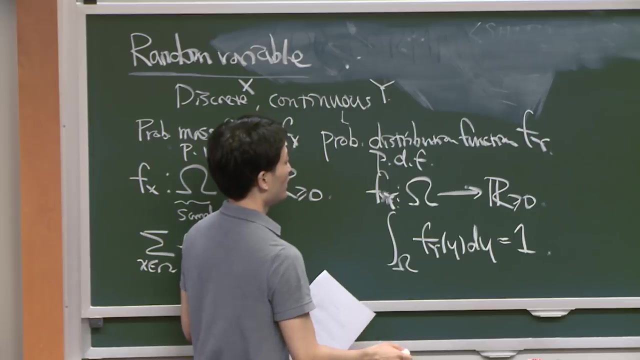 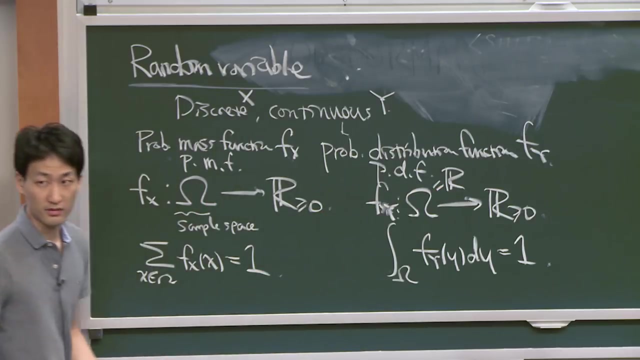 The probability distribution is very similar, The function from the sample space non-negative reals, But now the integration over the domain is equal to 1. So it's pretty much safe to consider our sample space to be the real numbers for continuous random variables. 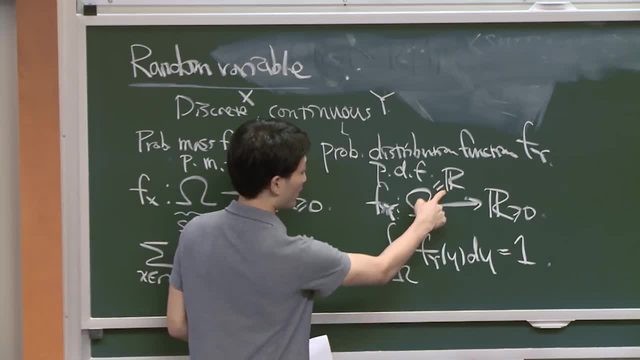 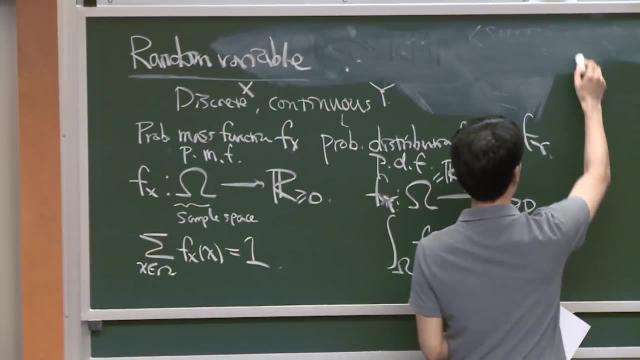 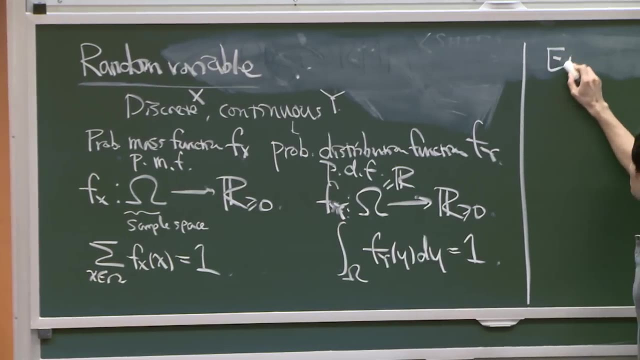 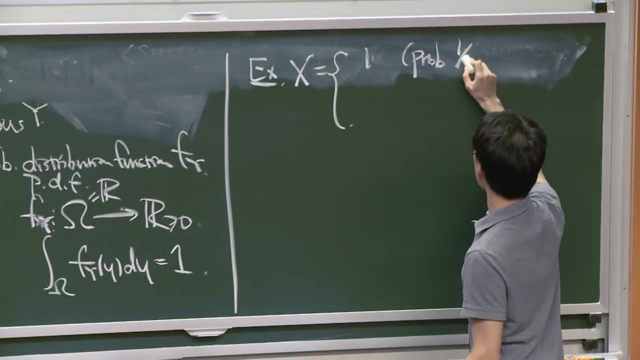 Later in the course you will see some examples where it's not the real numbers, But for now just consider it as real numbers. And then so, for example, probability mass function: if x takes 1 with probability 1. third, 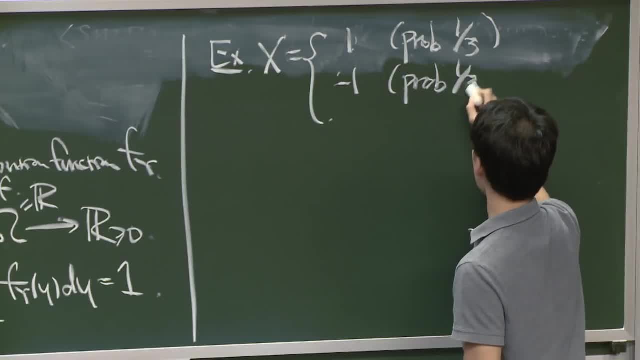 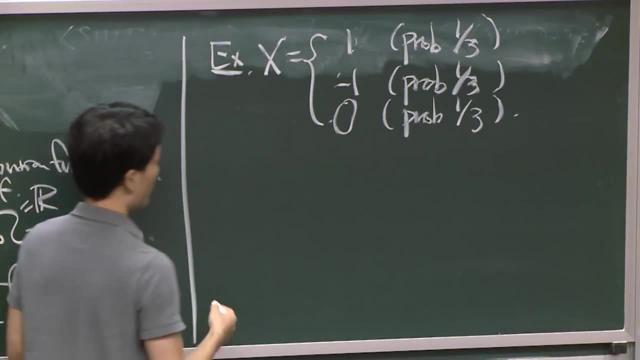 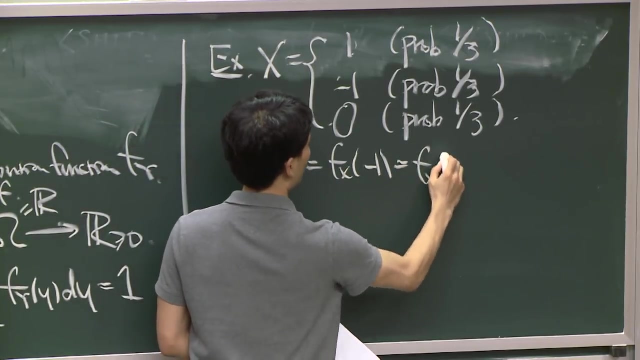 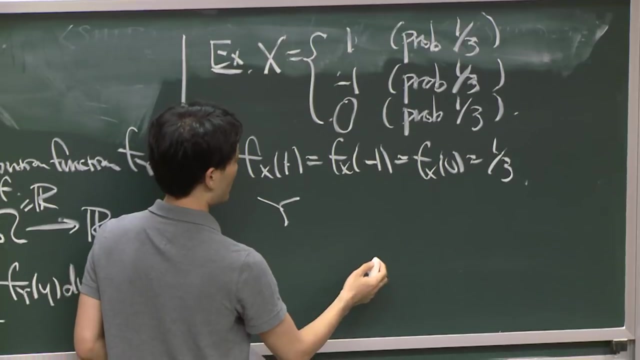 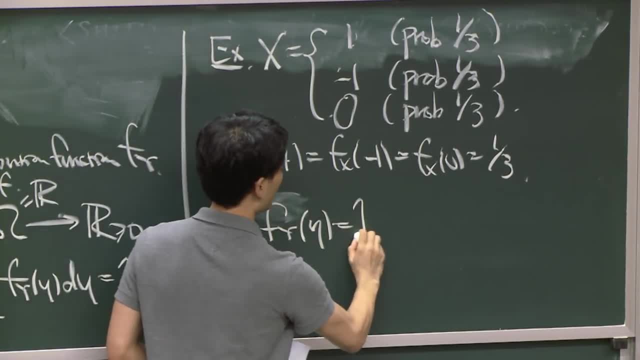 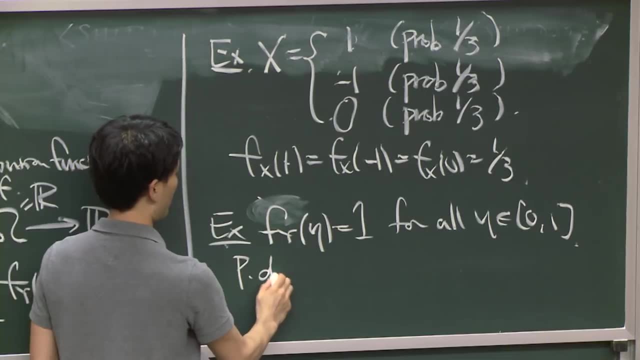 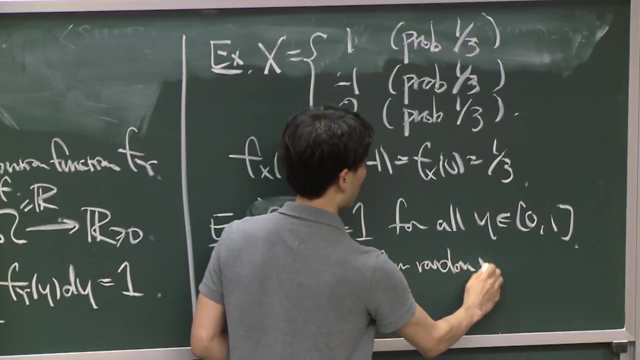 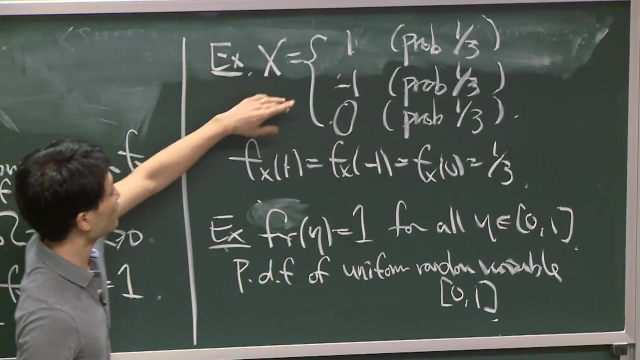 1, then f sub y is equal to 1 for all y in 0, 1.. Then this is PDF of uniform random variable where the space is 0. So this random variable just picks one out of those three numbers with equal probability. 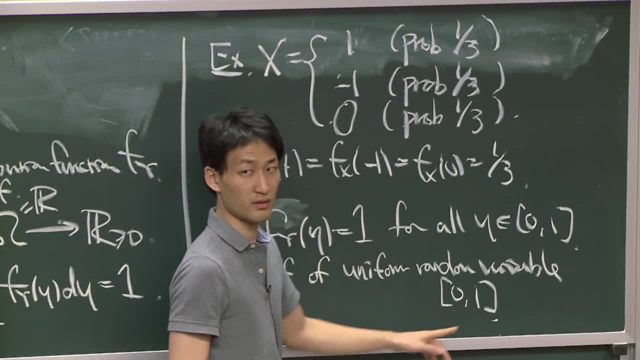 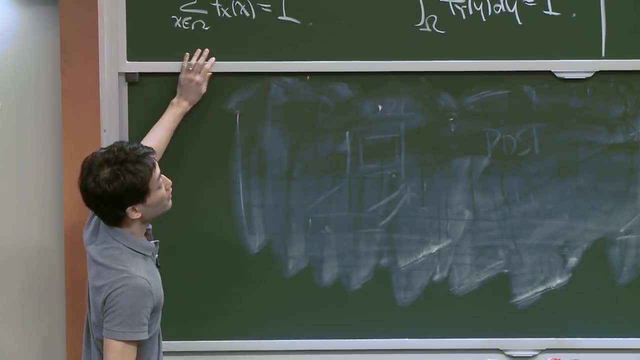 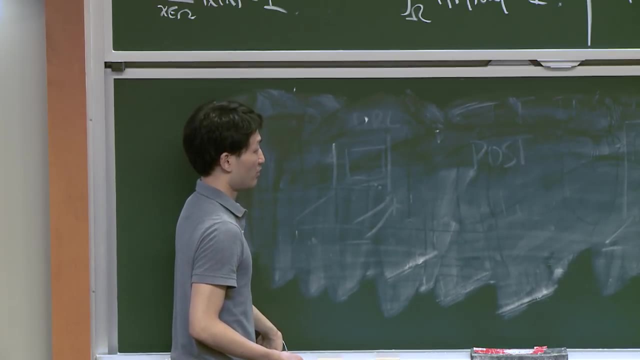 This picks one out of this: All the real numbers between 0 and 1 with equal probability. These are just some basic stuff. You should be familiar with this, but I wrote it down just so that we agree on notation. OK, both of the points now slide. 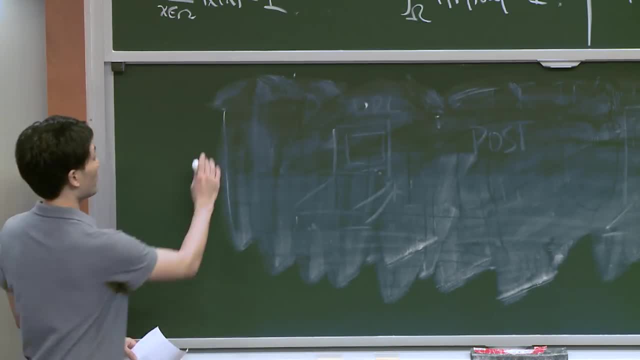 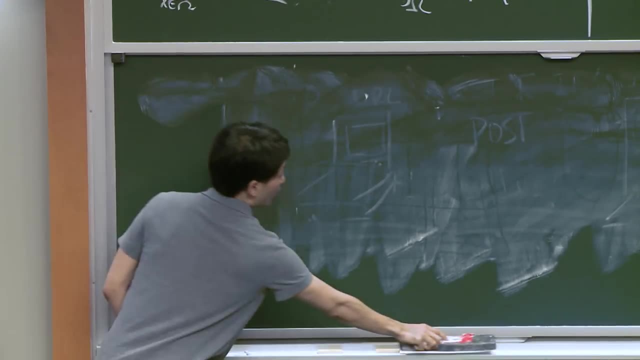 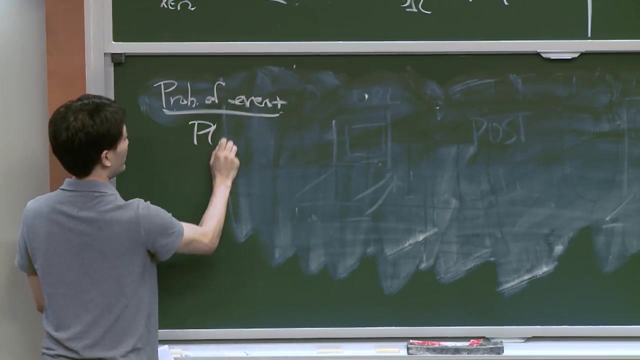 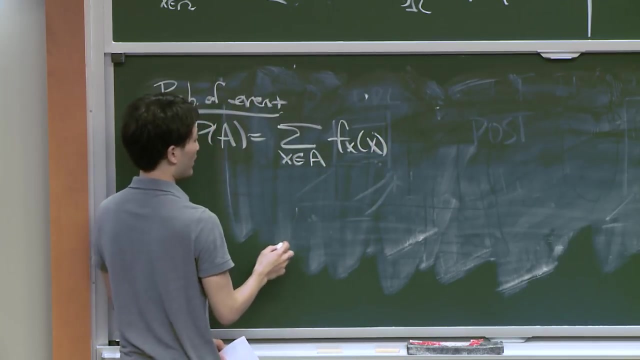 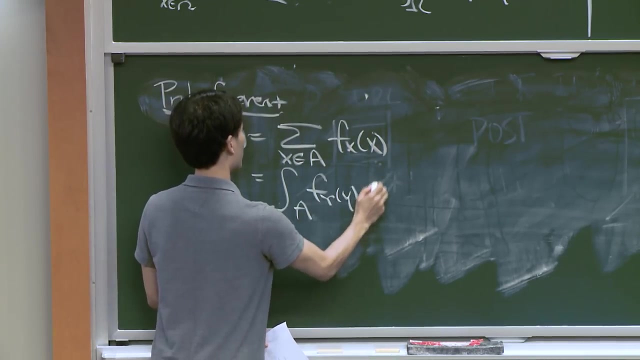 That's good. A few more stuff. Expectation Probability first. Probability of an event. It can be computed as: probability of A is equal to either sum of all points in A, this probability mass function or integral over the set A. 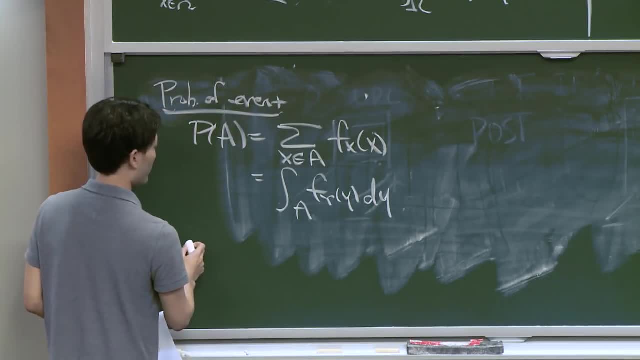 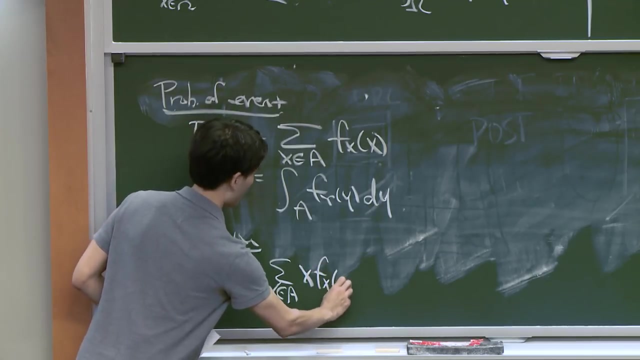 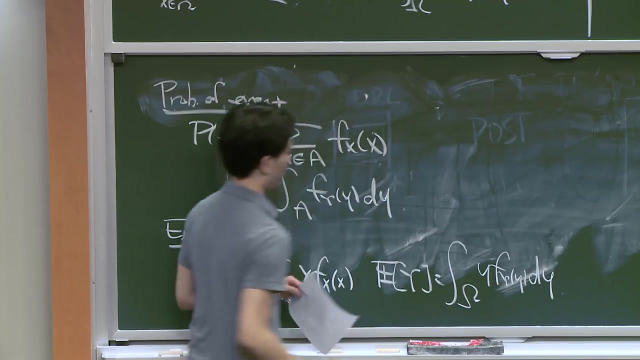 depending on what we're using, And expectation, Expectation. Expectation Our mean Is: expectation of x is equal to the sum of all x, x times that, And expectation of y is the integral over omega- sorry space, y times A. 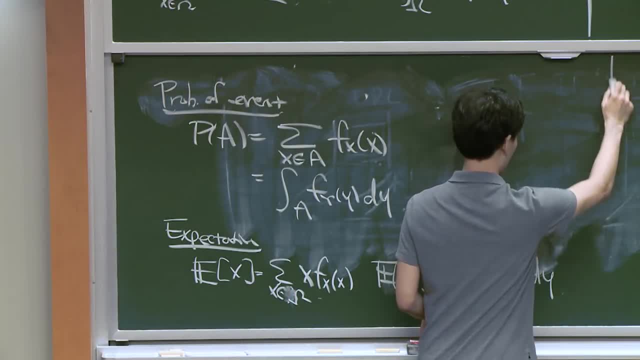 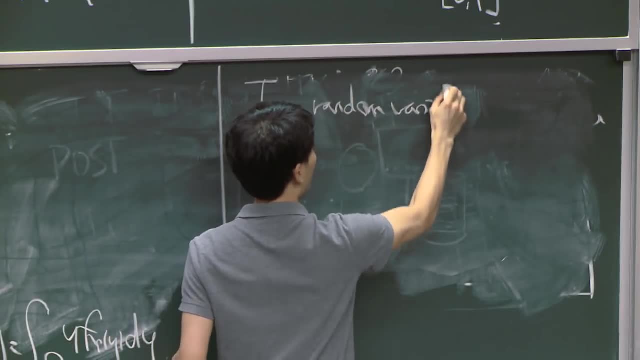 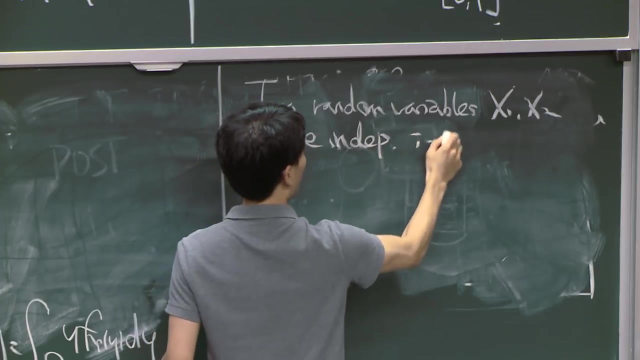 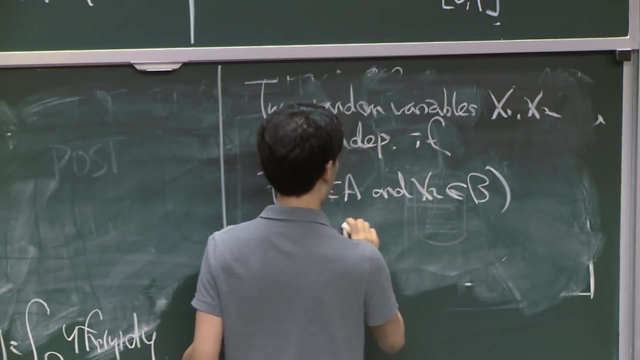 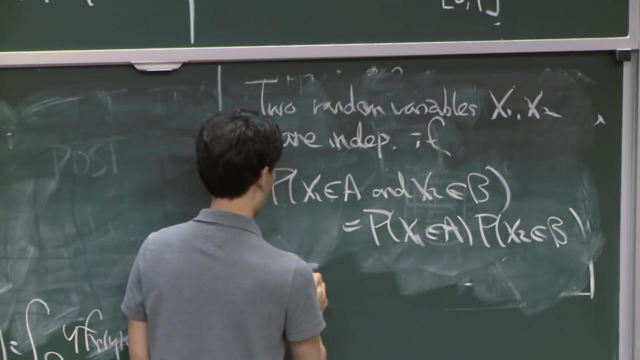 And one more basic concept I want to Review is two random variables- x1, x2, are independent. if probability that x1 is in A and x2 is in B equals the product of the probabilities for all events A- n. 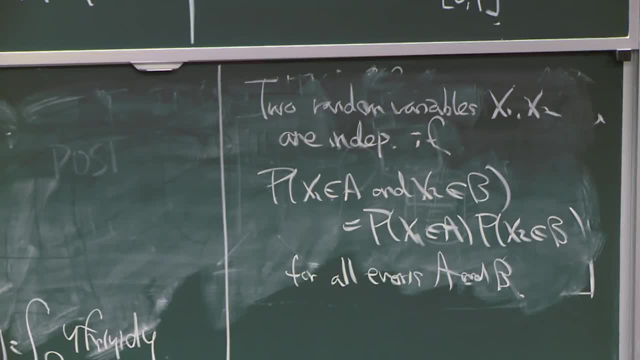 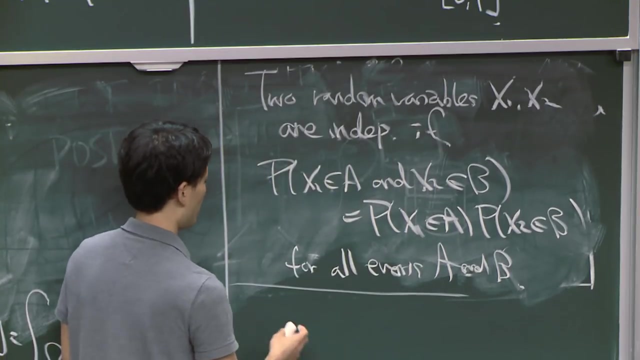 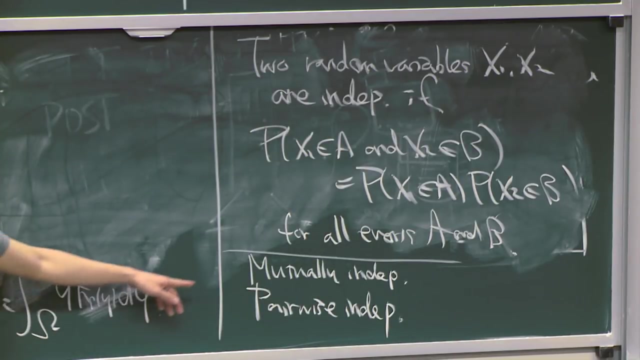 OK, All agreed. So for independence, I will talk about independence of several random variables as well. There are two concepts of independence, Not two but several, But two most popular are mutually independent events And pairwise independent events. Can somebody tell me the difference between these two? 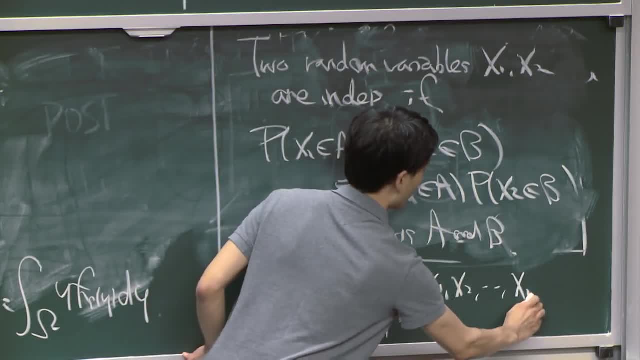 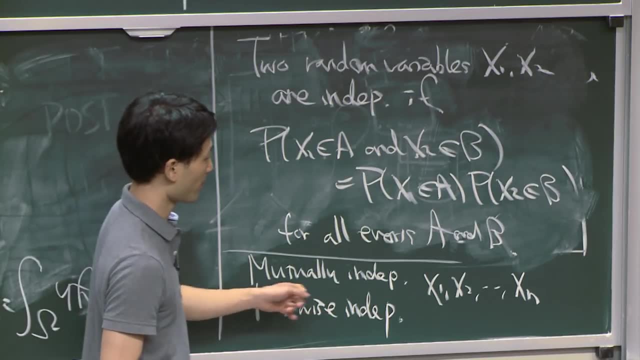 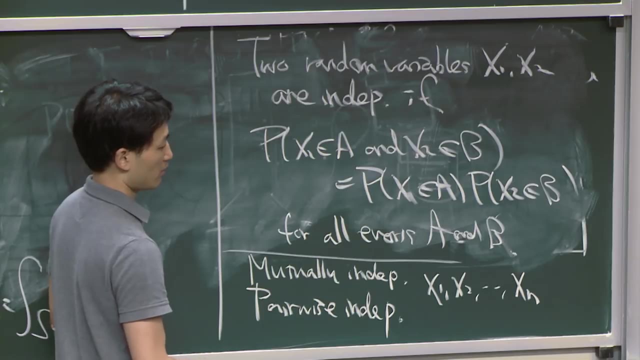 For several variables. let's say x2, xn. Yeah, So mutually independent means all the random variables are independent, like x1 is independent with every other. But pairwise means x1 and x2 are independent, But x1, x2, and x3, they may not be independent. 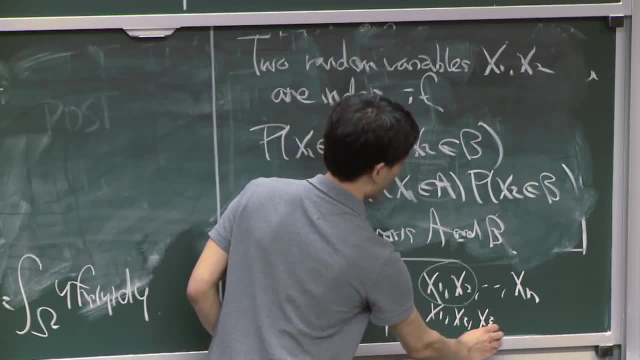 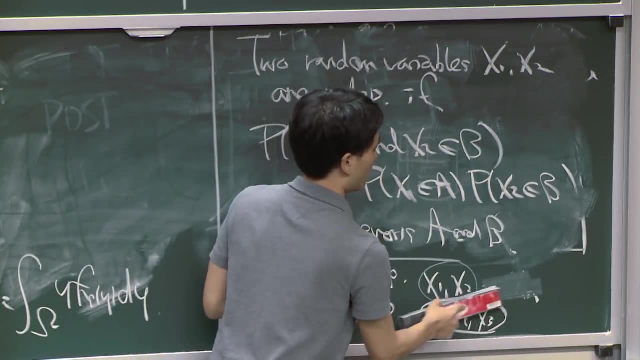 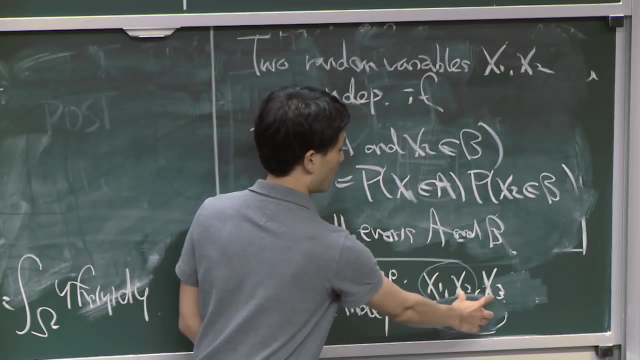 OK, Maybe, Yeah, So that's good. So let's see in the example of three random variables. it might be the case that each of them, so each pair, are independent: x1 and x2.. One is independent with x2, x1 is independent with x3.. 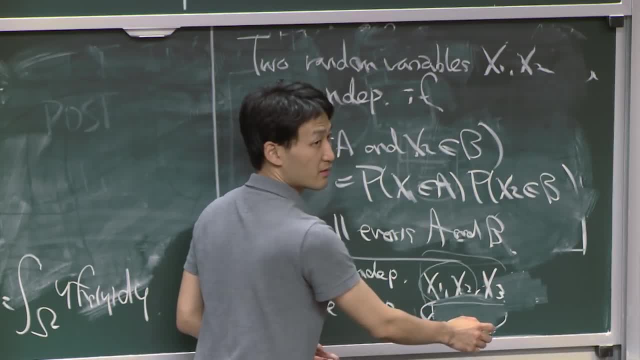 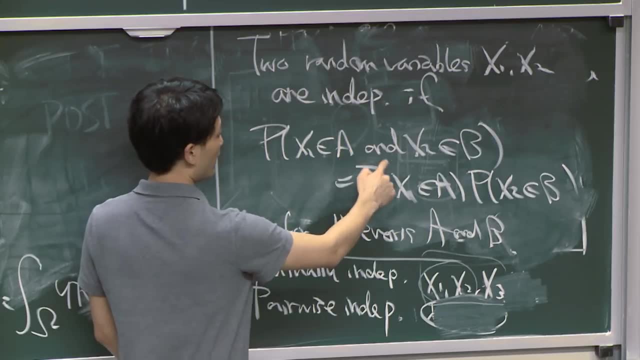 x2 is with x3. But altogether it's not independent. So what that means is: this type of statement is not true. So there are steps a1,, a2, a3 for which this does not hold. But that's just some technical detail. 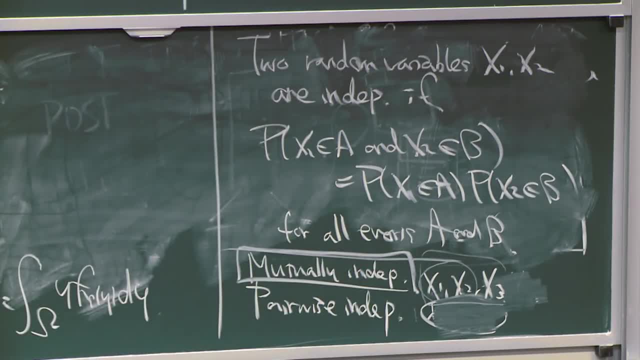 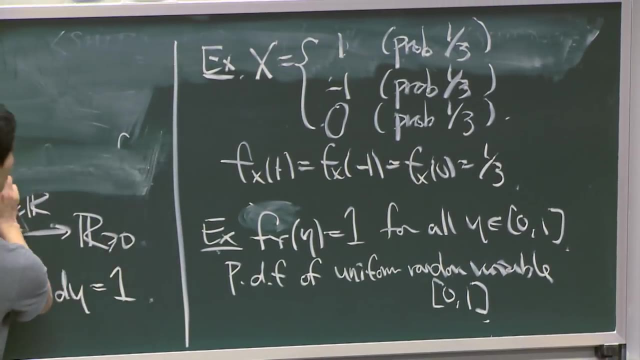 We will mostly just consider mutually independent events. So when we say that several random variables are independent, it just means, whatever collection you take, they're all independent. OK. So a little bit more fun stuff. let's do a little review, OK. 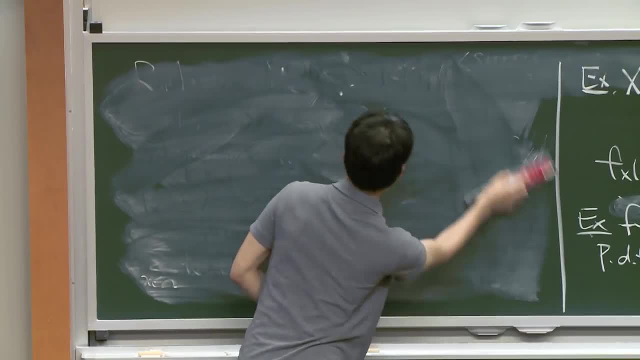 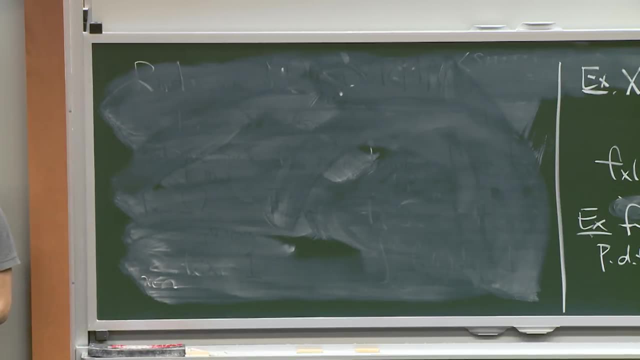 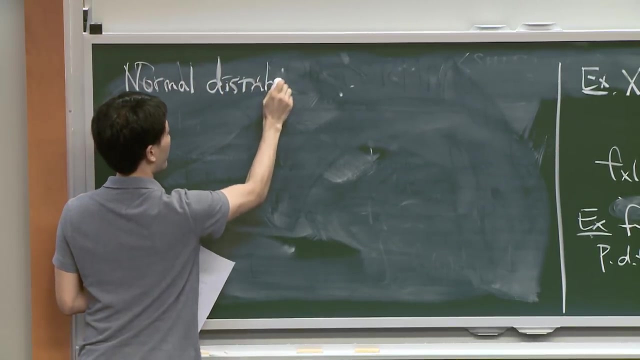 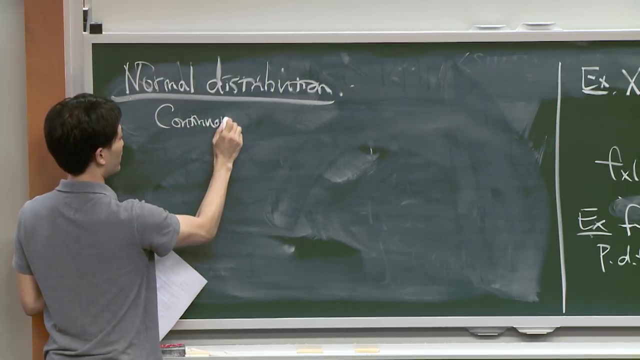 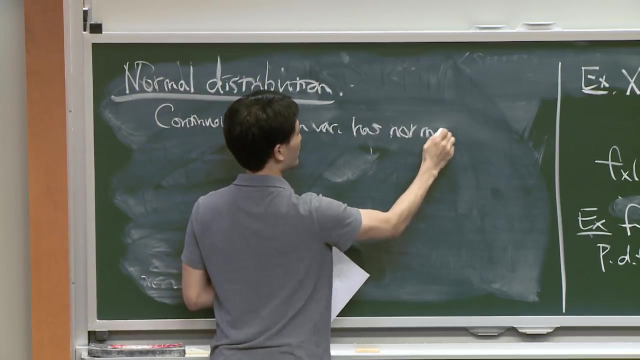 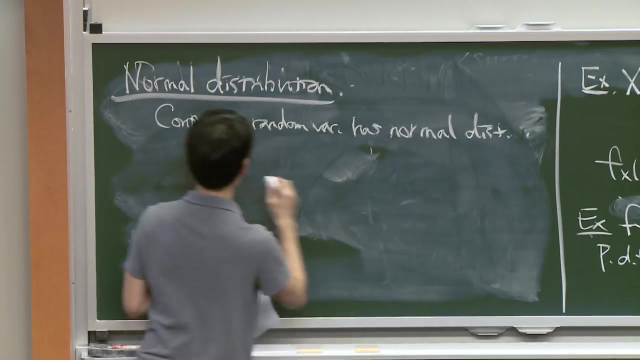 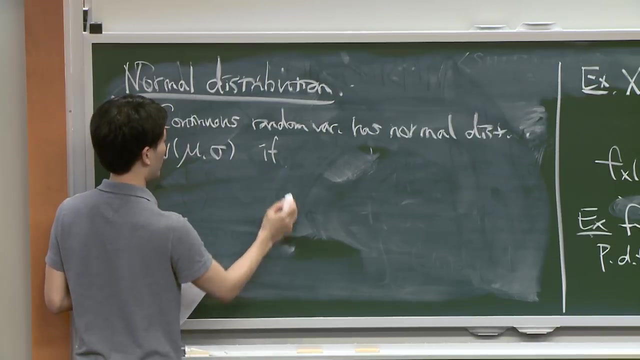 So we defined random variables And one of the most universal random variables, our distribution is a normal distribution. It's a continuous random variable. A continuous random variable has normal distribution is said to have normal distribution if n, mu, sigma, if the probability distribution. 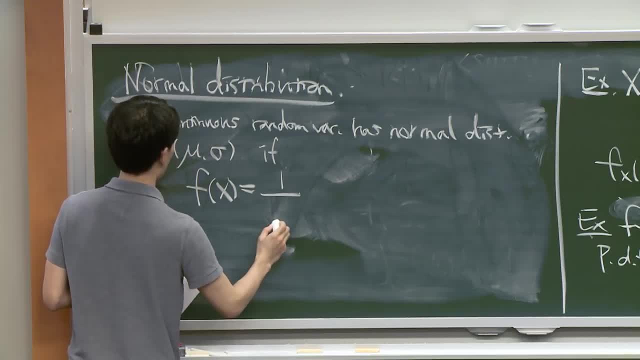 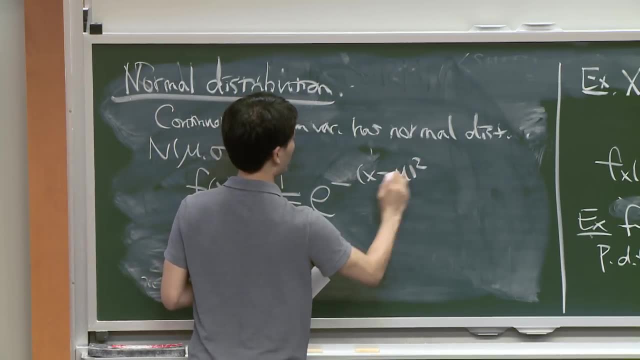 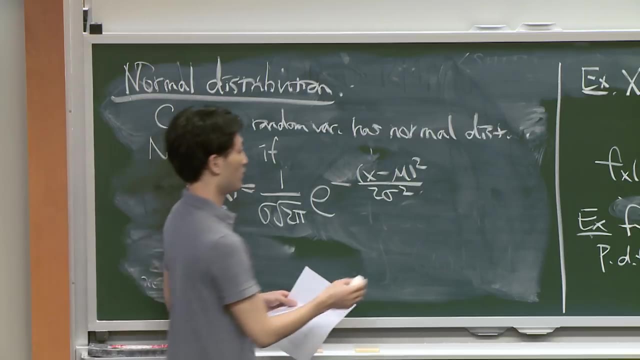 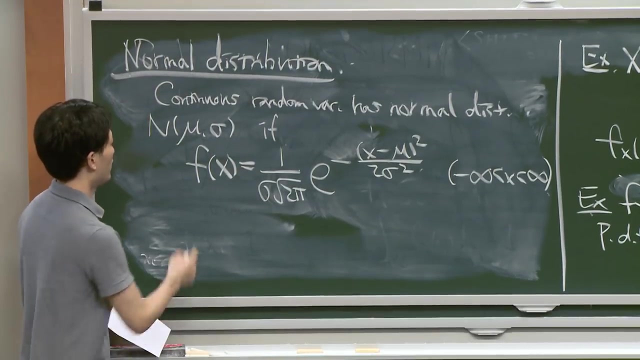 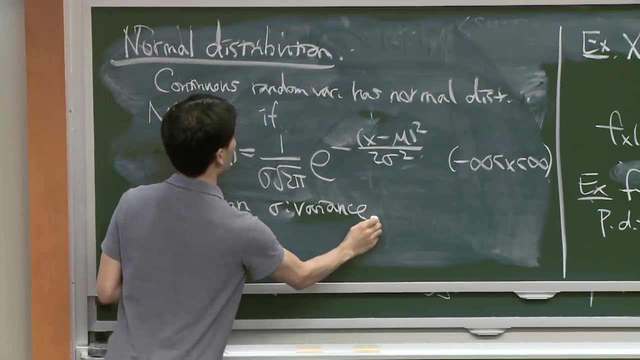 function is given as 1 over sigma squared, n mu squared, n mu squared. So it's 2 pi e to the minus s mu squared, for all reals. So mu mean that's one of the most universal random variables distribution. 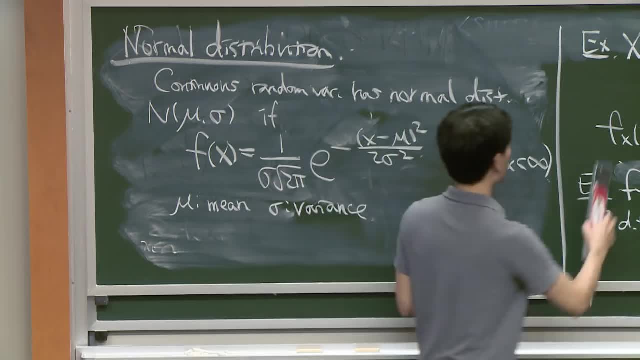 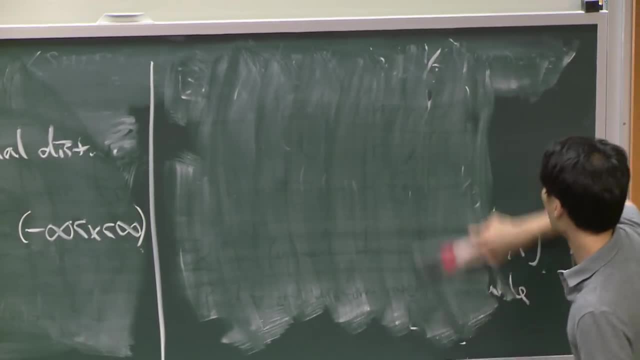 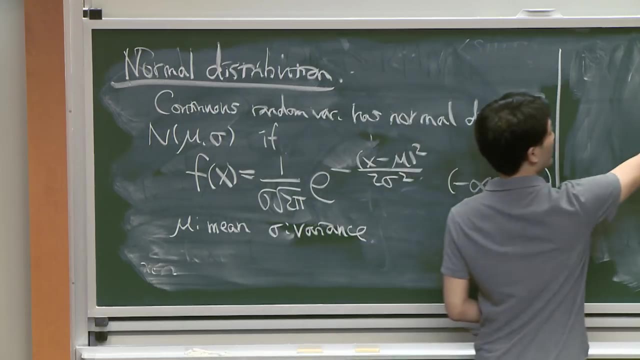 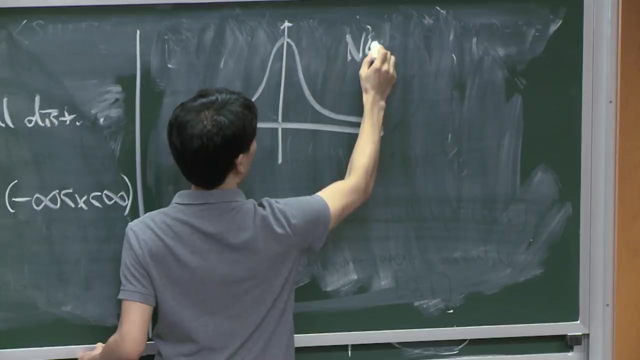 The most important one as well. OK, So this distribution, how it looks like. I'm sure you saw this bell curve before. It looks like this: If it's n, 0,, 1,, let's see. and that's the y. 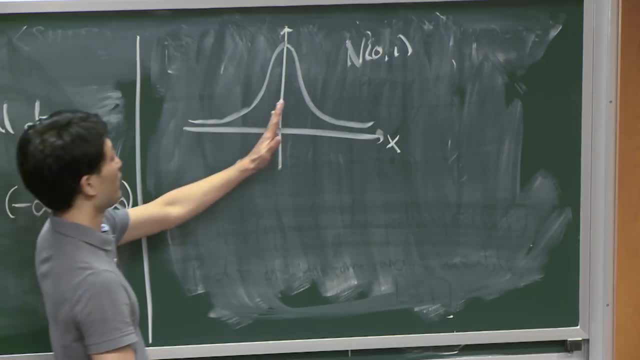 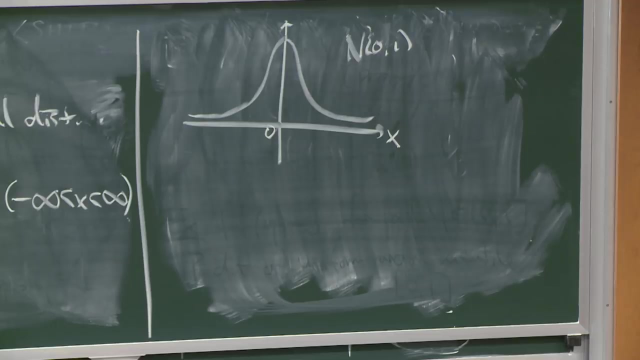 OK, So it's centered around the origin and it's symmetric around the origin. OK, So now let's look at our purpose. Let's think about our purpose. We want to model a financial product or, like a stock, the price of the stock- using some random variables. 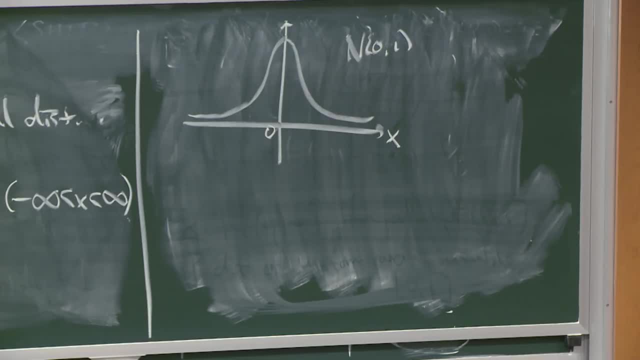 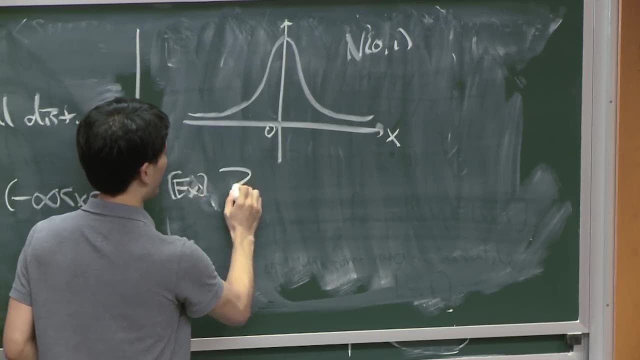 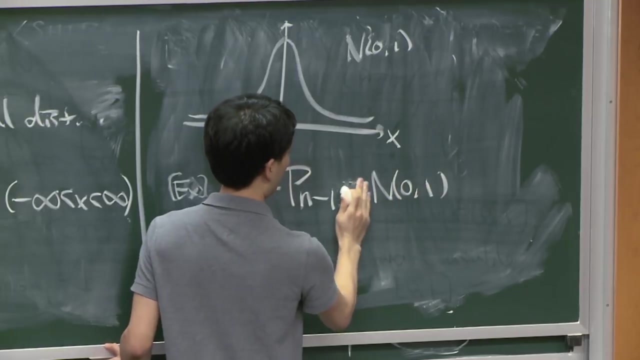 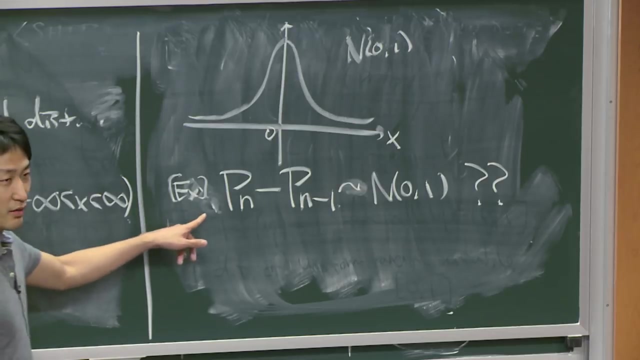 The first thing you can try is to use normal distribution. Normal distribution doesn't make sense, but we can say: the price at day n minus the price at day n minus 1, is normal distribution. Is this a sensible definition? That's not really so. it's not a good choice. 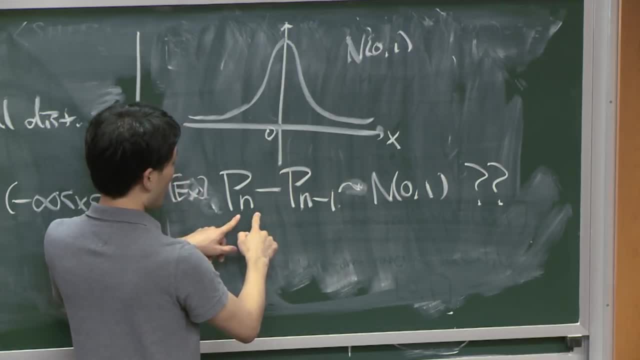 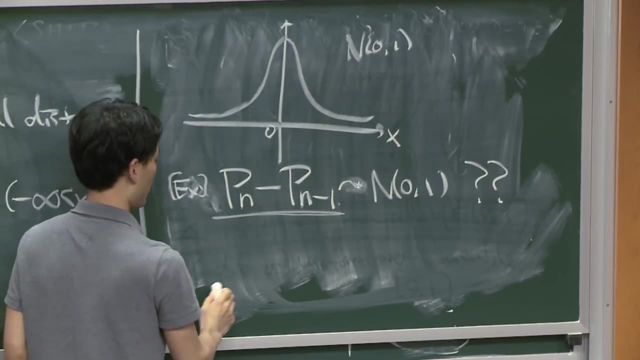 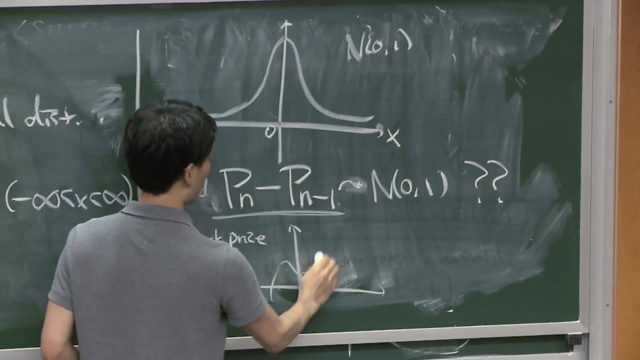 You can model it like this, but it's not a good choice because there might be several reasons, But one reason is that it doesn't take into account the order of magnitude of the price itself. So the stock. let's say You have a stock price. I don't know something like that. 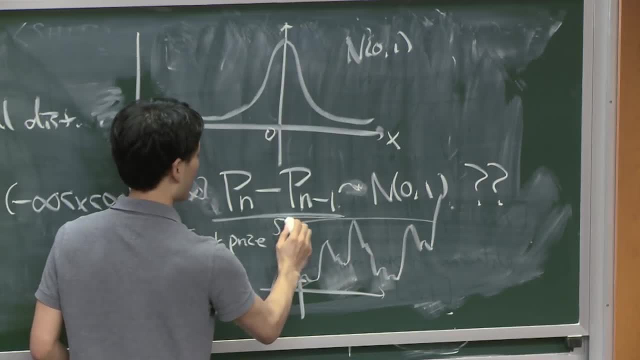 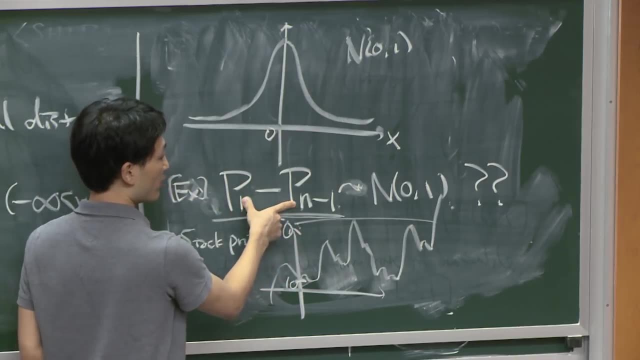 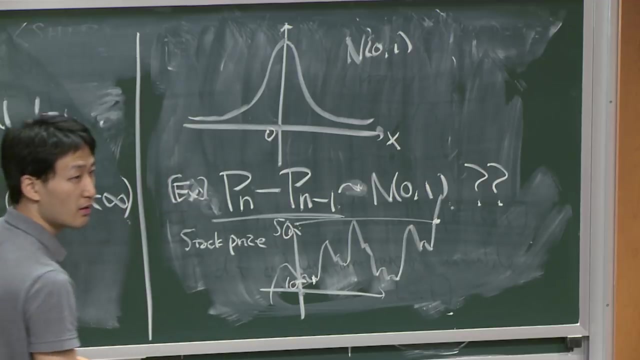 And say it was $10 here and like $50 here. So regardless of where your position is at, it says that the increment, the absolute value of the increment, is identically distributed at this point and at this point. But if you observed like how much. 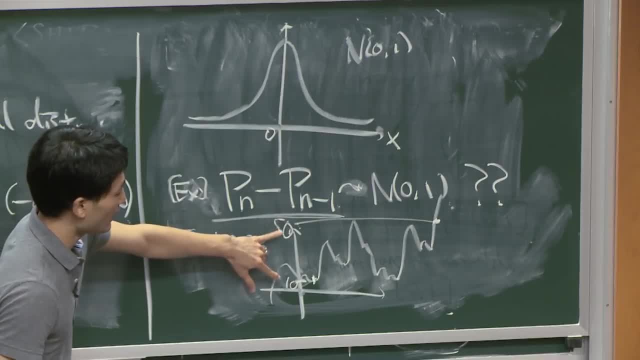 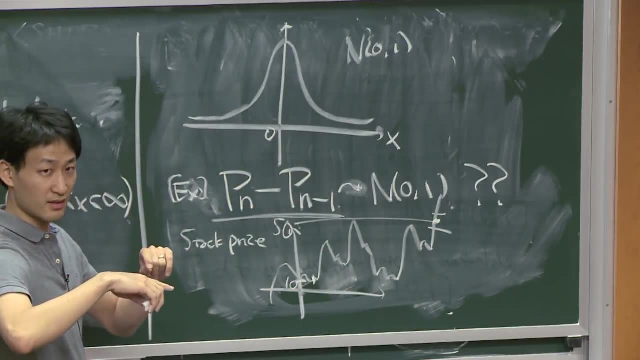 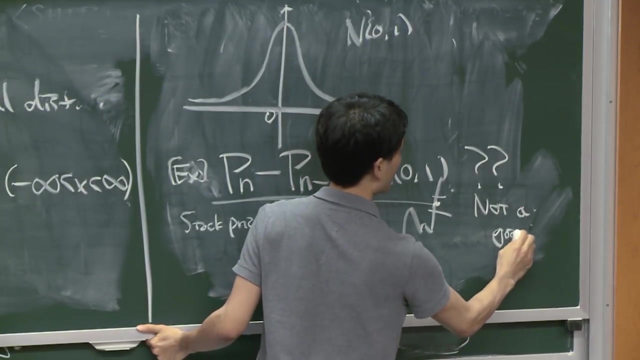 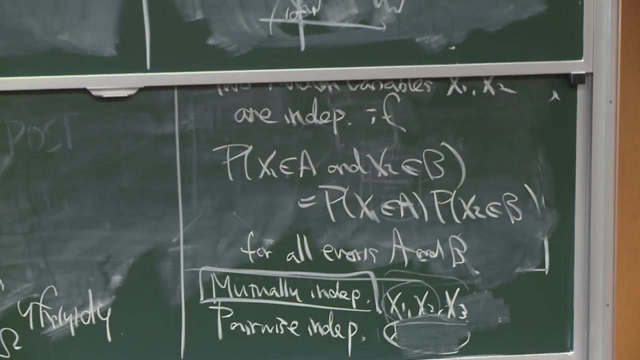 how it works. usually that's not normally distributed. What's normally distributed is the percentage of how much it changes daily. So this is not a sensible model, not a good model, But still we can use normal distribution to come up with a pretty good model. 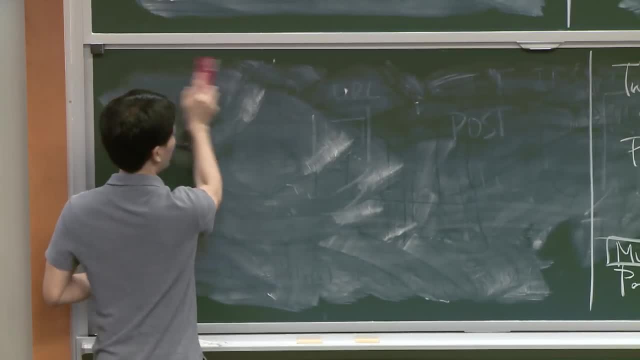 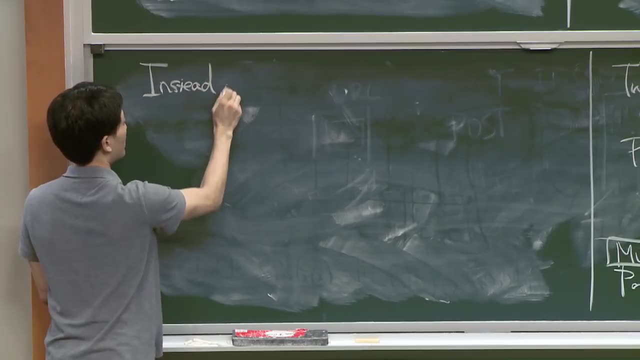 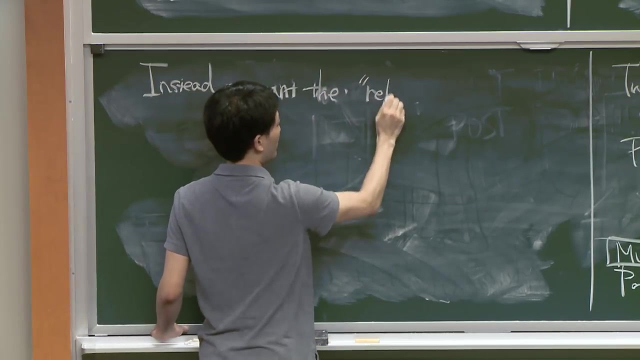 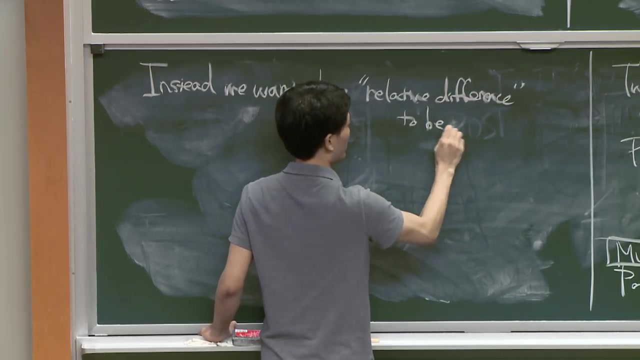 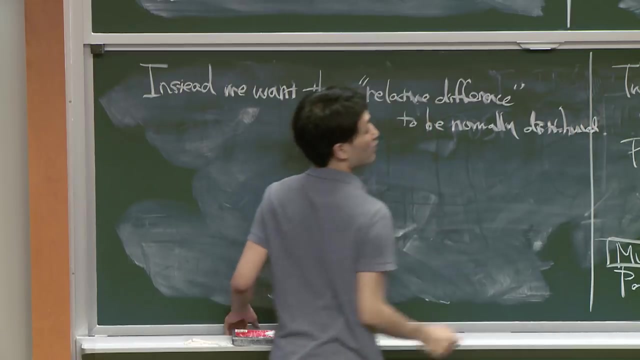 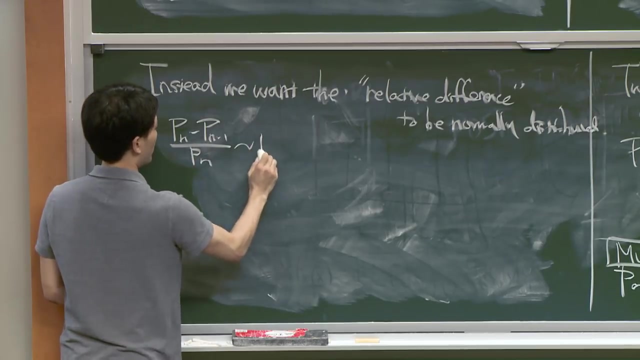 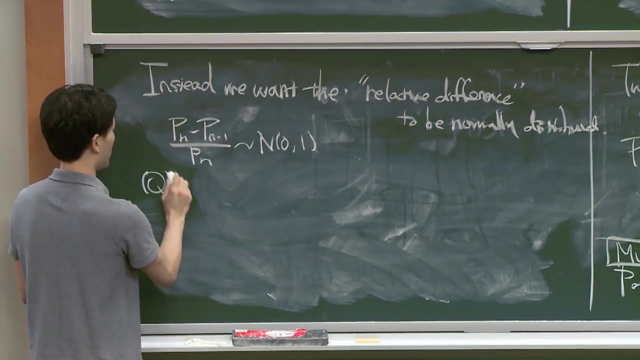 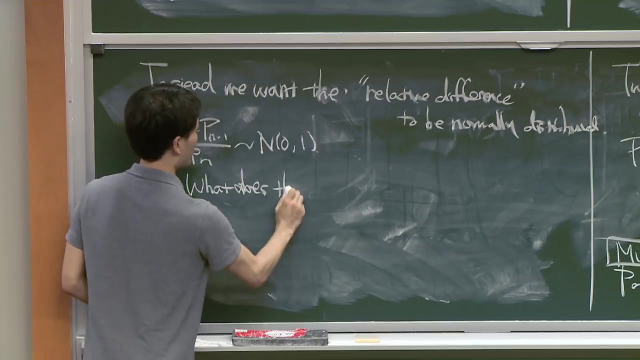 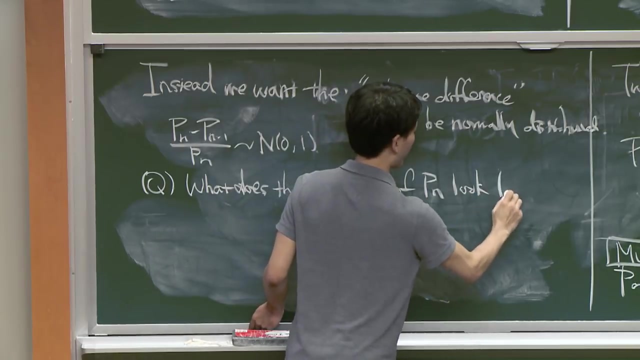 Instead, we want the relative difference to be normally distributed, That is, the percent. the question is: what is the distribution of price? What does the distribution of price? What does the distribution of price look like at this point? So it's not a very good explanation. 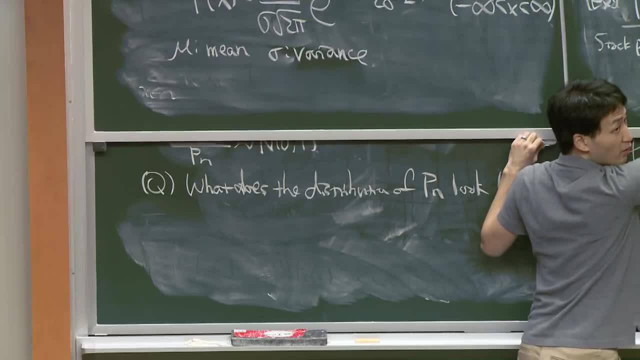 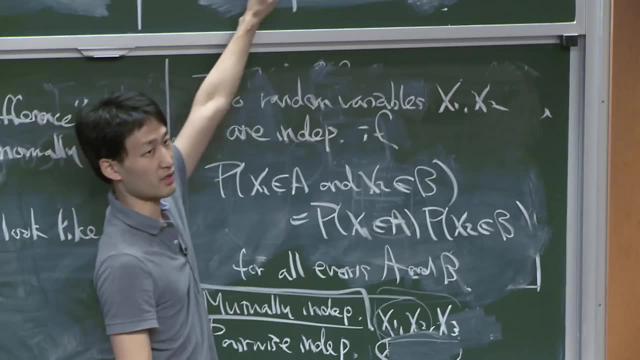 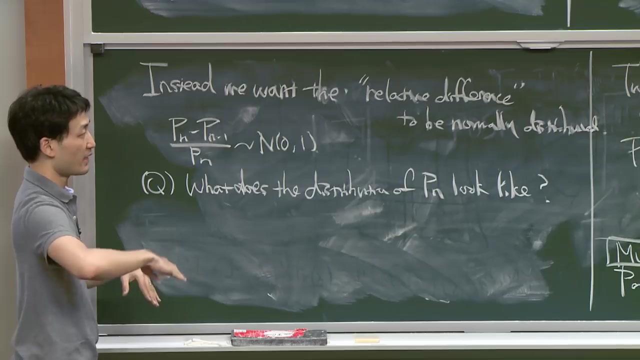 because I'm giving just discrete increments, while these are continuous random variables and so on. But what I'm trying to say here is that normal distribution is not good enough. Instead, we want the percentage change to be normally distributed. And if that is the case, what will? 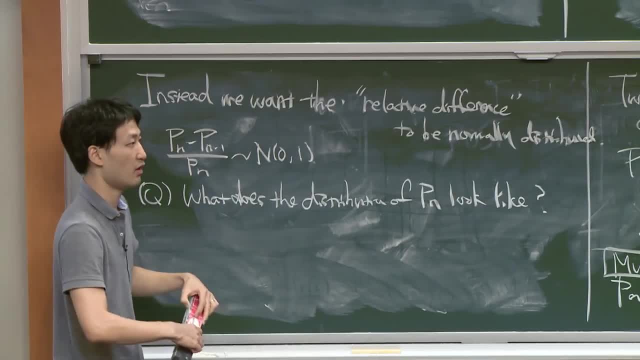 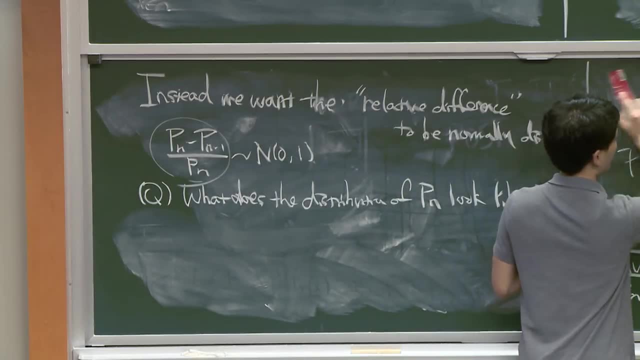 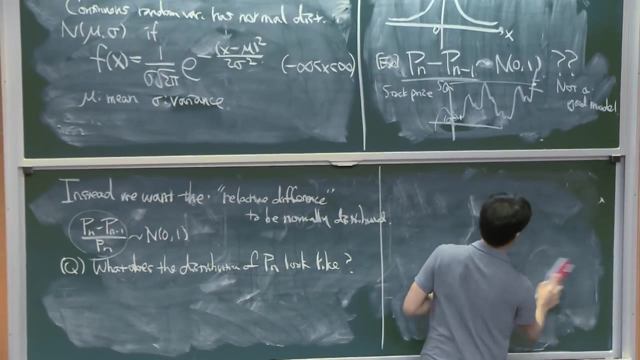 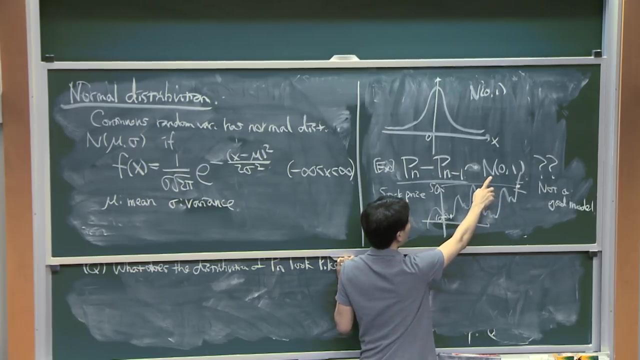 be the distribution of the random variable, Like in this case. what will be the distribution of the price? The one thing I should mention is, in this case, if each discriminant is normally distributed, then the price that they end, The price that they end- will still. 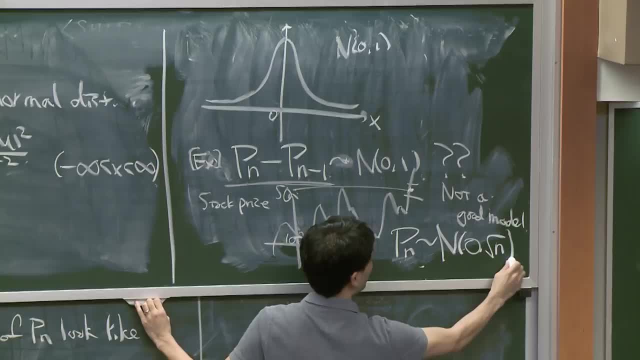 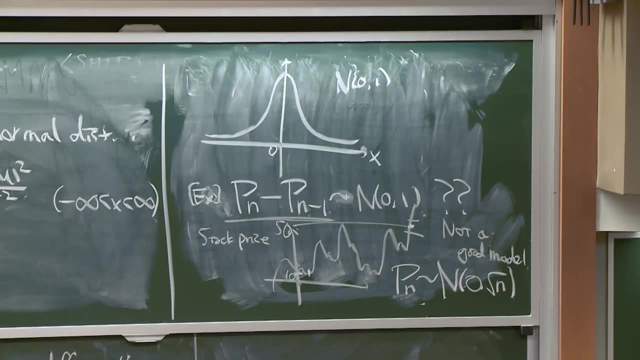 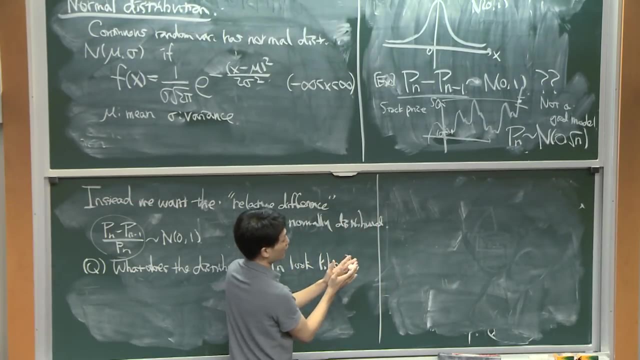 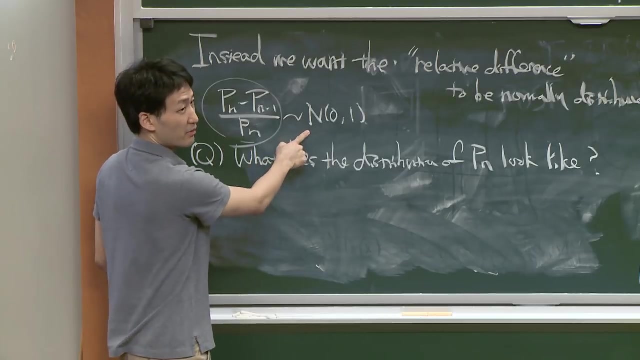 be a normal random variable distributed like that. So if there is no tendency, if the average increment is 0,, daily increment is 0, then no matter how far you go, your random variable will be normally distributed. But here that will not be the case. 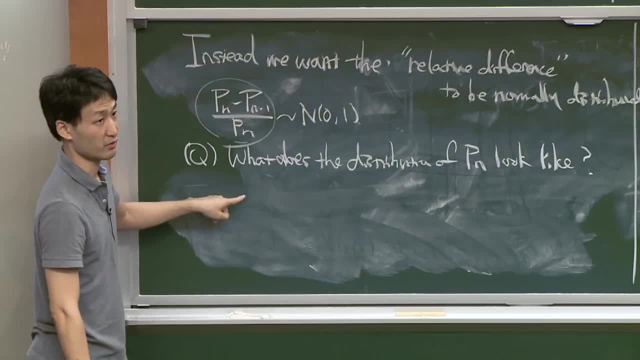 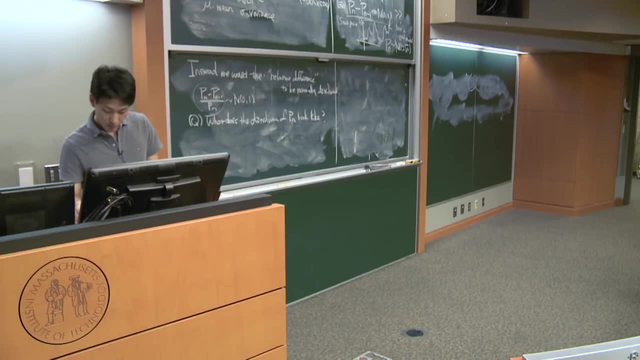 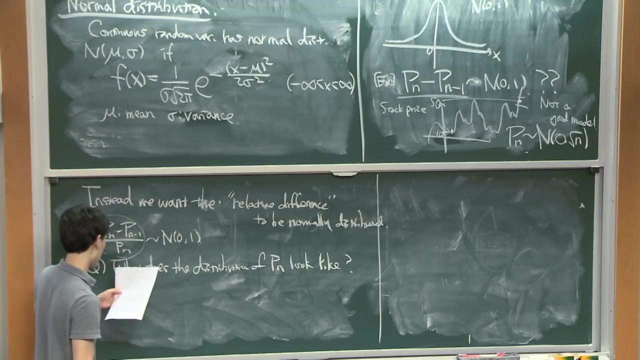 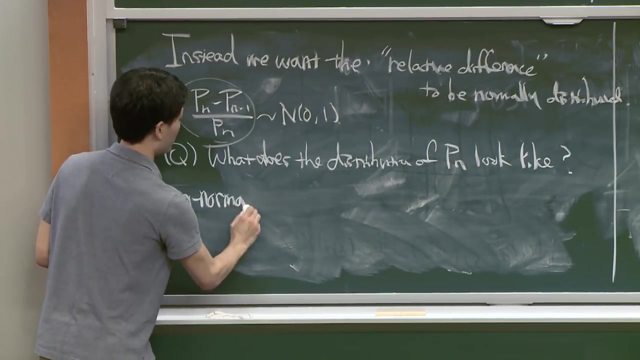 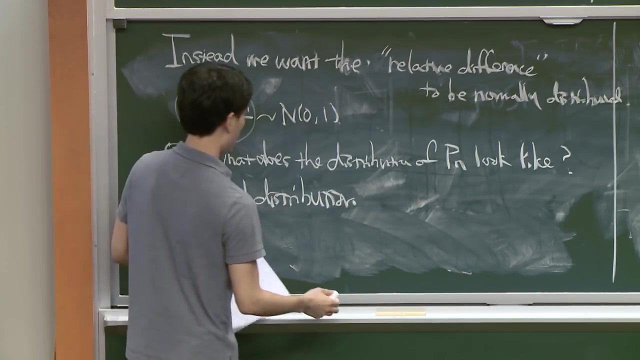 So we want it to come up. We want to see what the distribution of Pn will be in this case. Yeah, To do that, let me formally write down what I want to say. What I want to say is this: I want to define a log-normal distribution y. 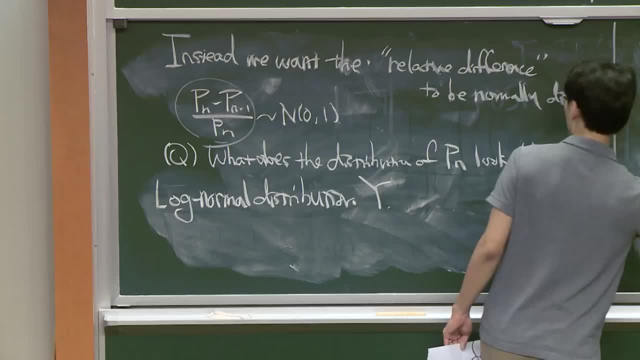 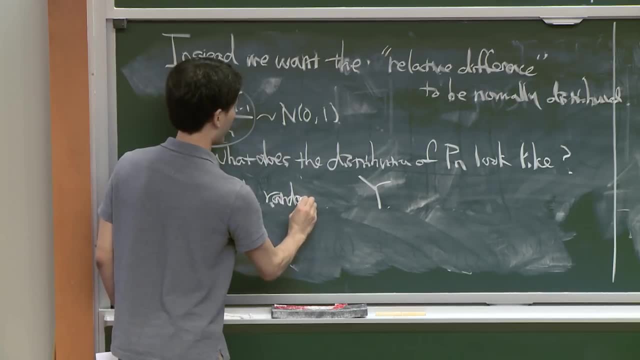 our log-normal random variable, y. And here, in this case, I'm going to write down: I'm going to write down that the number of times this term is equal to 0, is the number of times this term is equal to y. 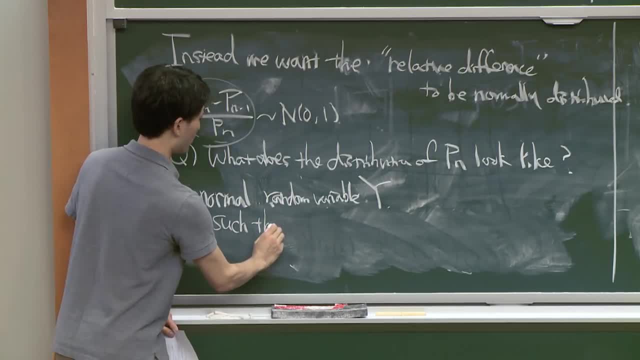 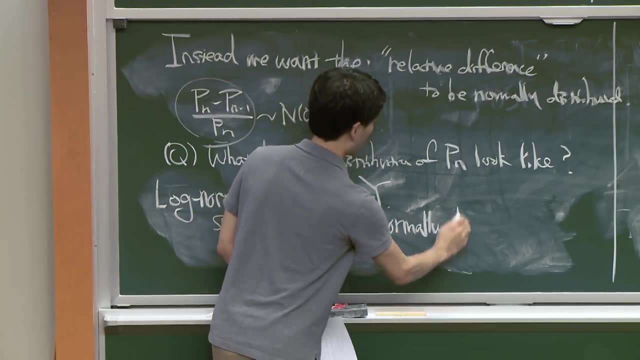 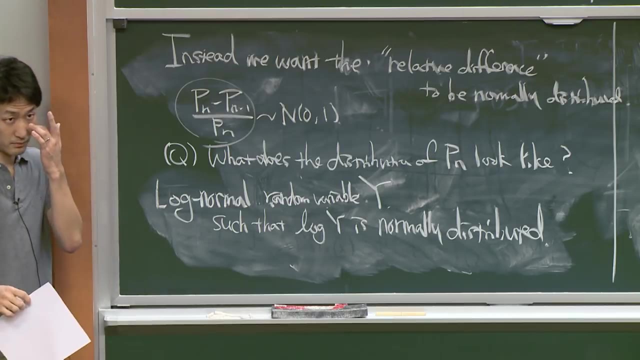 and the number of times this term is equal to y is the number of times this term is equal to y, And so the only thing you can do is break it down. That's that log of y. Oh, This is too big. 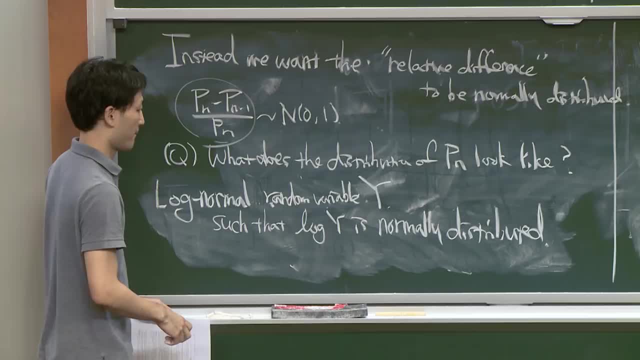 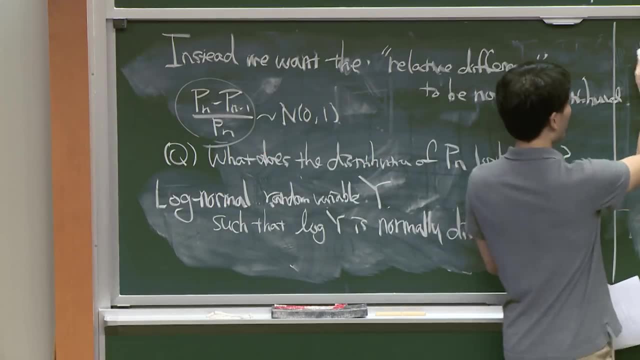 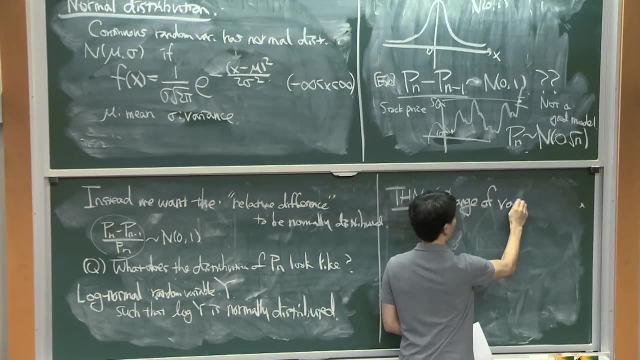 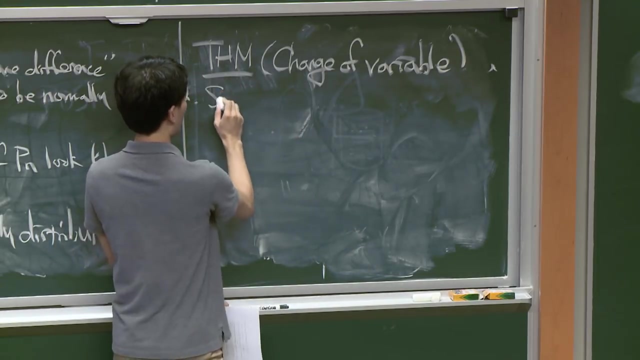 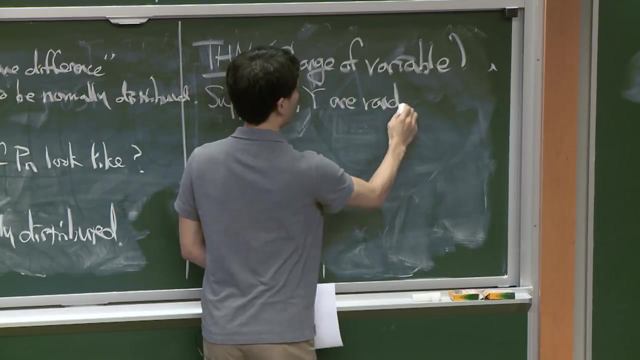 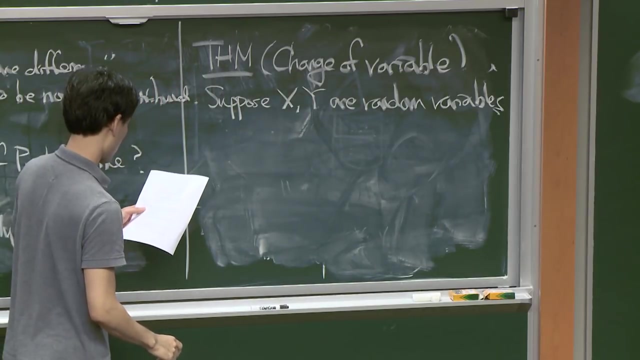 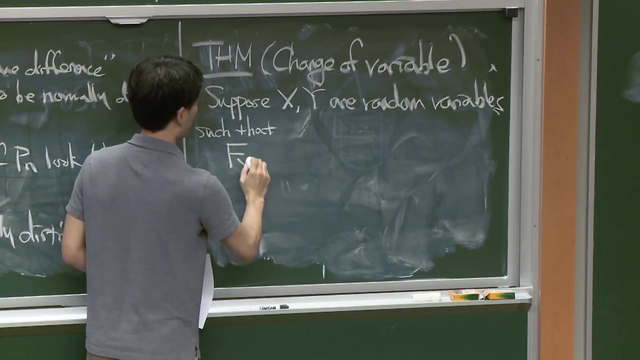 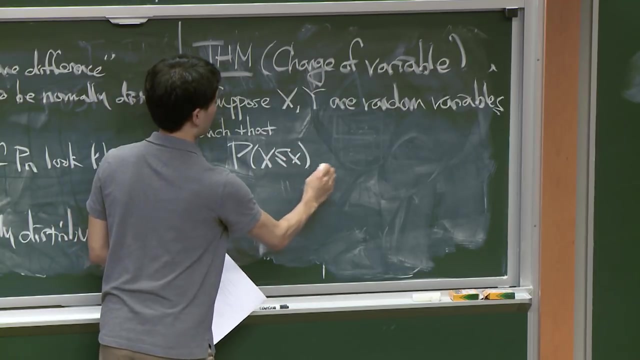 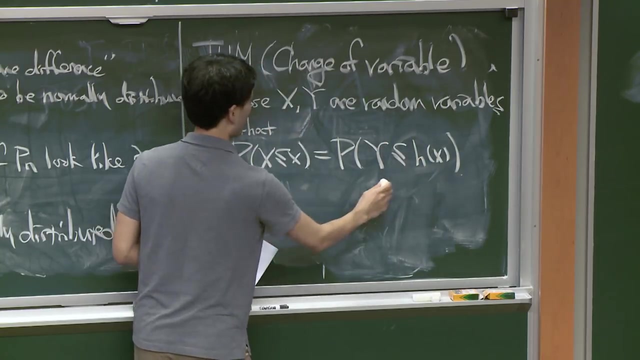 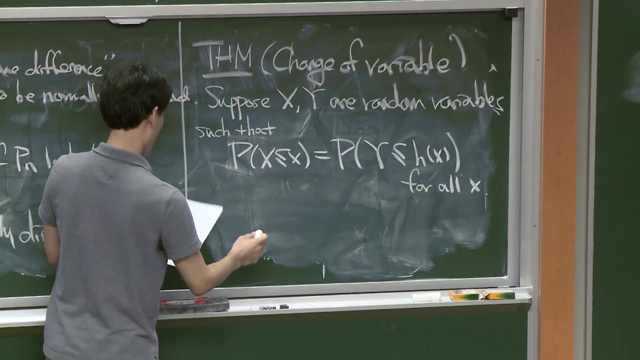 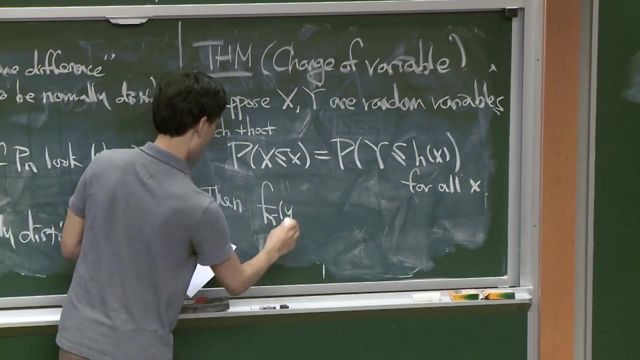 So to derive the probability distribution of this from the normal distribution, we can use the change of variable formula, which says the following: Suppose x and y are random variables such that I should have defined this: x times x for all x and f of y for y. 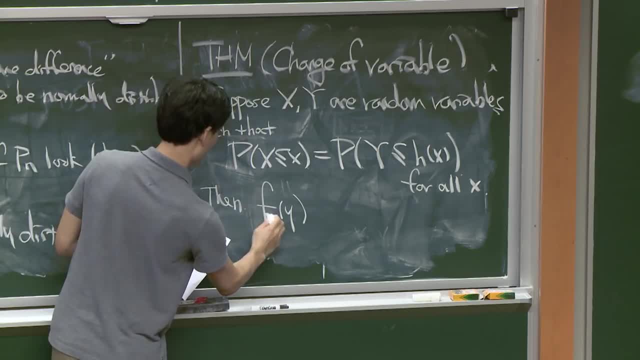 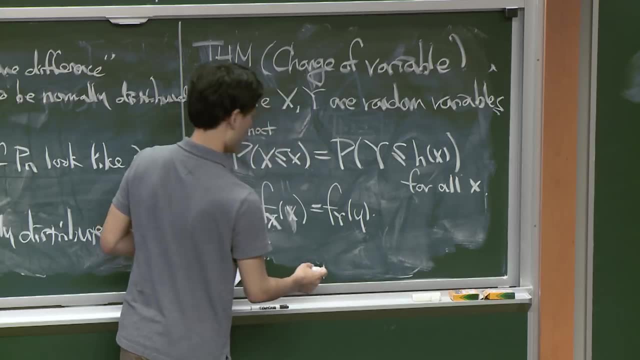 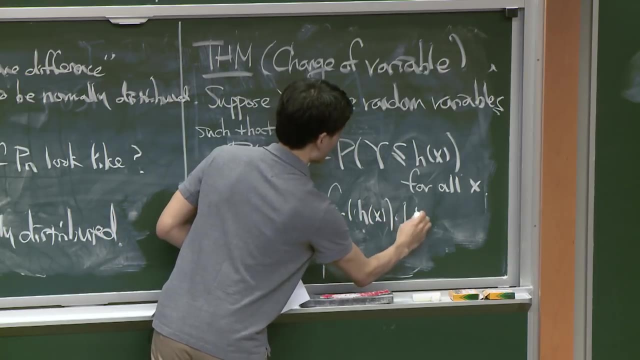 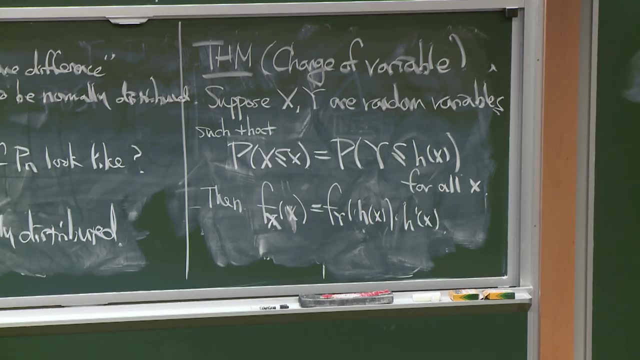 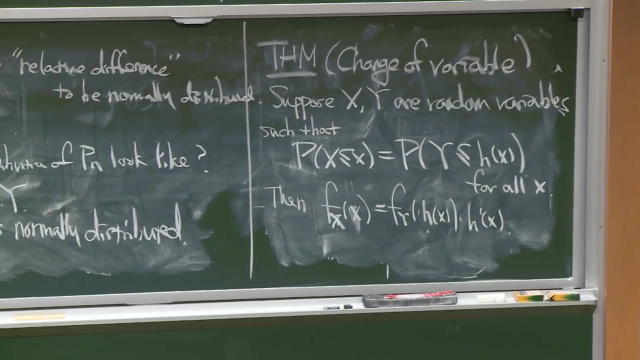 f of x, f of y, f of x, f of x, f of y, f of x, f of x, f of y. So let's try to fit into this story. We want to have a random variable y, such that log y is normally distributed. 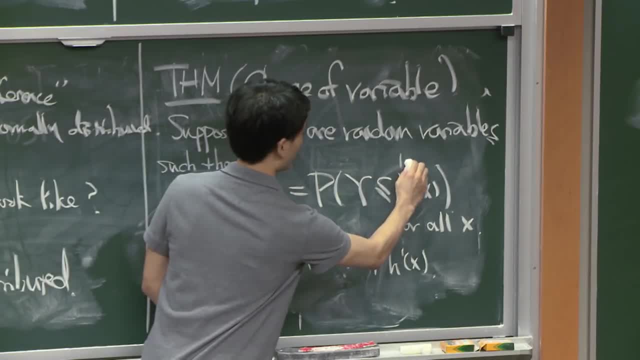 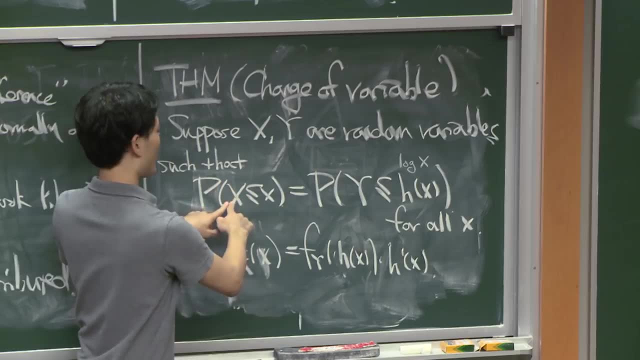 Here. so if you put log of x here, if y is normally distributed, x will be the distribution that we're interested in. So using this formula we can find probability distribution function of the log normal distribution using the probability distribution of normal. 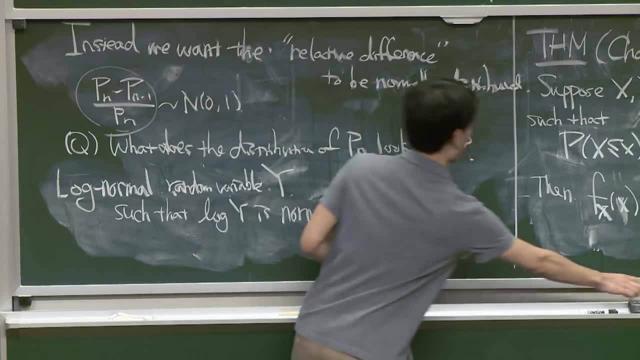 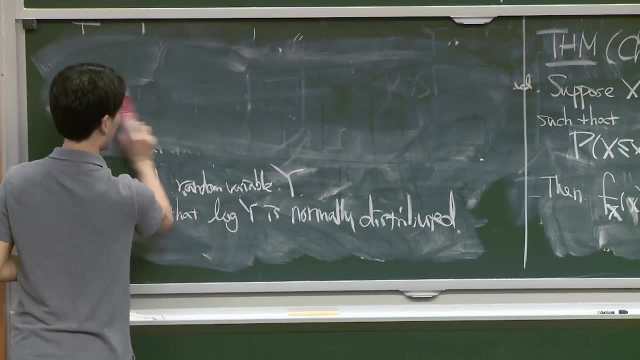 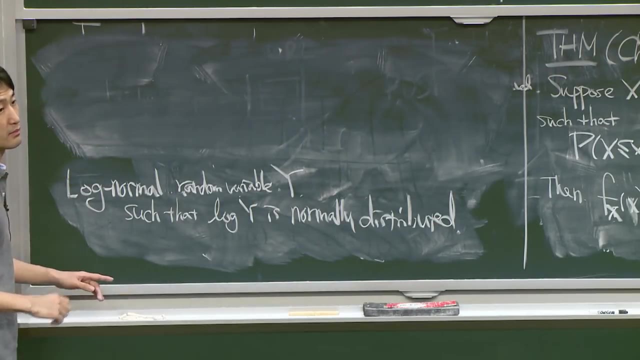 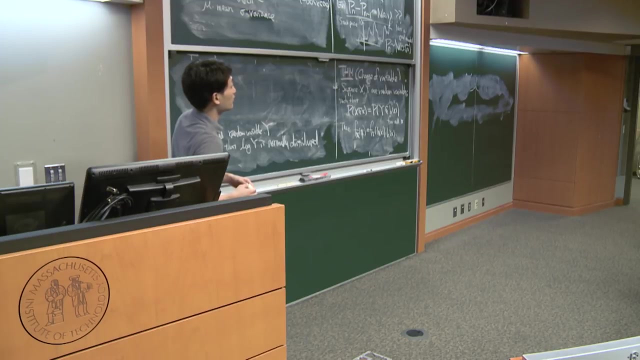 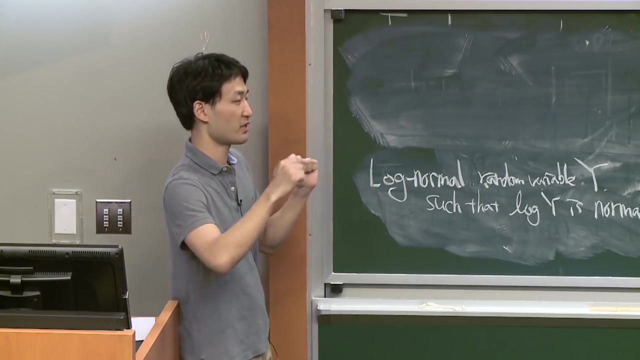 So let's do that. Yes, Yes, No, Not. So it's not a good choice. Locally it might be a good choice, But if you take it over a long time it won't be a good choice, because it will also. 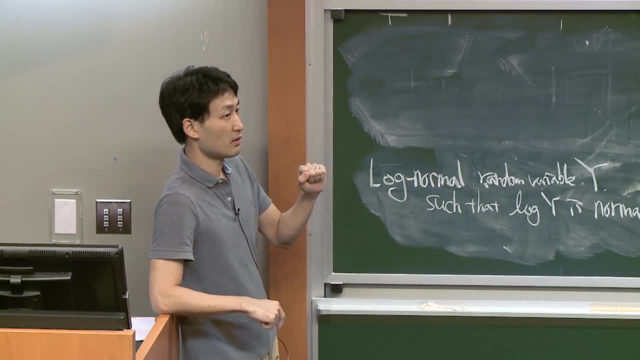 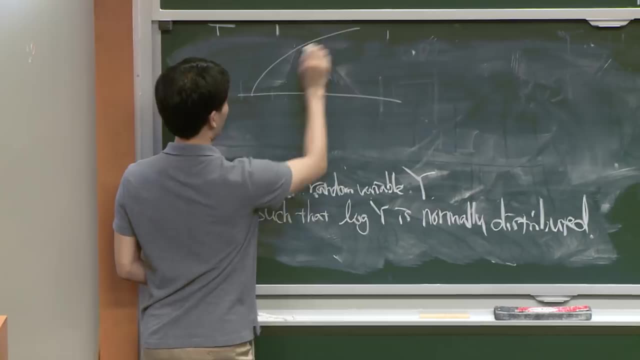 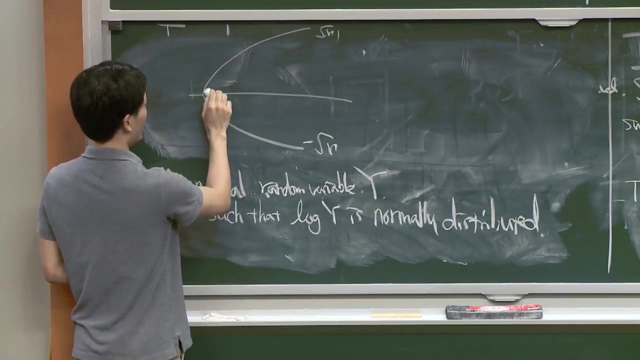 take negative values, for example. So if you just take this model, what's going to happen over a long period of time is it's going to hit this square root of n- negative square root of n- like infinitely often, And then it can go up to infinity. 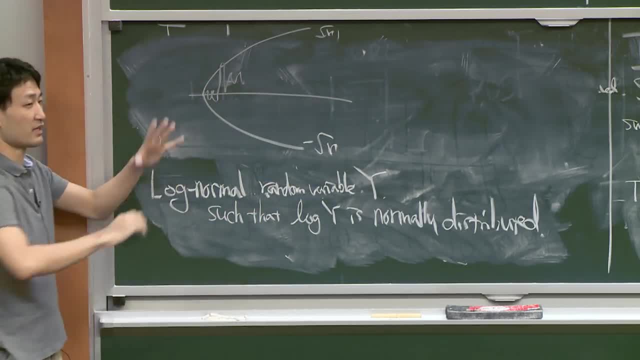 or it can go down to infinity eventually. So it will take negative values and positive values. Yeah, So that's one reason, But I mean there are several reasons why that is not a good choice. If you look at a very small scale, 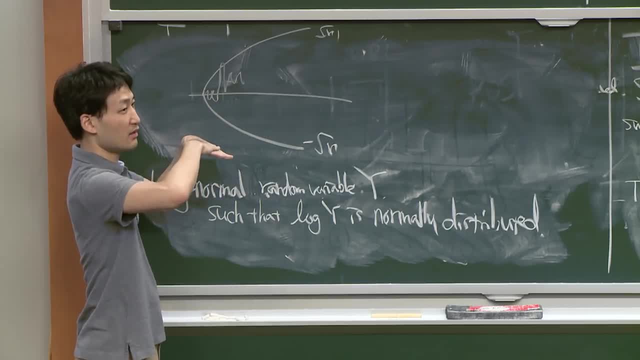 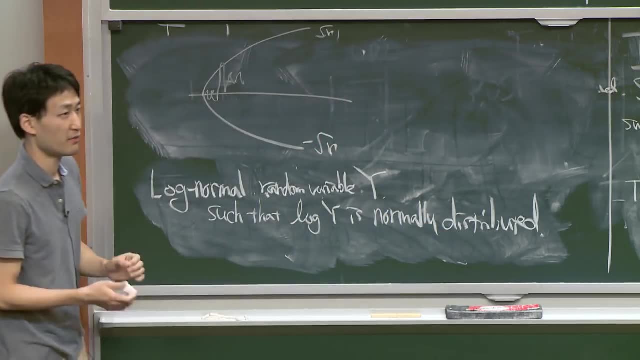 it might be OK, because the base price doesn't change that much. So if you model it in terms of ratio or if you just model it in an absolute way, it doesn't change, It doesn't matter that much. But if you want to do it in a little bit more large scale, 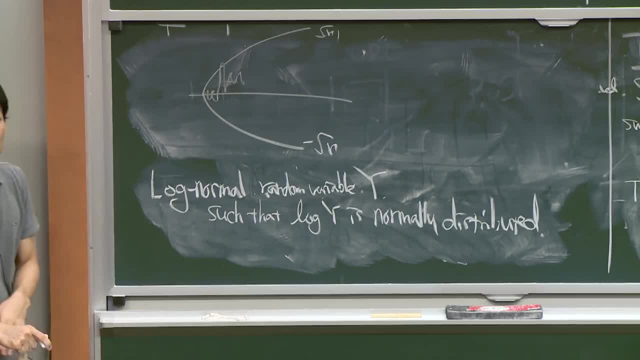 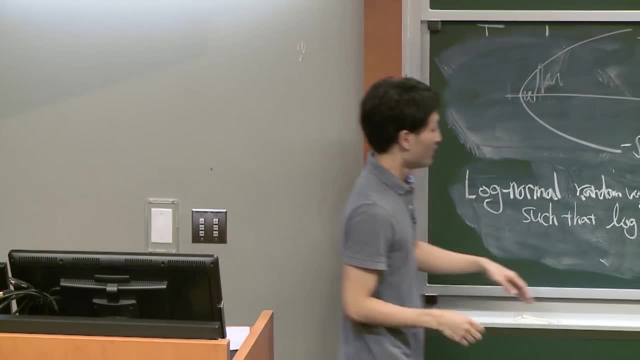 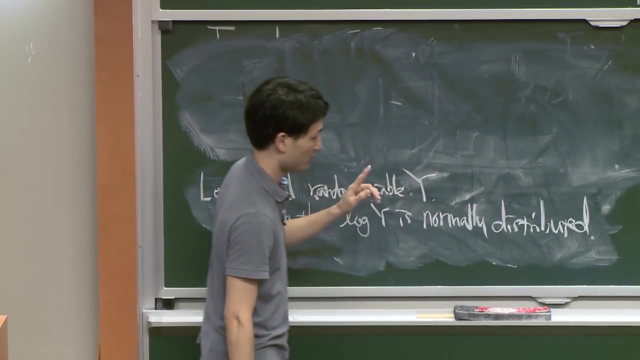 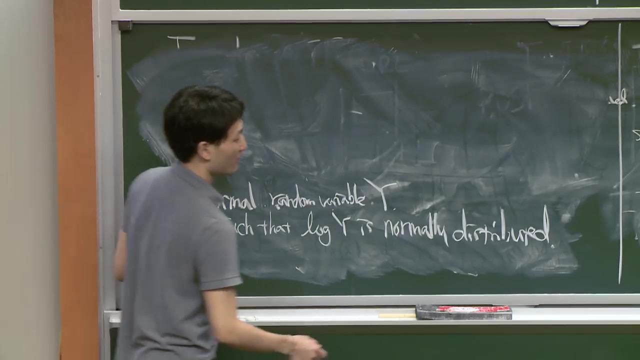 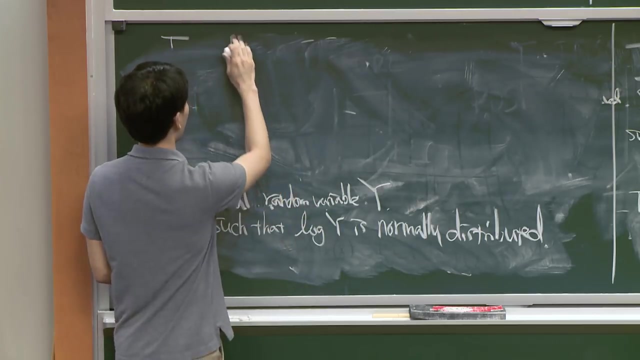 then that's not a very good choice. Other questions: Do you want to add some explanation? OK, So let me get this right. Let me make sure what I'm trying to do. 1. I want x to be the log-normal distribution. 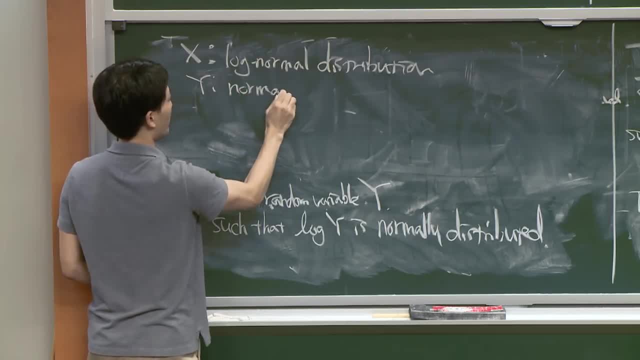 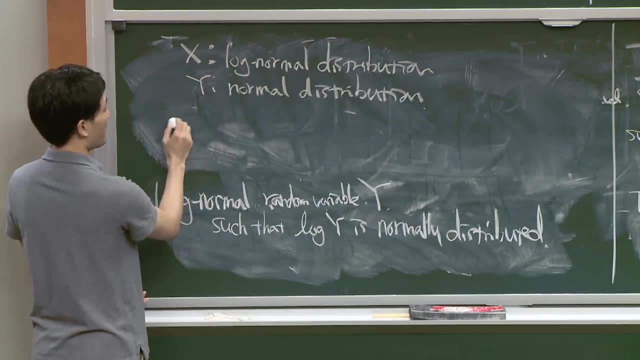 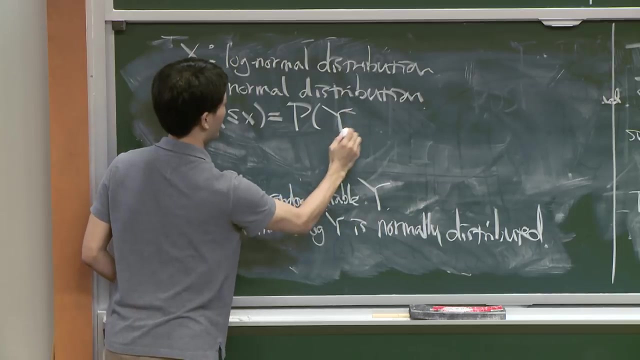 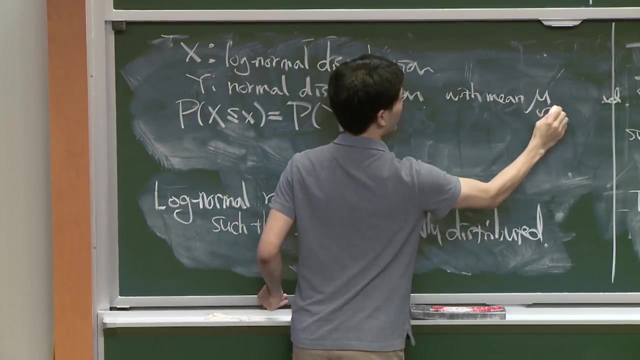 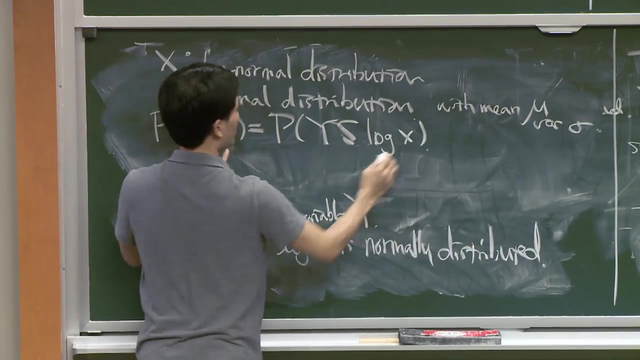 Then I want y to be normal distribution or normal random variable. Then the probability that x is at most x equals the probability that y is at most y is at most log x. That's the definition of log-normal distribution. Then, by using this change of variable formula, 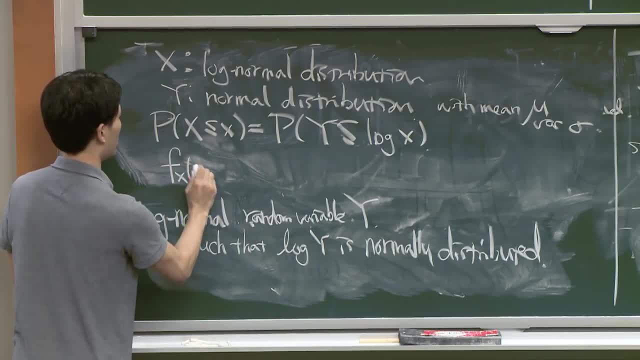 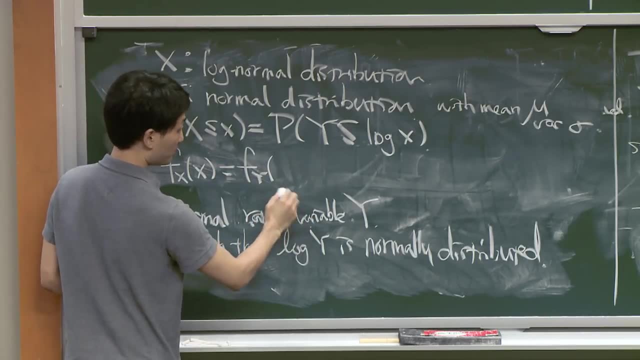 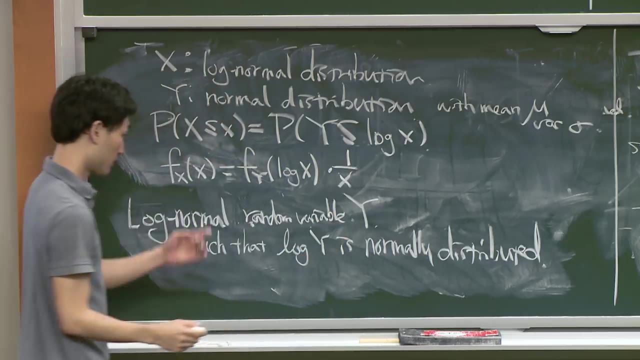 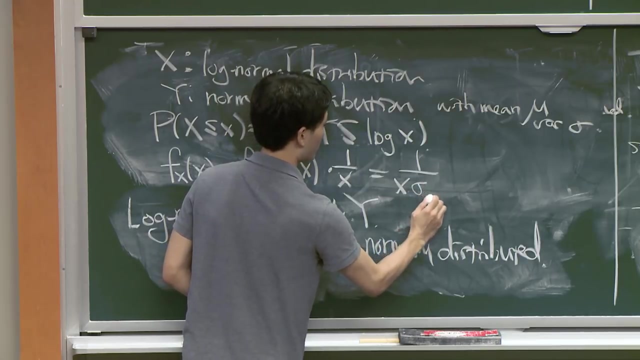 OK. The probability density function of x is equal to the probability density function of y at log x times the differentiation of log x, which is 1 over x, So it becomes 1 over x. sigma square root of 2 pi. e to the minus log x minus 2 pi. 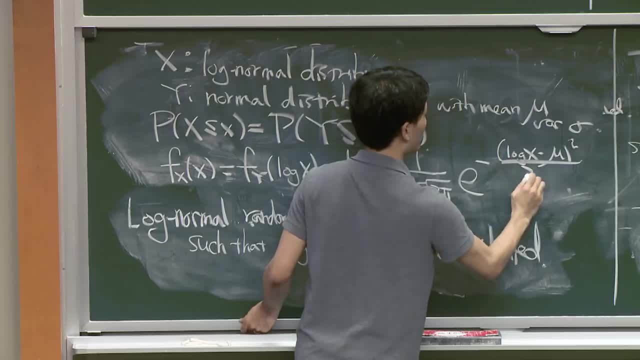 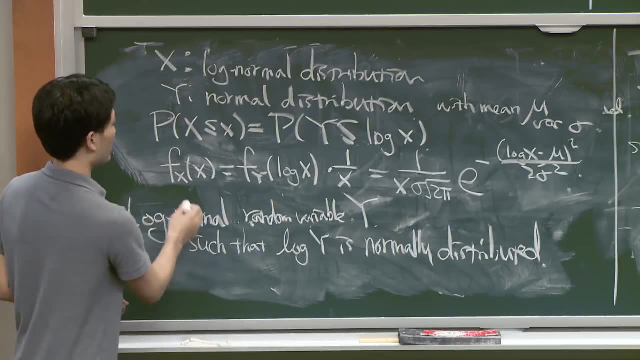 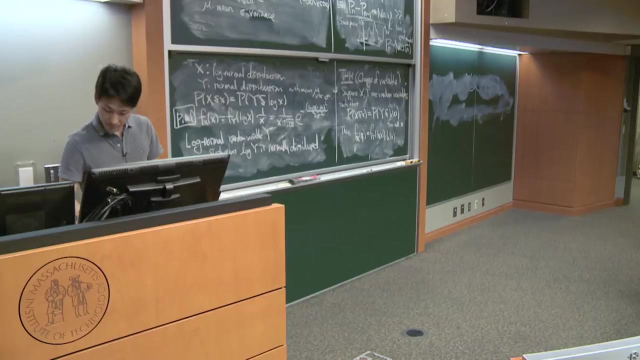 OK. OK, So log-normal distribution can also be defined as a distribution which has probability mass function. this, I mean you can use either definition. Let me just make sure that I didn't mess up in the middle. Yes, And that only works for x greater than 1.. 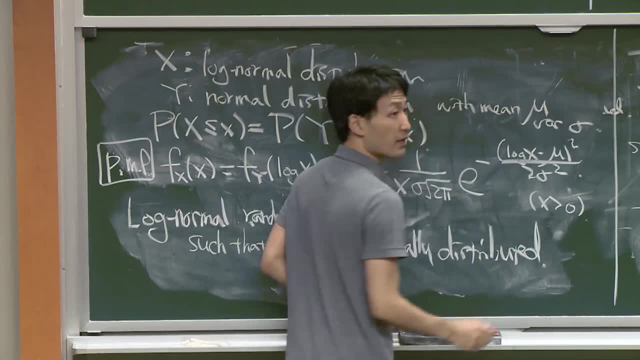 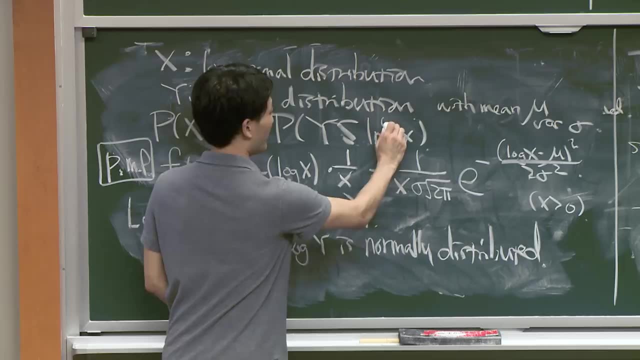 OK, OK, And that only works for x greater than 0.. OK, Yes, It looks like a natural log. Natural, Yeah, So all logs are natural logs. It should be log ln. Yeah, Thank you OK. 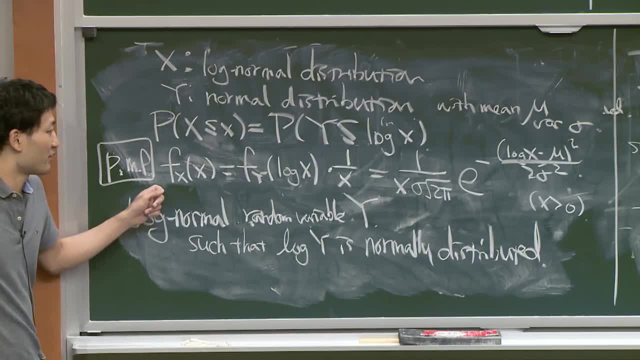 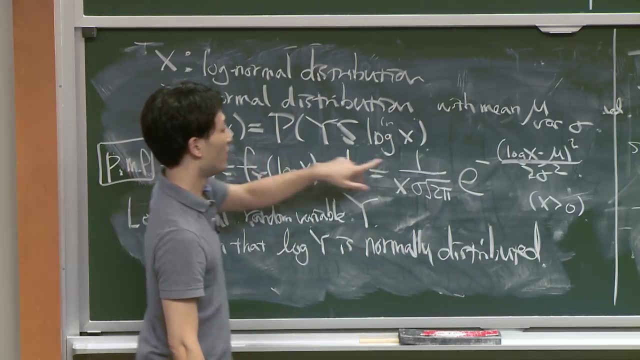 So question: What's the mean of this distribution here? Yes, 1.. Not 1.. Might be mu, Is it mu? Oh sorry, It might be e to the mu, because log x, The normal distribution, had mean mu. 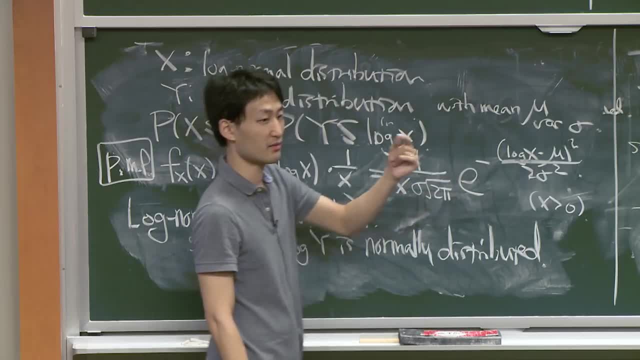 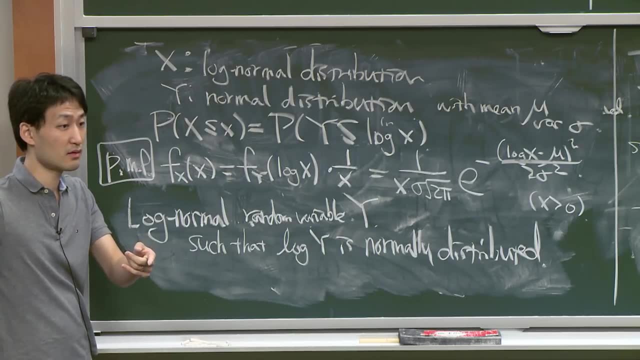 Log x equals mu might be the center. If that's the case, x is e to the mu will be the mean. Is that the case Yes, e to the mu minus 1 half to the first? Probably right, I don't remember what's there. 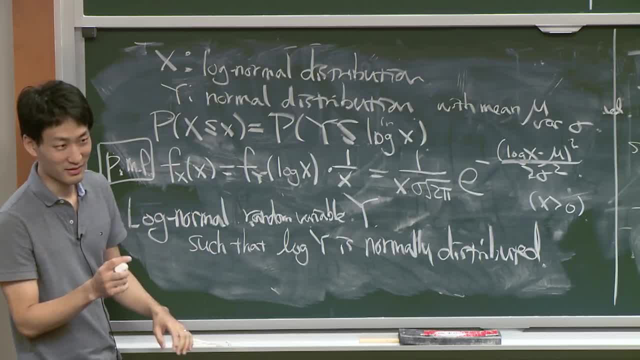 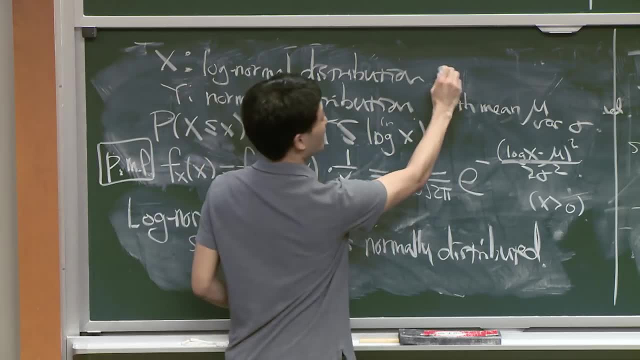 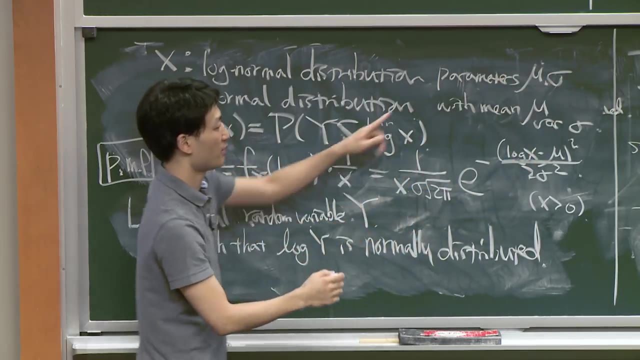 There is a correcting factor. I don't remember exactly what that is, but I think you're right, All right. So one very important thing to remember is: log normal distribution are referred to in terms of the parameters mu and sigma, because that's the mu and sigma appearing here coming. 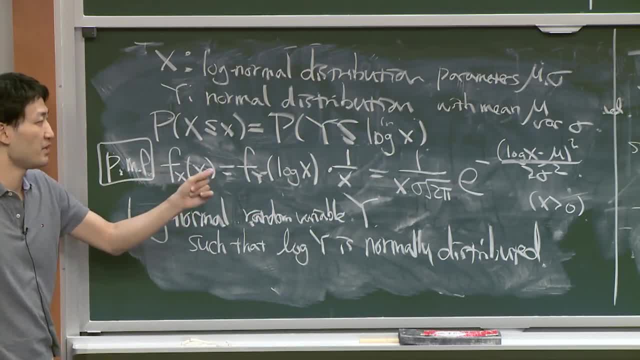 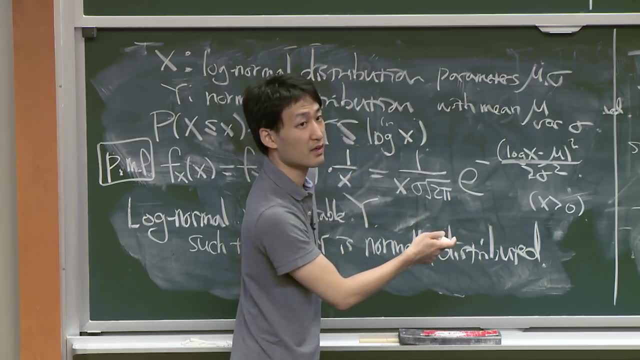 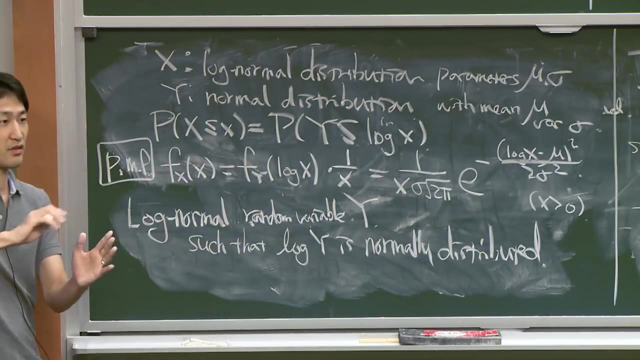 from the normal distribution. But those are not the mean and variance anymore, Because you skewed the distribution. it's no longer centered at mu, Log x, Log x, Log x is centered at mu, but when you take the exponential it becomes skewed and we take the average. 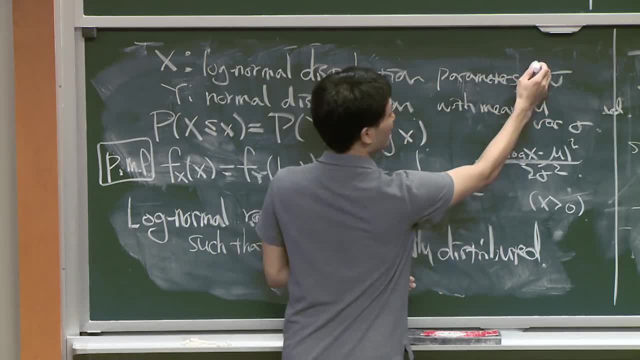 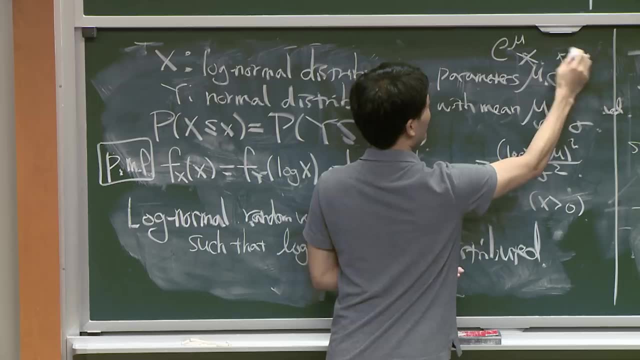 You'll see that the mean is no longer e to the mu. So that doesn't give the mean. That doesn't imply that the mean is e to the sigma, That doesn't imply that the variance is something like e to the sigma. I mean, that's totally nonsense. 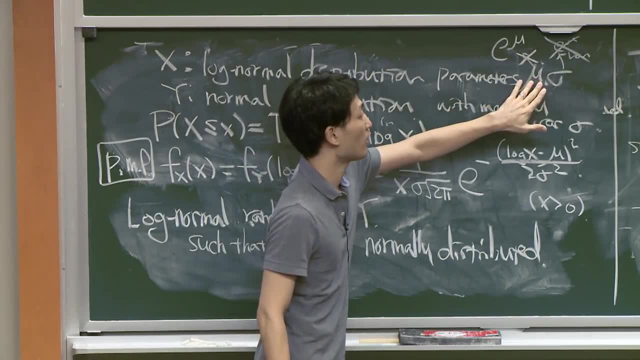 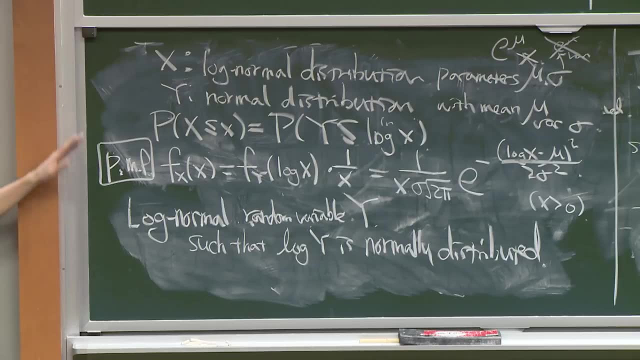 Just remember, these are just parameters, some parameters. It's no longer mean or variance And in your homework one exercise will ask you to compute the mean and variance of this random variable. But really just try to remember, Try to have it stick in your mind. 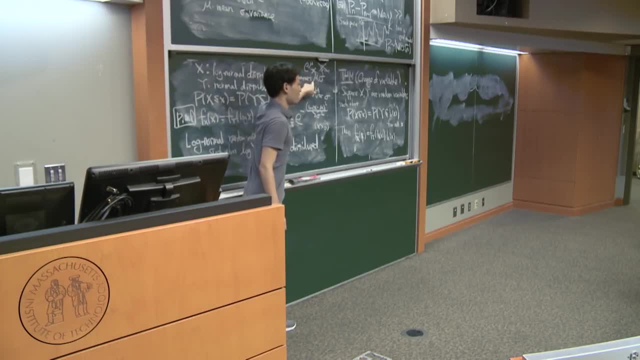 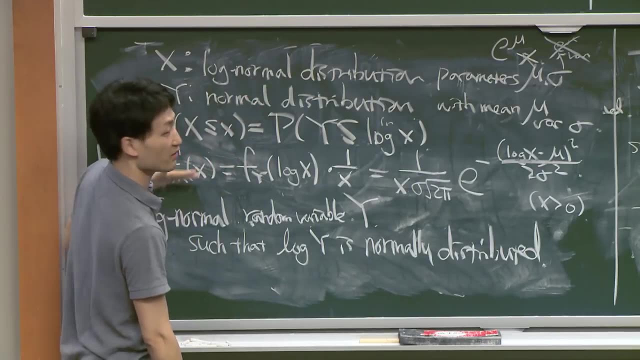 that mu and sigma is no longer mean and variance. That's only the case for normal random variables, And the reason we're still using mu and sigma is because of this derivation, And it's easy to describe it in this. All right, OK. 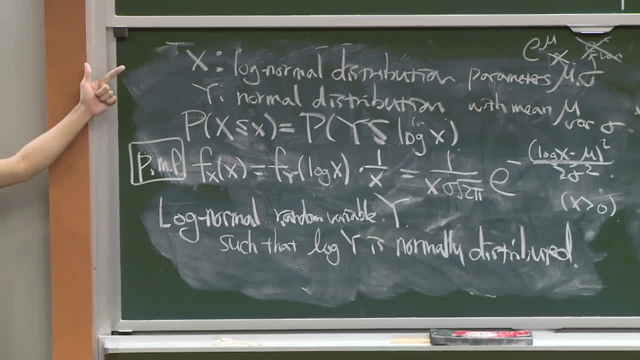 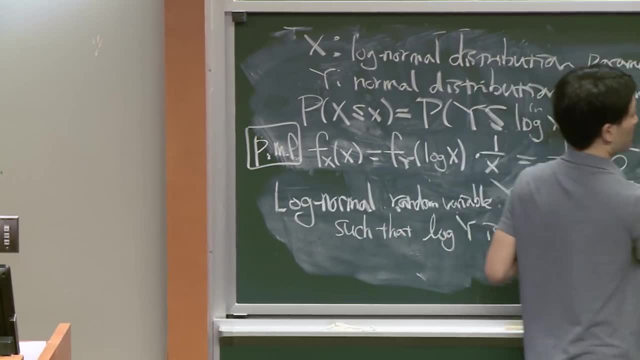 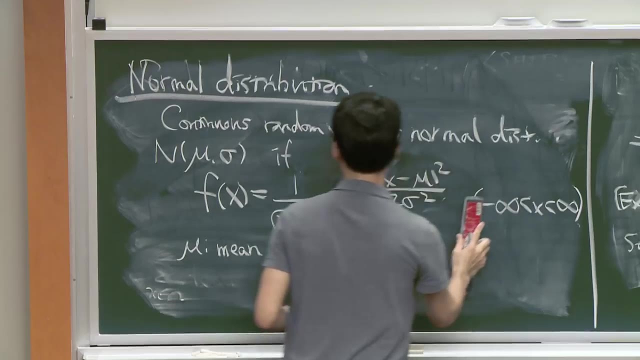 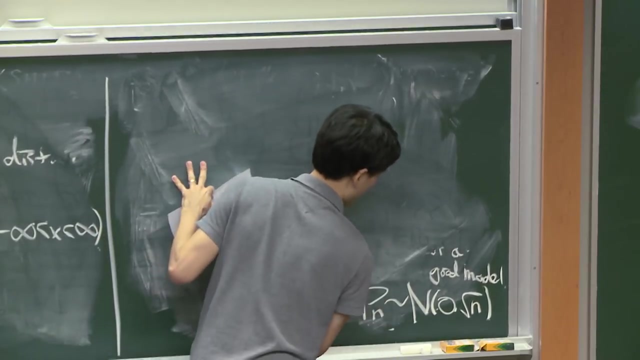 So this will be the normal distribution, And log-normal distribution will probably be the distribution that you'll see the most throughout the course, But there are some other distributions that you'll also see. I need this. I will not talk about it in detail. 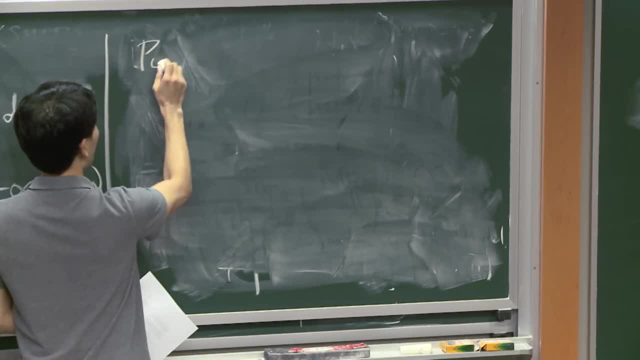 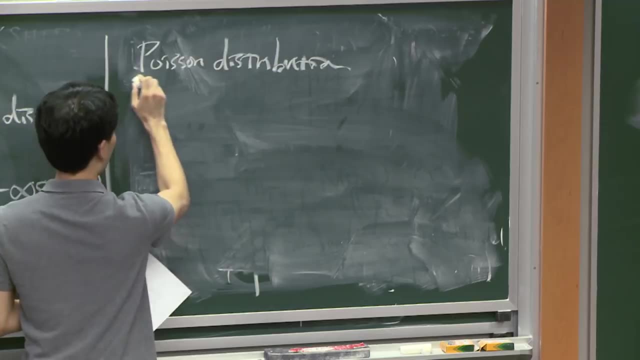 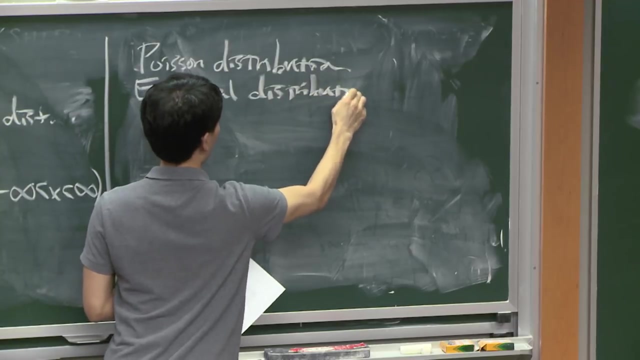 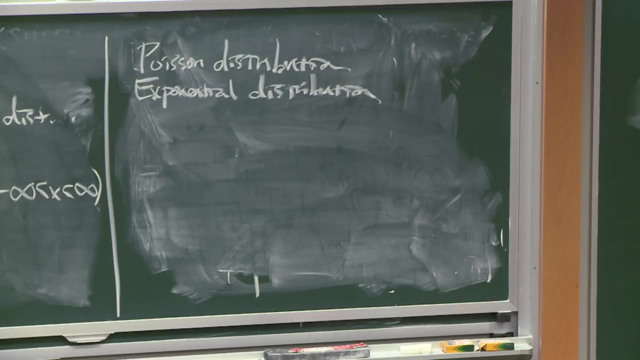 It will be some exercise questions. For example, you have Poisson distribution or exponential distributions. These are some other distributions that you'll see, And all of these normal, log-normal, Poisson, exponential and a lot more can be grouped. 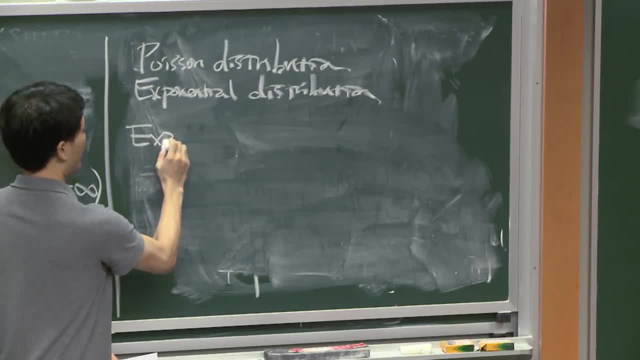 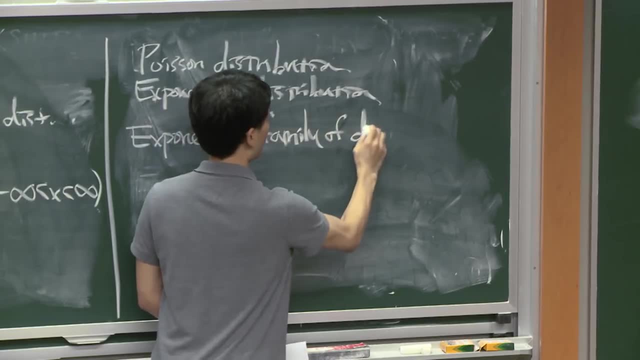 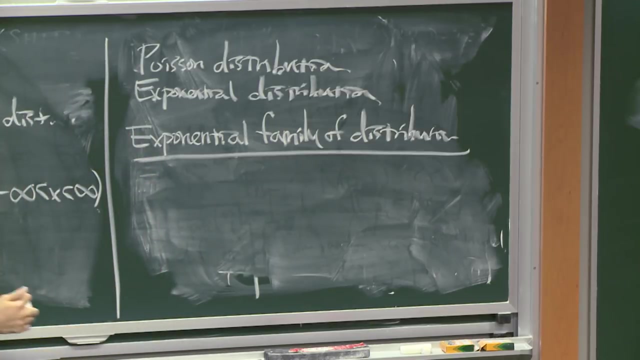 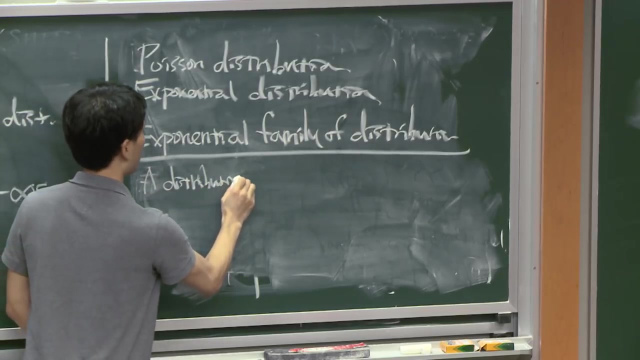 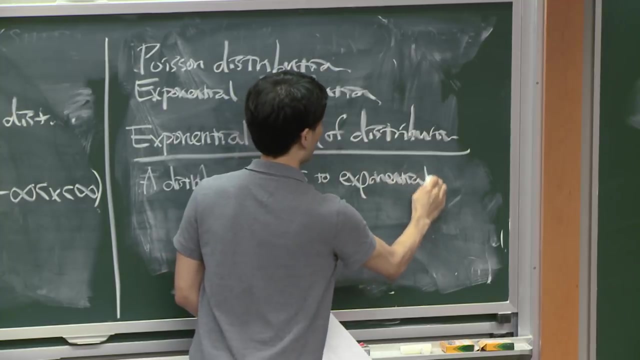 into a family of distributions called, for example, mu and sigma, And this is called the exponential family. So a distribution is called to be in an exponential family. A distribution belongs to exponential family. This is just a practical example, but probably we can be able to do better. 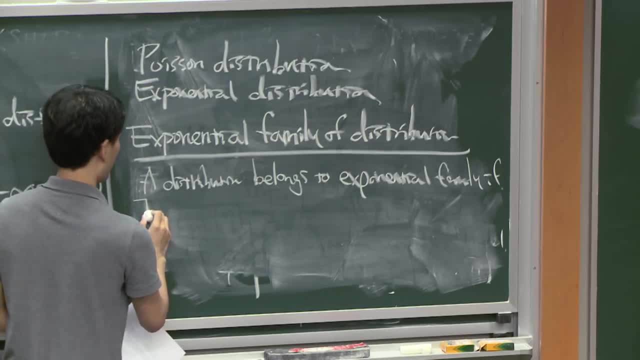 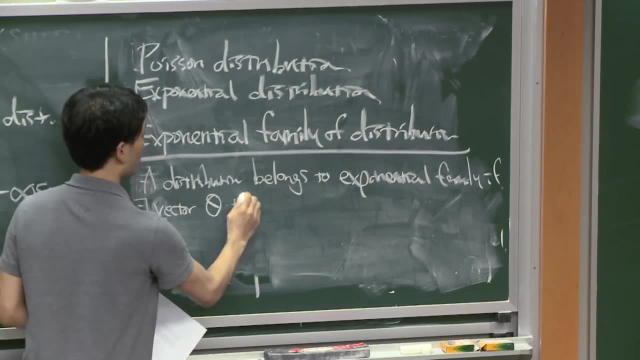 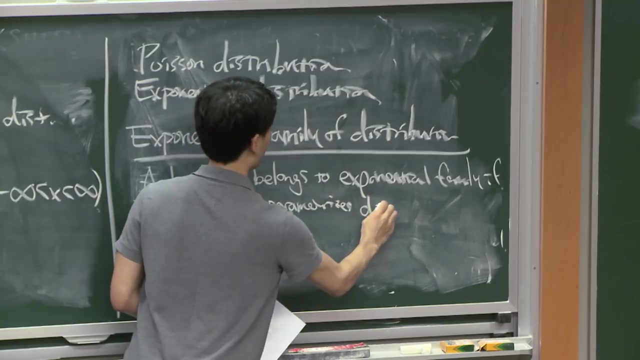 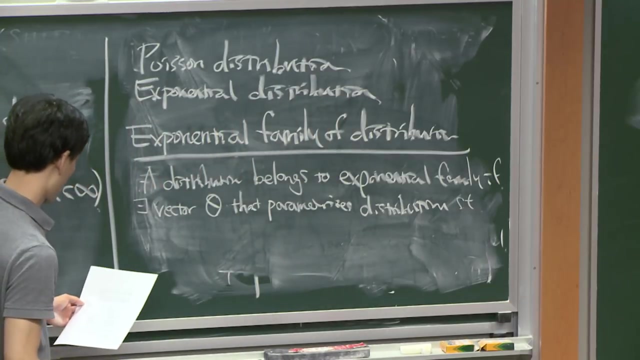 than this at some point, And there are other distributions that you'll see. So, for example, if there exists a theta, a vector that parametrizes the distribution, such that the parameter sigma, where the theta is, is constant, 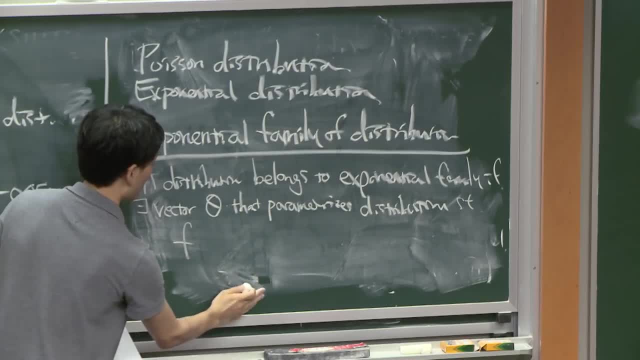 And so that's going to be the distribution. So this is going to be a function And we're going to use it to define the distribution that I'll show you later. And we'll show you later Probability density function for this choice of parameter: theta. 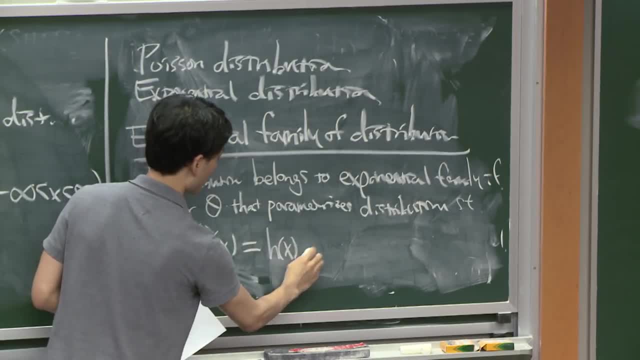 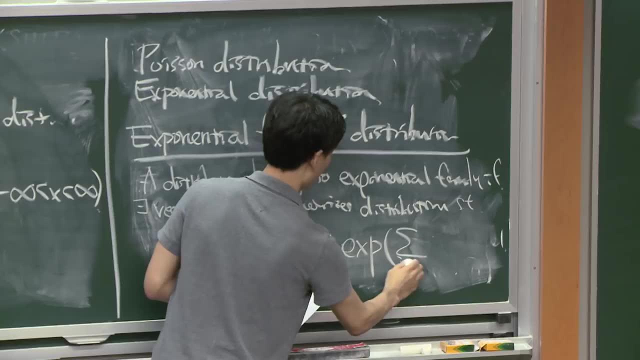 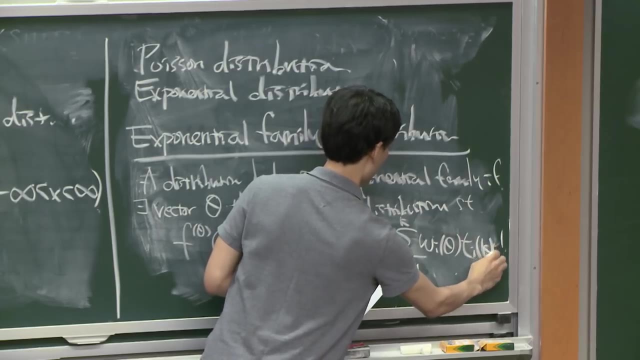 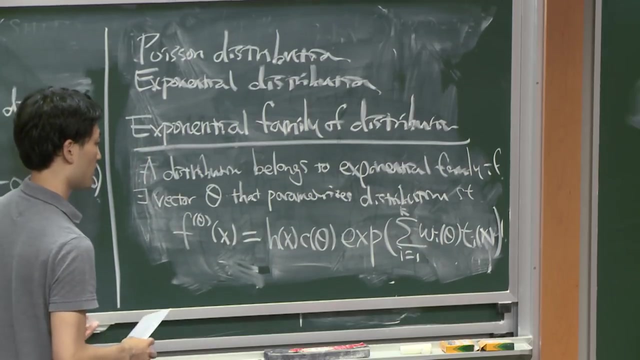 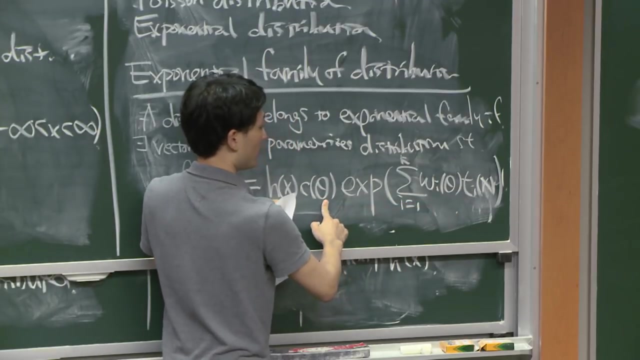 can be written as h of x times c of theta times exponent of sum from i equal 1 to k of x. So here, when I write only x, x should only depend on x, not on theta. When I write some function of theta, 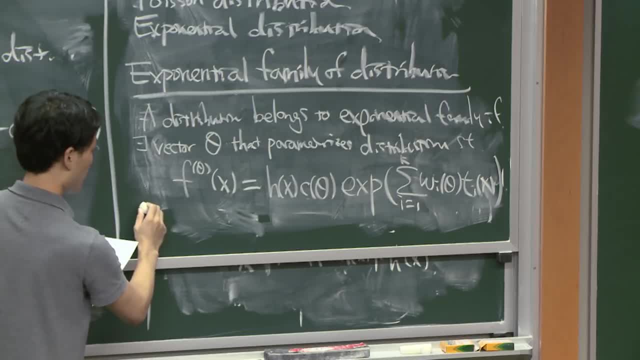 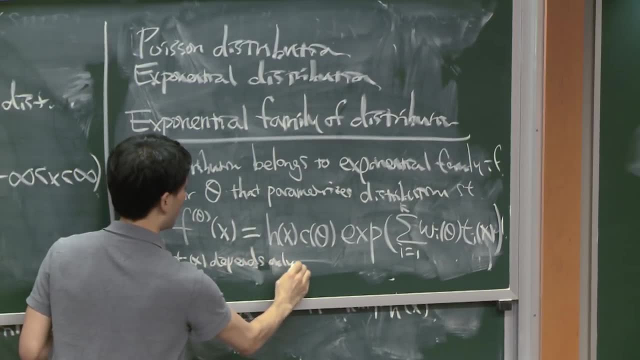 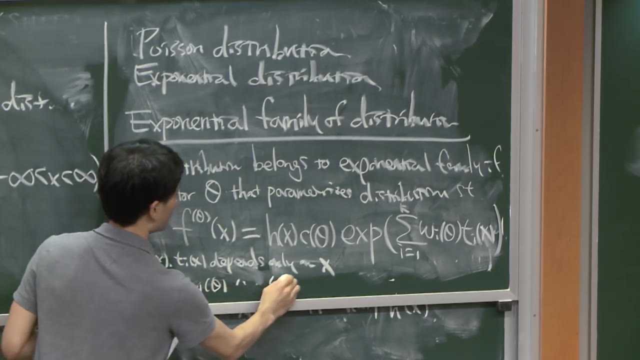 it should only depend on theta, not on x. So h x, t, i x depends only on x And c theta and i theta depends only on theta. That's some abstract thing. It's not clear why this is so useful. at least. 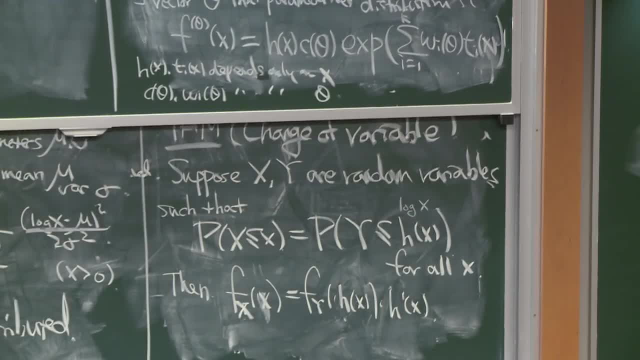 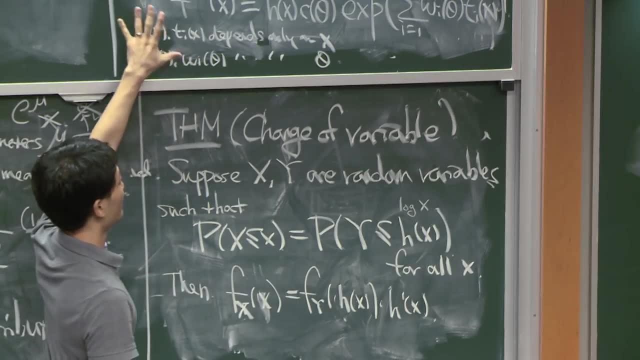 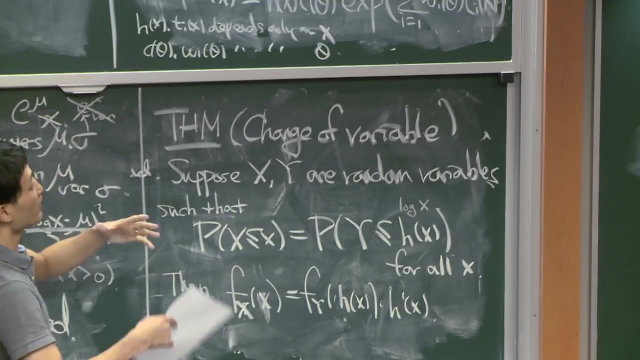 from the definition, But you're going to talk about some distributions and explanations. Yeah, So you will see something about this. But one good thing is they exhibit some good statistical behavior When you group them into all distributions in the exponential family, have some nice statistical. 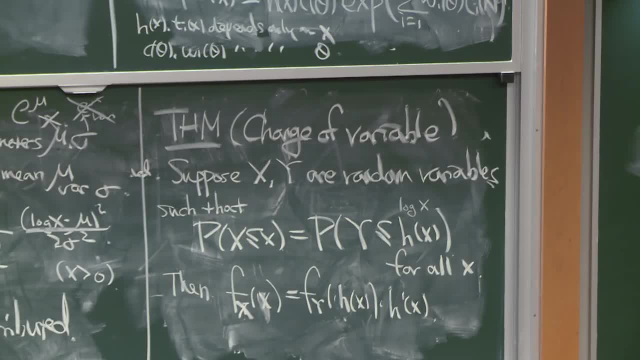 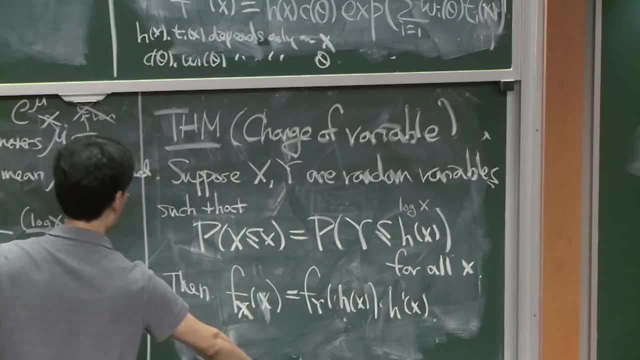 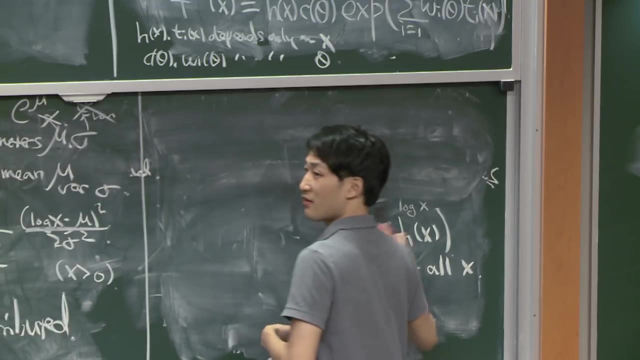 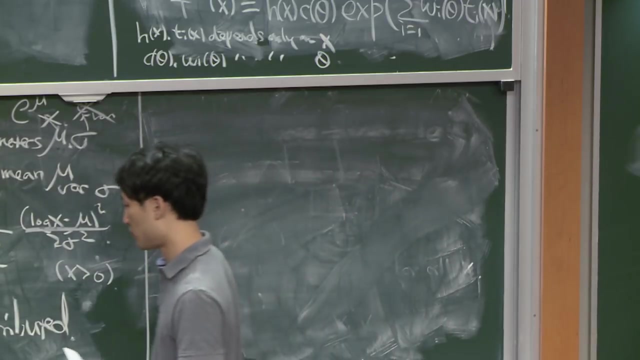 properties, which makes it good. That's too abstract. Let's see how log normal distribution actually falls into the exponential family. So we'll come to this comment with the notion of independent random variables. You went over how the probability density functions of collections of random variables. 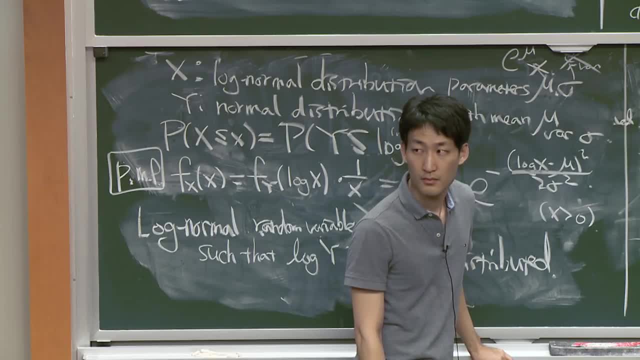 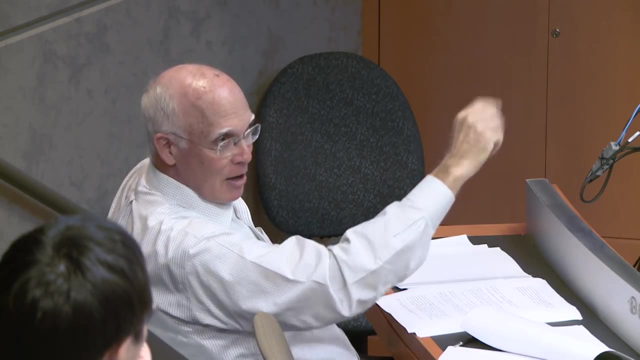 if they're mutually independent, is the product of the probability densities of the individual variables. And so, with this exponential family, if you have random variables from the same exponential family, products of this density function, which is the same function, factor out into a very simple form: 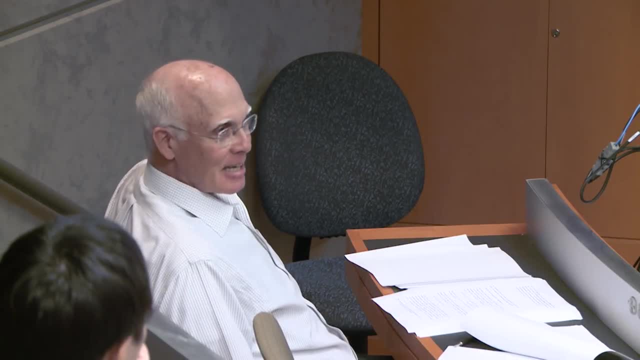 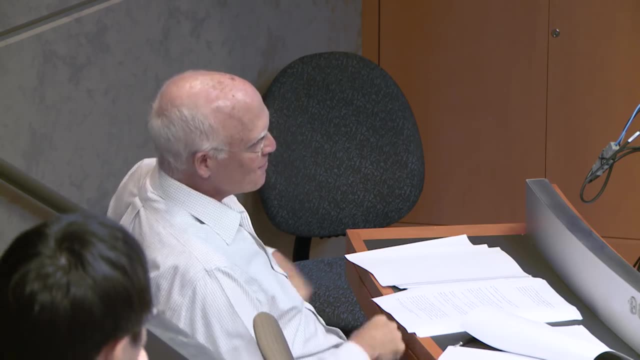 It doesn't get more complicated as you look at the joint density of many variables And in fact simplifies to the same exponential family. So that's where that becomes very useful. So it's designed so that it factors out when it's multiplied. 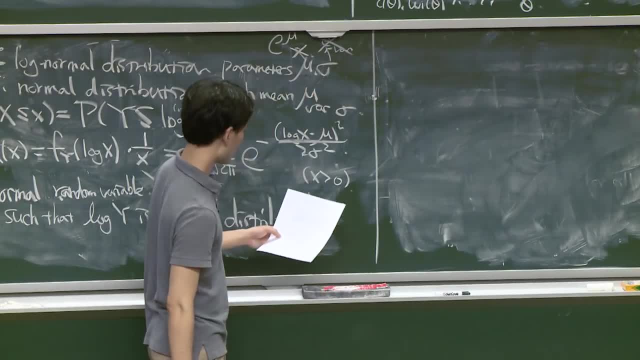 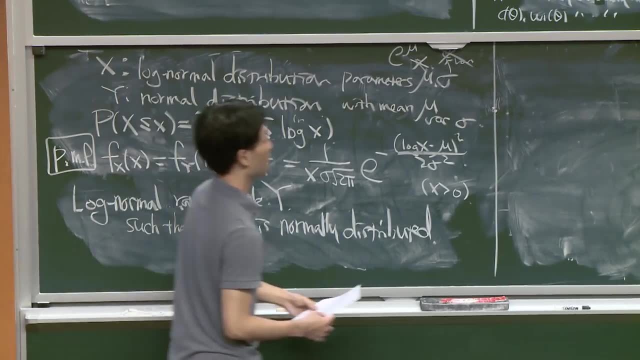 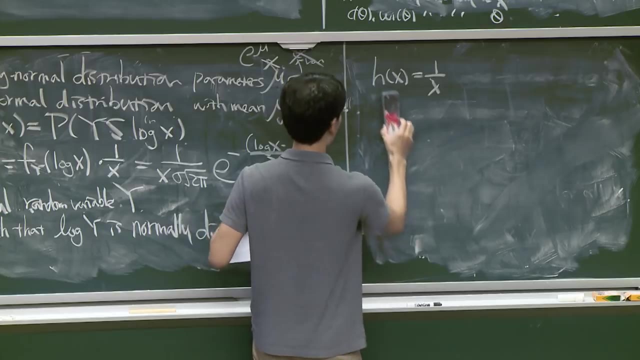 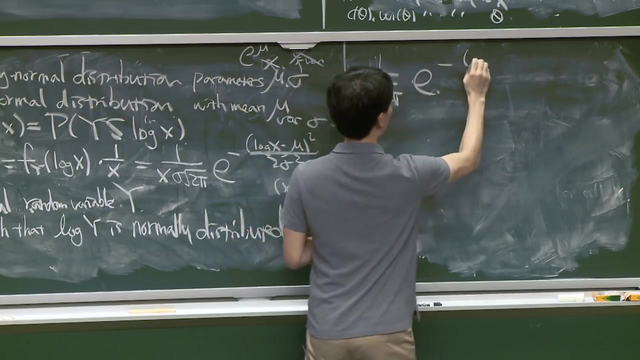 So it factors out well, OK, So sorry about that. Yeah, Log normal distribution. So take h of x, 1 over x Before that, let's just rewrite that in a different way. So 1 over x, sigma squared. 2 pi e to the minus log x squared. 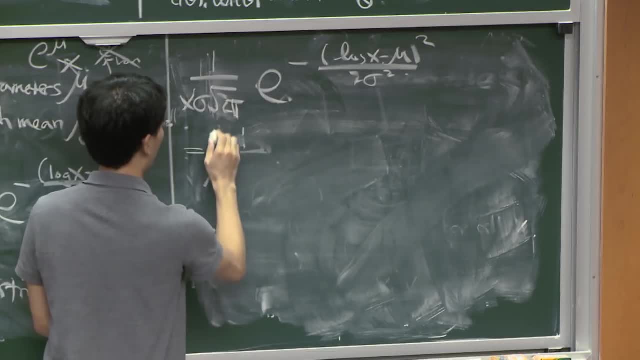 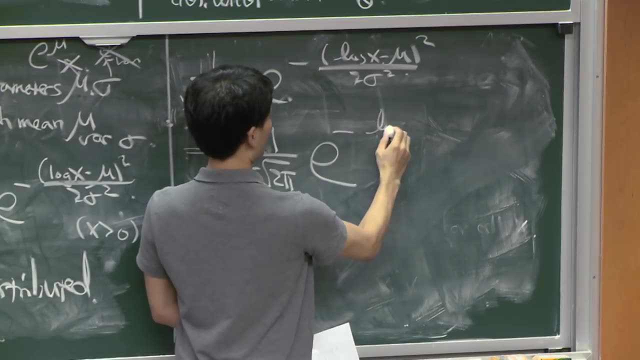 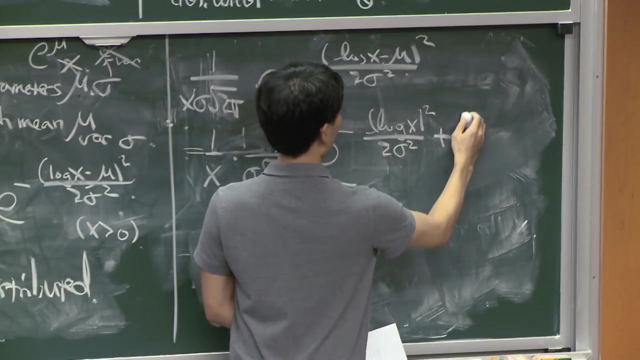 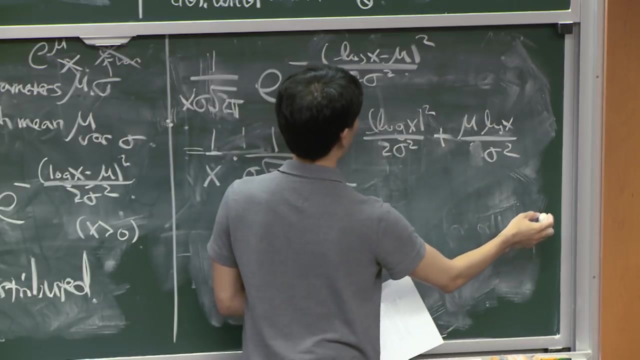 can be rewritten as 1 over x times 1 over sigma squared. 2 pi e to the minus log x squared. OK, OK, OK, OK, OK OK. Square over 2 sigma squared plus mu log x over sigma squared minus mu squared. 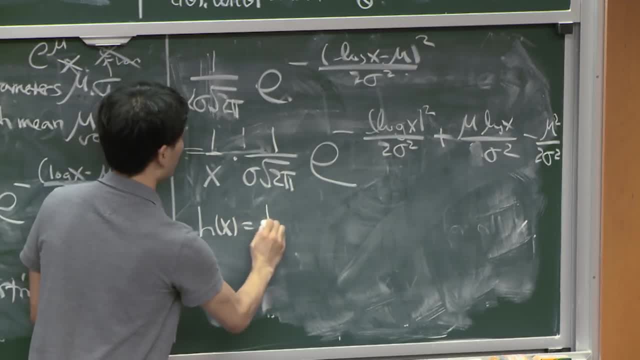 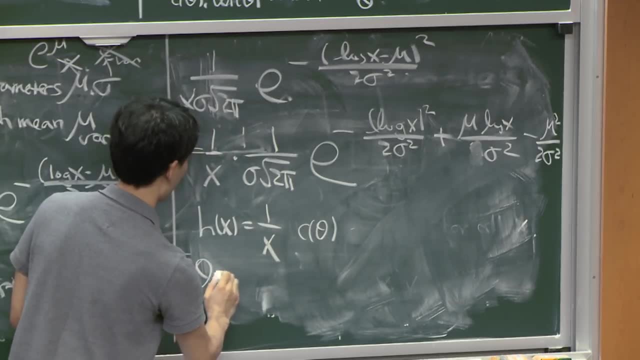 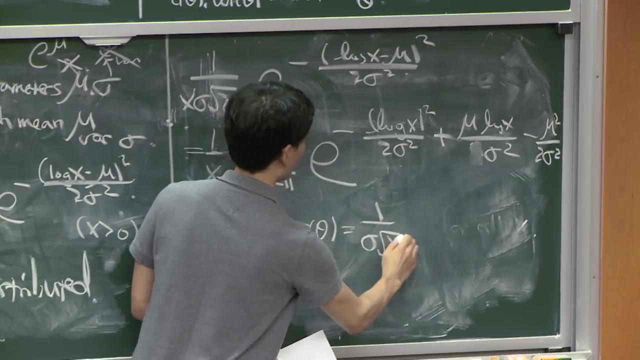 To write it like that: set up: hx equals 1 over x c of theta. Oh, sorry, You have to first let theta equals mu sigma, Then c. theta is equal to 1 over sigma squared 2, pi e to the minus mu squared squared. 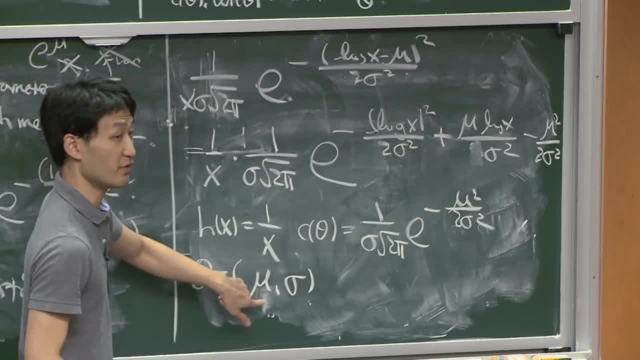 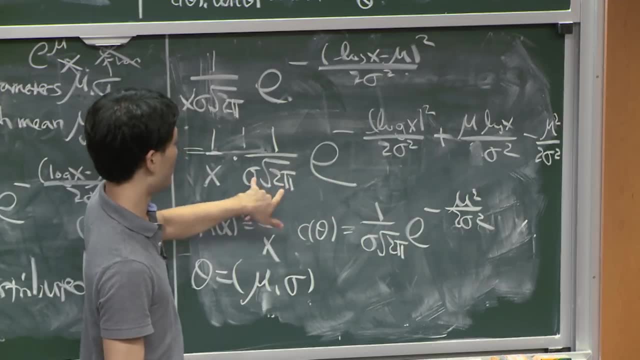 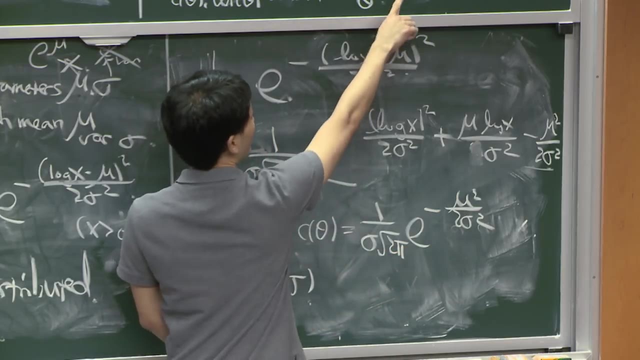 OK, So you will parametrize this family in terms of mu and sigma. Your h of x here will be 1 over x. Your c, theta, will be this term and the last term here, because this doesn't depend on x. And then you have to figure out what w and t is. 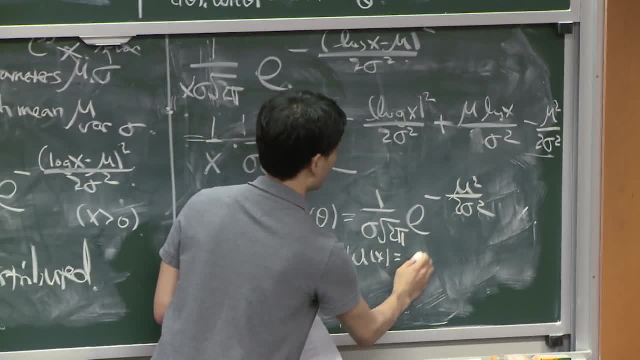 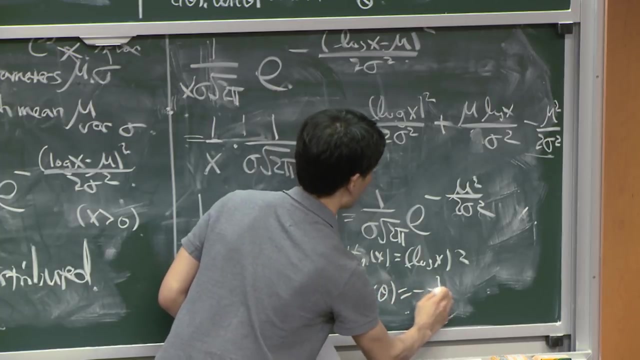 You can let w1 of x be log x squared: See t1.. Oh no, t1 of x be log x squared, w1 of theta be minus 1 over 2 sigma squared. And similarly you can let t2 equals log x. 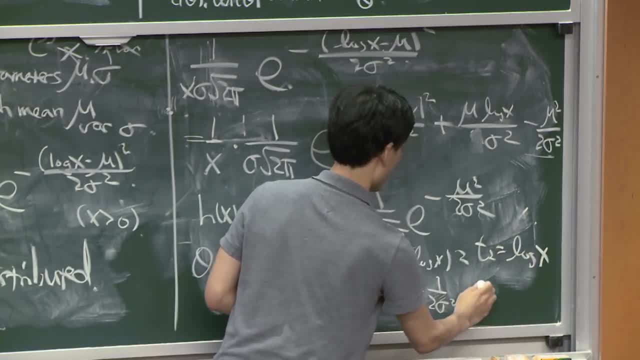 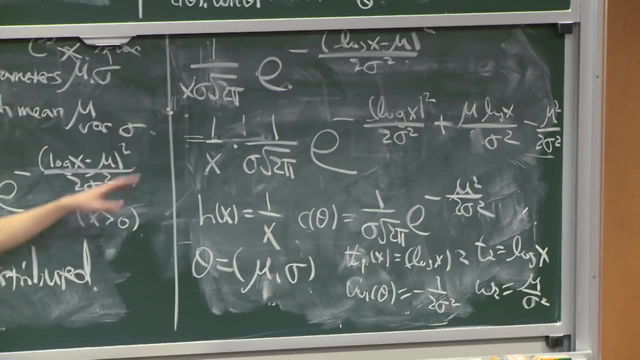 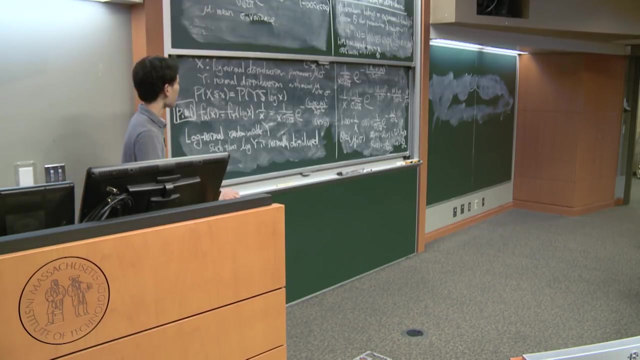 And w2 equals mu over sigma. It's just some technicality, but at least you can see that it really fits in, OK. So that's all about distributions that I want to talk about, And then let's talk a little bit more about more interesting. 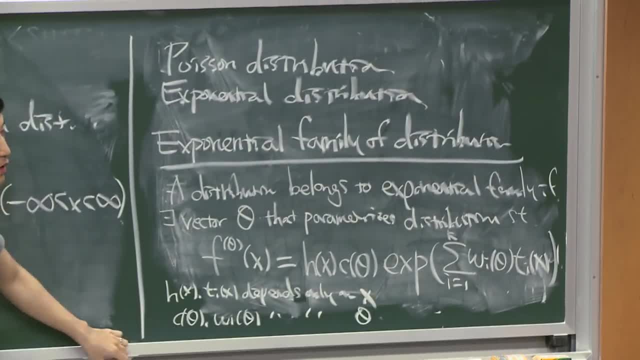 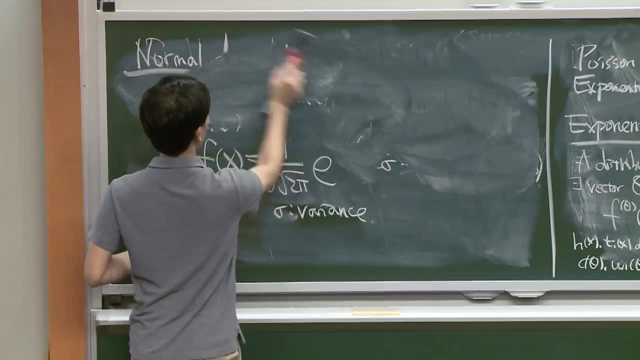 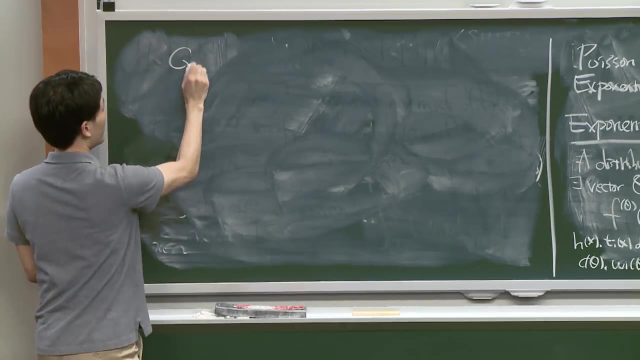 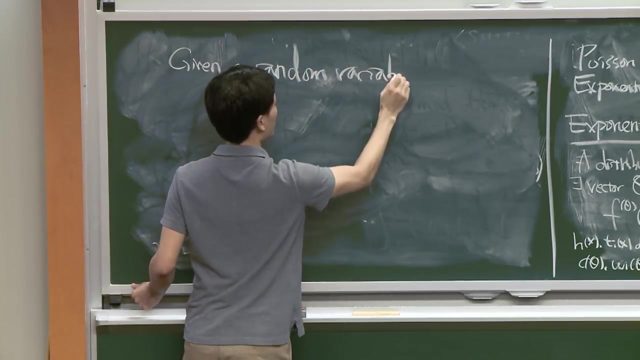 stuff. In my opinion, I like these stuff better. There are two main things that we're interested in When we have a random variable, at least for our purpose, what we want to study is: given a random variable first, we want to study its statistics. 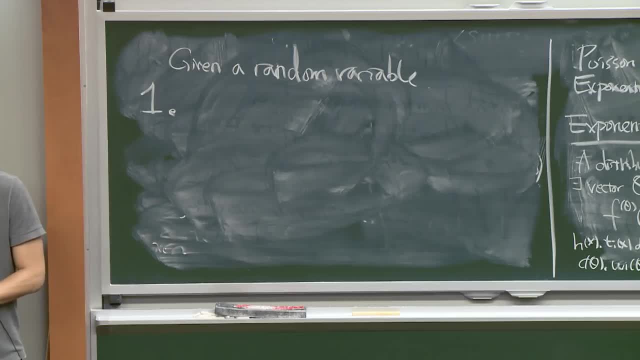 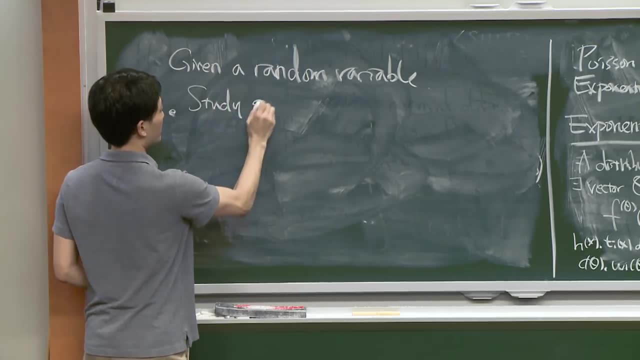 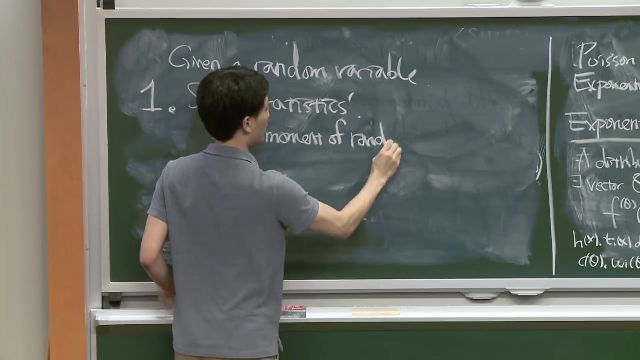 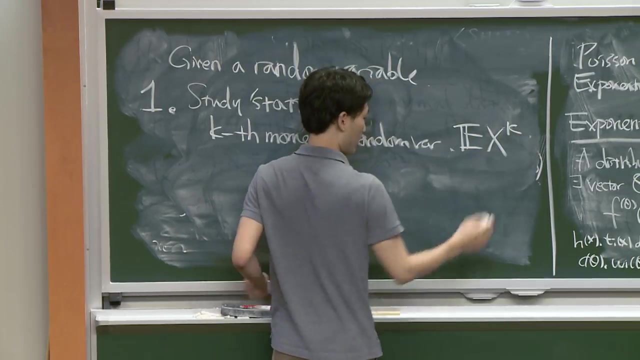 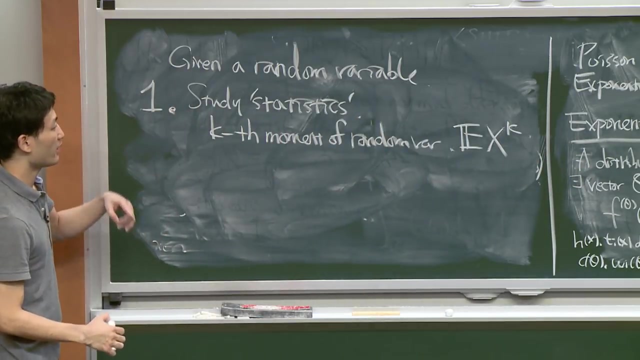 So we want to study its statistics, whatever that means, And that will be represented by the case moments of the random variable. Our case moment is defined as expectation Expectation of x to the k, And a good way to study all the moments. 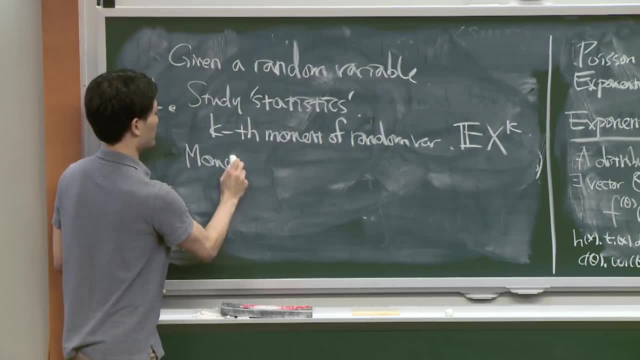 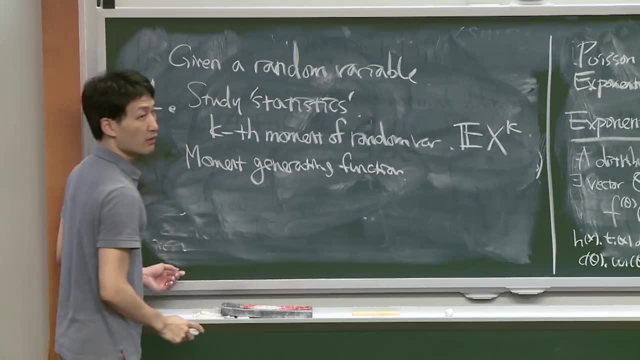 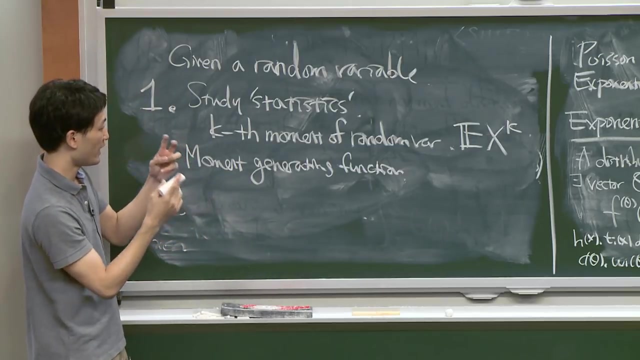 together in one function is a moment-generating function. So this moment-generating function encodes all the case moments of a random variable, So it contains all the statistical information of a random variable. That's why moment-generating function will be interesting to us, because when 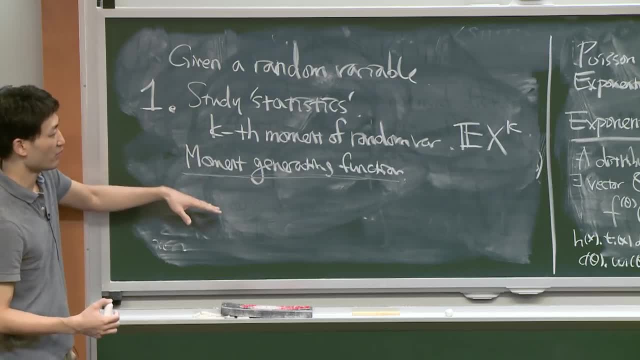 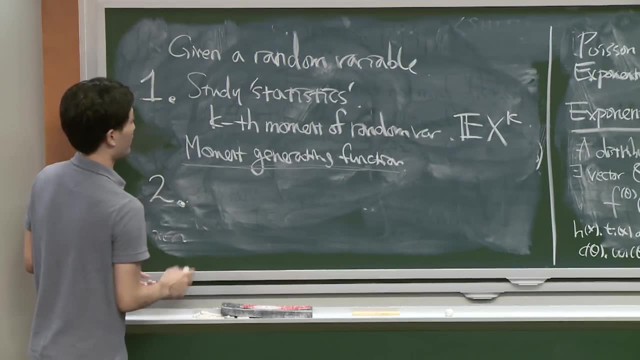 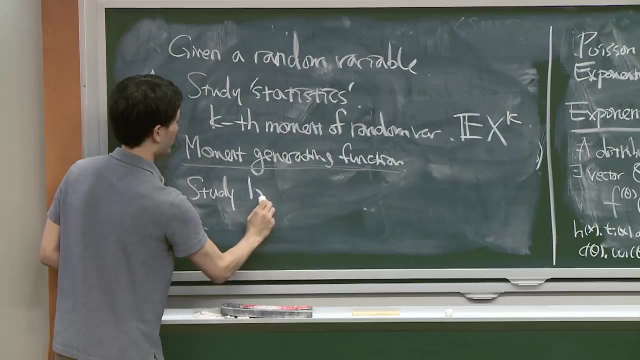 you want to study it. you don't have to consider each moment separately. It gives some unified way. It gives a very good feeling about your function. That will be our first topic. Our second topic will be: we want to study its long-term- yes, kind of long-term- our large 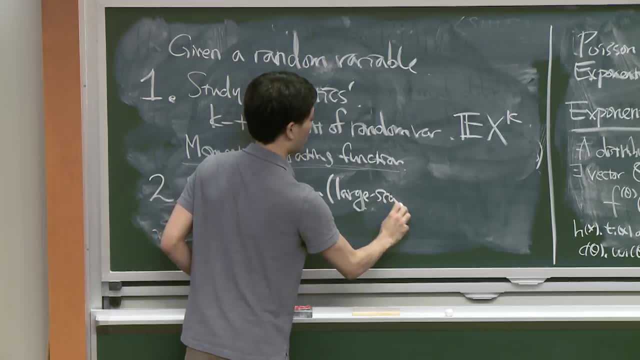 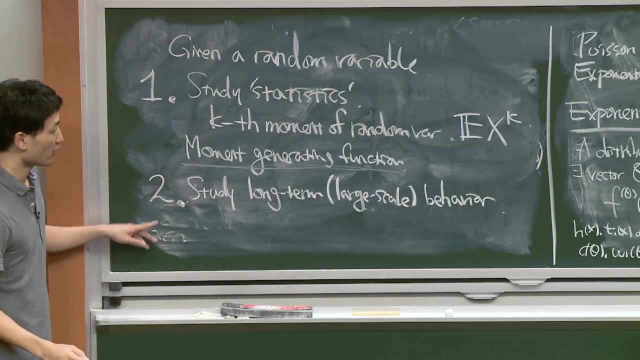 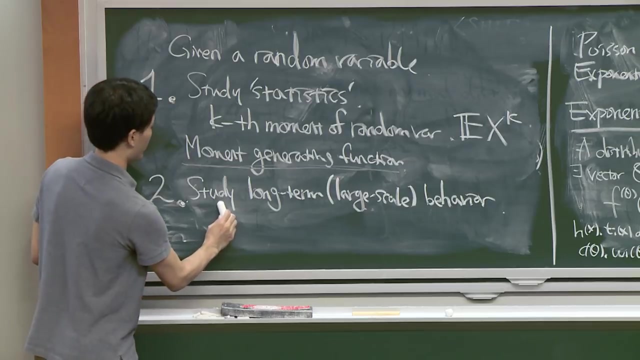 our large-scale behavior. So, for example, assume that you have a normal distribution, one random variable's normal distribution. If you just have a single random variable, you really have no control. It can be anywhere, The outcome can be anything according to that distribution. 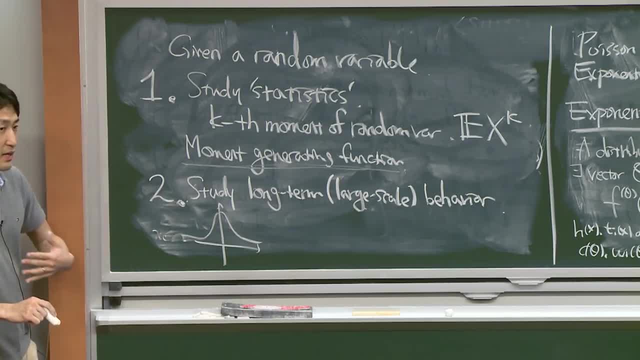 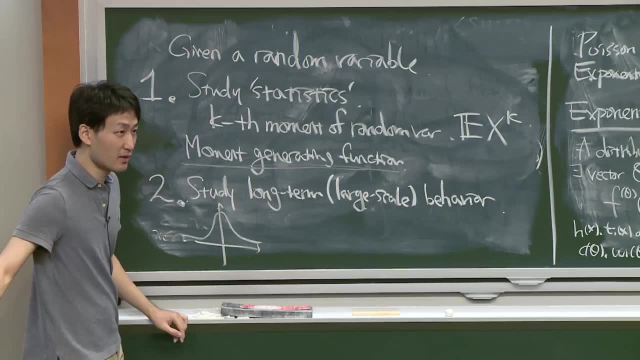 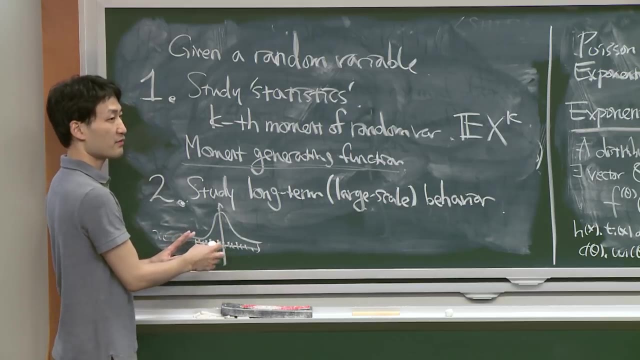 But if you have several independent random variables with the exact same distribution, if the number is super large- let's say 100 million- and you plot how many random variables fall into each point into a graph, you'll know that it has to look very close to this curve. 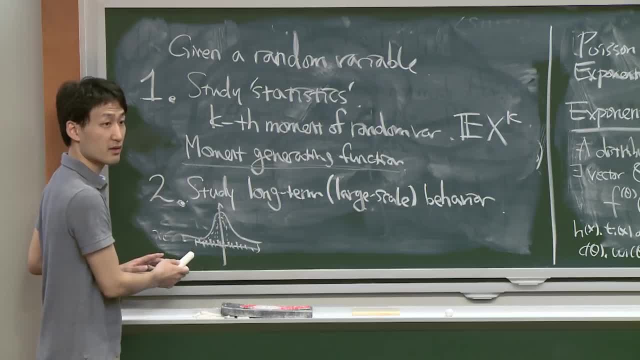 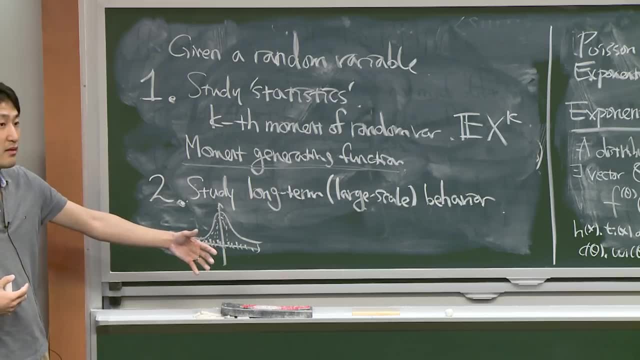 It will be more dense here, sparser there and sparser there. So you don't have individual control, You don't have control on each of the random variables. But when you look at large scale you know, at least with very high probability. 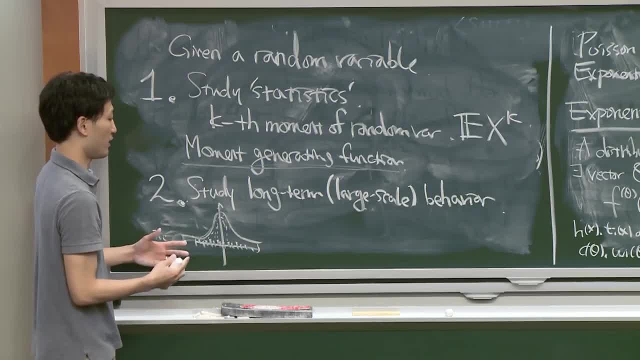 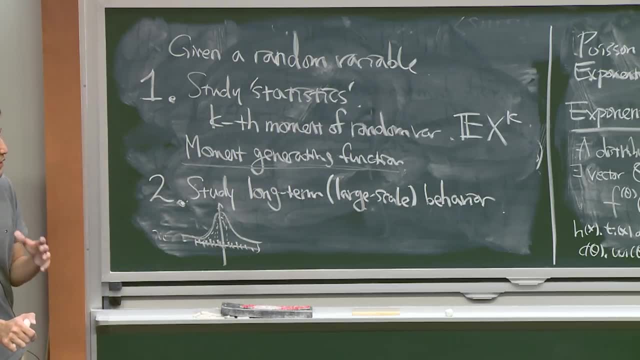 it has to look like this curve. Those kind of things are what we want to study. When we look at this long-term behavior, large-scale behavior, what can we say? What kind of events are guaranteed to happen with probability, let's say, 99.9%? 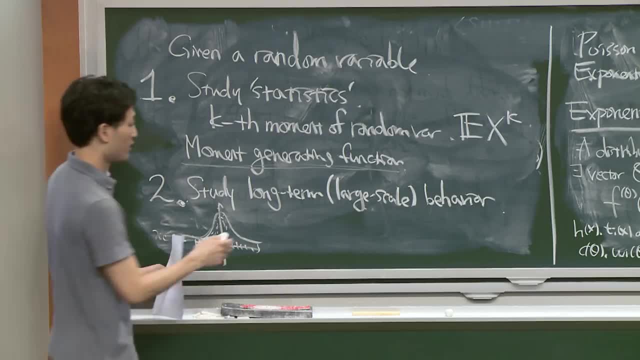 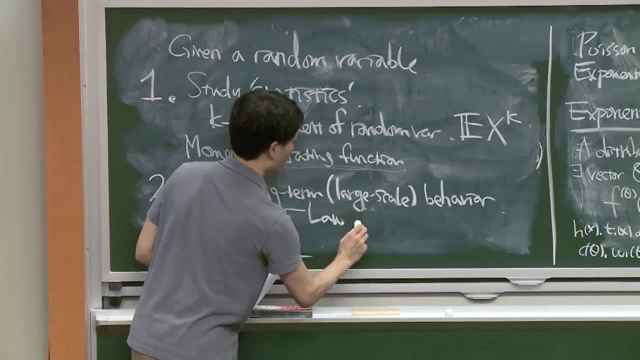 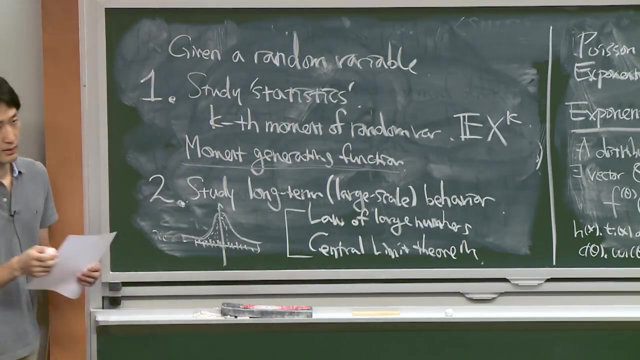 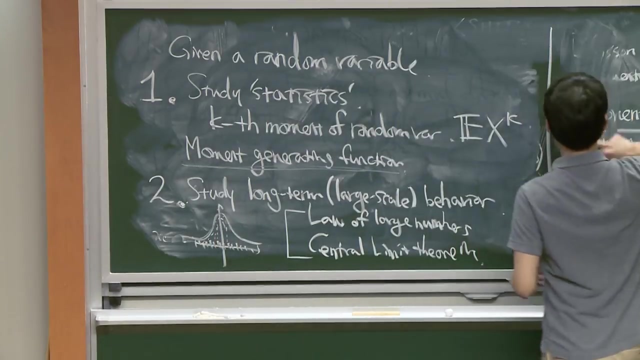 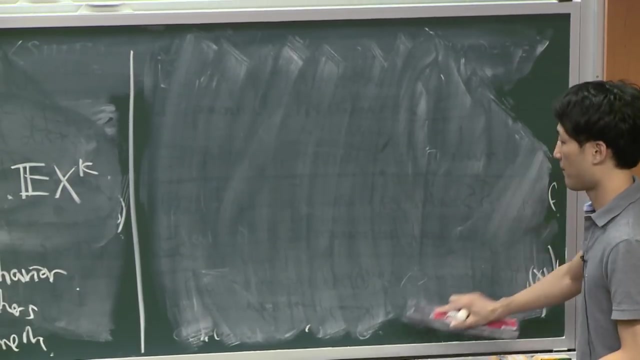 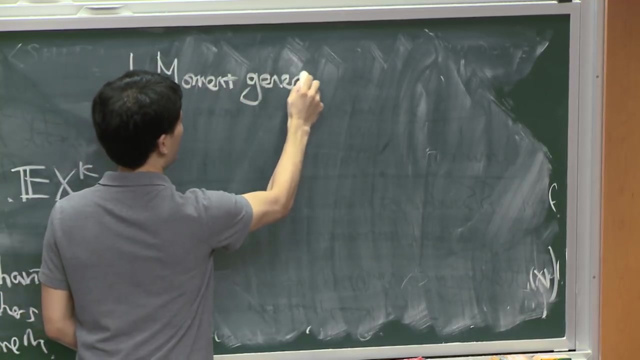 Things are happening. As you might already know, two typical theorems of this type in this topic will be law of large numbers and central limit theorem. So let's start with our first topic, the moment-generating function. The moment-generating function of a random variable. 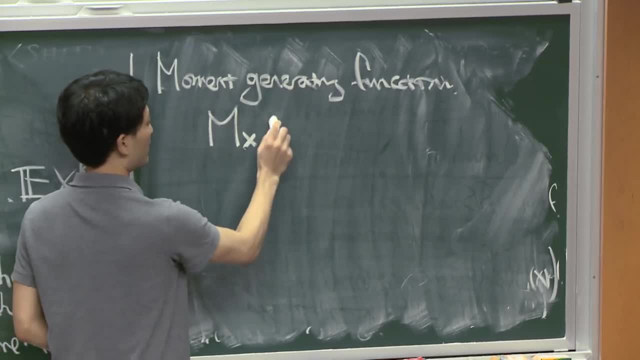 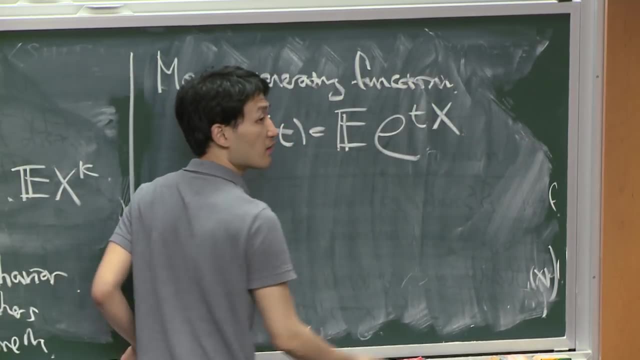 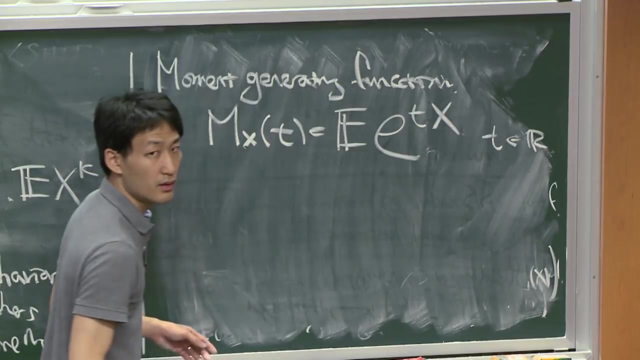 is defined, as I write it, as m sub x. It's defined as e to the expectation of e to the t times, x where t is some parameter. t can be any real. You have to be careful, It doesn't always converge. 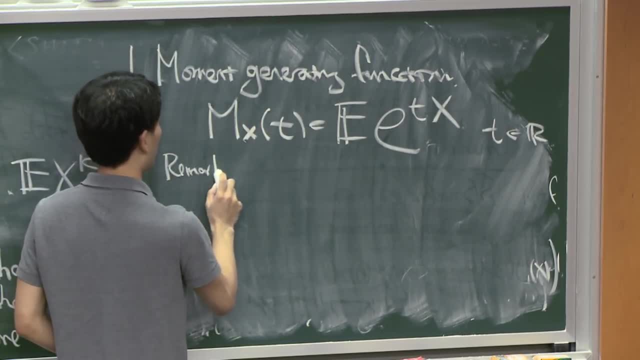 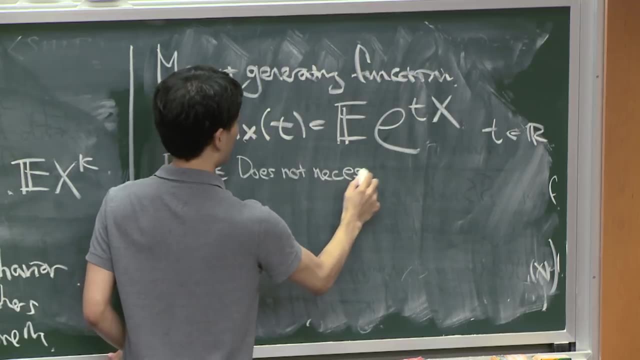 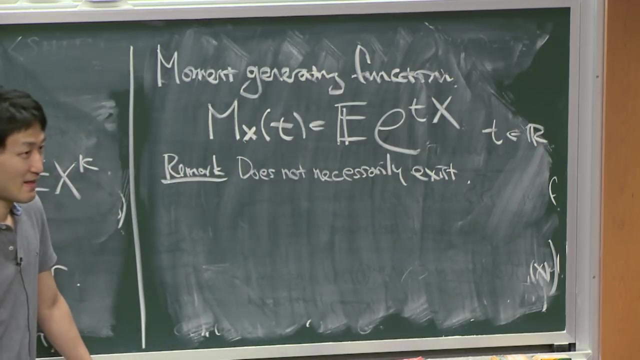 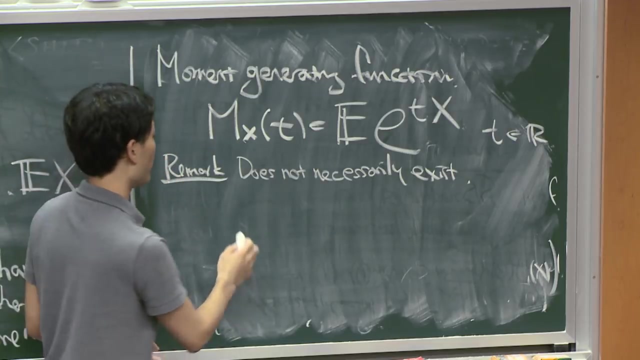 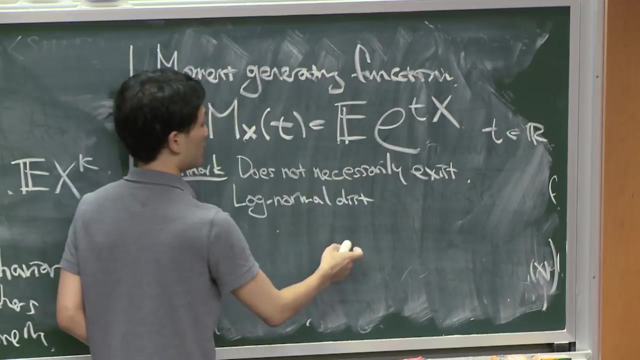 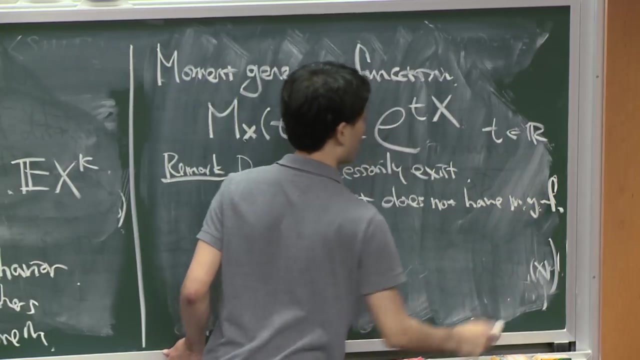 So remark does not necessarily exist, Do not necessarily exist, Yeah. So, for example, one of the distributions you already saw does not have moment-generating function. The log-normal distribution does not have any moment-generating function. That's one thing you have to be careful. 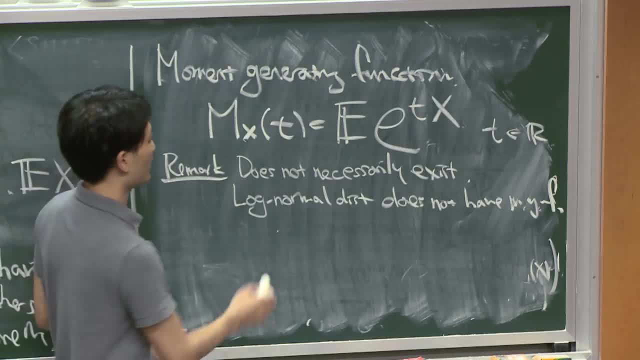 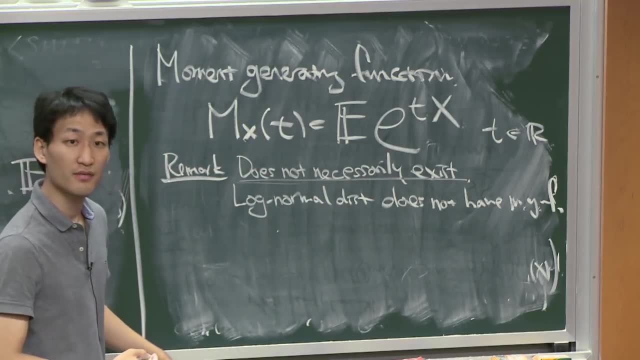 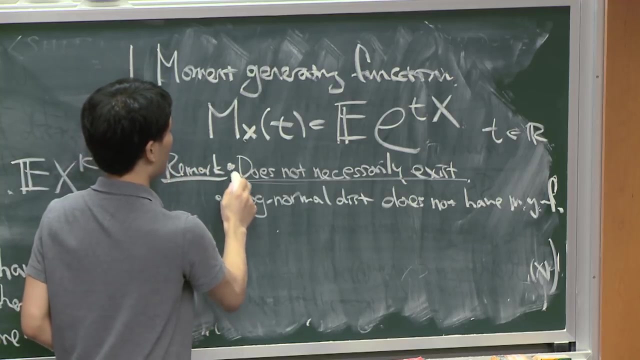 It's not just some theoretical thing. This statement is not something theoretical. It actually happens for some random variables that you encounter in real life, So be careful, And that will actually show some very interesting things. I'll later explain Some very interesting facts. 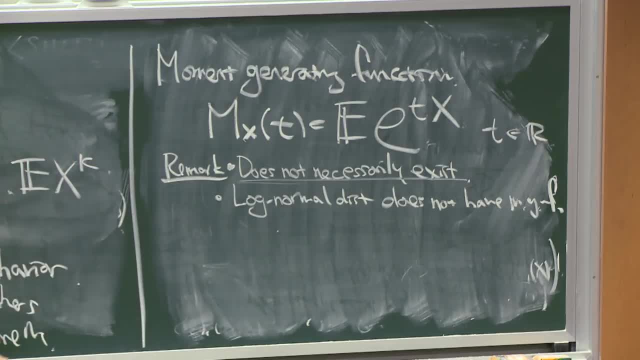 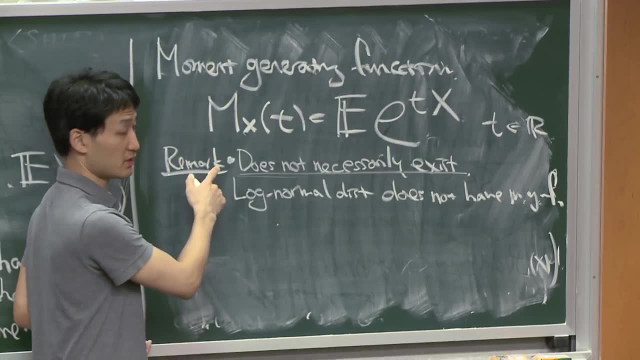 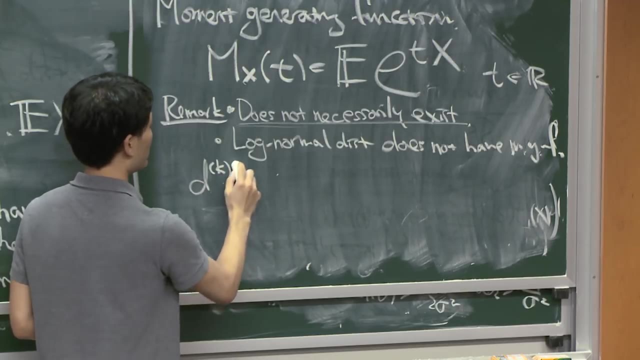 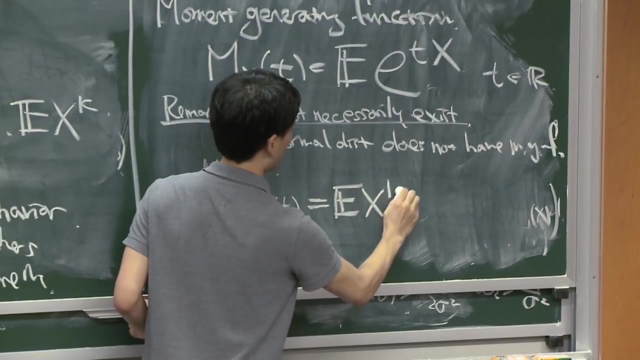 Some very interesting facts arise from this fact. Before going into that, first of all, why is it called moment-generating function? It's because if you take the case derivative of this function, then it actually gives the case moment. It gives the case moment of your random variable. 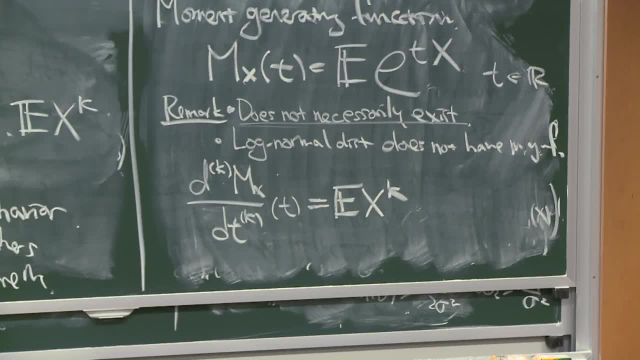 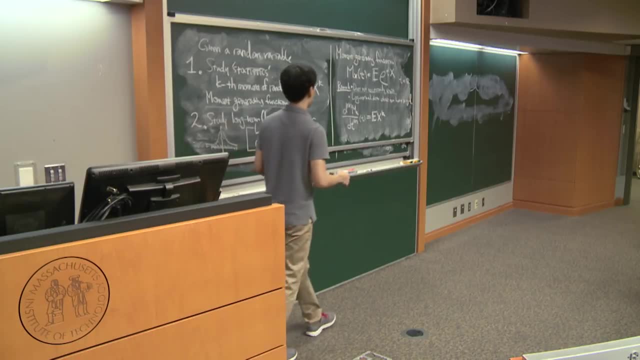 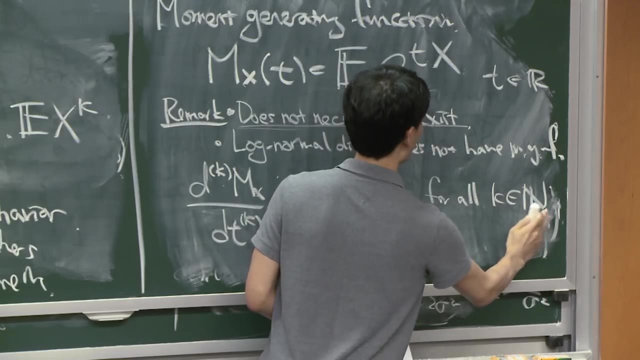 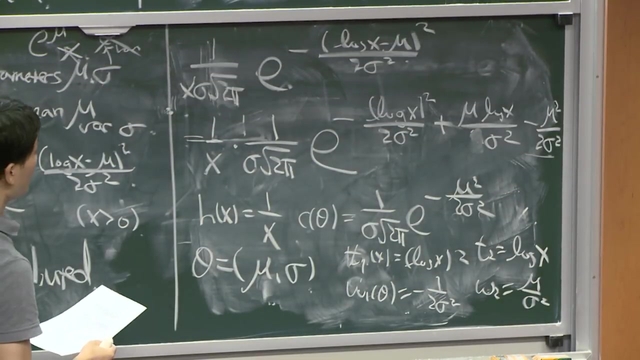 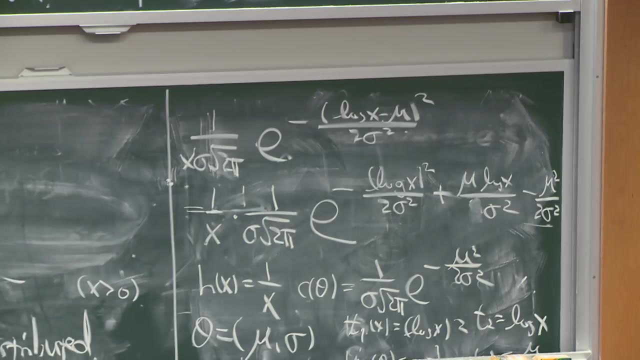 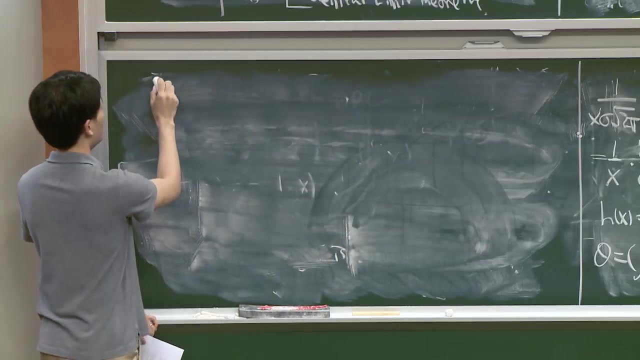 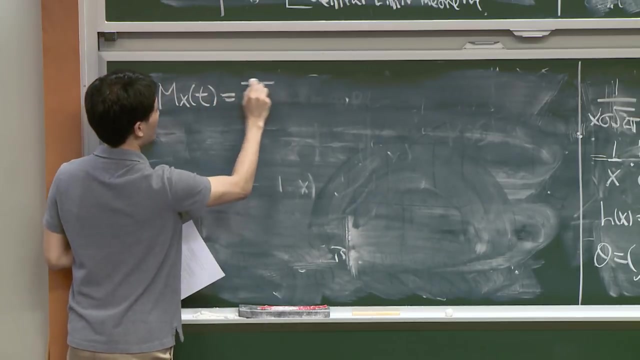 That's where the name comes from, For all integers, OK, And that gives a different way of writing a moment-generating function. So because of that we may write the moment-generating function as the sum from k equals 0 to infinity, t to the k, k factorial. 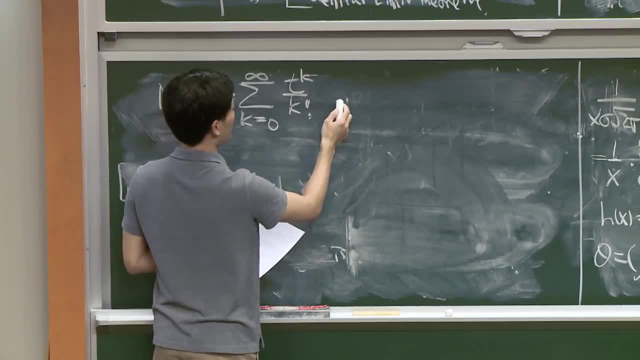 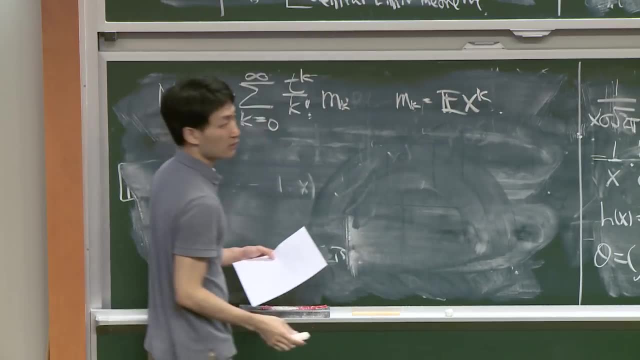 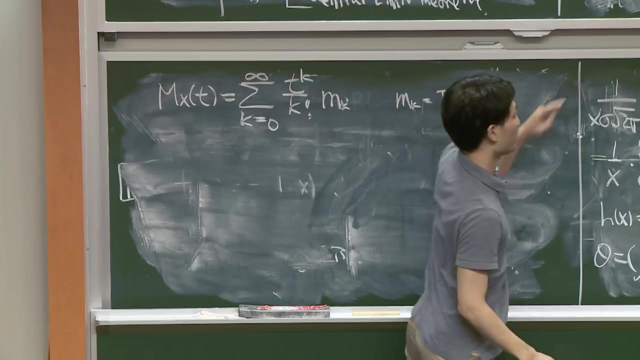 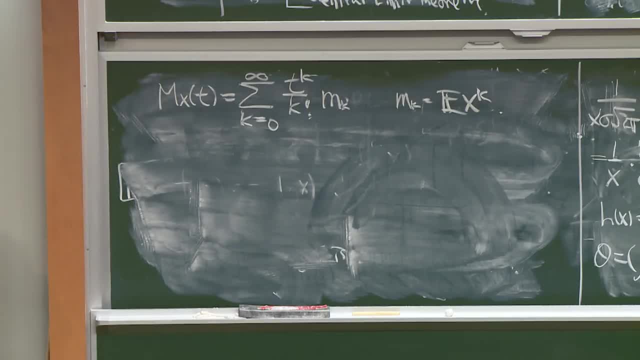 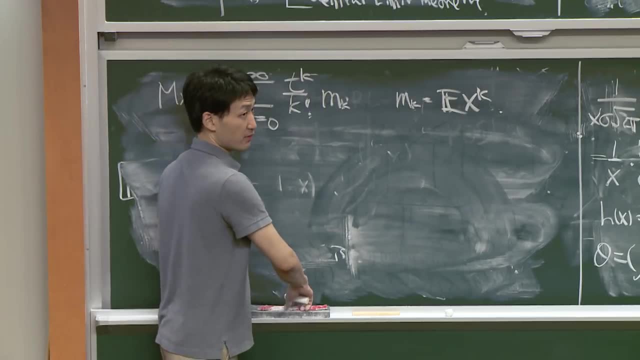 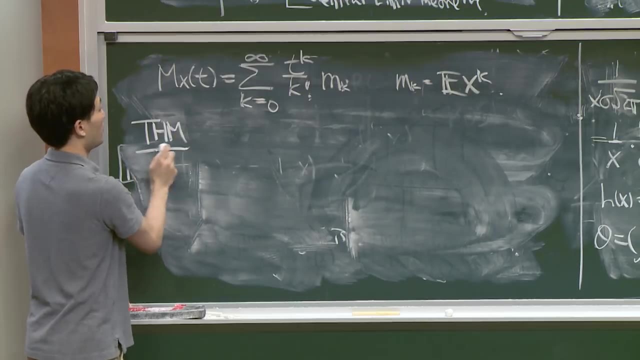 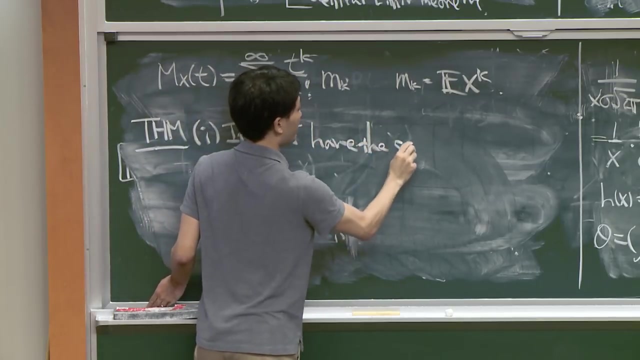 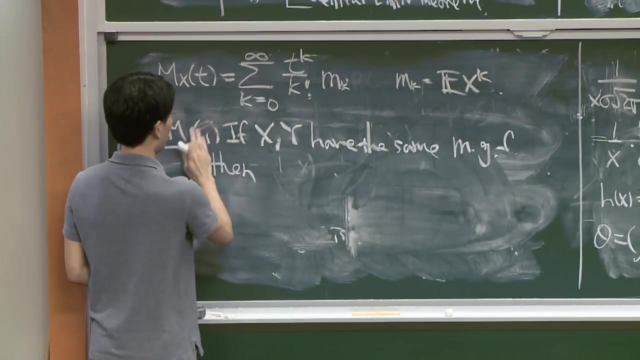 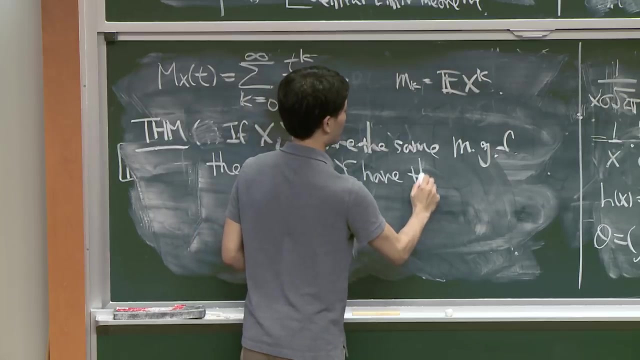 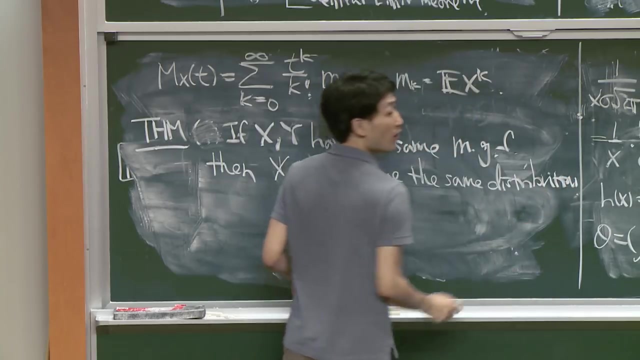 This might not converge. So if moment-generating function exists, they pretty much classify your random variables. So if two random variables, x, y, have the same moment-generating function, then x and y have the same distribution. I will not prove this theorem. 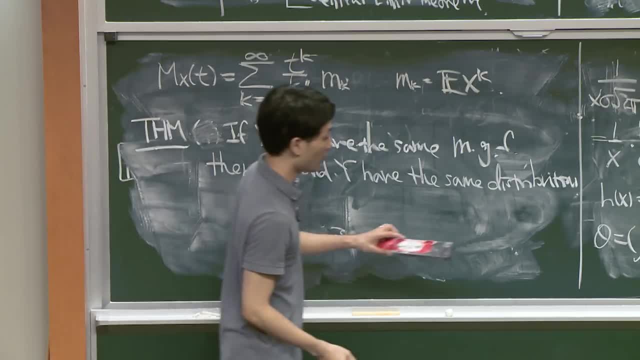 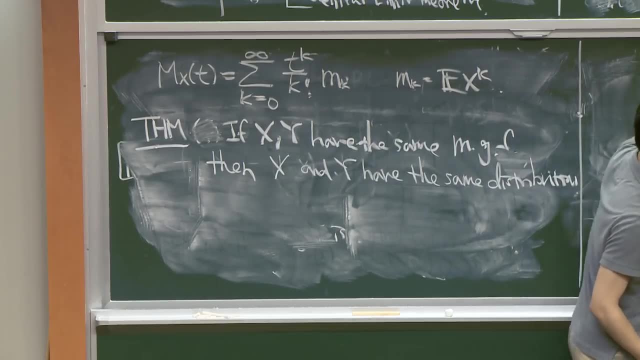 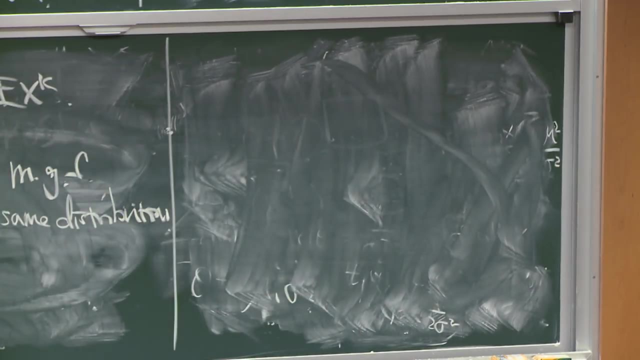 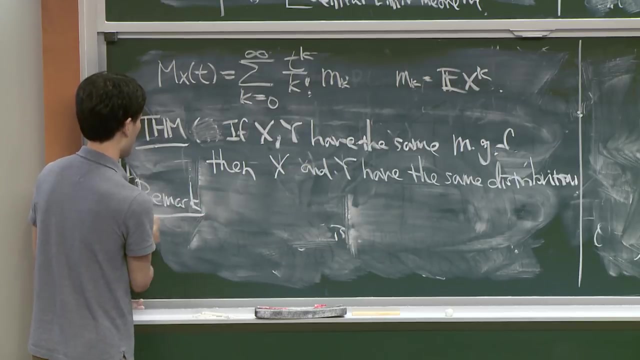 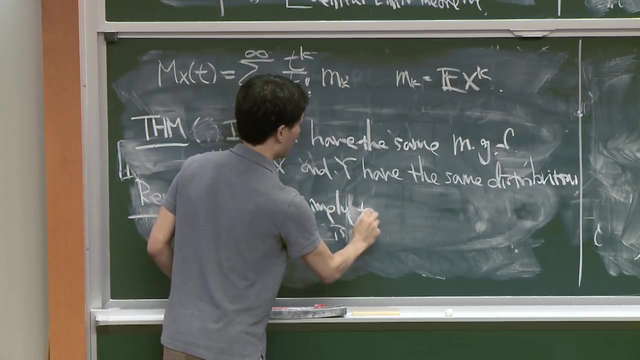 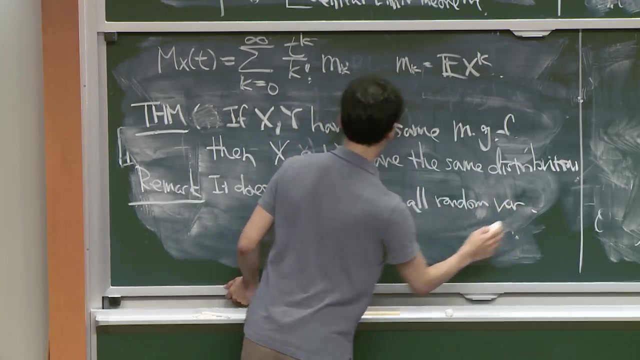 But it says that moment-generating function, if it exists, encodes really all the information about your random variables. You're not losing anything. However, be very careful when applying this theorem because- remark it does not imply that all random variables with 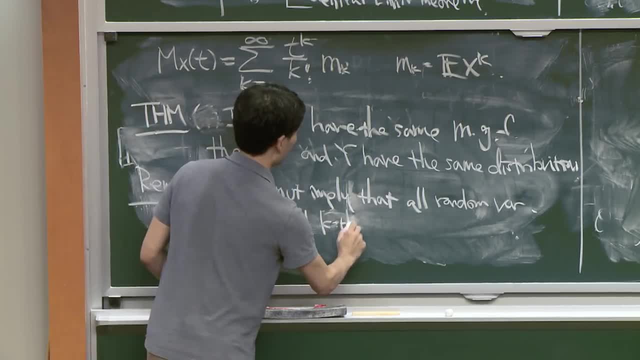 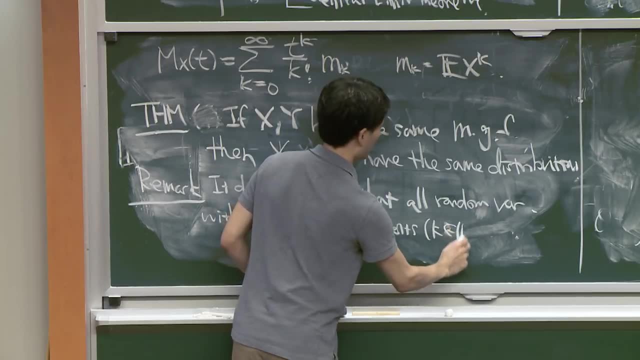 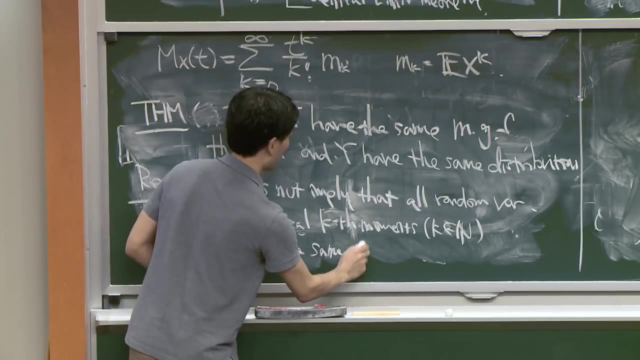 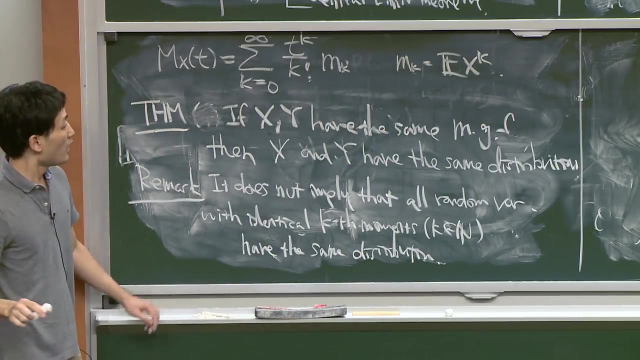 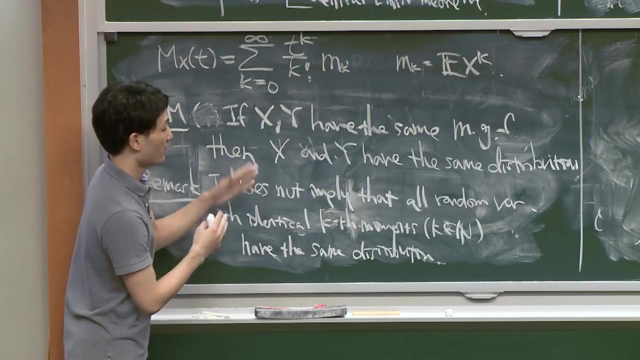 identical k-th moments for all. k has the same distribution. Do you see it? If x and y have a moment-generating function and they're the same, then they have the same distribution. This looks a little bit controversial to this theorem. 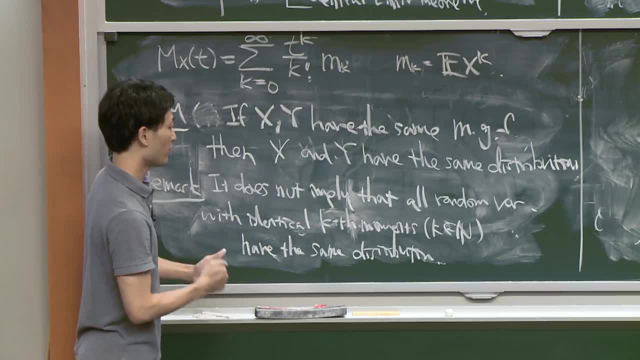 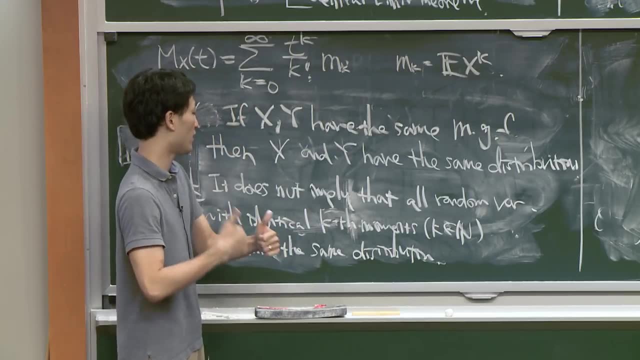 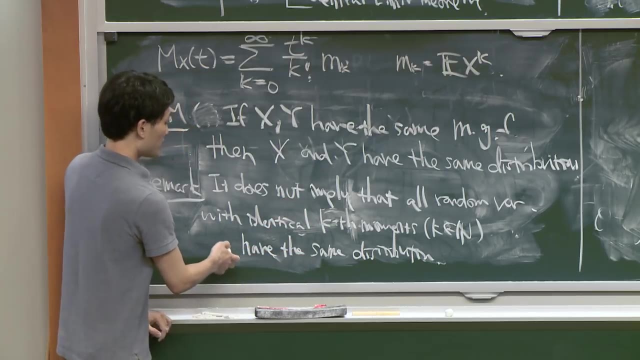 It says that it's not necessarily the case that two random variables which have identical moments, so all case moments are the same for two variables. even if that's the case, they don't necessarily have to have the same distribution, Which seems like it doesn't make sense. 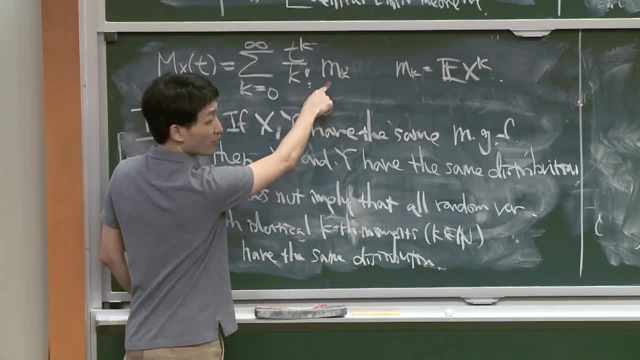 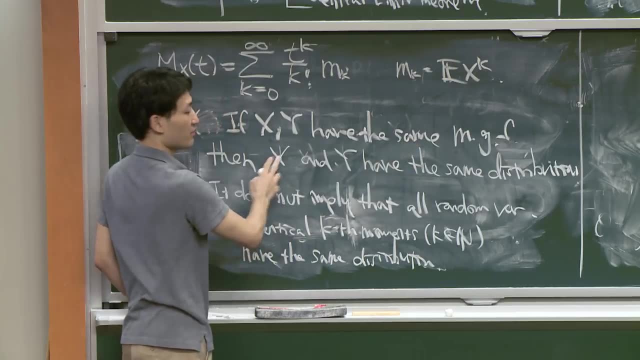 if you look at this theorem, because moment-generating function is defined in terms of the moments. If two random variables have the same moment, they have the same moment-generating function. If they have the same moment-generating function, they have the same distribution. 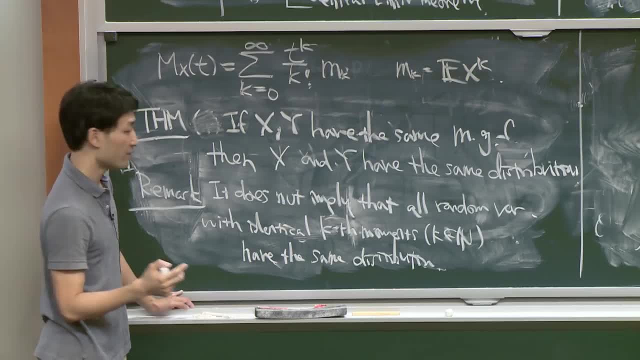 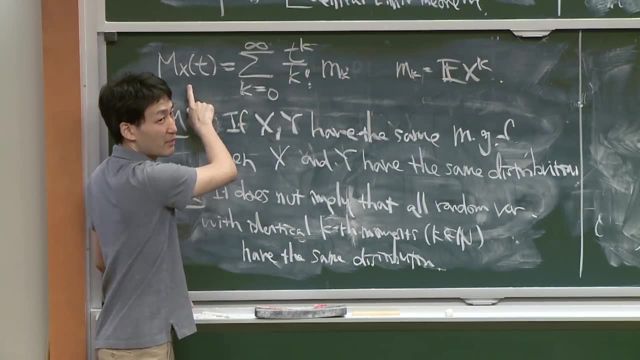 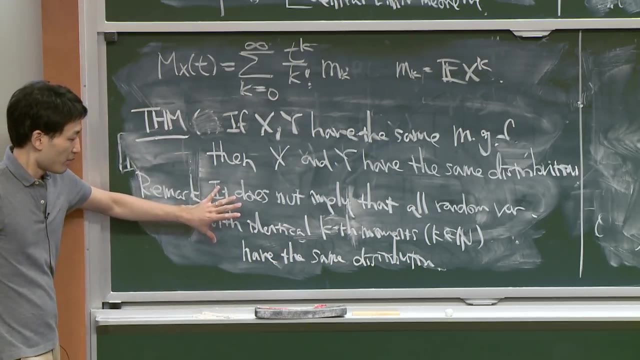 There's a hole in this argument. Even if they have the same moments, it doesn't necessarily imply that they have the same moment-generating function. They might both not have moment-generating functions. That's a glitch, Be careful. So just remember that even if two random variables have the 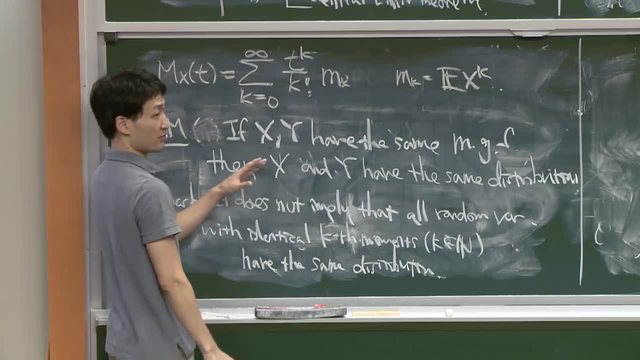 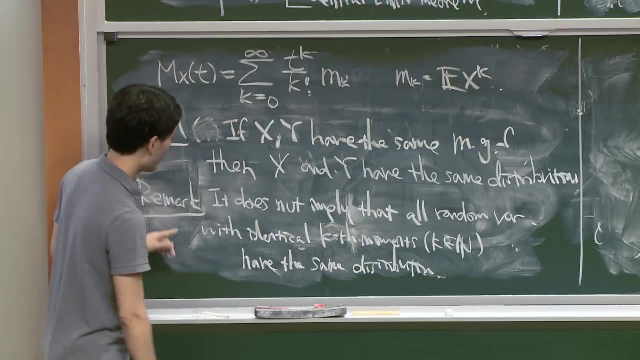 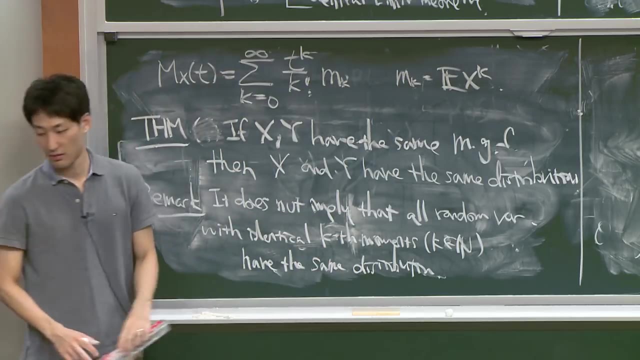 same moment-generating function. they have the same moments. They don't necessarily have the same distribution And the reason is because. one reason is because the moment-generating function might not exist And if you look into Wikipedia, you'll see an example of two random variables where this happens. 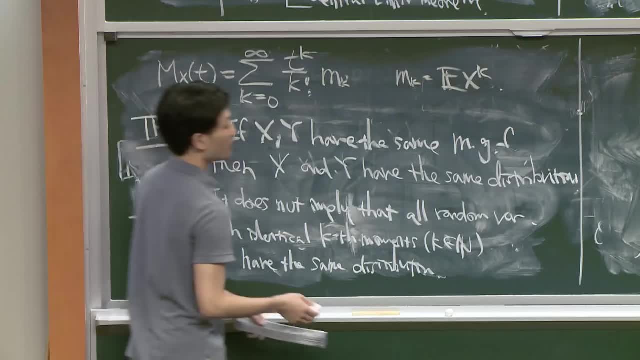 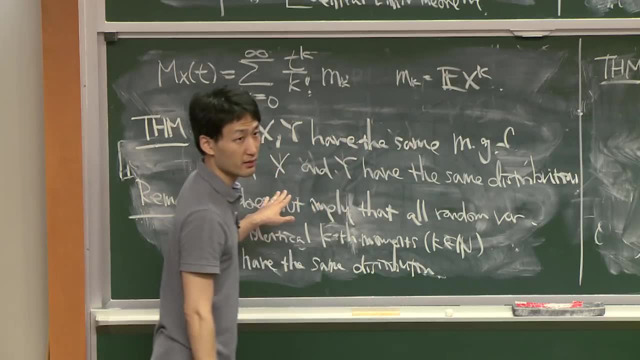 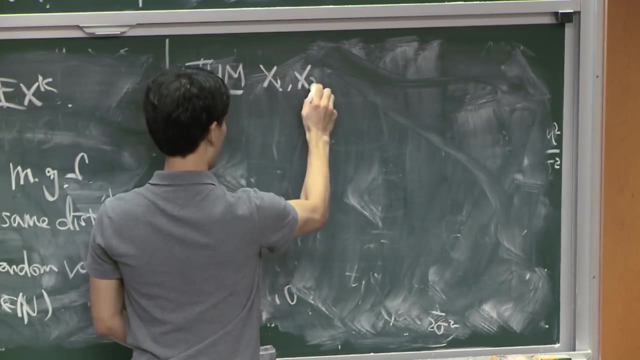 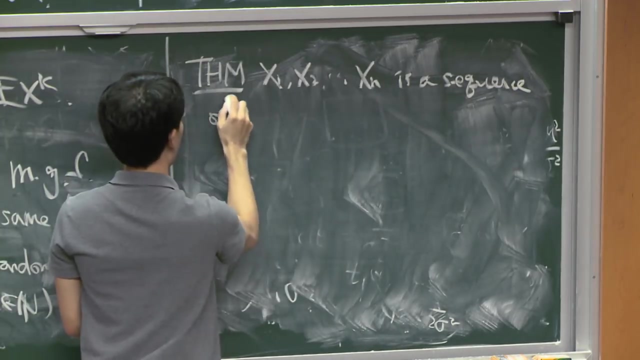 So that's one thing we will use later. Another thing that we will use later, it's a statement really similar to that, but it says something about a sequence of random variables. So if x1,, x2, up to xn is a sequence of random variables, 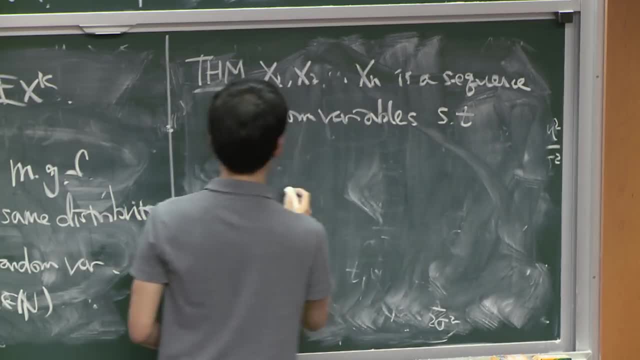 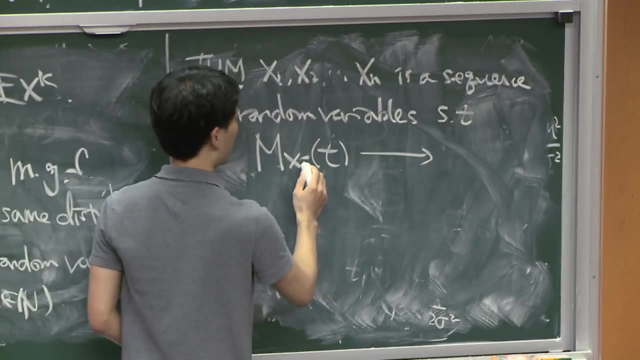 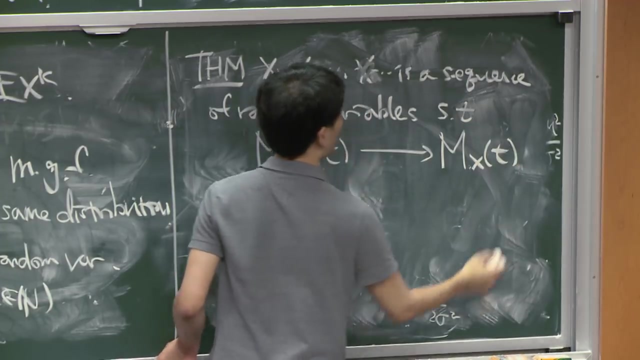 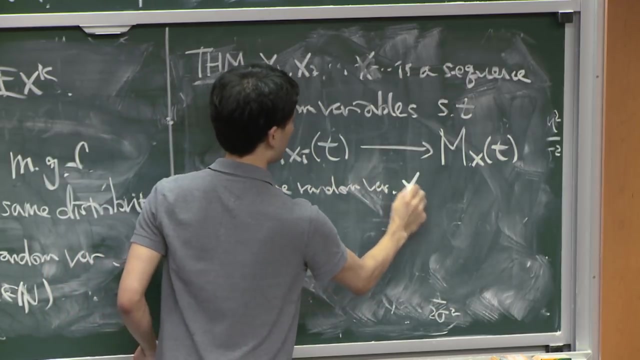 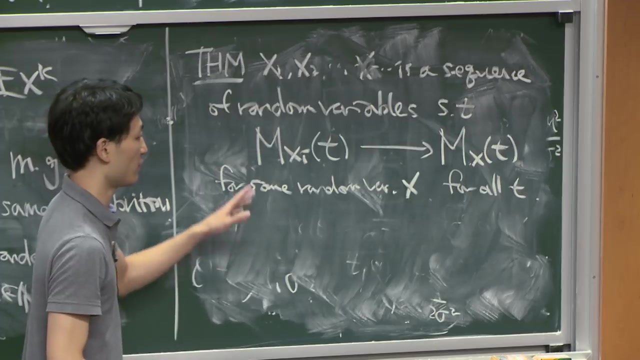 such that the moment-generating function which exists and it converges it goes to infinity. it tends to the moment-generating function of the random variable t, x for some random variable, x for all t. Here we're assuming that all moment-generating functions exist. 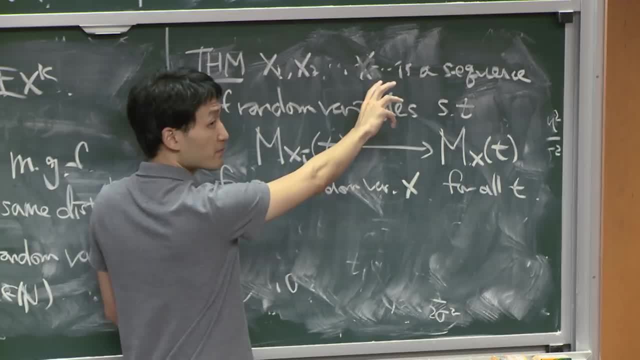 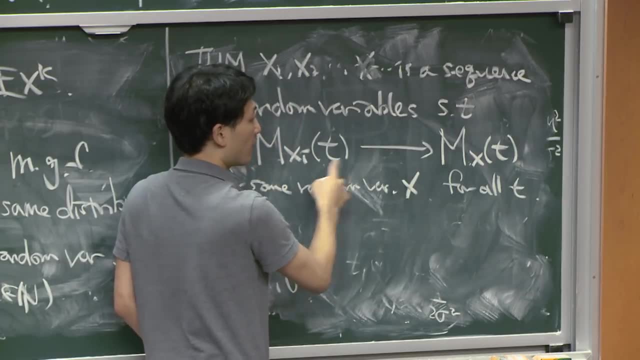 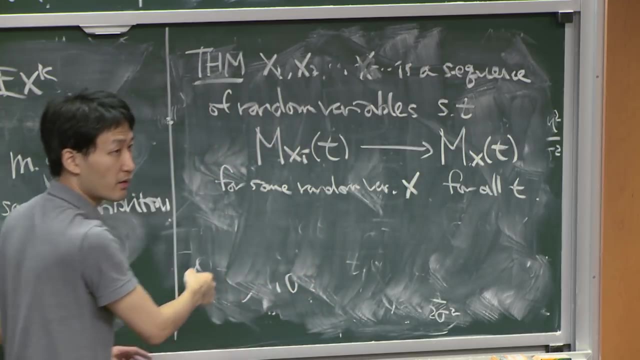 So, again, the situation is: you have a sequence of random variables, Their moment-generating function exists And at each point t it converges to the value of the moment-generating function of some other random variable, x. And what should happen in light of this theorem? 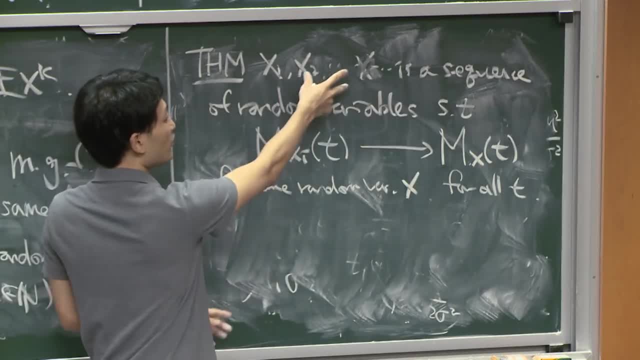 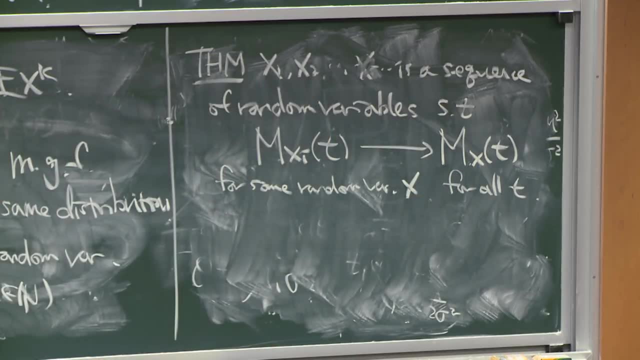 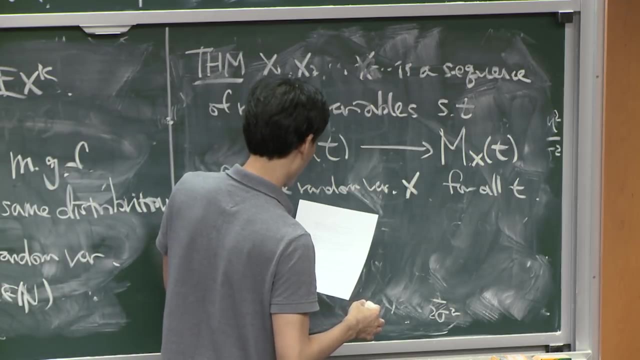 it should be the case that this sequence, the distribution of this sequence, gets closer and closer to the distribution of this random variable x. And to make it formal, to make that intuition formal, what we can conclude is: for all x. 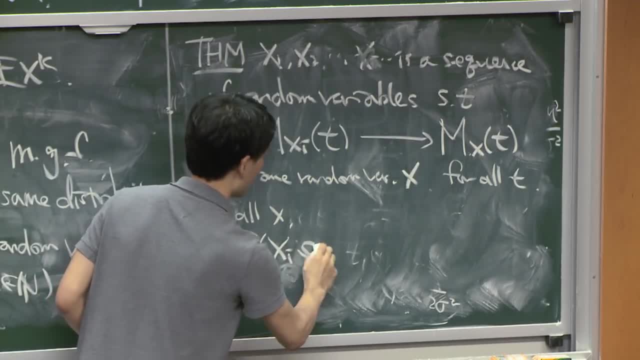 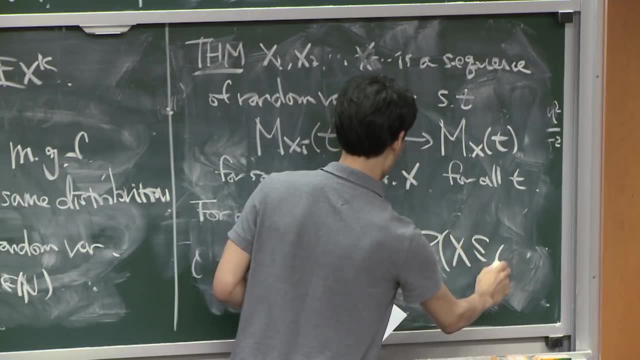 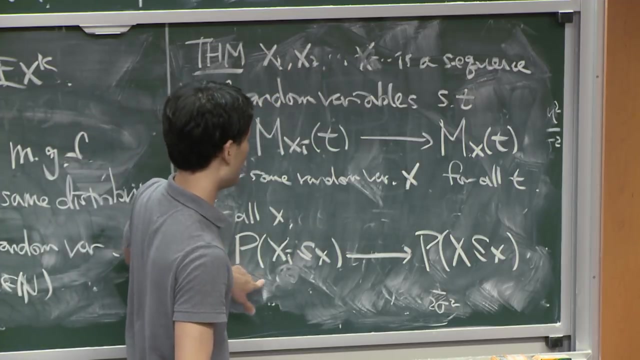 the probability xi is less than or equal to x tends to the probability. The probability at x. So in this sense the distributions of these random variables converges to the distribution of that random variable. So it's just a technical issue. 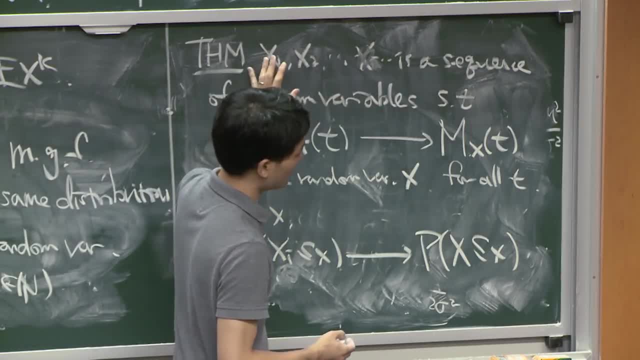 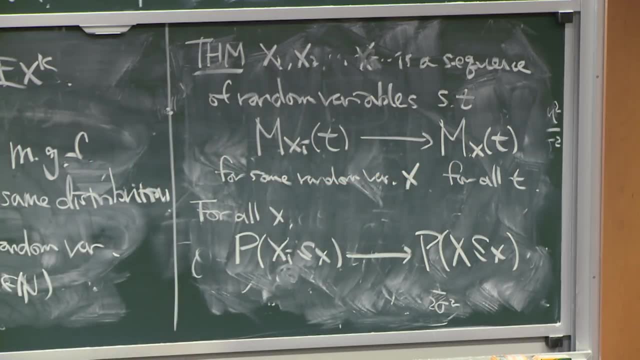 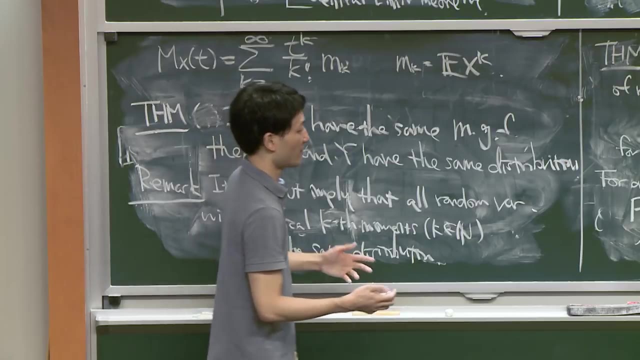 You can just think of it as these functions kind of converge to the, these random variables converge to that random variable. If you take some graduate probability course, you'll see that there's several concepts, several possible ways to define convergence. But that's just some technicality. 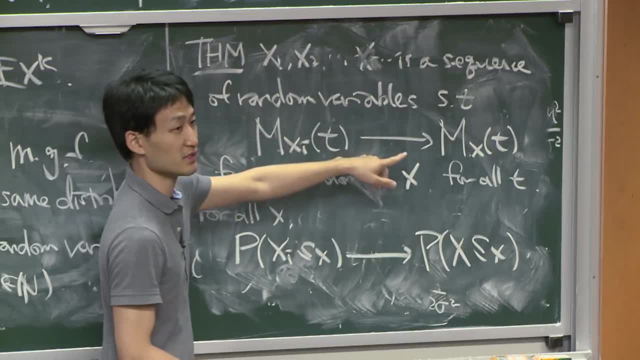 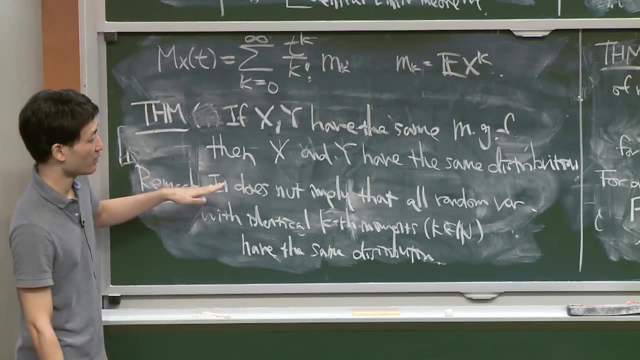 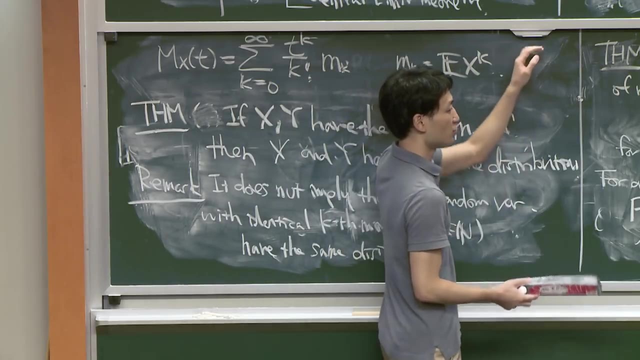 And the spirit here is just really the sequence: converges if its moment-generating function converges. So, as you can see from these two theorems, moment-generating function, if it exists, is a really powerful tool. where you can, it allows you to control the distribution. 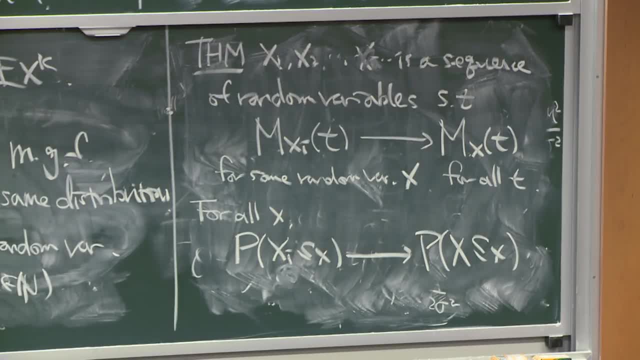 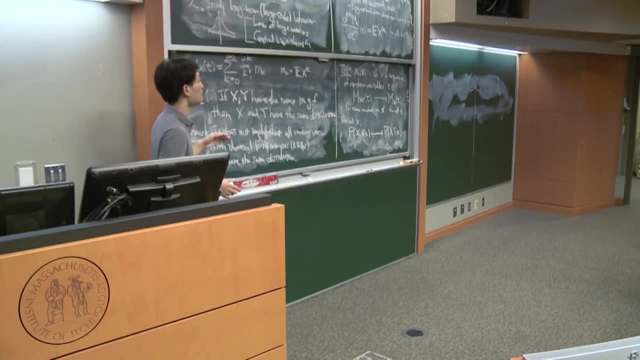 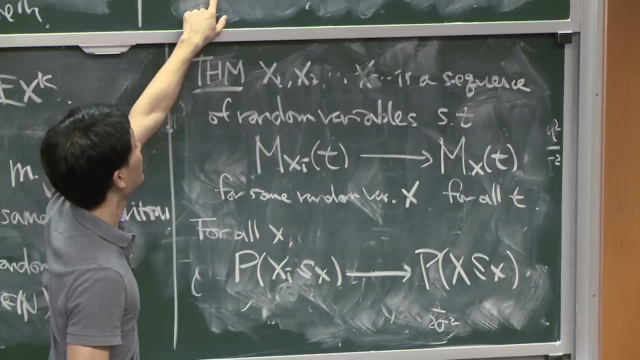 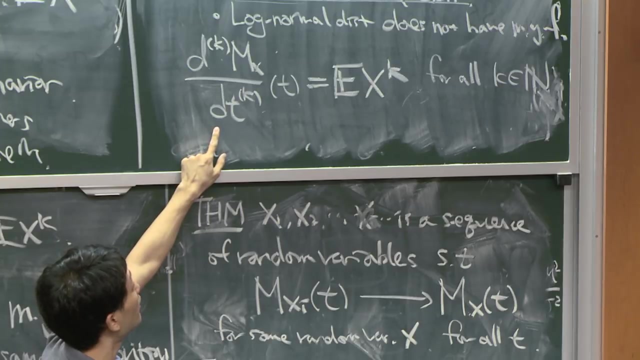 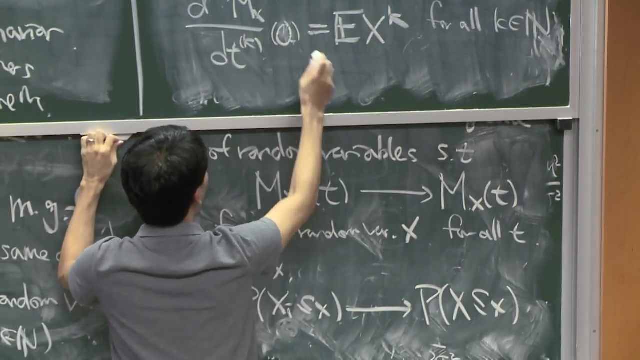 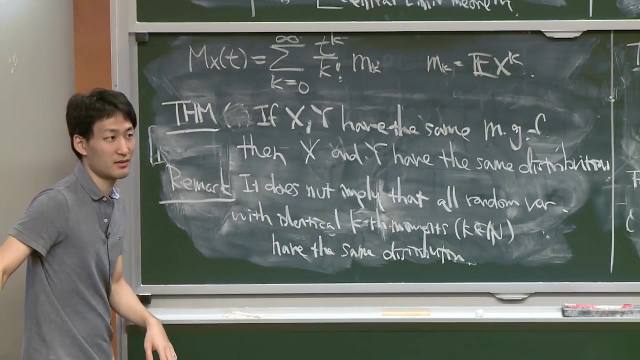 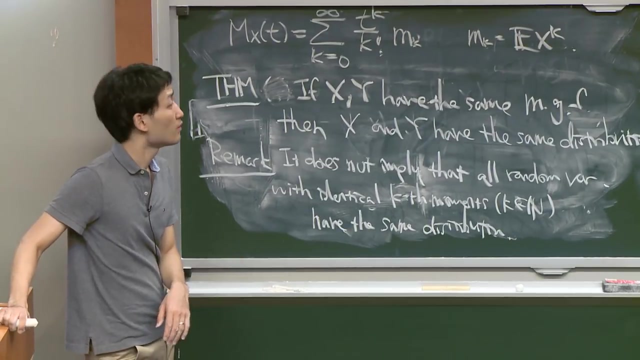 So you'll see some applications later in central limit theory. Any questions? This one, Why The right-hand side does not depend on Ah Zero, Thank you. They evaluated at zero. Other questions, Other questions: When you say the moment-generating function? 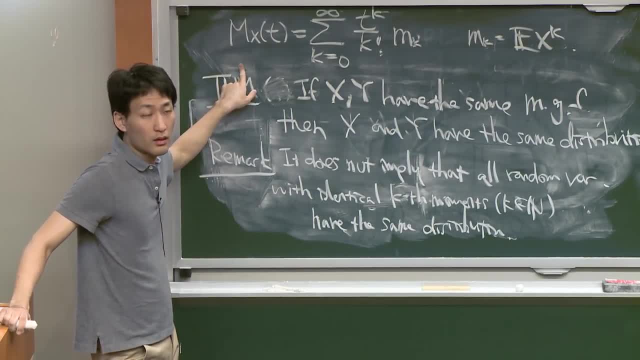 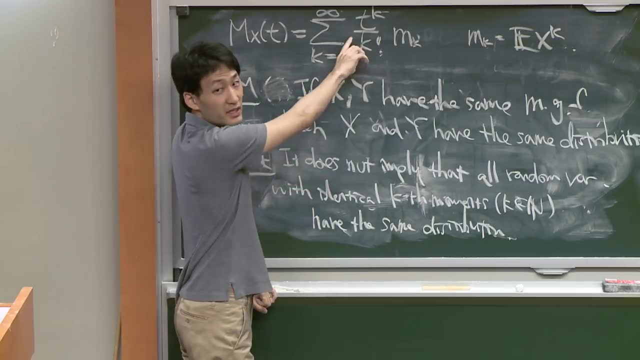 doesn't exist? do you mean that it isn't analytic or just doesn't converge anywhere? It might not converge anywhere. So log-normal distribution: it does not converge. So for all non-zero t it does not converge. It does not converge for log-normal distribution. 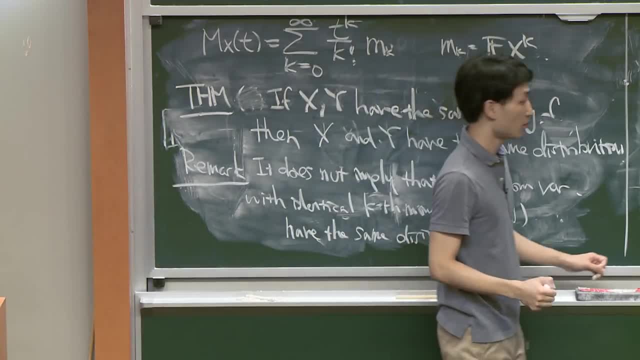 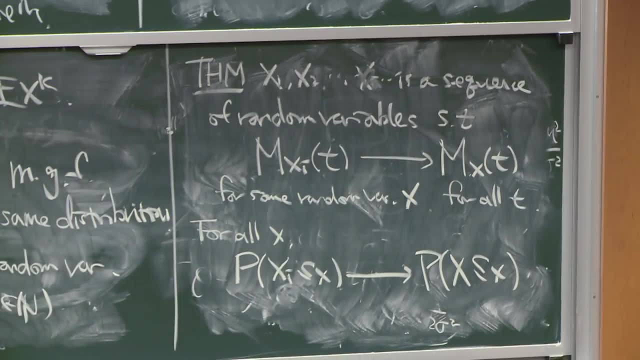 Here: Yes, Point-wise convergence implies point-wise convergence. No, no, no. So because, yeah, because it's point-wise, this conclusion is also rather weak. It's kind of it's almost the weakest convergence in distribution. 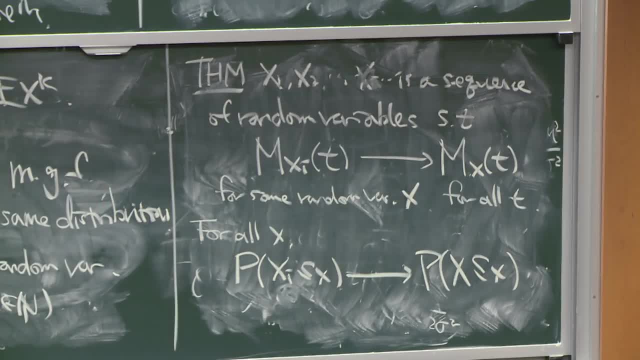 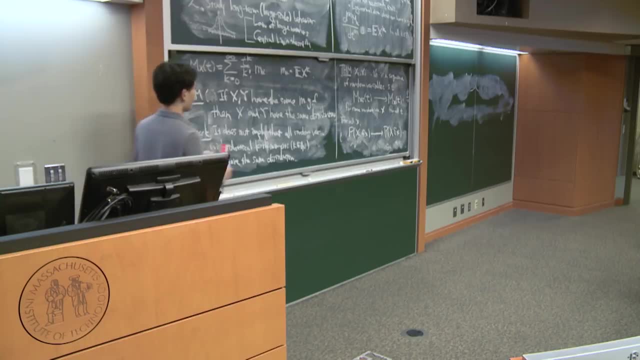 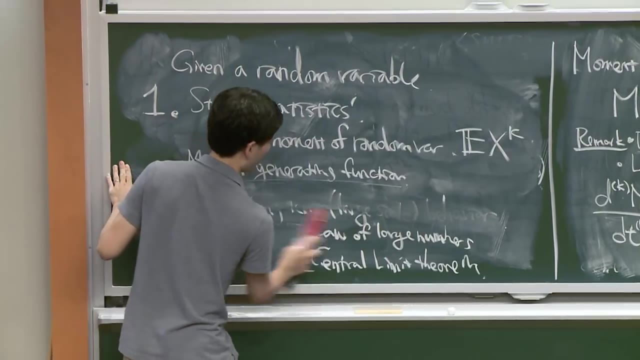 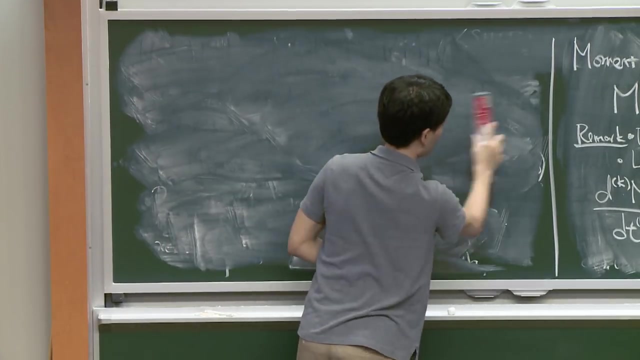 Ah, OK, there we are. so what you can reacts. all of this is very much Schulder-like. OK, draw the other, It's a little a little jar. you get two, OKalnız. 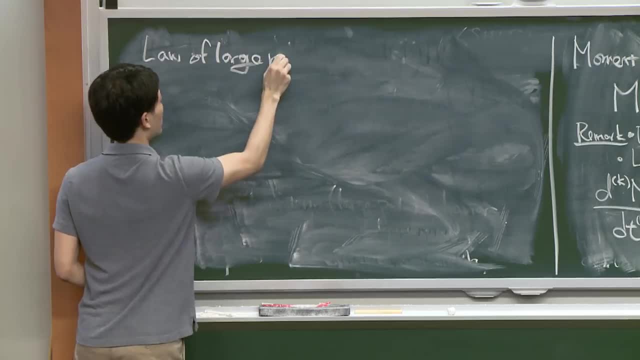 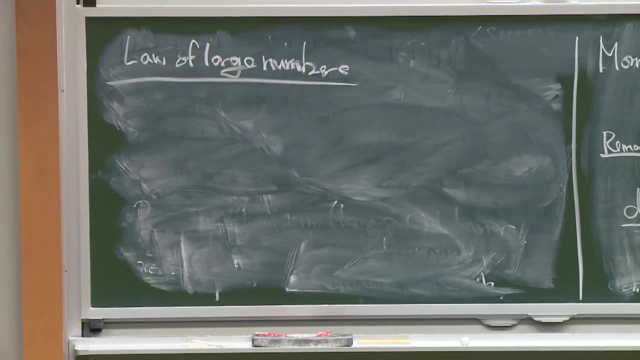 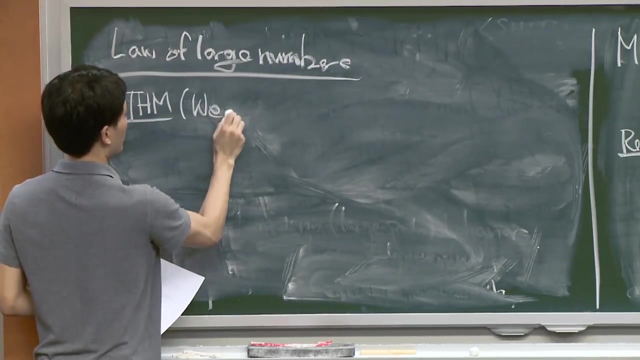 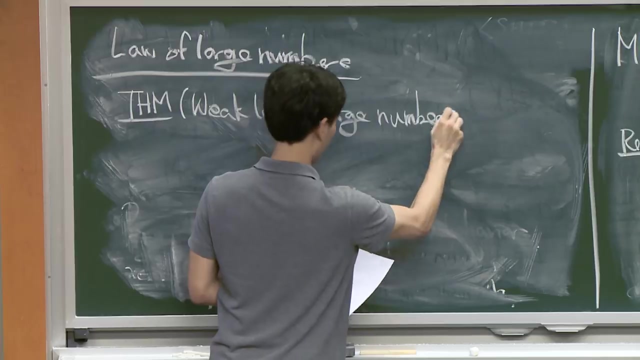 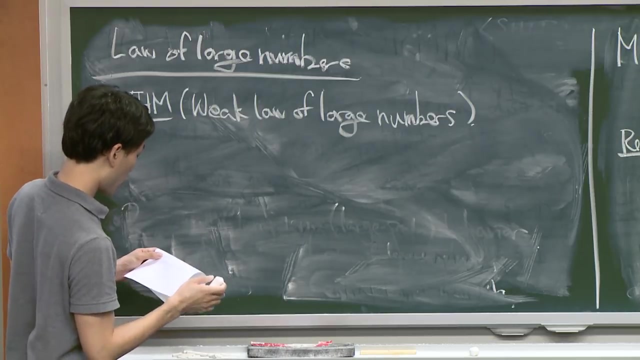 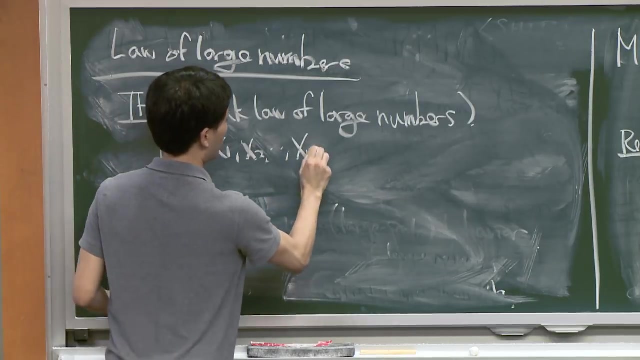 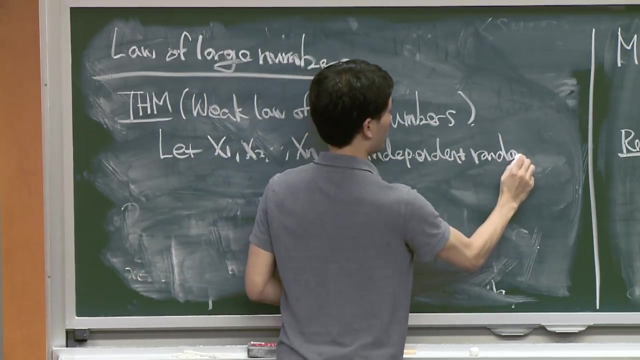 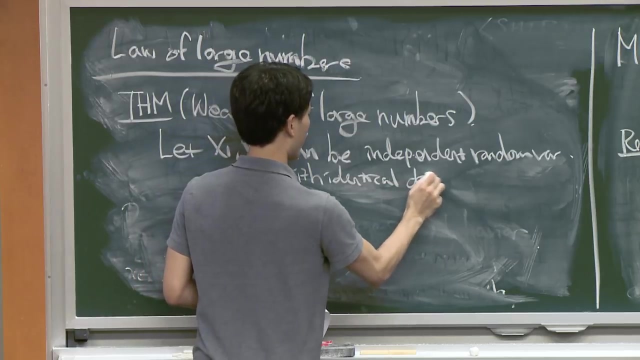 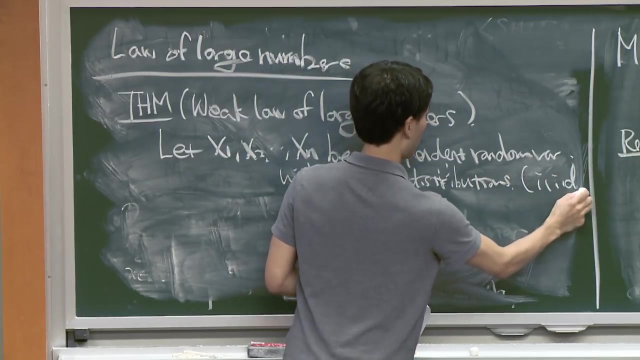 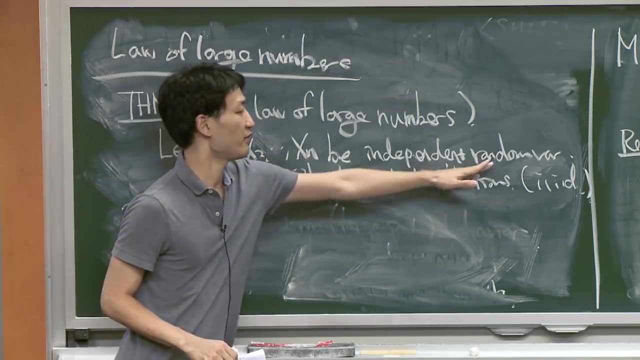 So this, of course you have probably understood There's. So now we're talking about large-scale behavior. Let x1 up to xn be independent random variables with identical distribution. We don't really know what the distribution is, but we know that they're all the same. 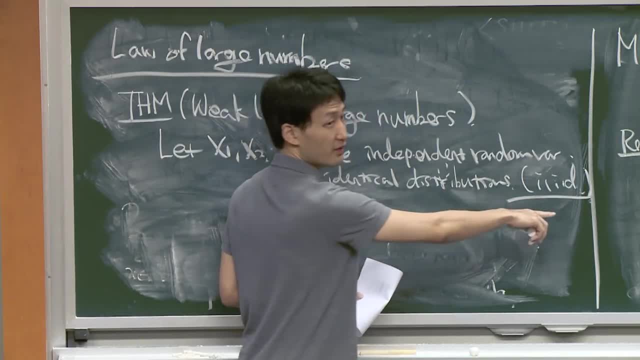 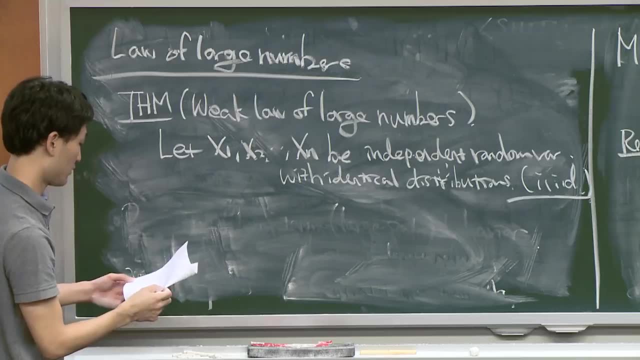 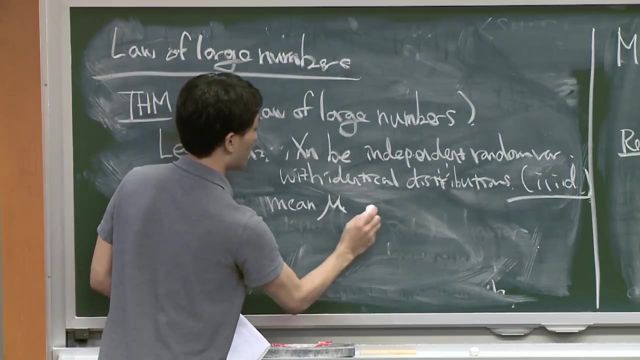 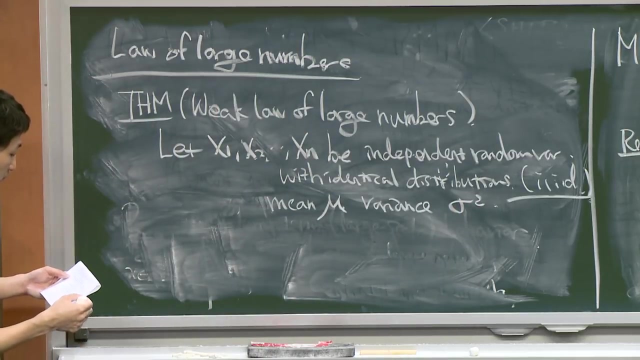 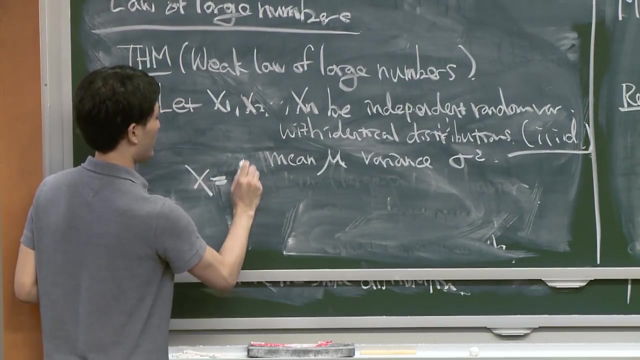 In short, I'll just refer to this condition as iid random variables, later Independent, identically distributed random variables, And let mean be mu variance, be sigma squared. OK, Let also define x as the average of n random variables. 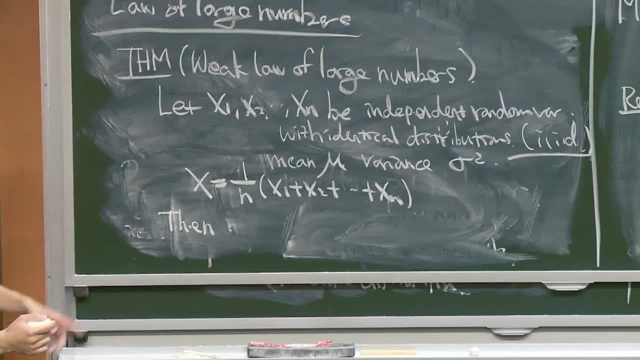 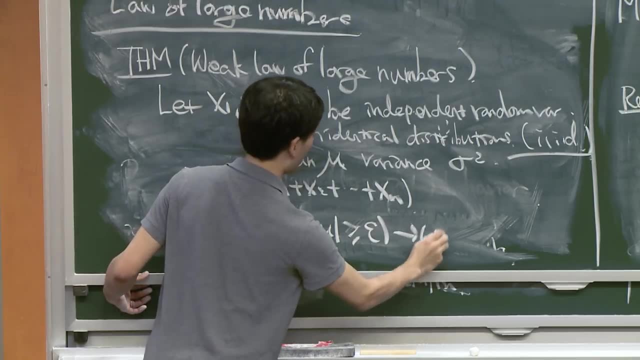 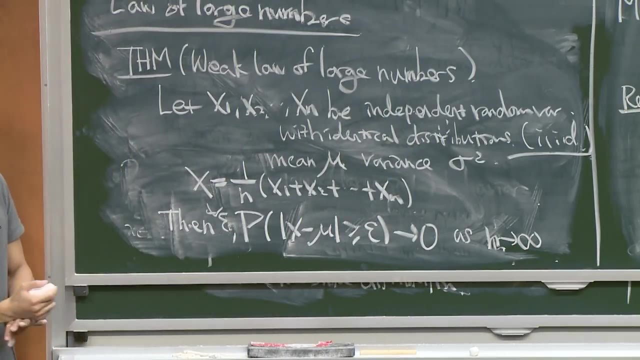 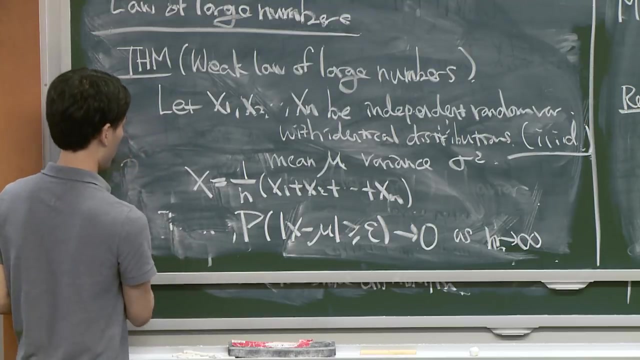 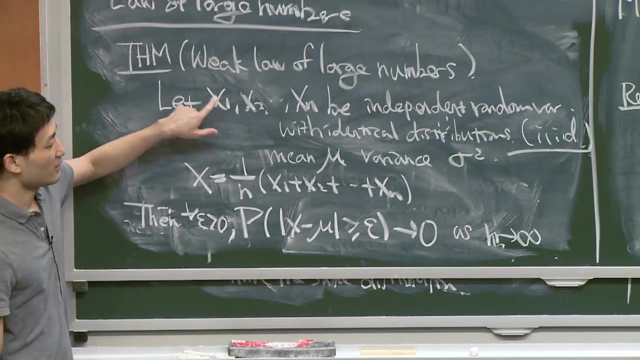 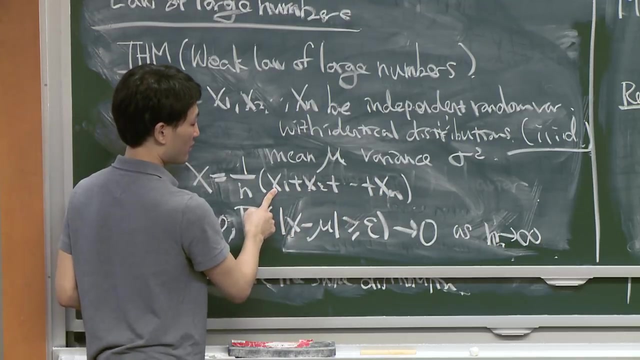 Then the probability that x is a positive epsilon, All positive epsilon. So whenever you have identical independent distributions, when you take their average, When you, if you take large enough number of samples, they will be very close to the mean, which makes sense. 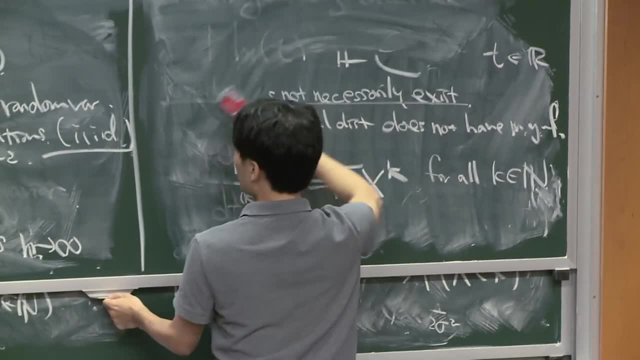 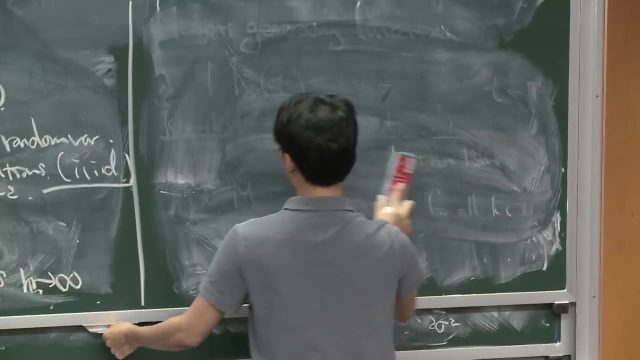 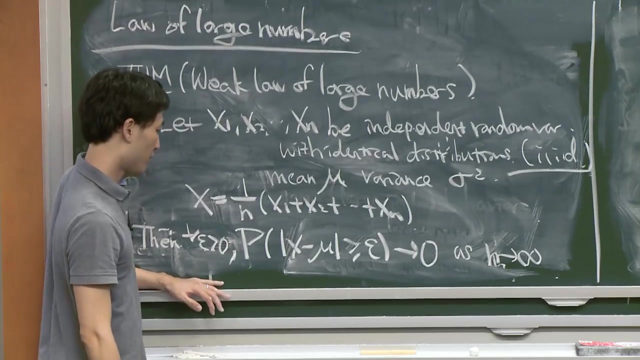 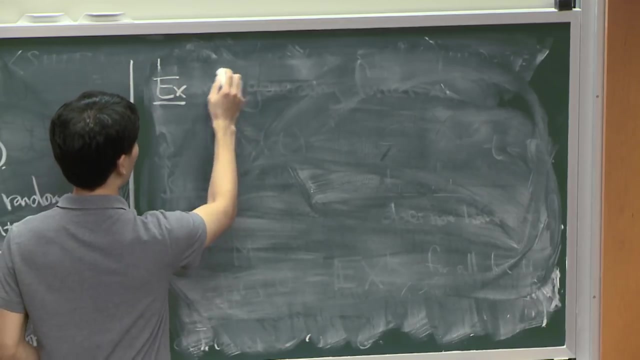 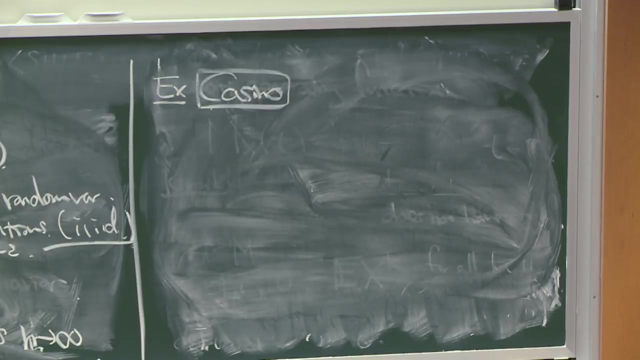 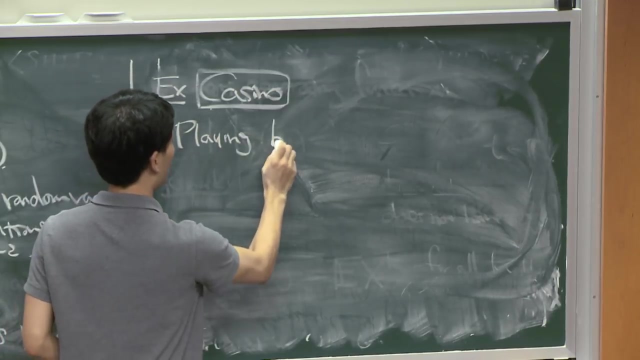 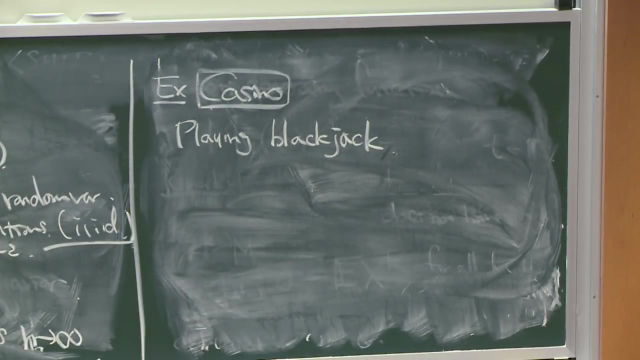 So what's an example of this, Before proving it? an example of this theorem in practice can be seen in the casino. So, for example, if you're playing blackjack in a casino, I'm playing blackjack When you're playing against a casino. 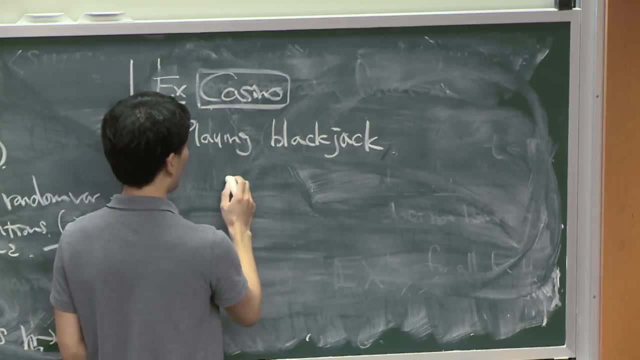 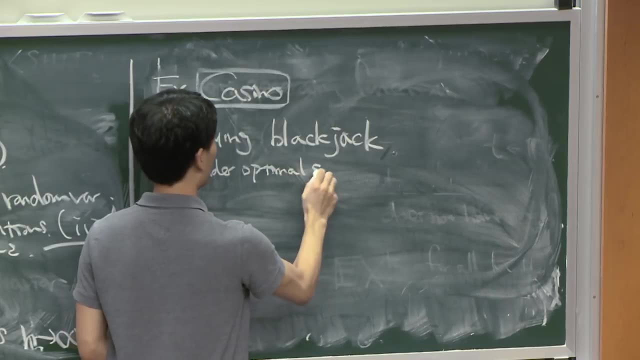 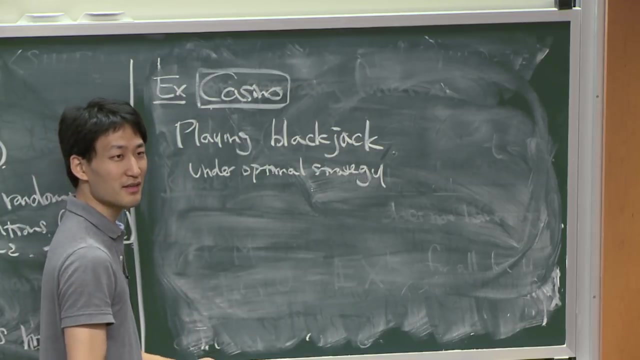 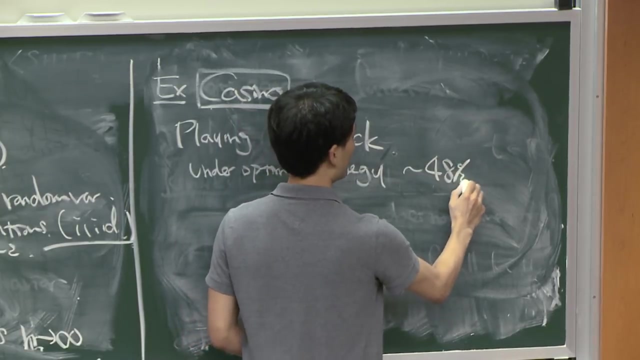 you have a very small disadvantage, So you're winning If you're playing the optimal strategy you have. does anybody know the probability? I think it's about 48, 49%, about like 48% chance of winning. 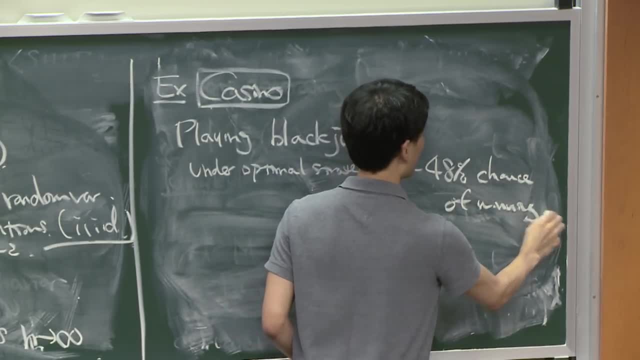 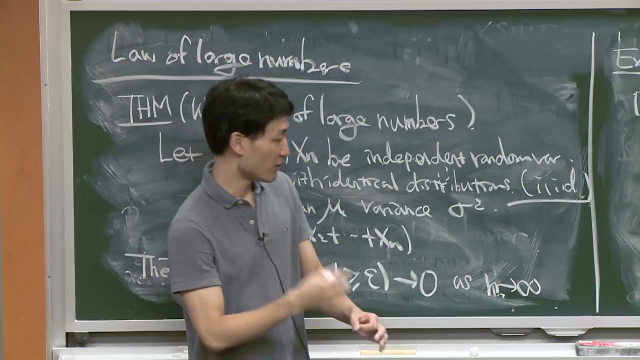 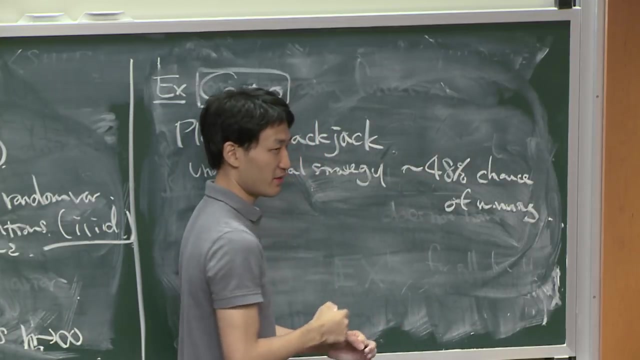 That means that if you beat $1 at the beginning of each round, you are expected the expected amount you will win about win is $0.48,. the expected amount that the casino will win is $0.52, OK. 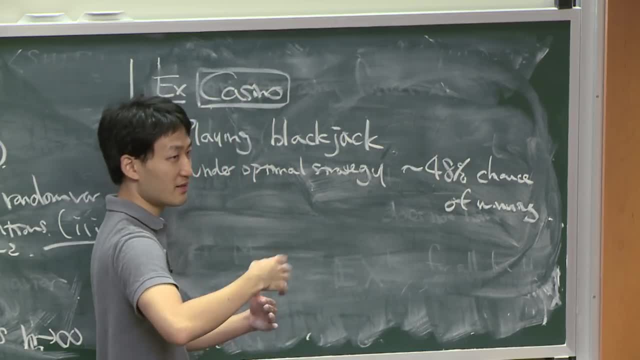 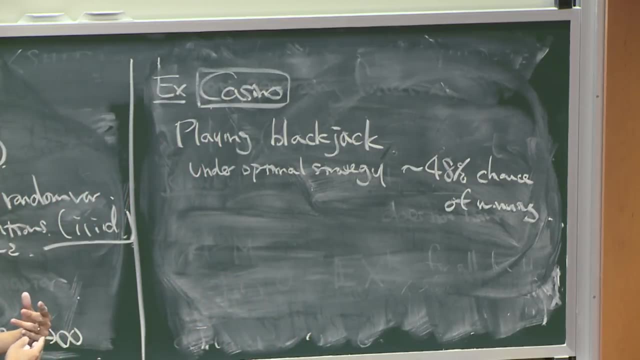 But it's designed so. the variance is so big that this expectation is hidden. the mean is hidden. From the player's point of view, you only have a very small sample, so it looks like the mean doesn't matter because the variance takes over. 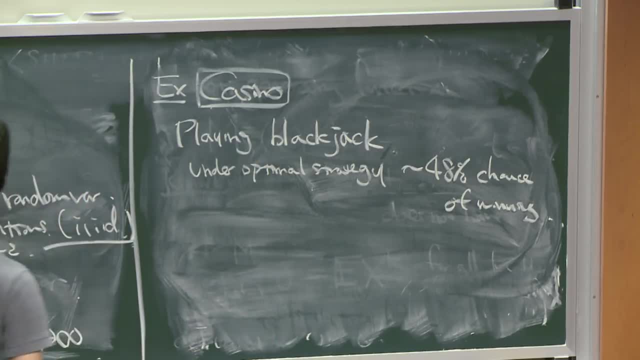 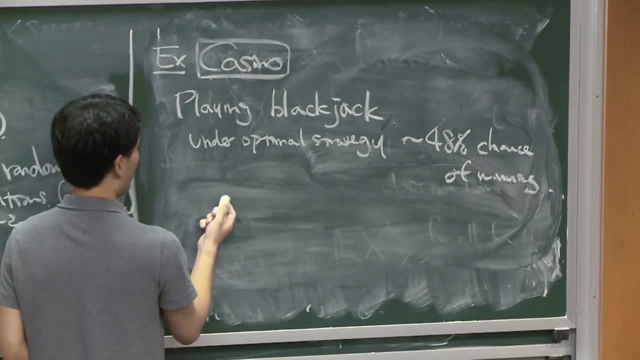 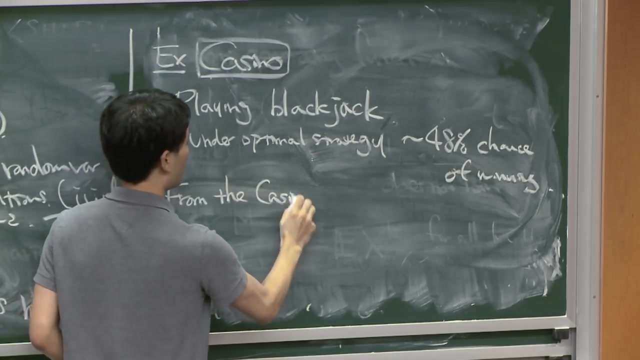 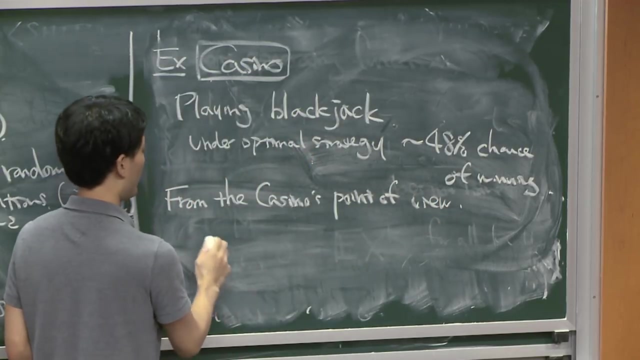 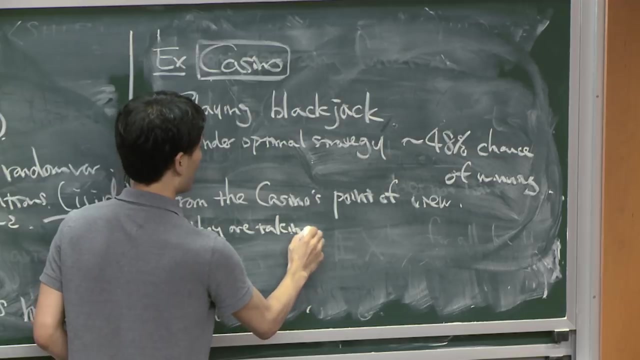 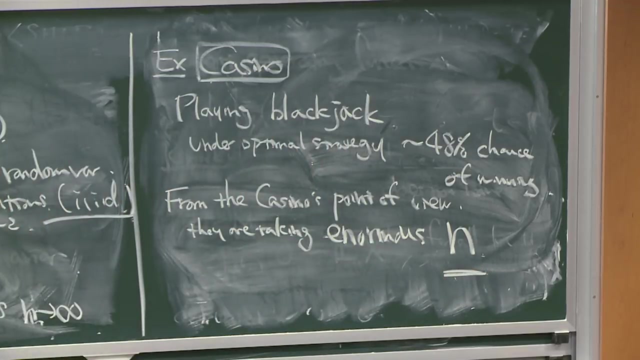 in a very short scale, But from the casino's point of view they're taking a very large n there. So for each round, let's say, from the casino's point of view it's like taking enormous value of n? n here. 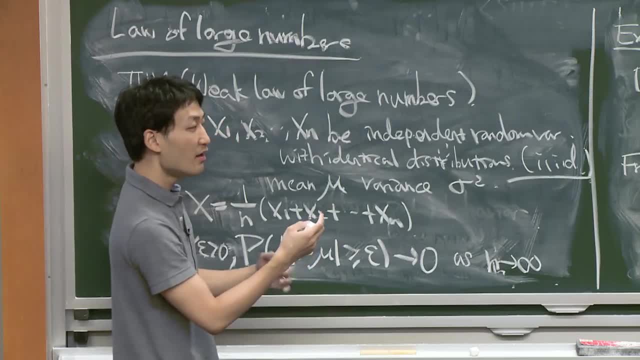 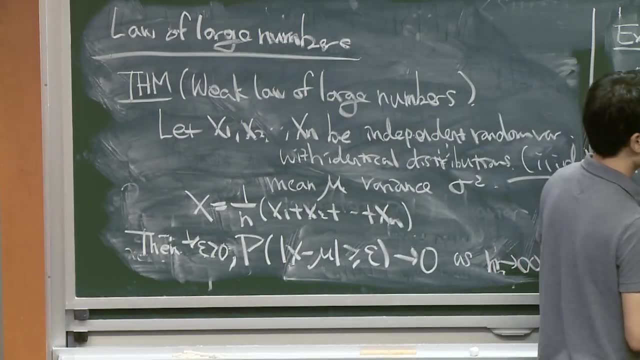 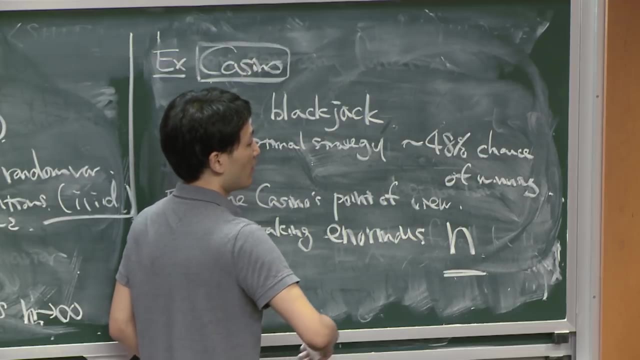 And that means as long as they have a slightest advantage, they'll be winning, They'll be making money, and a huge amount of money, And most games played in the casinos are designed like this. It looks like the mean is really close to 50%. 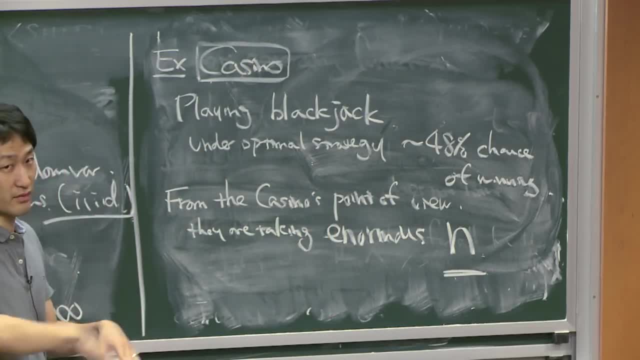 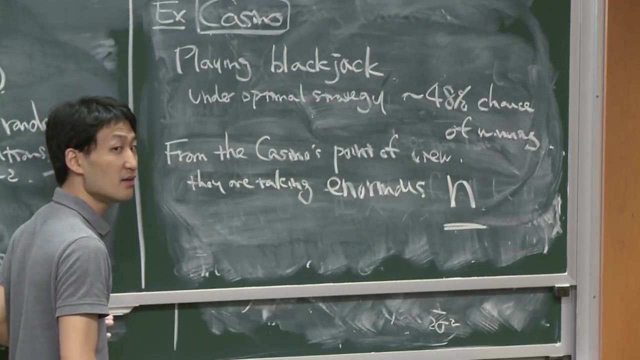 but it's hidden because they designed it. so the variance is big. A variance is big, But from the casino's point of view, they have enough players to play the game, so that the law of large numbers just makes them money. So the casino was: yeah, the moral is: don't play blackjack. 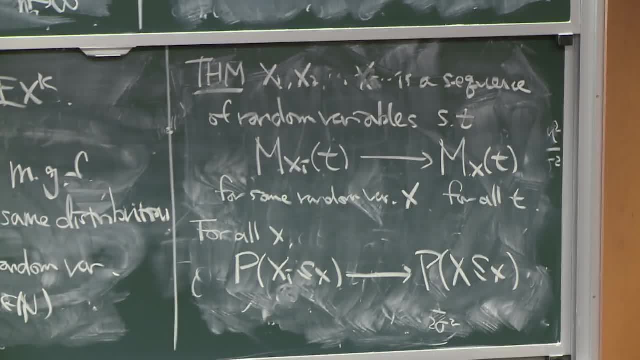 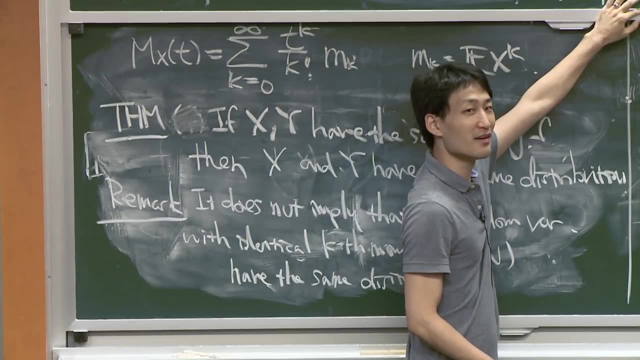 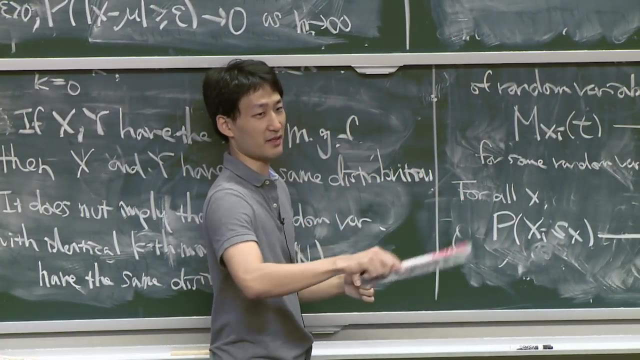 Play poker. The reason that poker doesn't the rule of law of large numbers doesn't apply, at least in this sense, to poker. can anybody explain why It's? because, poker, you're playing against other players. OK, If you have a disadvantage, you're playing against other players. 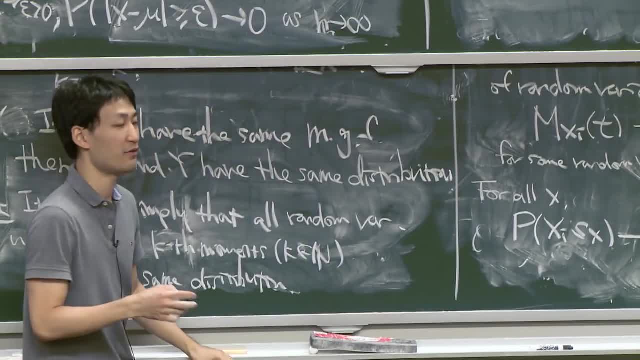 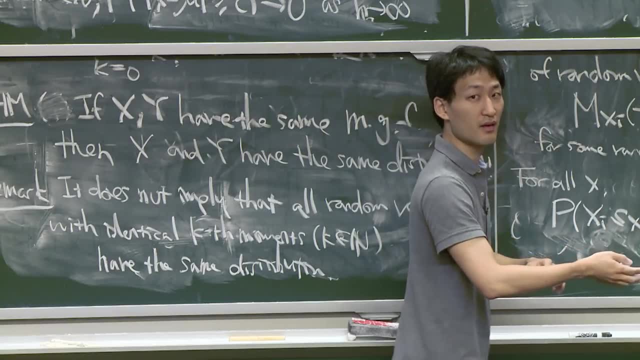 OK, If you have an advantage, if your skill, if you believe that there's skill in poker, if your skill is better than the other player by, let's say, 5% chance, then you have an edge over that player. 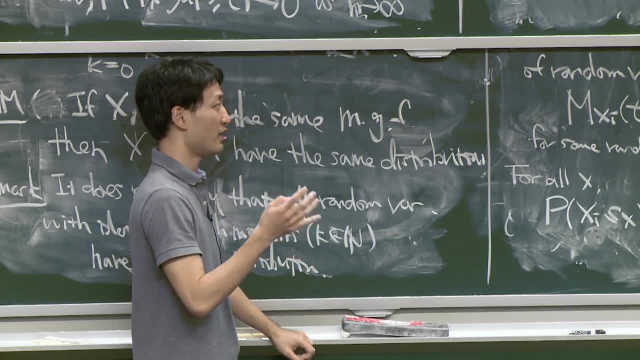 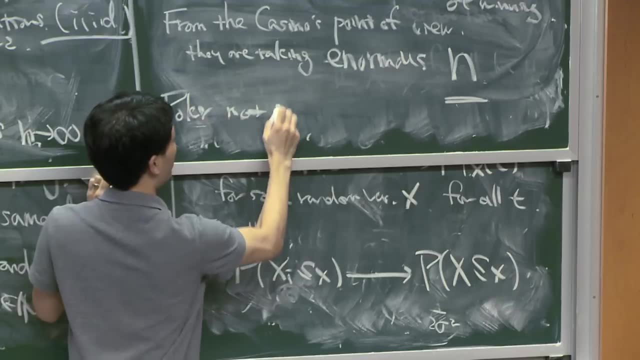 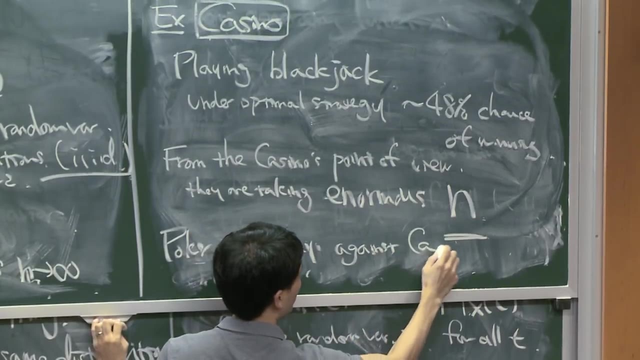 So you can win money. The only problem is that casino, because they're not playing against the poker. you're not playing against the casino, Not play, don't play against the casino. But they still have to make money. So what they do instead is they take rake. 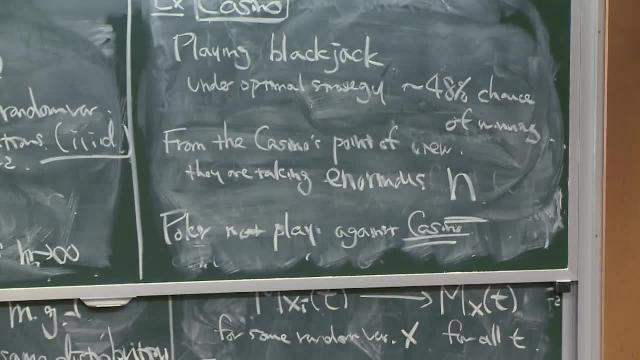 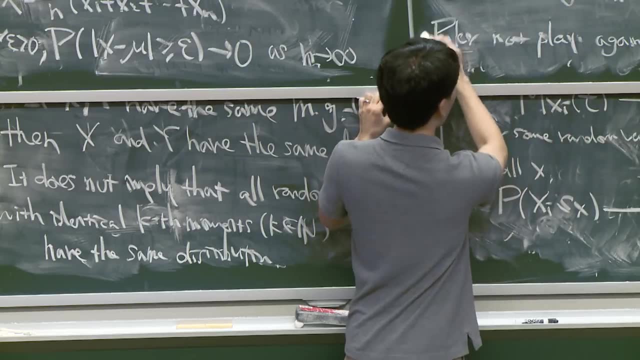 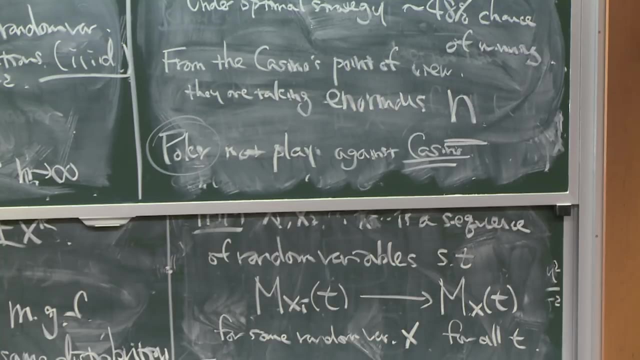 So for each round that the players play they pay some fee to the casino, And how the casino makes money in the poker table is by accumulating those fees. They're not taking chances there, But from the player's point of view, if you're better than the other player and the amount of edge 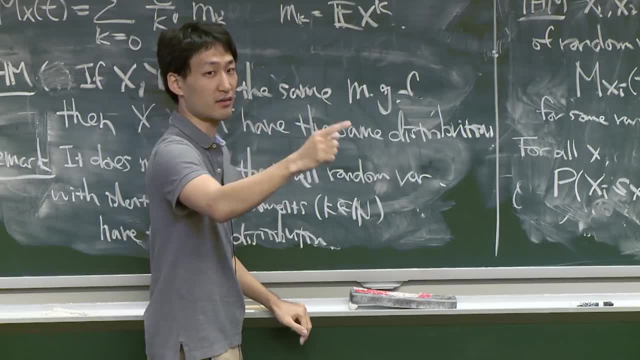 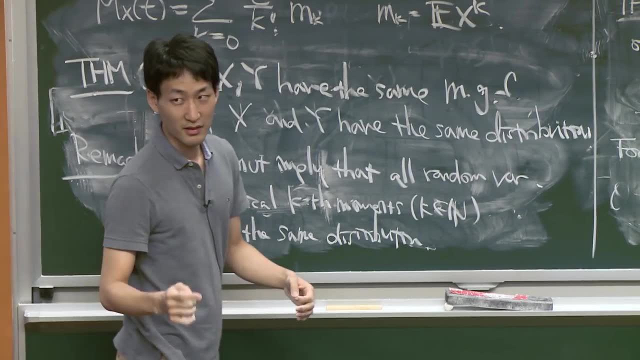 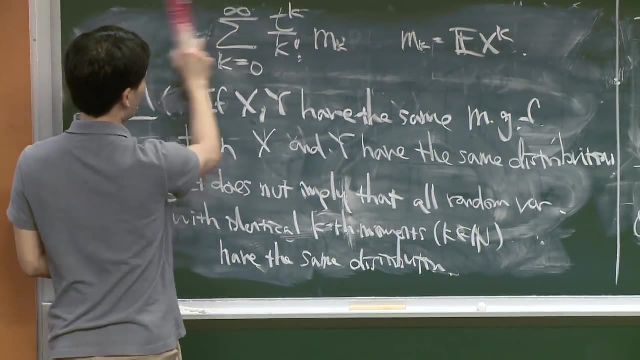 you have over the other player is larger than the fee that the casino charged to you, then now you can apply law of large numbers to yourself and win. And if you take an example as poker, it looks like, OK, I'm not going to play poker. 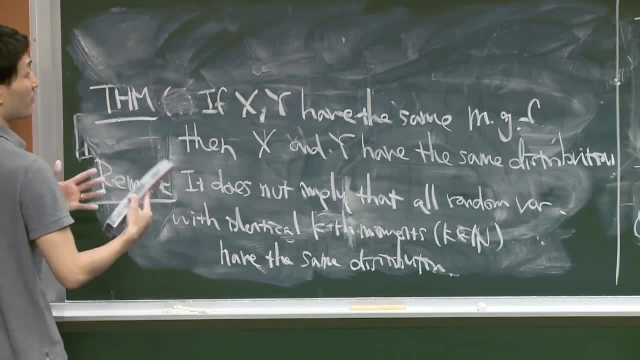 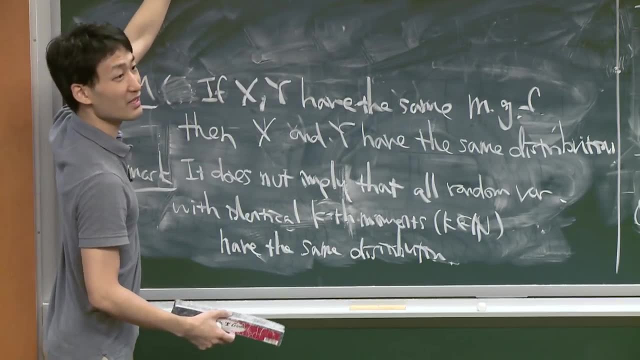 If it's like a hedge fund or put for like I don't know if you're doing high frequency trading. that's the moral behind it. So that's the belief you should have. You have to believe that you have an edge. 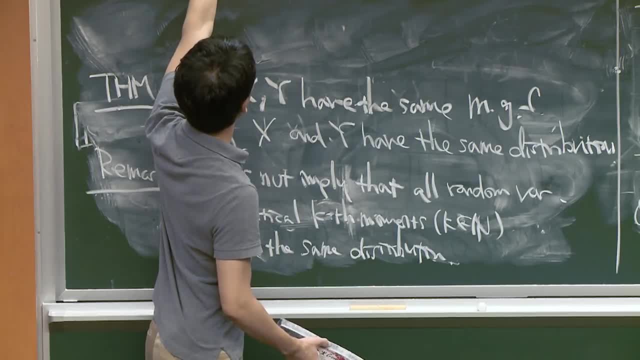 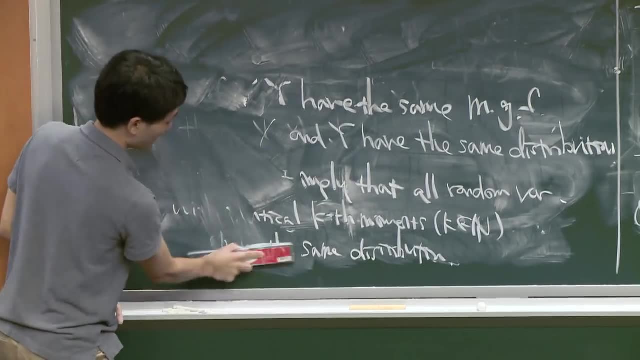 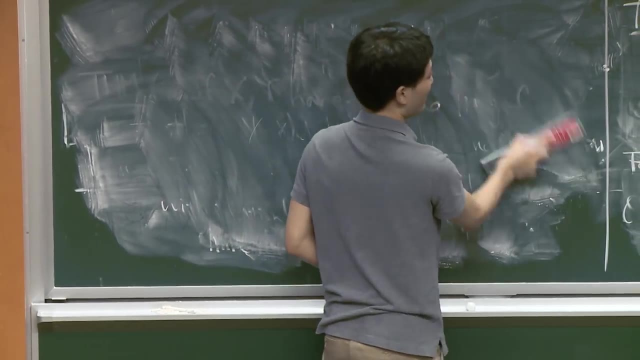 Even if you have a tiny edge, if you can have enough number of trials, if you can trade enough of time using that strategy, using some strategy that you believe is winning over time, then law of large number will take it from there and will bring you money profit. 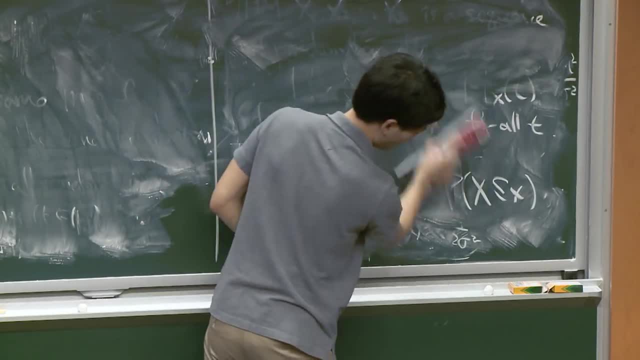 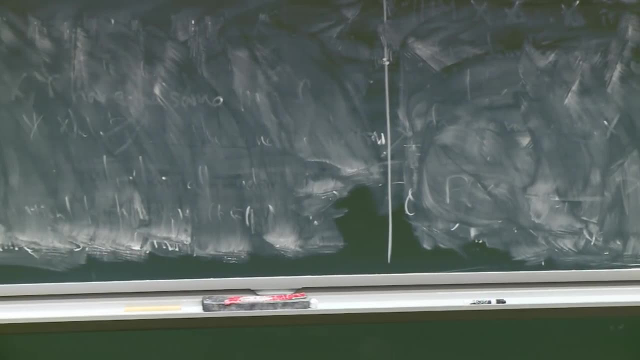 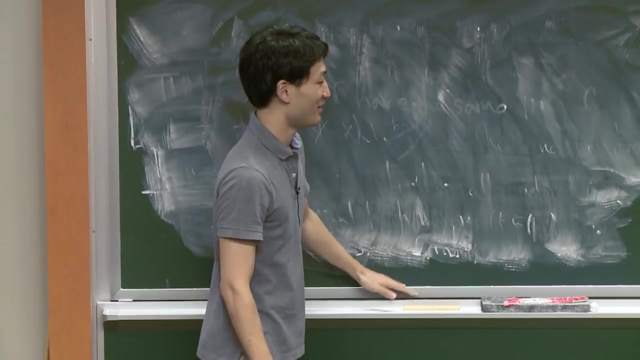 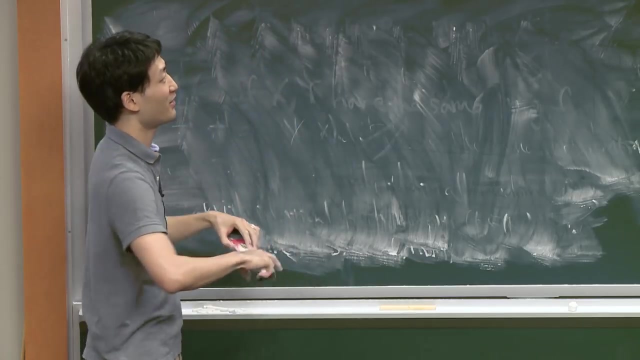 Of course, the problem is when the variance is big, your belief starts to fall. At least, that was the case for me when I was playing poker, Because I believe that I have an edge, but when there is really swing, it looks like your expectation is negative. 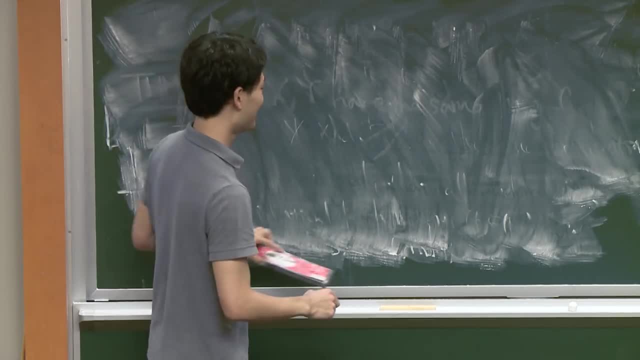 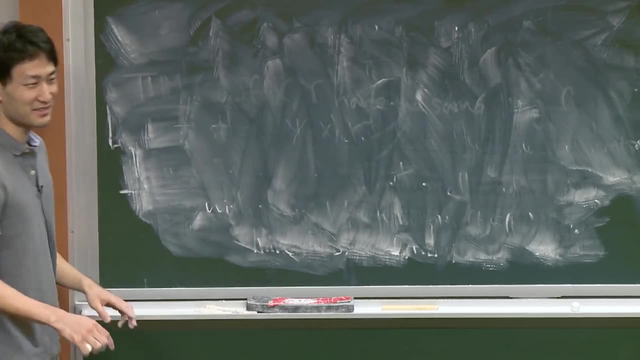 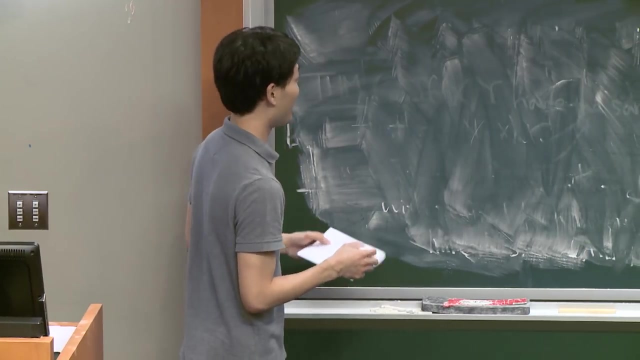 And that's when you have to believe in yourself. Yeah, That's when your faith in mathematics is being challenged. Yeah, It really happens. I hope it doesn't happen to you. Anyway, that's proof of law of large numbers. How do you prove it? 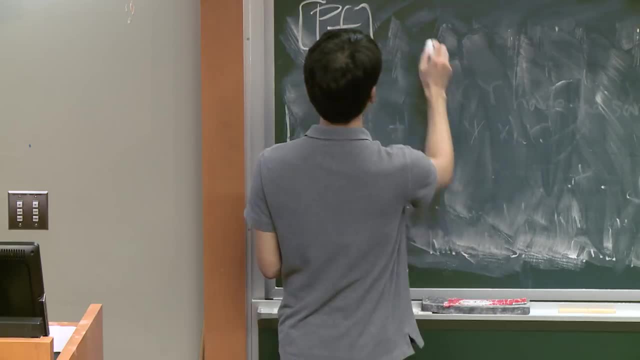 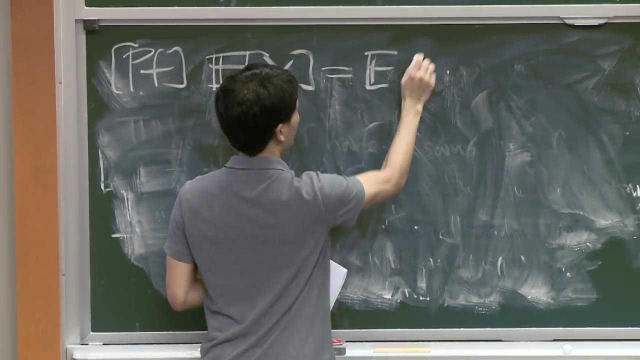 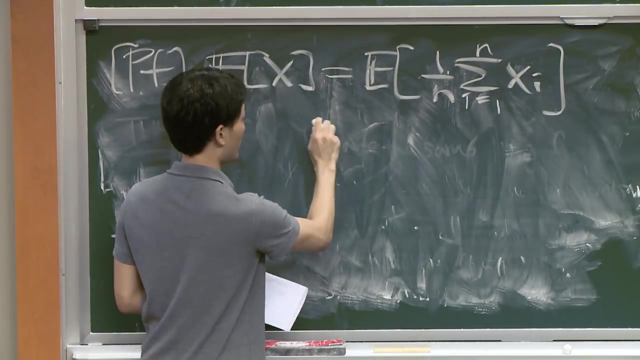 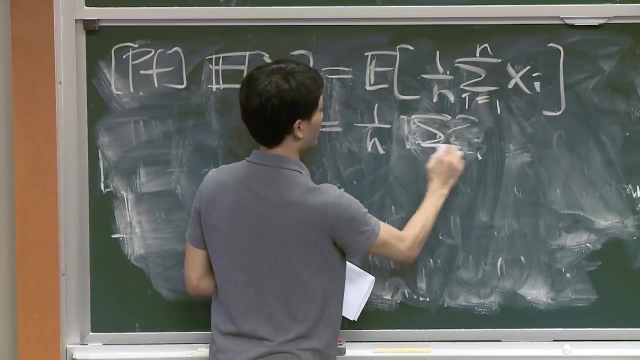 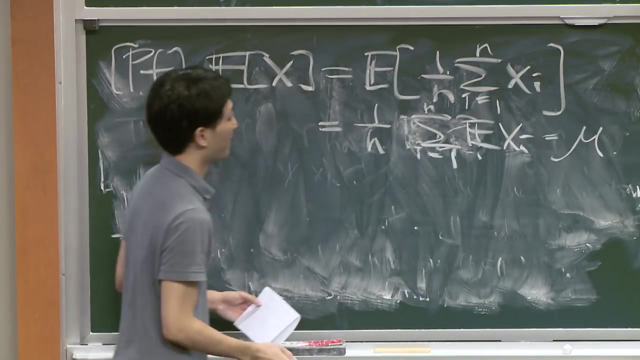 The proof is quite easy, OK. So first of all one observation: expectation of x, It's just the expectation of 1 over n times the sum of xi's, And that by linearity just becomes the sum out, And that's mu. 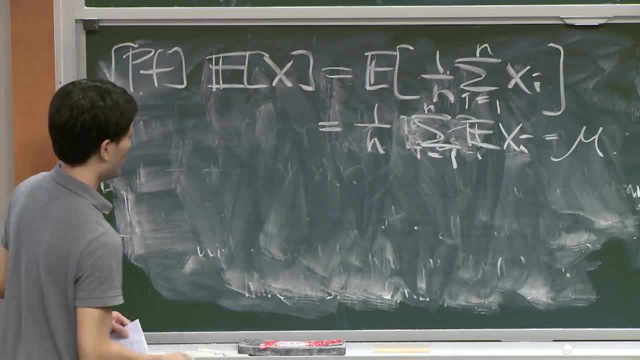 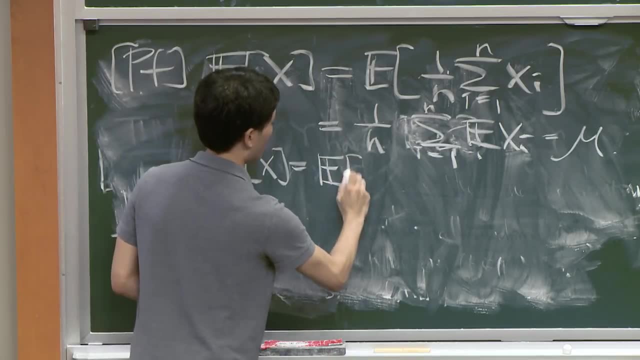 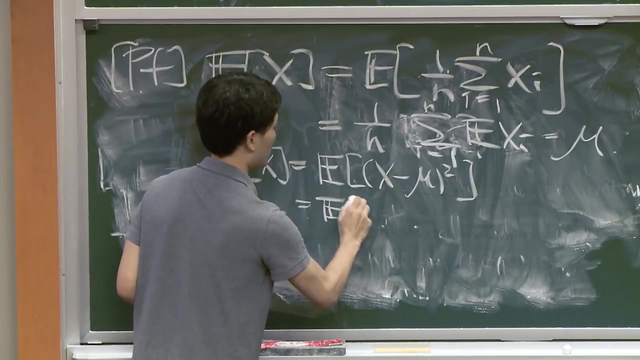 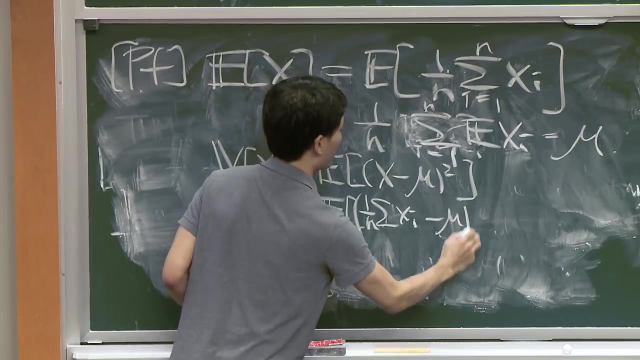 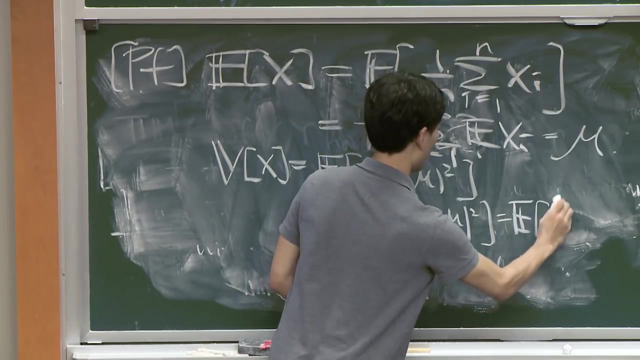 OK, So that's good. And then the variance. What's the variance of x? That's the expectation of x minus mu squared, which is the expectation sum over all i's minus mu squared. Yeah, Now group them. That's the expectation of 1 over n. sum of xi minus mu squared. 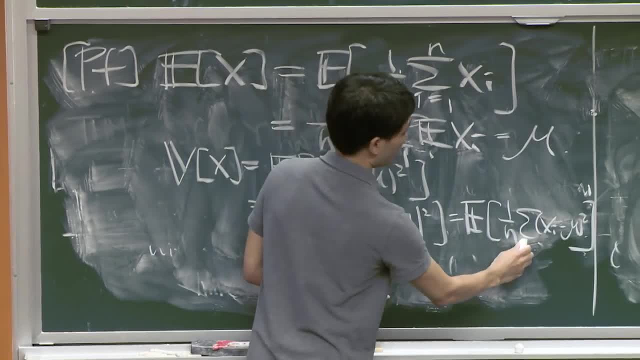 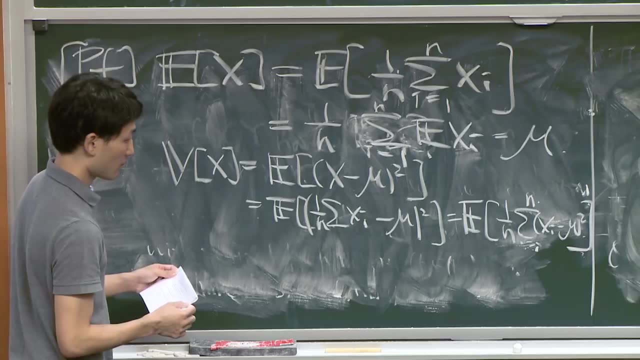 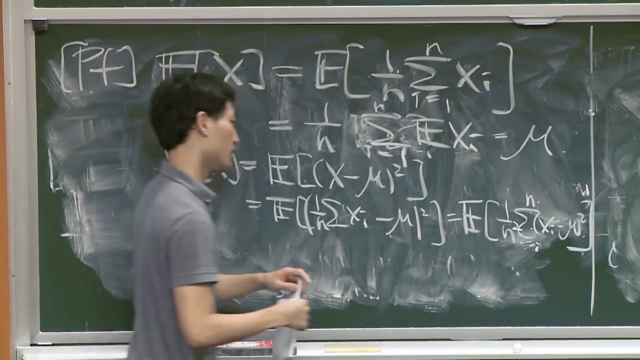 OK, So that's the expectation of 1 over n. sum of xi minus mu squared i's from 1 to n. What did I do wrong here? 1 over n is inside the square, So if you take it out, it's 1 over n squared. 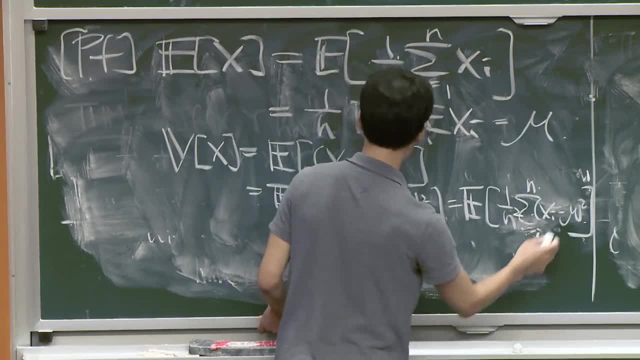 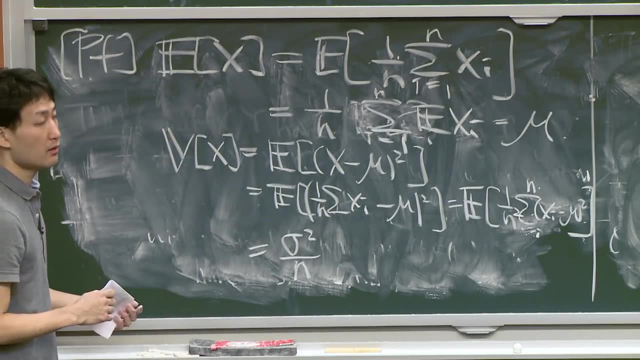 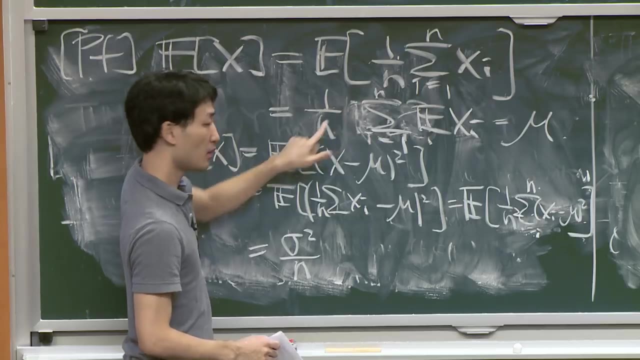 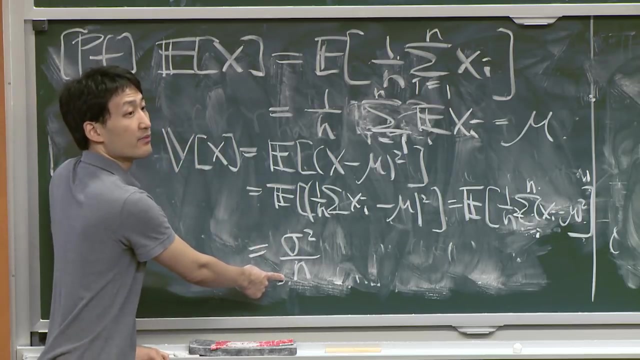 And then you're summing n terms of sigma squared. So that is equal to sigma squared over n. OK, So that means the effect of averaging n terms does not affect your average, but it affects your variance by dividing like. it divides your variance by n. 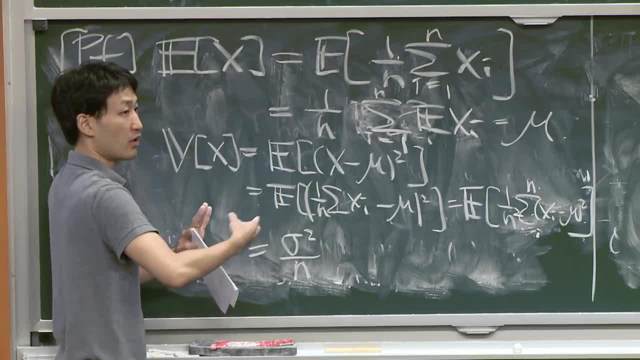 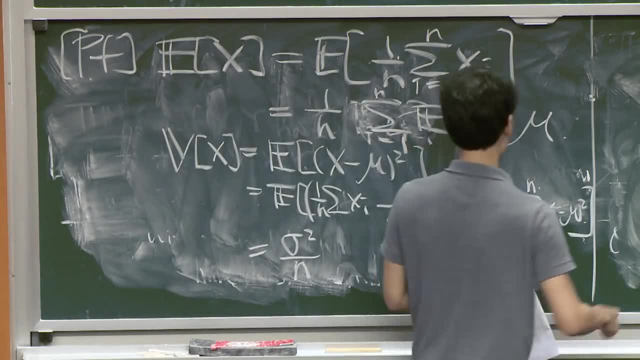 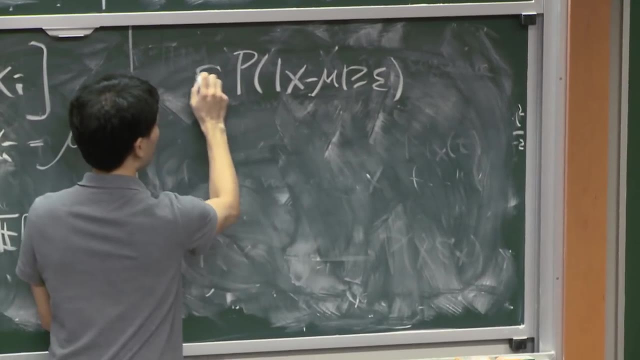 So if you take larger and larger n, your variance gets smaller and smaller, And using that we can prove this statement. There's only one thing you have to notice is the probability that x minus mu is greater than epsilon When you multiply this by epsilon squared. 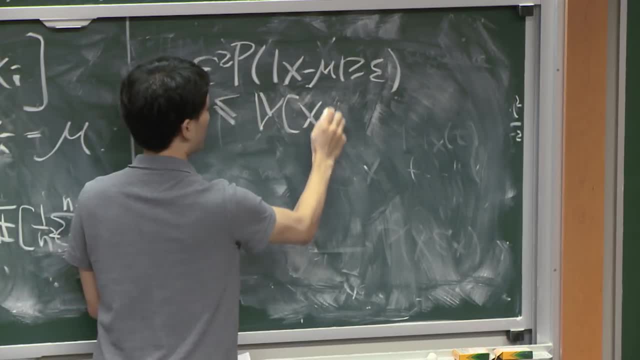 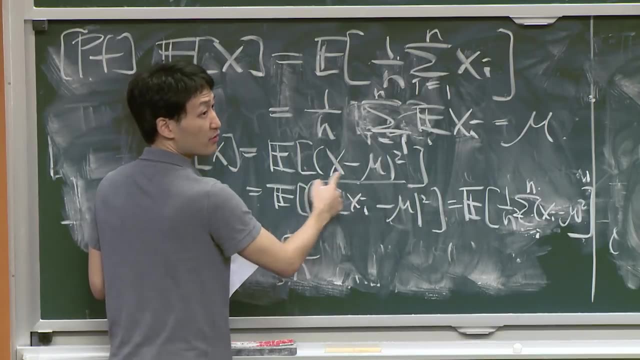 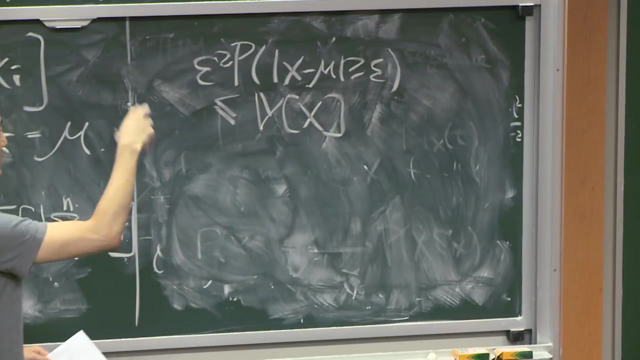 this will be less than or equal to the variance of x. The reason this inequality holds is because variance of x is defined as the expectation of x minus mu squared. For all the events, when you have x minus mu, at least epsilon, your multiplying factor x squared. 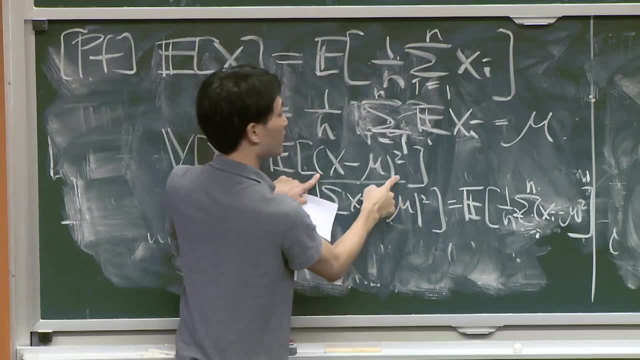 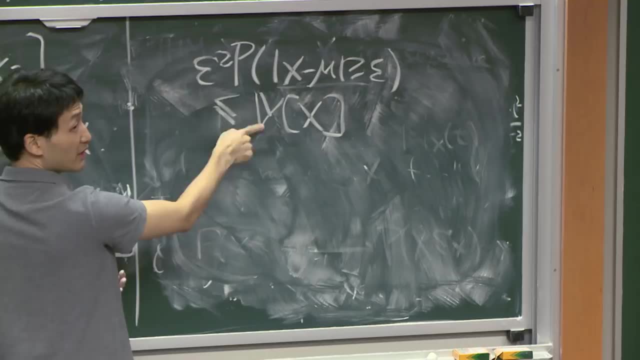 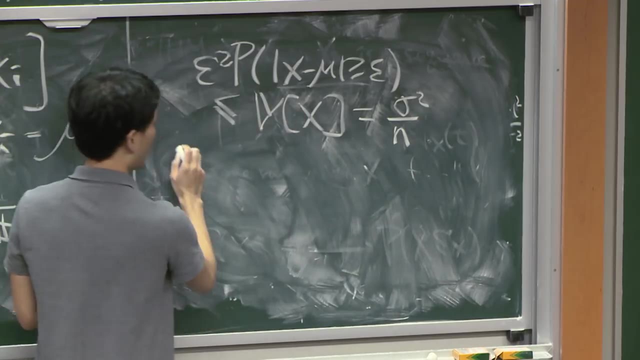 will be at least epsilon squared. This term, This term will be at least epsilon squared. when you fall into this equation, It will fall into this event. So your variance has to be at least n, And this is known to be sigma squared over n. 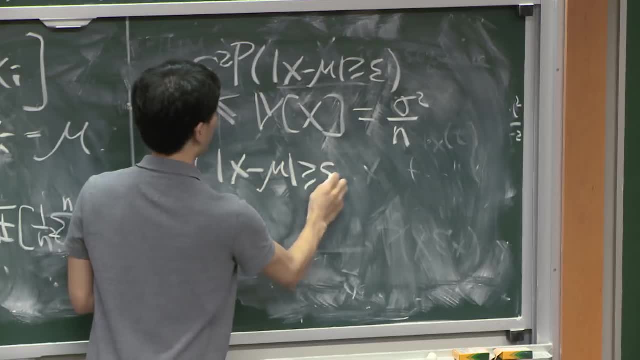 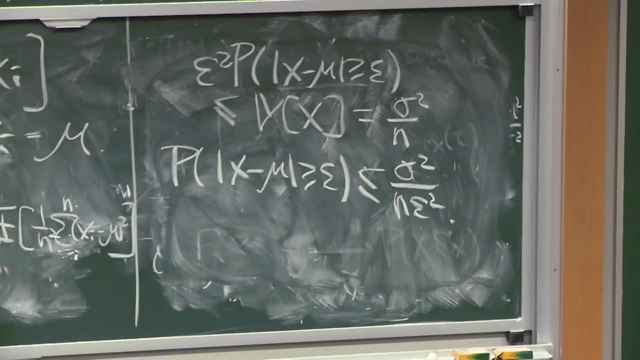 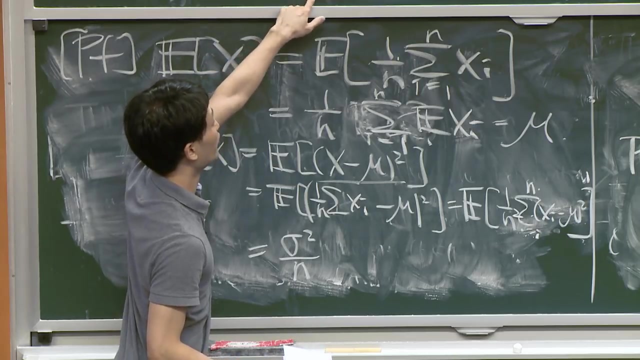 So probability that x minus mu greater than epsilon, is at most sigma squared over n. epsilon squared, That means if you take n to go to infinity, that goes to 0.. So the probability that you deviate from the mean by more than epsilon goes to 0.. 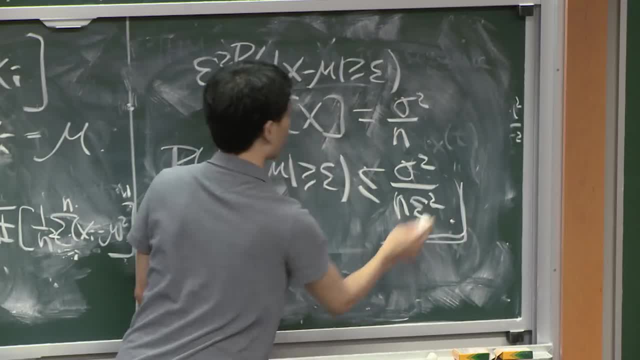 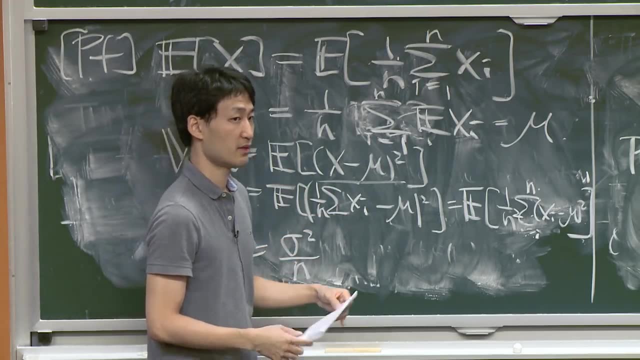 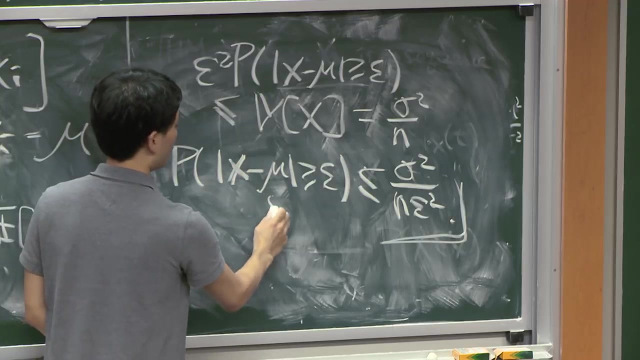 You can actually read out a little bit more from the proof. It also tells a little bit about the speed of convergence. So let's say your mean. you have a random variable x, Your mean is 50.. Your epsilon is like 0.1.. 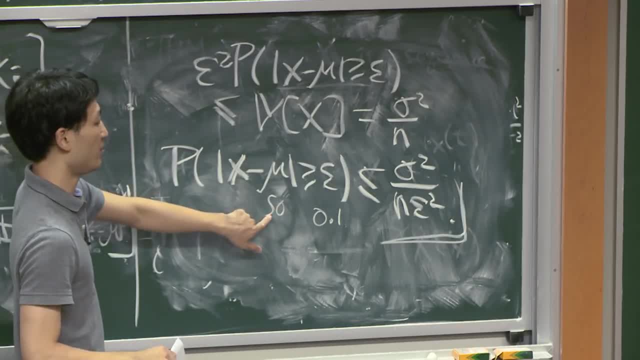 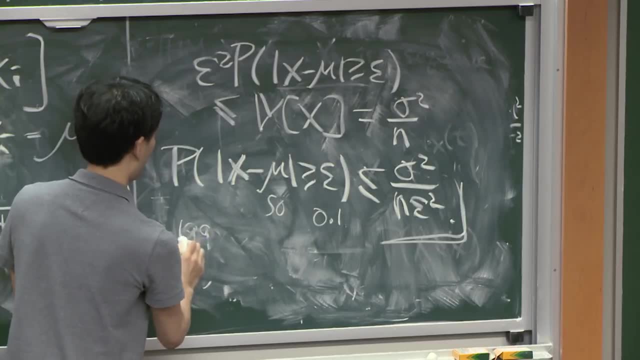 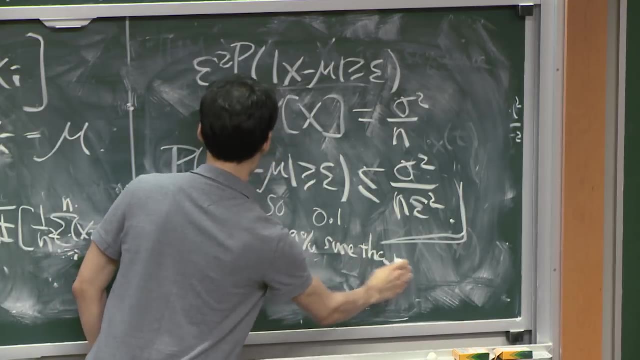 So you want to know the probability that you deviate from your mean by more than 0.1.. Let's say, You want to be sure, 99% sure, Want to be 99% sure that x minus mu is less than 0.1.. 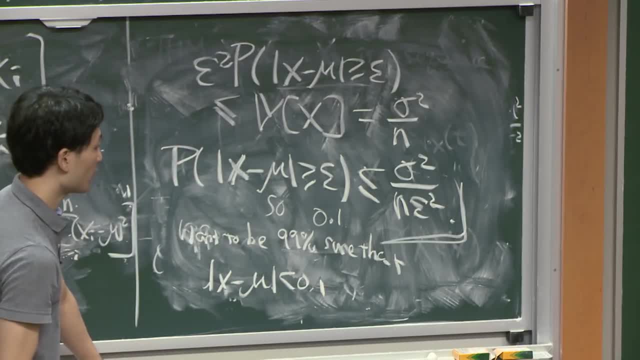 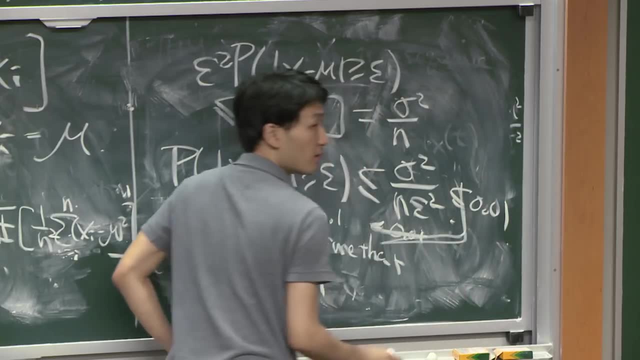 Or x minus 50 is less than 0.1.. In that case, what you can do is you want this to be 0.01.. Less to be 0.01.. So plug in that, Plug in your variance, Plug in your epsilon. 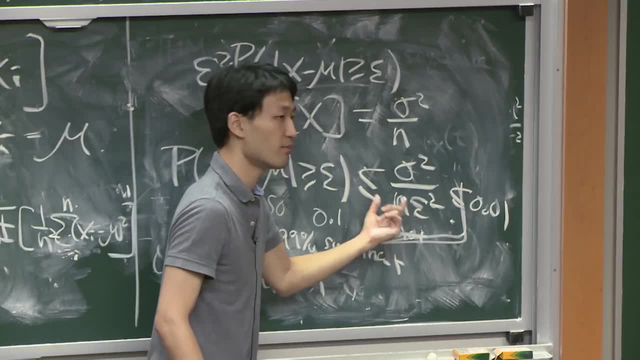 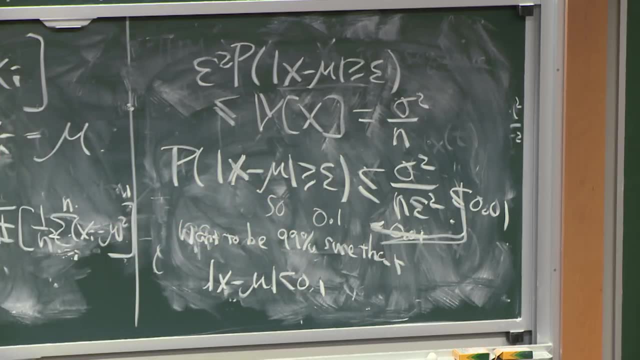 That will give you some bound on n. So if you have more than that number of trials, you can be 99% sure that you don't deviate from your mean by more than epsilon. So that does give some estimate, But I should mention that this is a very bad estimate. 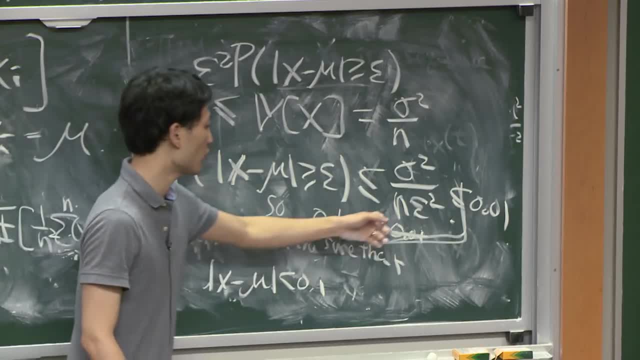 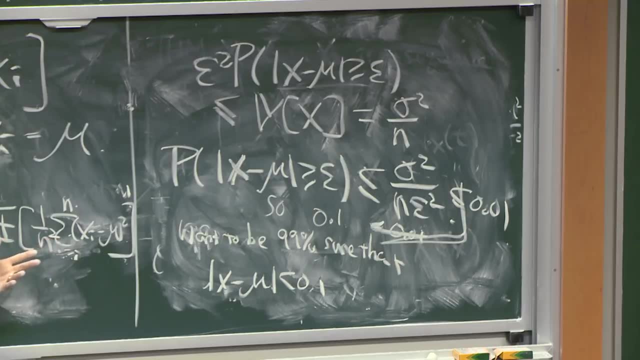 There are much more powerful estimates that can be done here. That will give the order of magnitude. I didn't really calculate here, But it looks like it's close to millions And it has to be close to millions. But in practice if you use a lot more powerful tool. 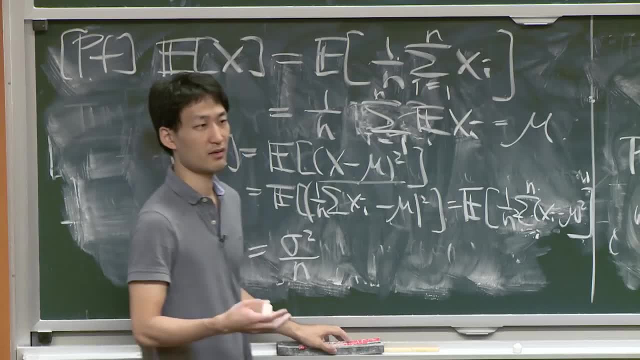 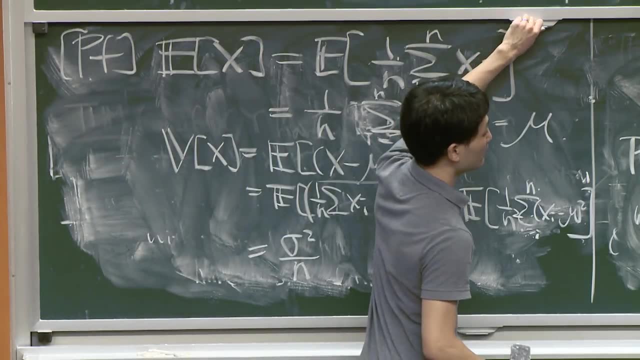 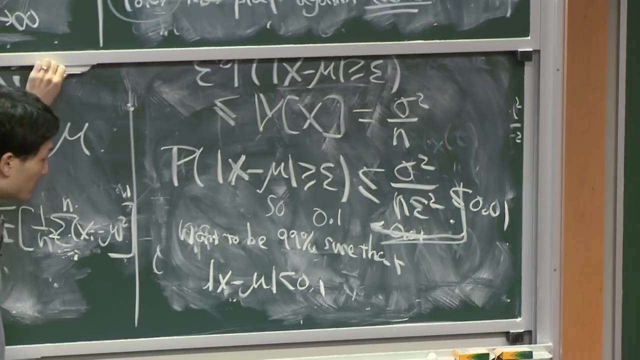 of estimating it. It should only be like hundreds or, at most, thousands, And, yeah, You can use. So the tool used there is moment-generating function, Something similar to moment-generating function, But I will not go into it. 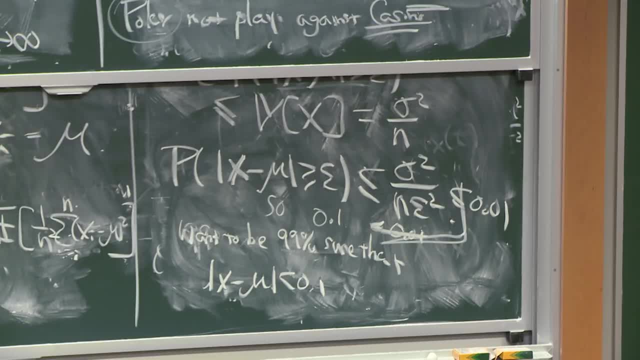 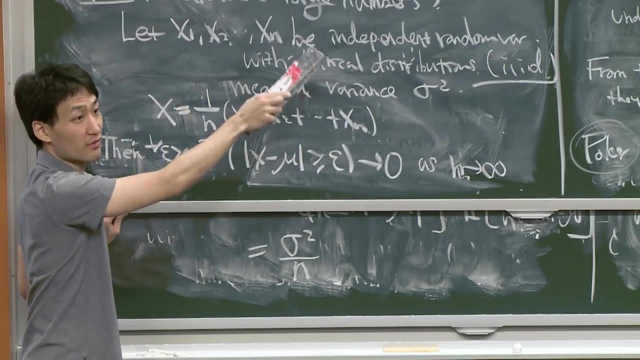 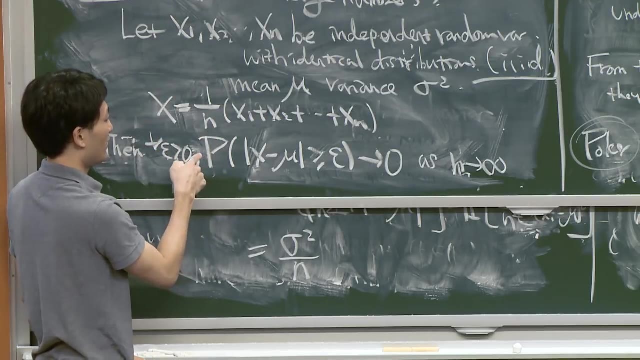 Any questions? OK, So one more thing For those who already saw large numbers before: there's also the name suggests there's also something called strong Large numbers In those theorems. in that theorem your conclusion is stronger. 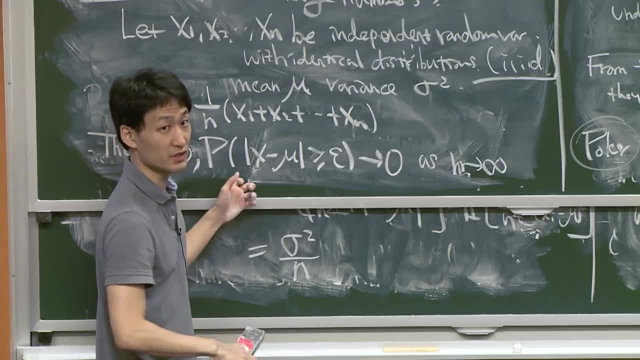 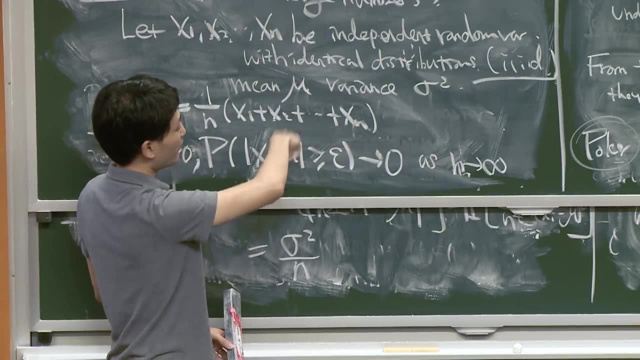 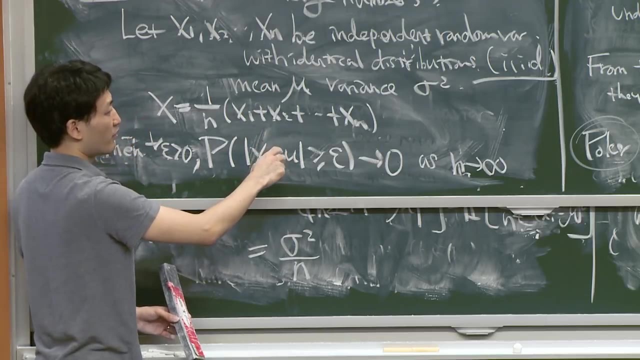 So the convergence is stronger than this type of convergence And also the conditions I gave here is a very strong condition. The same conclusion is true even if you weaken some of the conditions. So, for example, the variance does not have to exist. 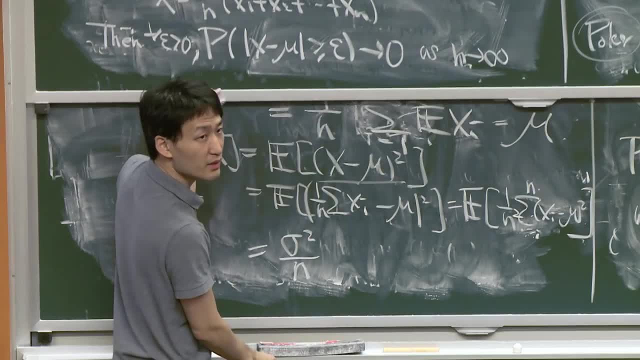 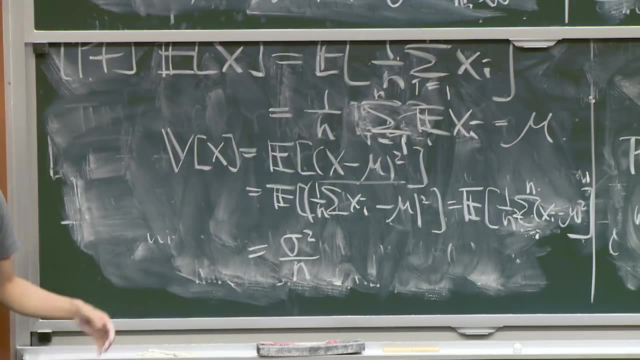 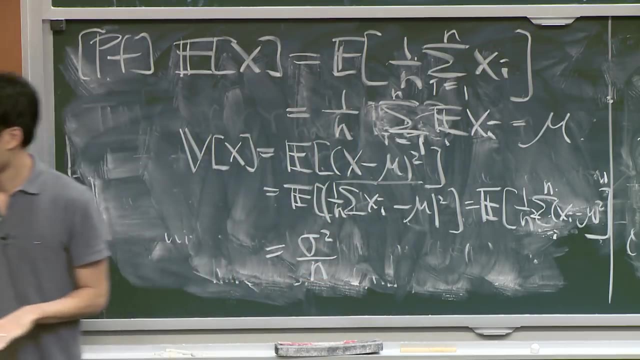 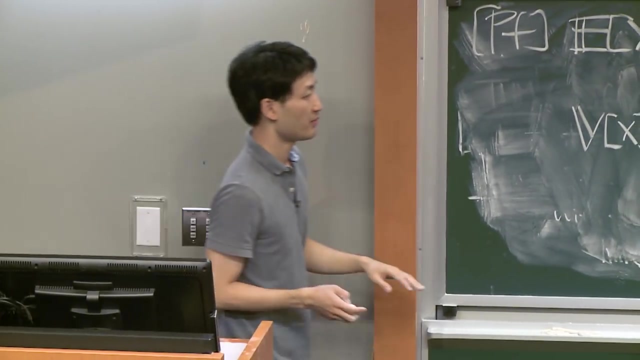 It can be replaced by some other conditions and so on, But here I just want it to be in a simple form, so that it's easy to prove And you- at least you just get the spirit of what's happening. OK, Now let's move on to the next topic: central limit theorem. 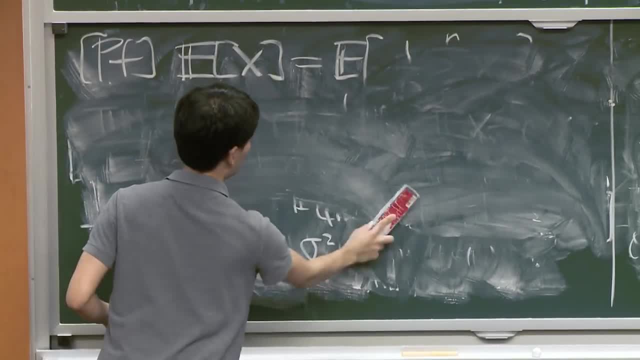 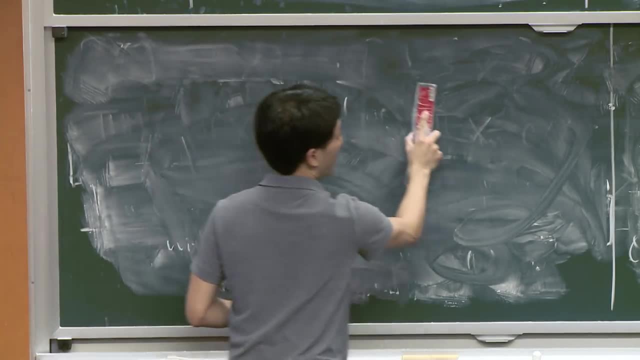 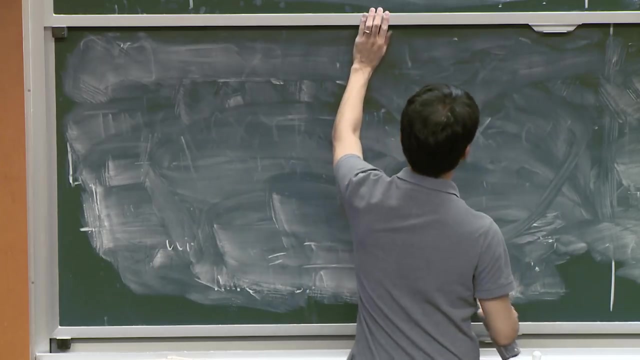 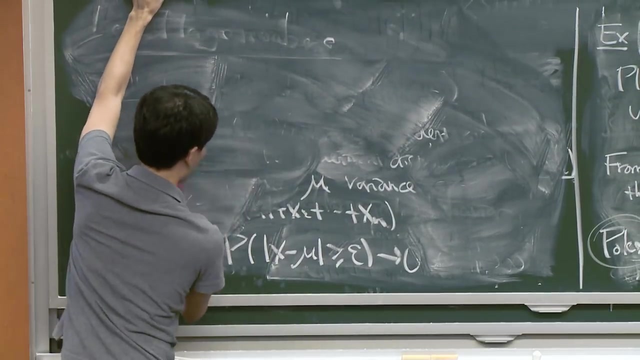 So our first dimension is to solve a problem. So this element is the element of the space. The element of the space is the size of this space. OK, So imagine that you're now taking up a large volume of space And you're actually finding out about that small amount of space. 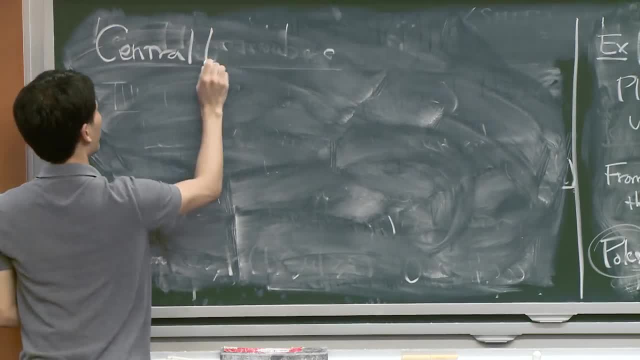 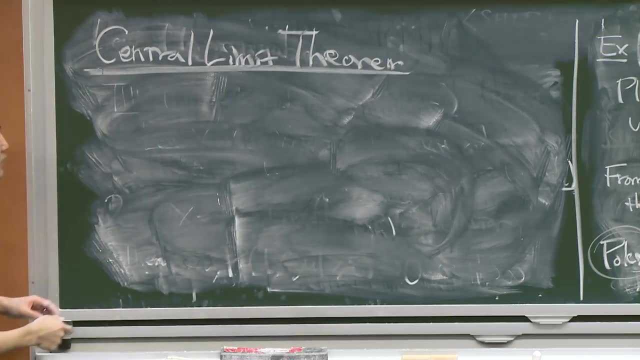 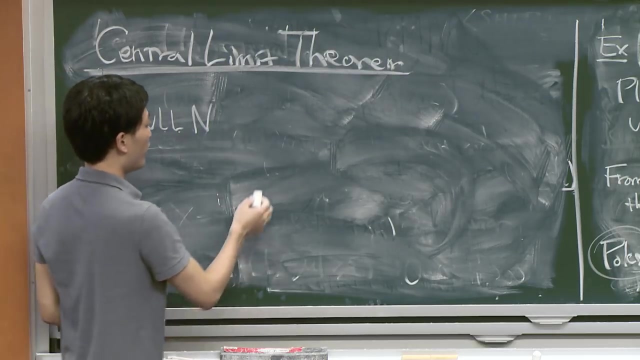 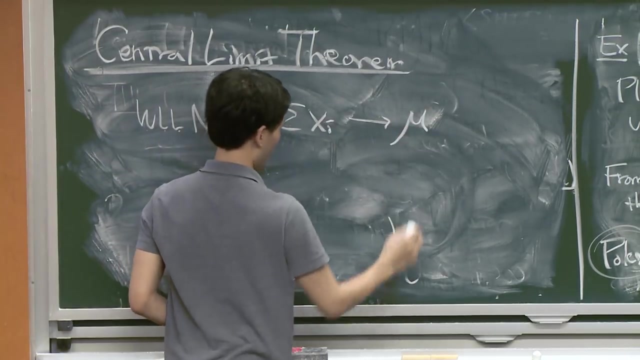 So you're doing the same thing. You just go like this: OK, OK, OK. So weak law of large number said that if you have iid random variables, 1 over n times, sum over xi converges to mu, the mean in some weak sense. 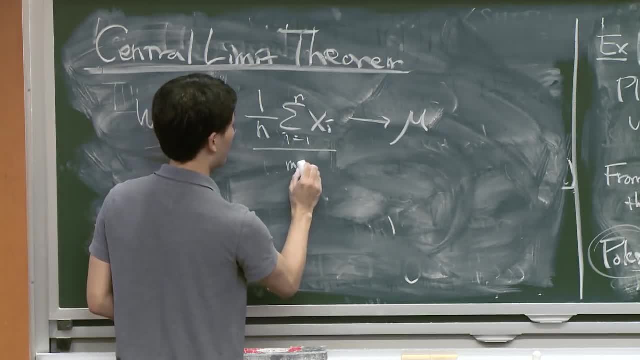 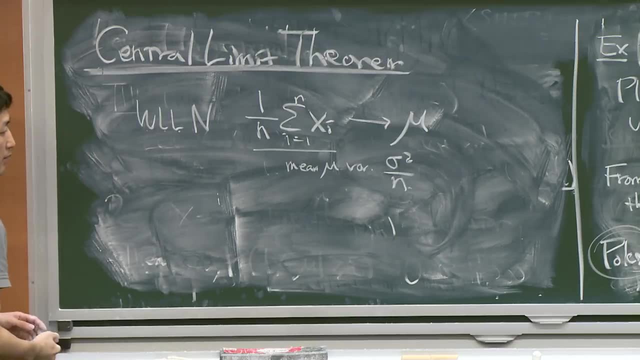 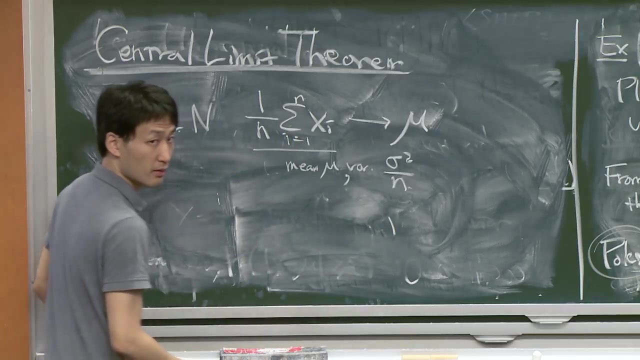 And the reason it happened was because this had mean mu and variance sigma squared over n, And we exploited the fact that variance vanishes to get this. So the question is, what happens if you replace 1 over n by 1 over square root n? 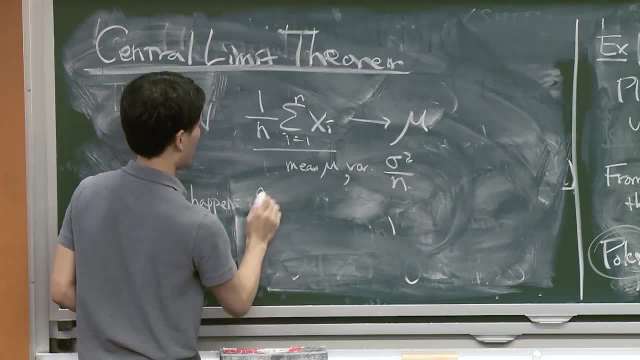 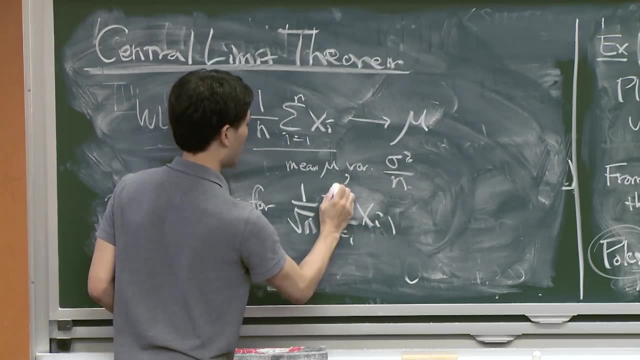 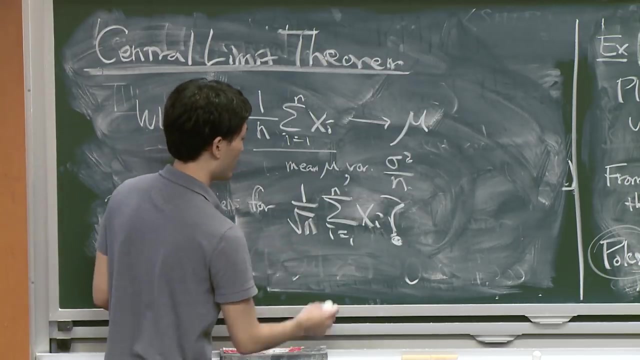 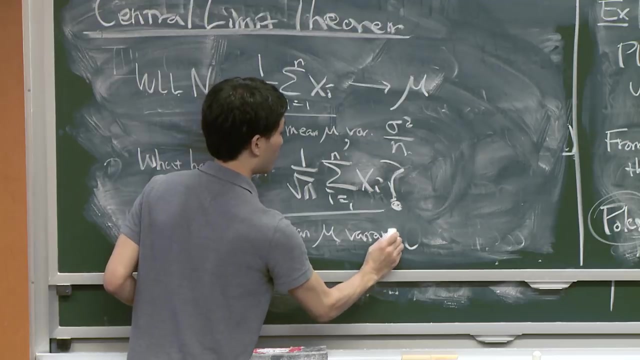 What happens if? What happens for the random variable 1 over square root n times xi? The reason I'm making this choice of 1 over square root n is because if you make this choice now, the average has mean mu and variance sigma squared. 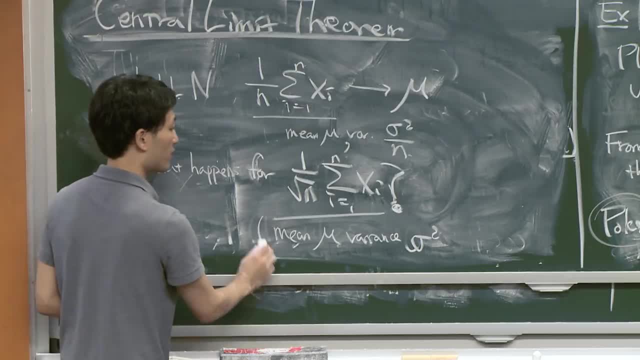 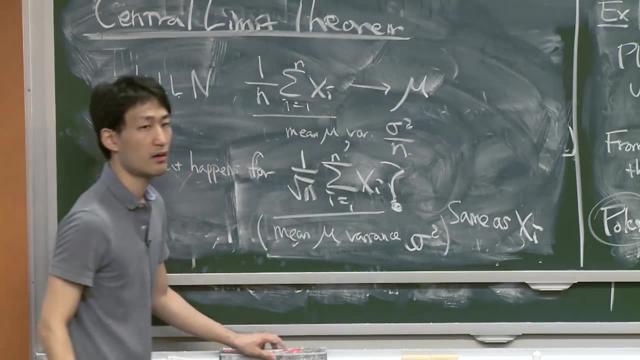 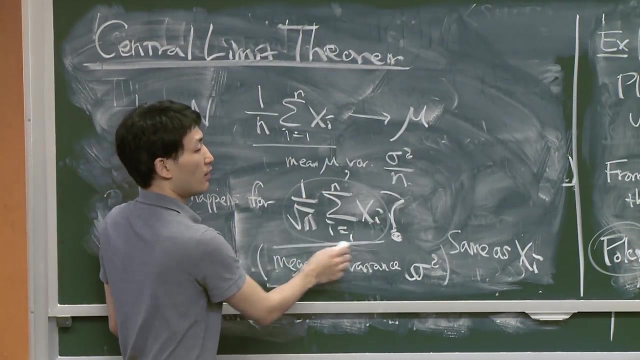 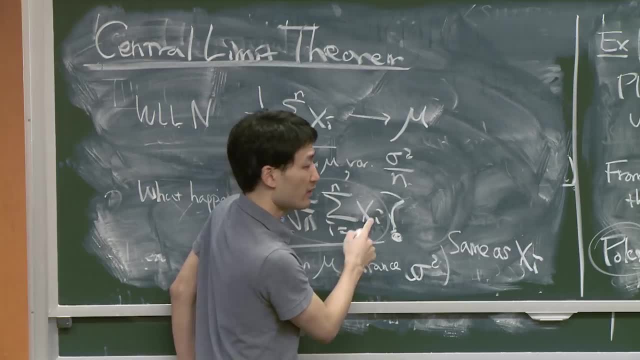 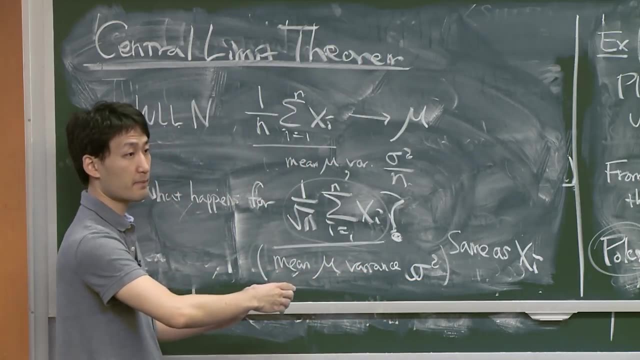 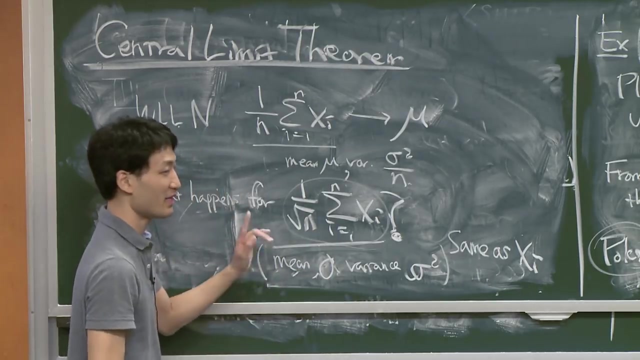 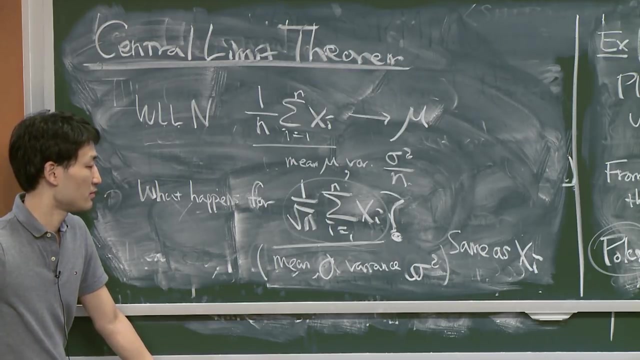 as your original random variable. should it look like the distribution of this? Should it look like the distribution of xi? Oh, If mean is mu, Thank you very much. The case when mean is 0.. Thank you For this special case. will it look like xi? 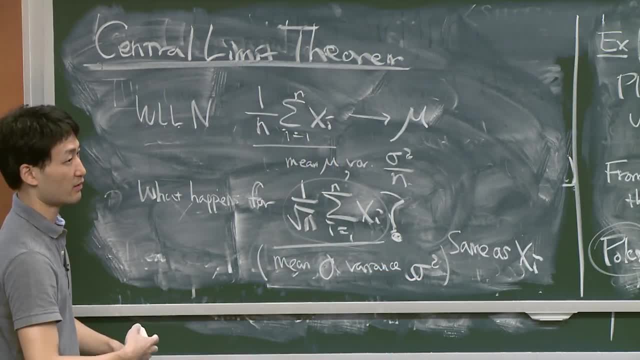 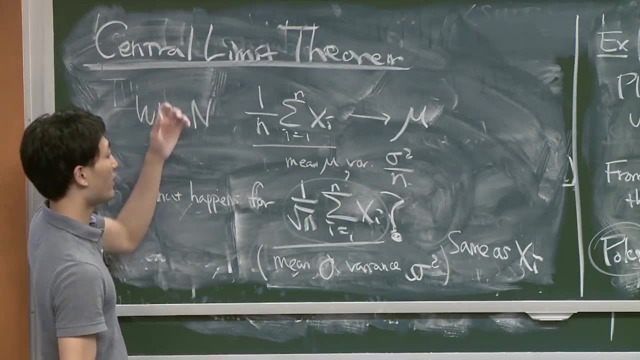 or will it not look like xi? If it doesn't look like xi, can we say anything interesting about the distribution of this? And central limit theorem answers this question, And it's actually. when I first saw it I thought it was really interesting. 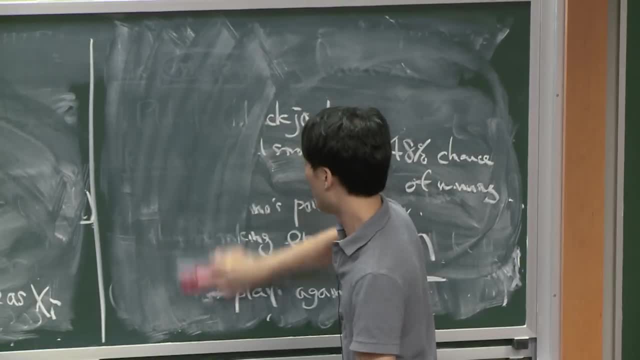 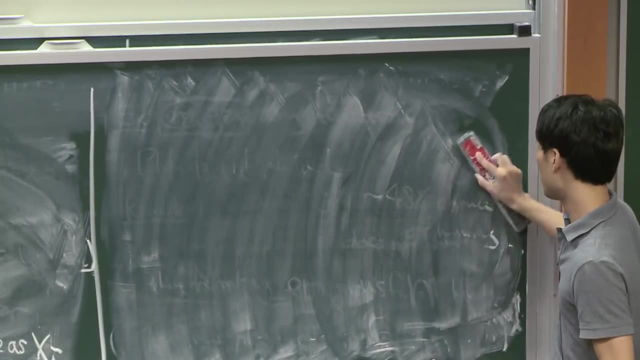 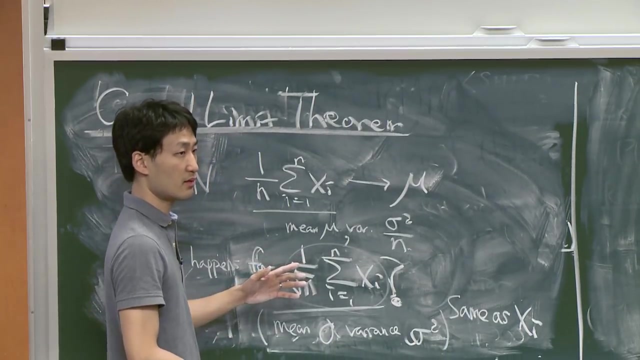 Because normal distribution comes up here, And that's probably one of the reasons that normal distribution is so universal, Because when you take many independent events and take the average, in this sense their distribution converges to a normal distribution. Yes, How did you get mean for? 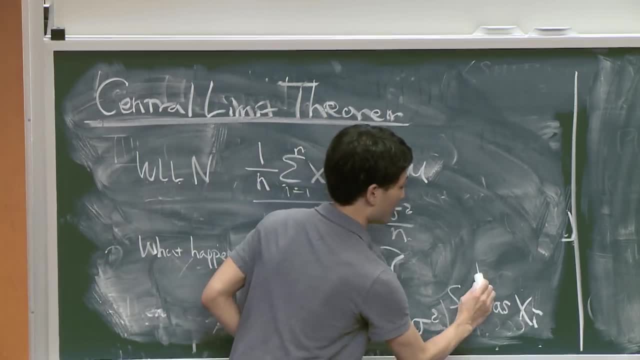 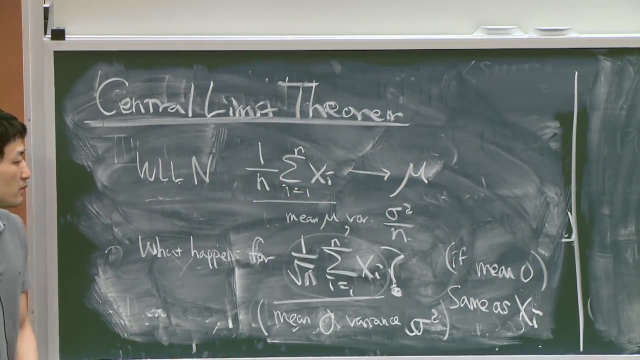 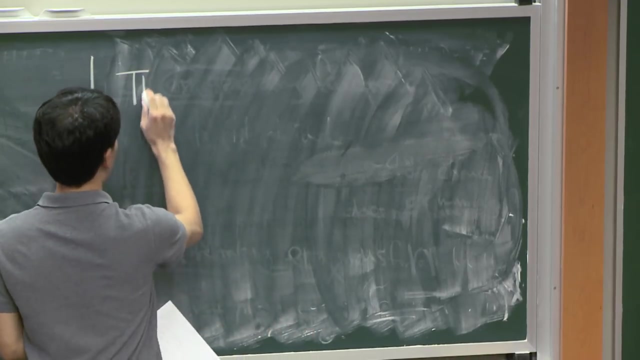 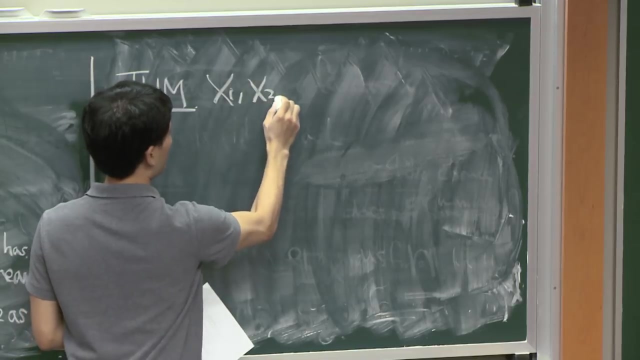 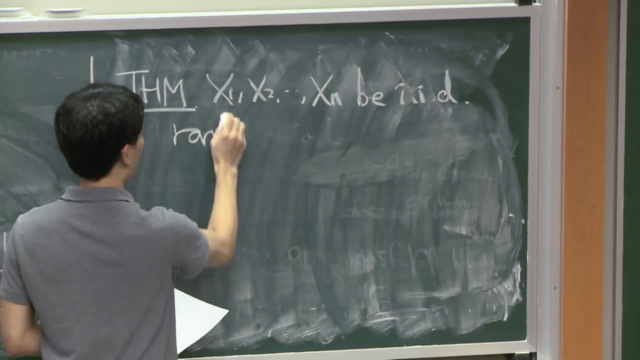 Oh no, I didn't get it. I assumed it. If x, yeah. If yeah, Yeah, xi, OK. So theorem: Let x1, x2, xN be. i i d random variables with mean. 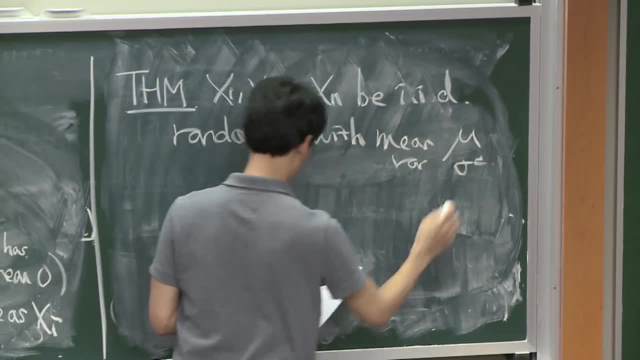 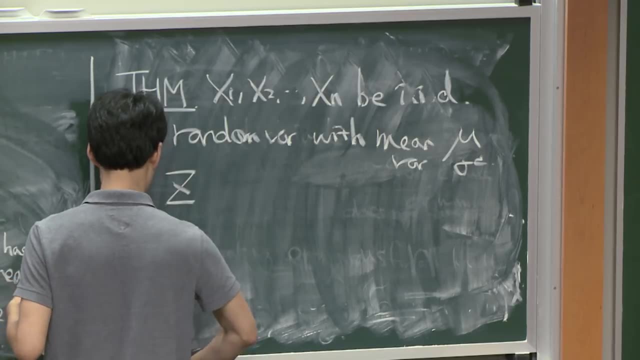 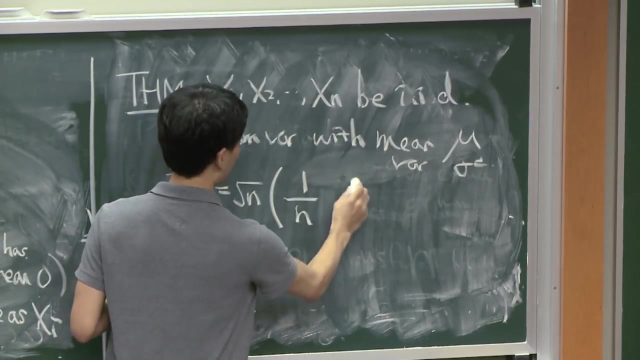 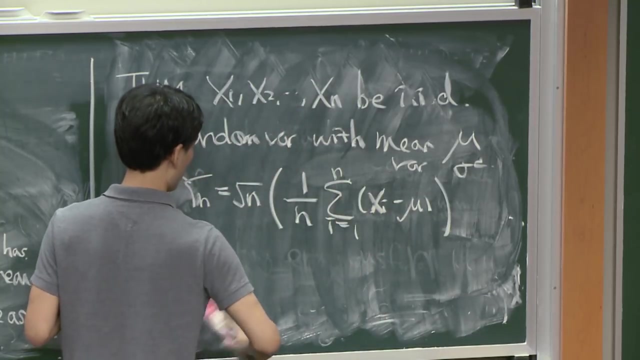 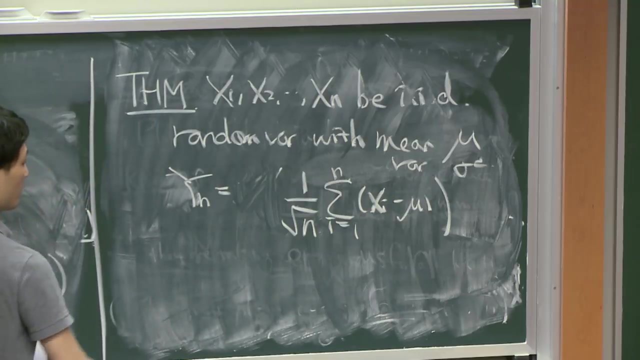 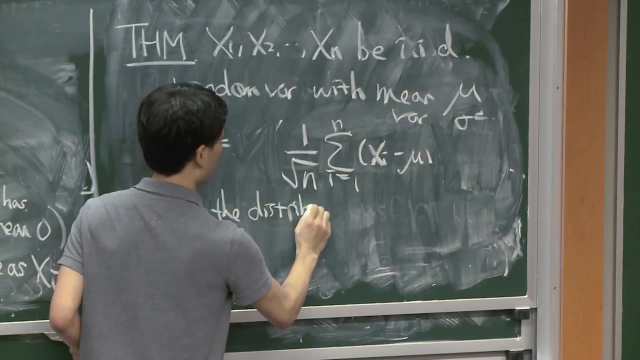 this time mu, and variable sigma-squared, And let v r yn, Let v and r yn. So the **** or yn yn b, squared n times 1 over n of xi, over mu, And then the distribution of yn. 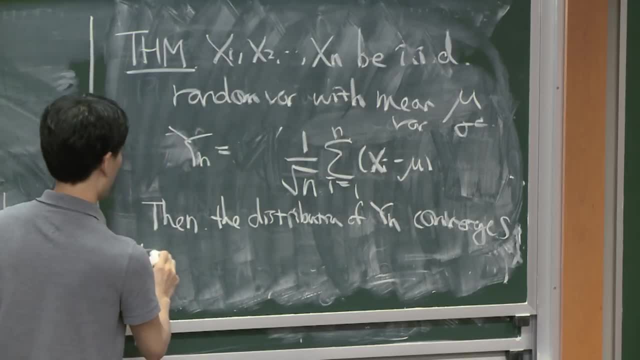 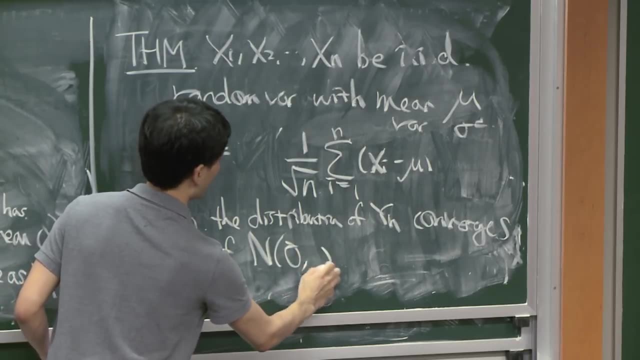 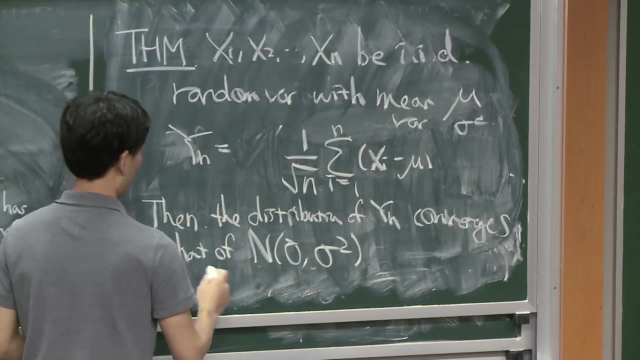 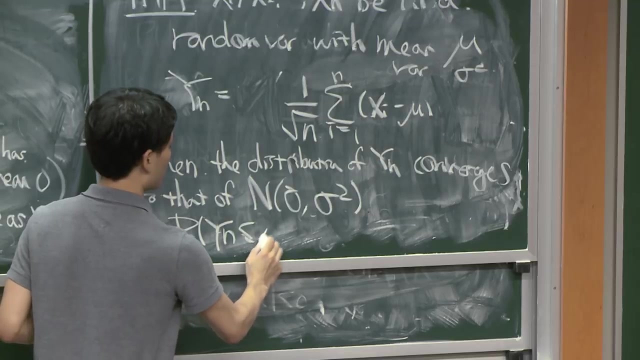 converges To that of normal distribution, with mean 0 and variance sigma. What this means I'll write it down again. It means for all x probability that yn less than or equal to x converges, the probability that normal distribution is less than or equal to x. 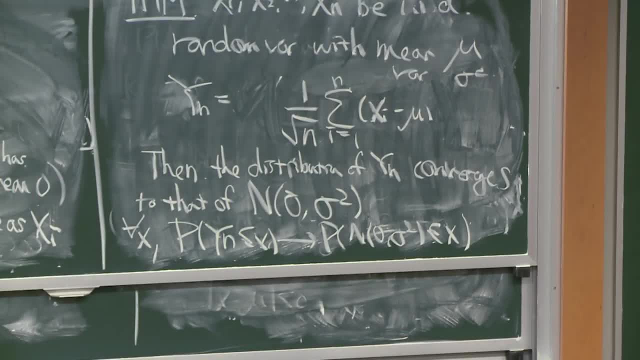 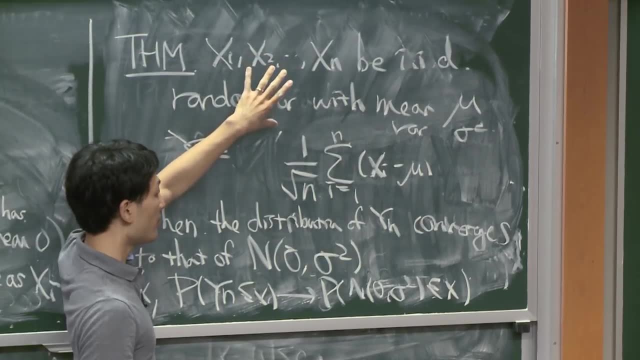 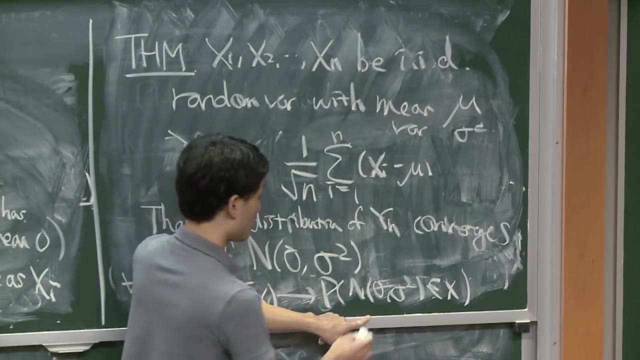 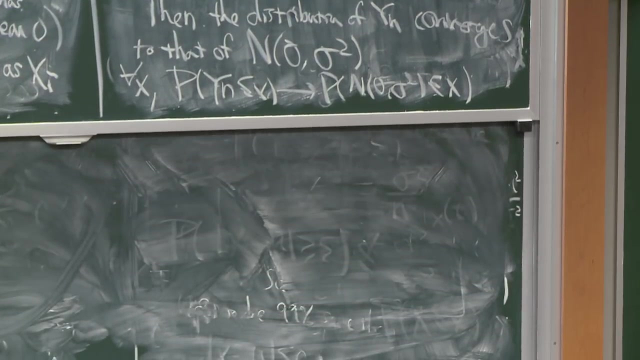 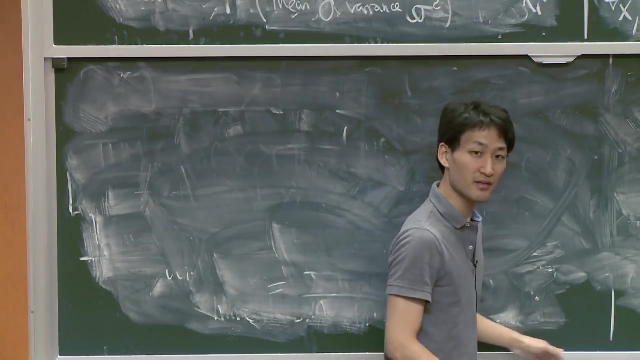 What's really interesting here is no matter what distribution you had in the beginning. if you average it out in this sense, then you converge to the normal distribution. Any questions about the statement or any corrections? Any mistakes that I made? OK? 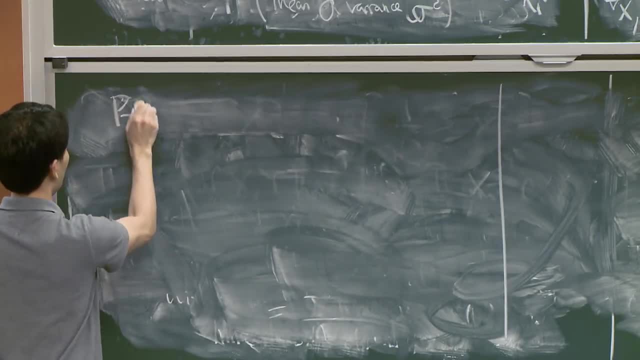 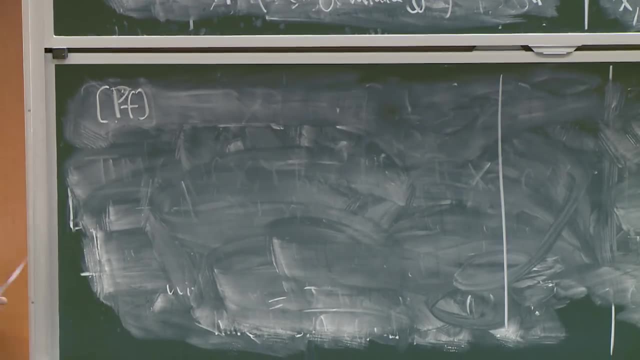 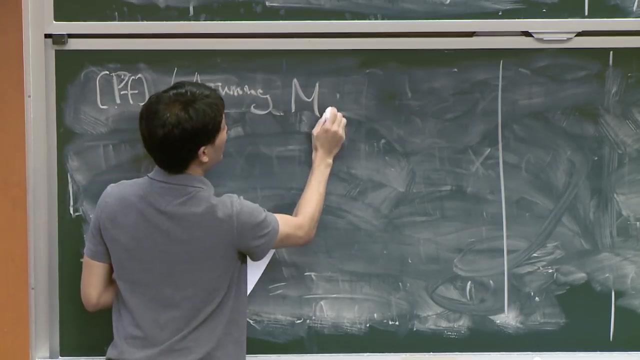 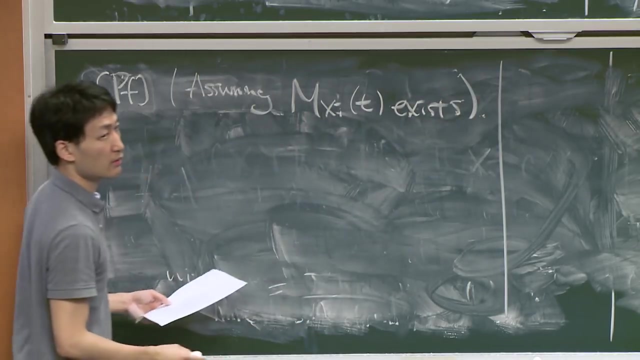 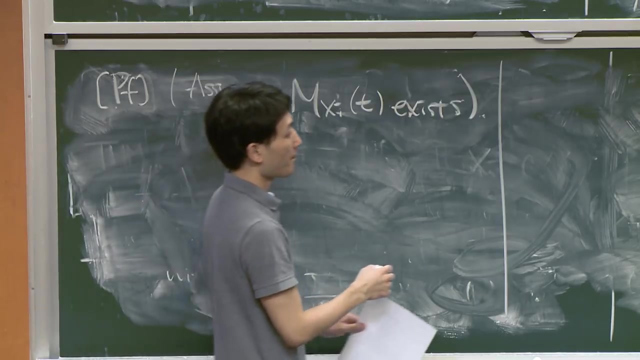 Now the proof. I will prove it. when the moment-generating function exists, So assume that the moment-generating function exists. So proof, assuming n of xi exists. So proof, assuming n of xi exists. So remember that theorem, Try to recall that theorem where, if you 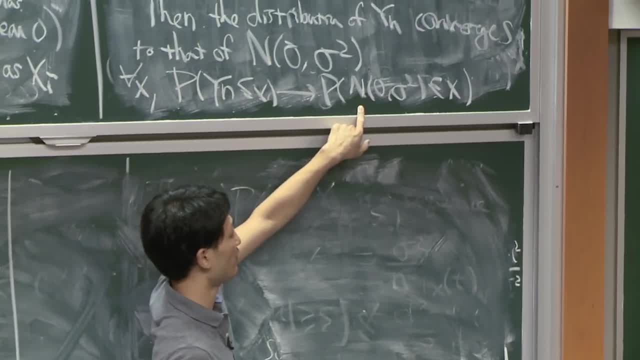 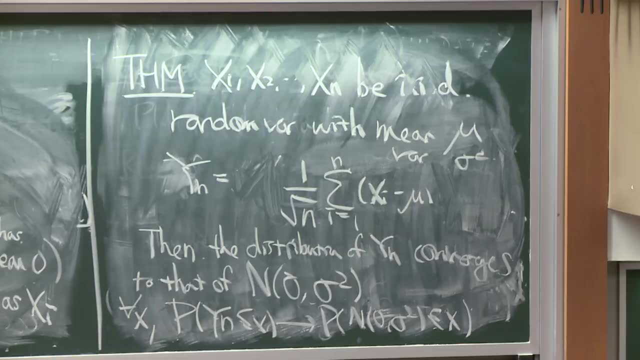 know that the moment-generating function of yn converges to the moment-generating function of the normal. then we have the statement: the distribution converges. So that's the statement we're going to use. That means our goal is to prove that the moment-generating 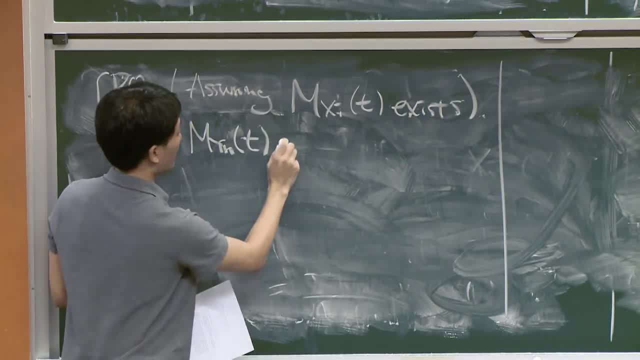 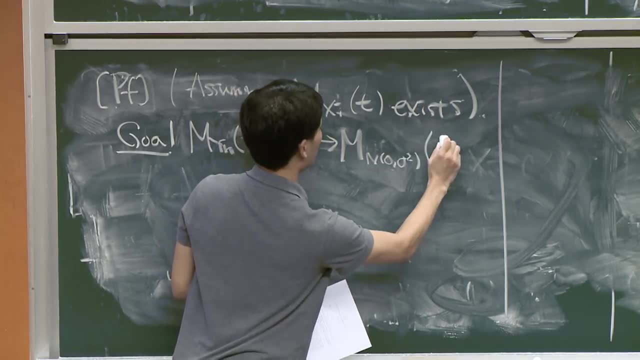 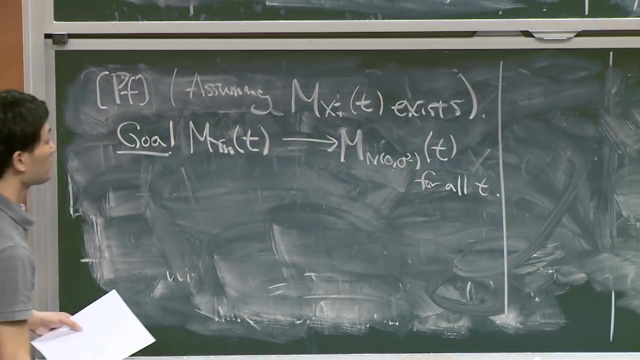 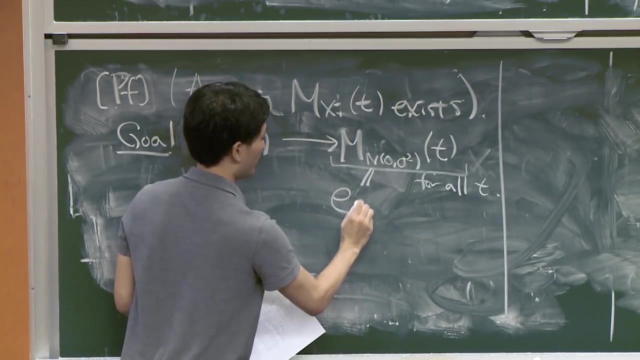 function of these yn's converges. OK, Of these yn's converge to the moment-generating function of the normal for all t point-wise convergence. And this part is well known. I'll just write it down. It's known to be e to the t squared sigma squared over 2.. 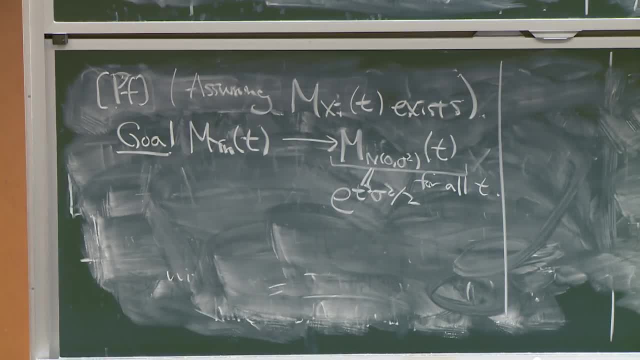 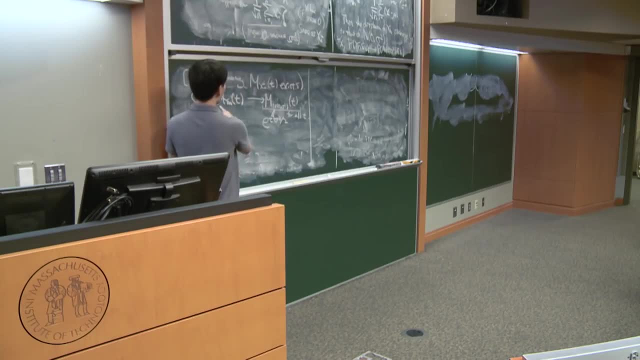 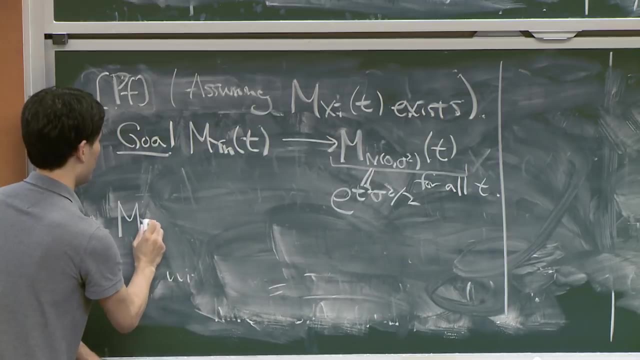 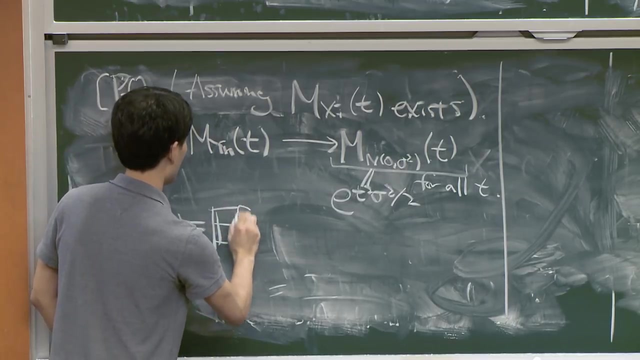 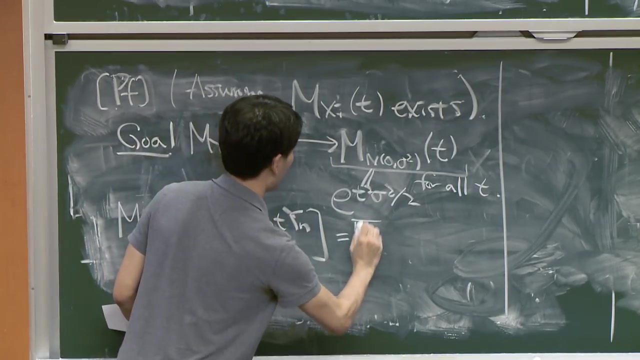 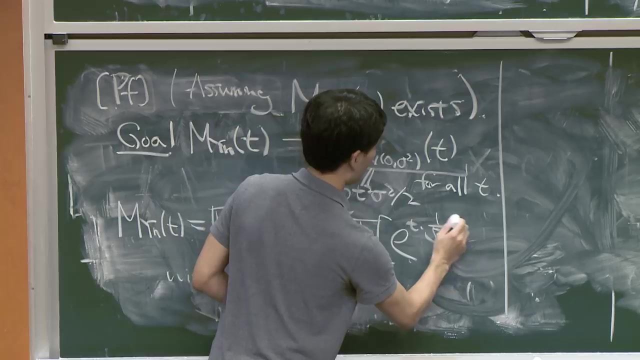 And that just can be computed. So we want to somehow show that the moment-generating function of this yn converges to that Moment-generating function of yn is equal to expectation of e to the t yn. So this is t: 1 over squared n, sum of xi minus mu. 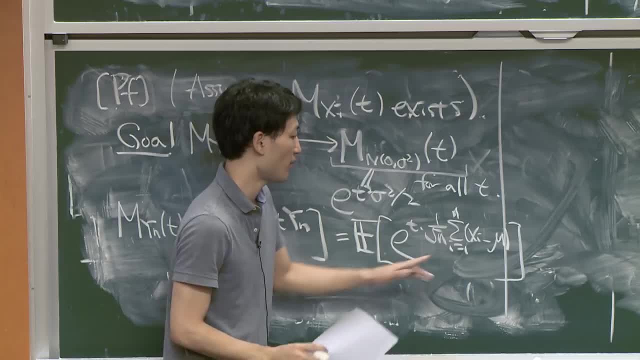 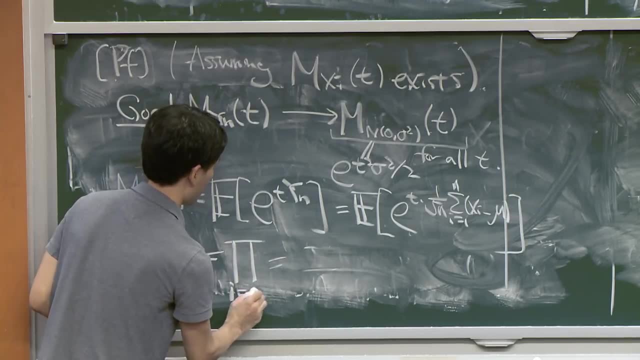 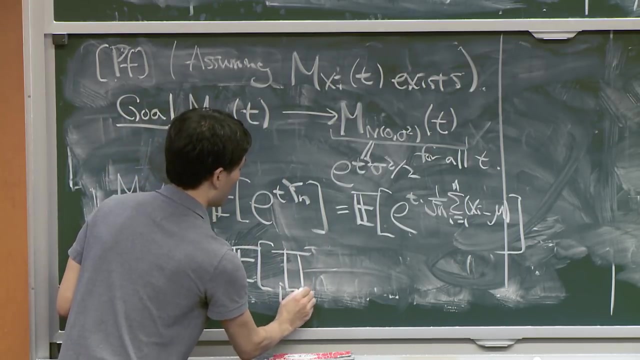 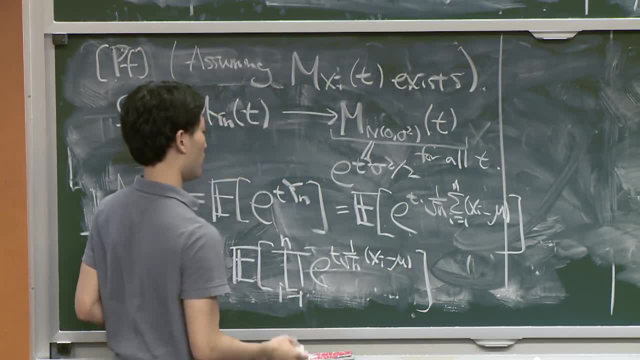 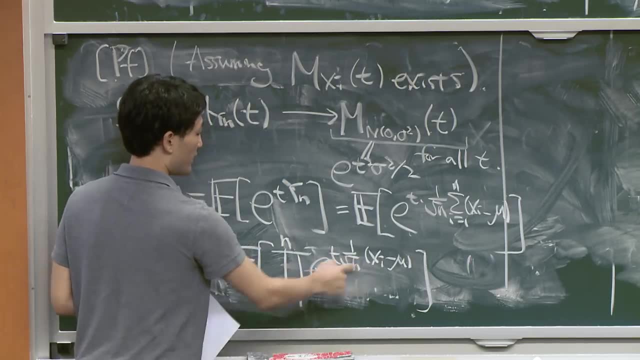 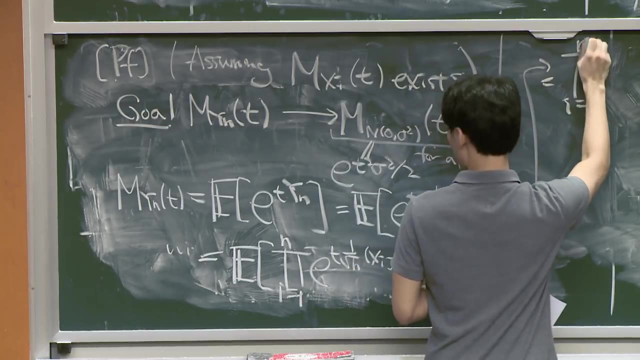 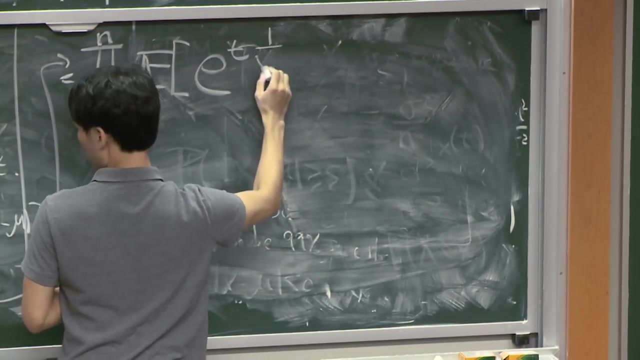 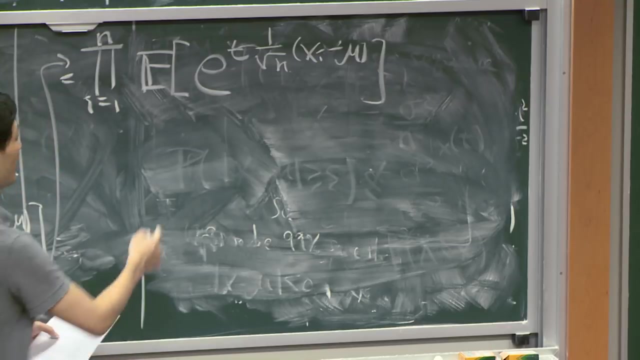 minus mu. And then, because they're independent, this product can go out. This product can go out. Equal to the product from 1 to n. expectation of e to the t squared n. OK, now they are identically distributed. 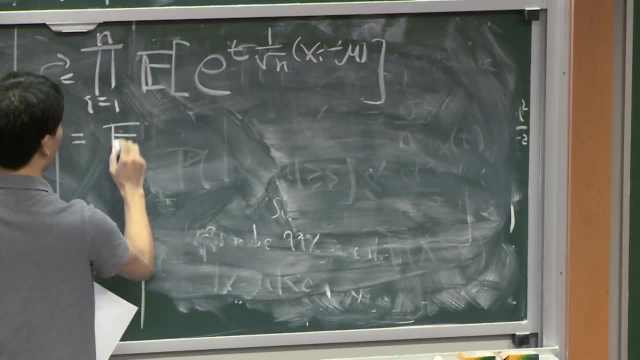 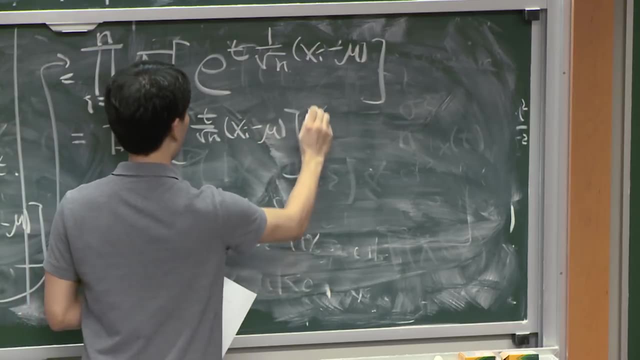 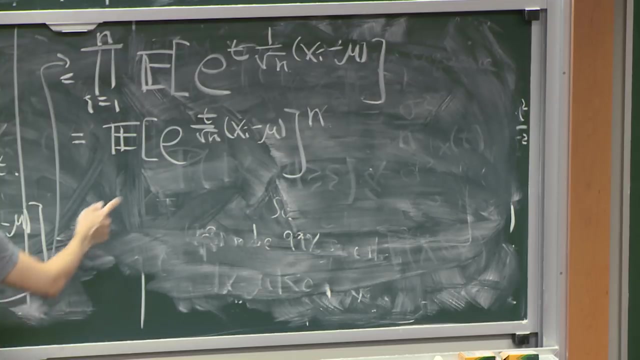 So you just have to take the nth power of that. That's equal to the expectation of e to the t over squared n, xi minus mu To the nth power. Now we'll do some estimation, So use a Taylor expansion of this. 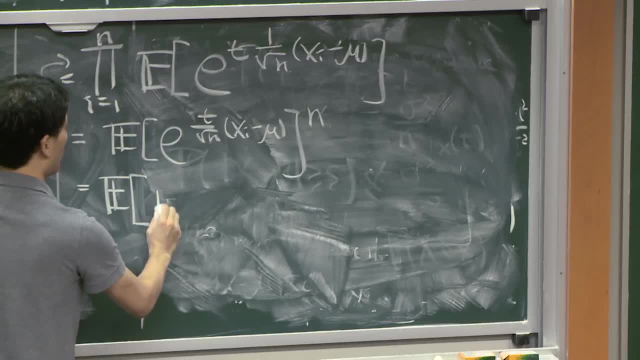 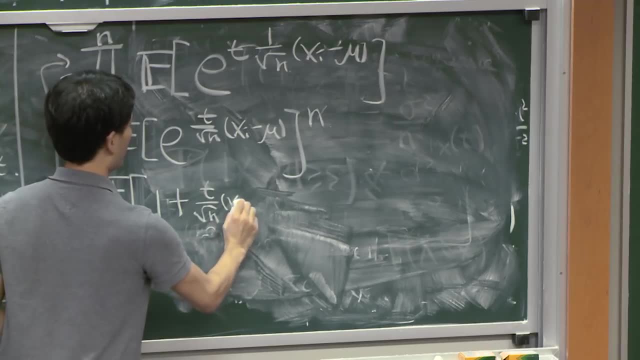 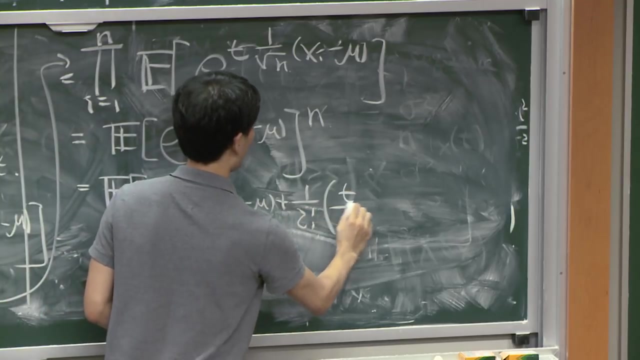 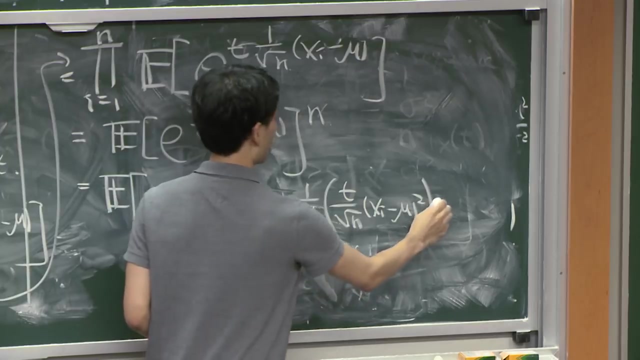 What we get is expectation of 1 plus that, t over squared n xi minus mu, plus 1 over 2. factorial that squared t over squared n xi minus mu, squared plus 1 over 3. factorial that cubed plus so on. 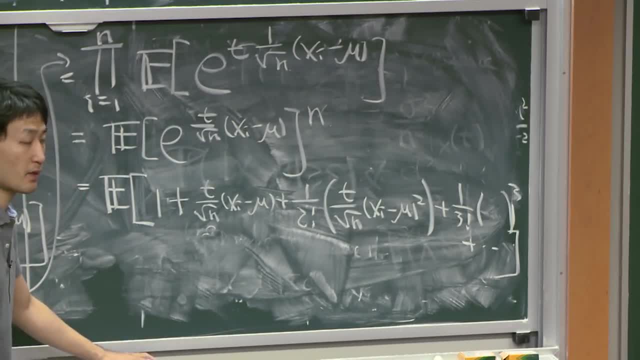 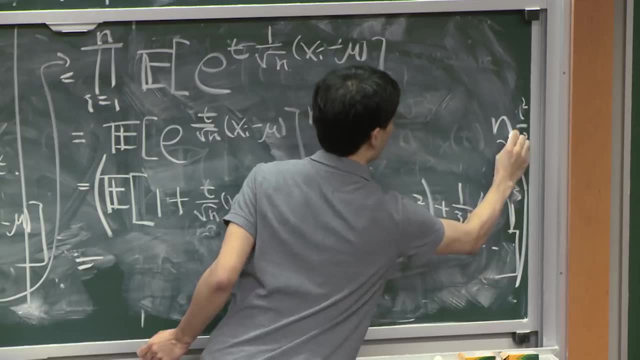 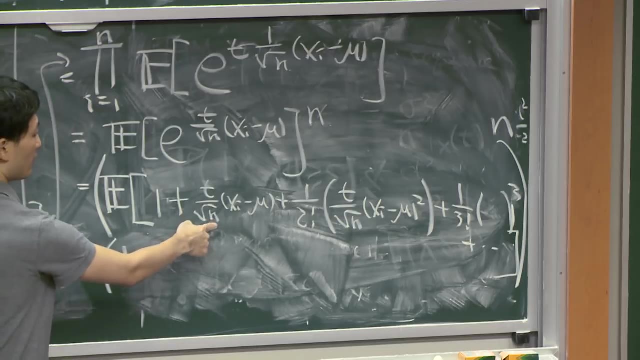 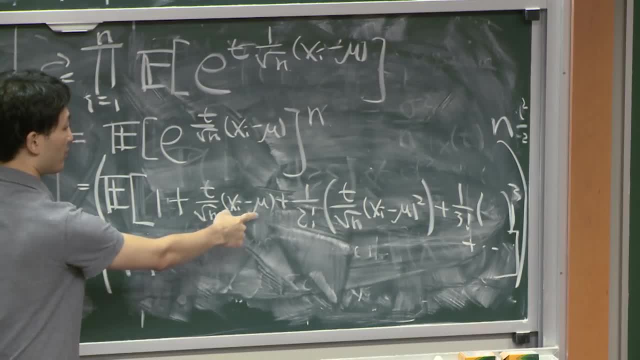 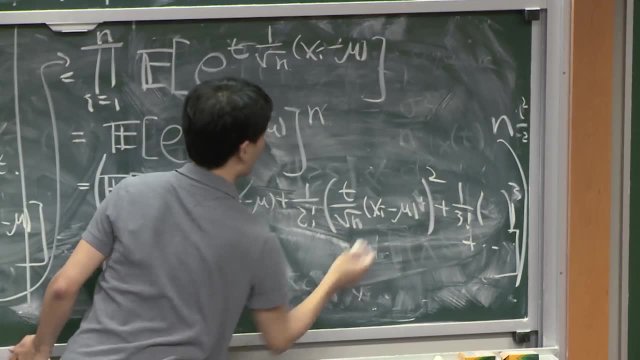 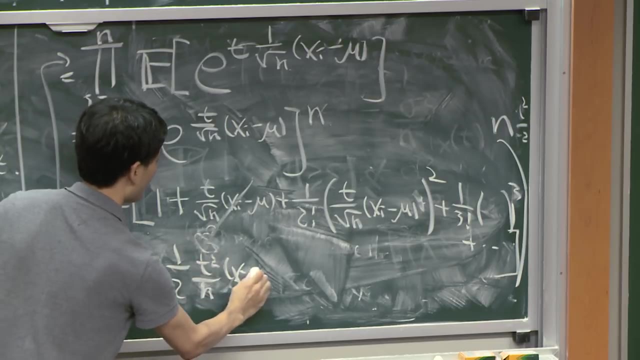 1 comes out, It's 0, because xi has a mean mu That disappears This term. we have 1 over 2, t squared over n. xi minus mu squared. xi minus mu squared. when you take expectation that will be sigma squared. 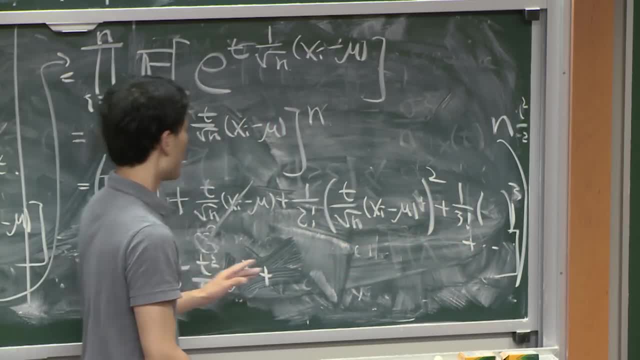 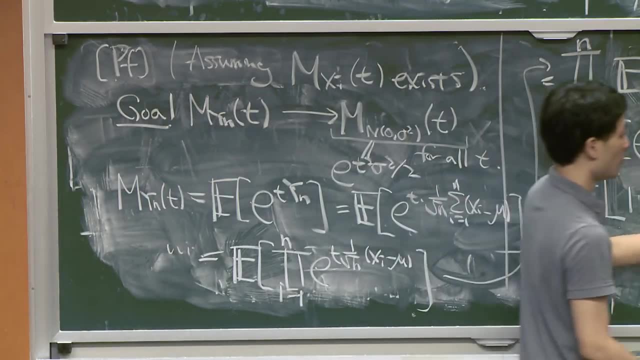 And then the terms after that, Because we're only interested in proving that for fixed t this converges. so we're only proving pointwise convergence. we may consider t as a fixed number, So as n goes to infinity if n is really really large. 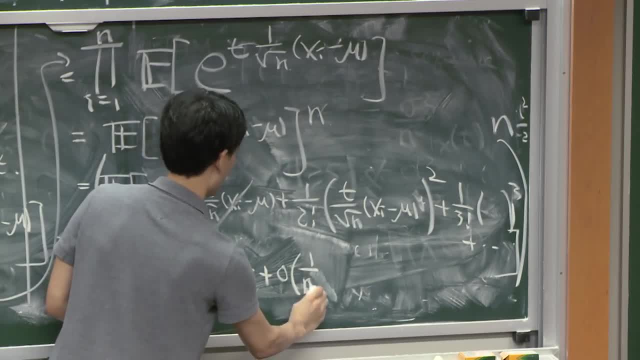 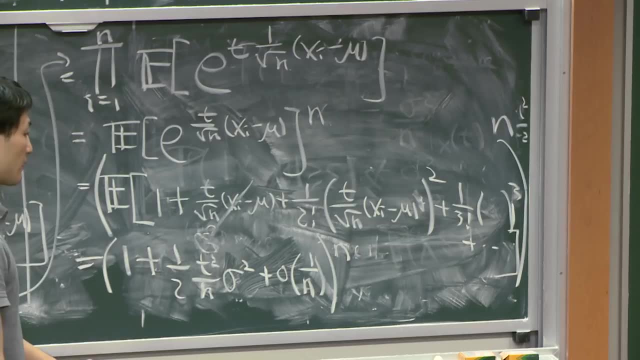 all these terms will be smaller order of magnitude than 1 over n. Something like that happens, And that's happening because for fixed t we have to prove it. If we're saying something uniformly about t, that's no longer true. Now we go back to the exponential form. 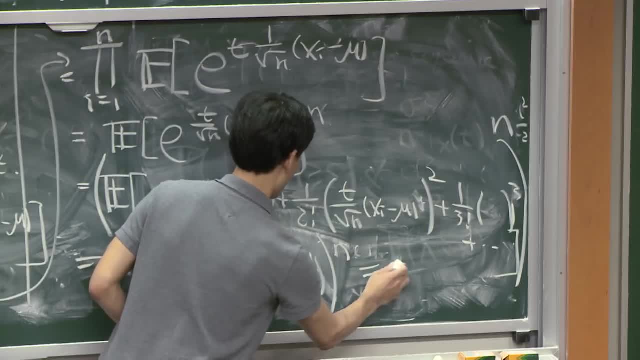 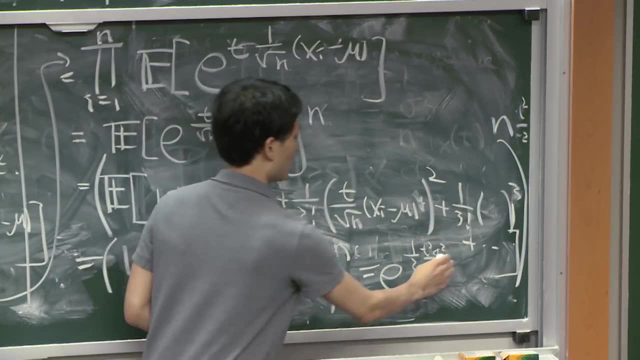 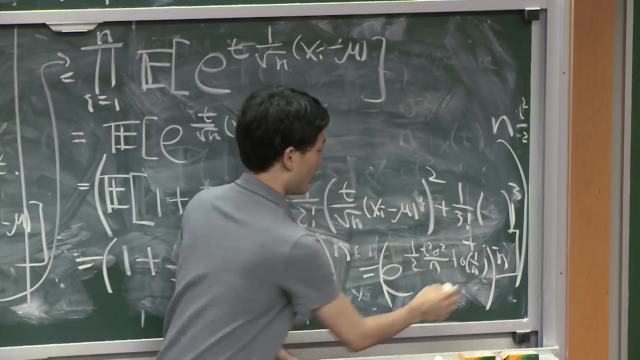 So this is pretty much just e to that term: 1 over 2, t squared sigma squared over n, plus a little over 1 over n to the n star. Now that n, That n, can be multiplied to cancel out, cancel out. 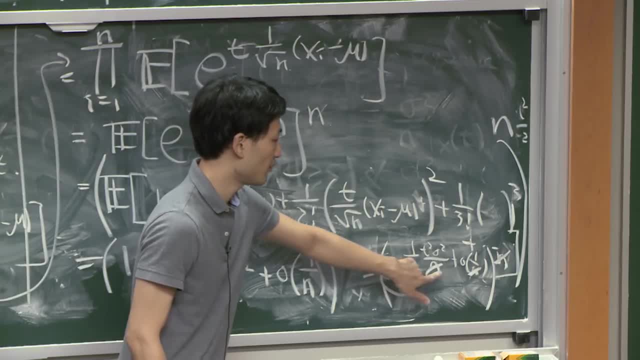 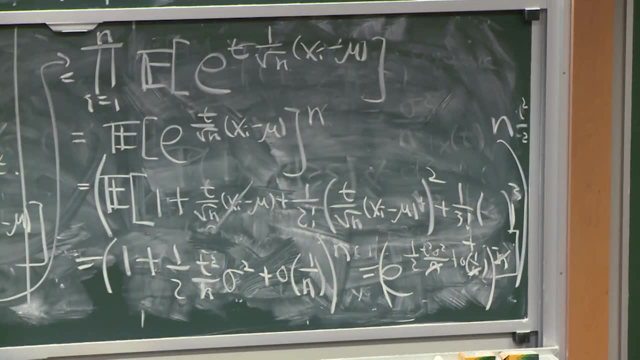 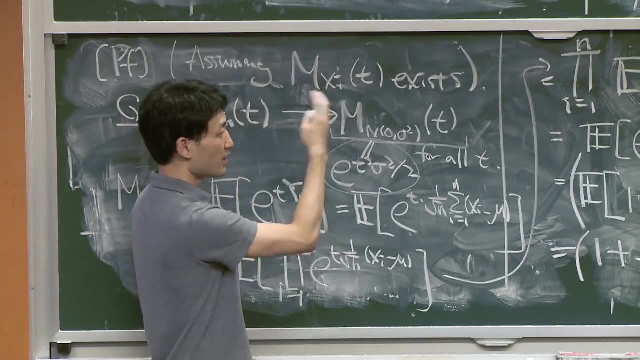 And we see that it's e to the t squared sigma, squared over 2, plus a little over 1.. So if you take n to go to infinity, that term disappears And we prove that it converges to that. And then, by the theorem that I stated before, if we have this,